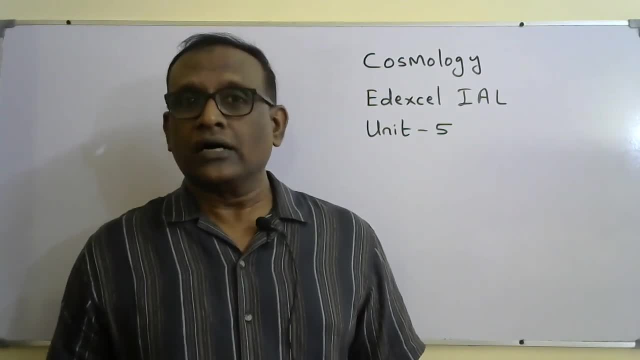 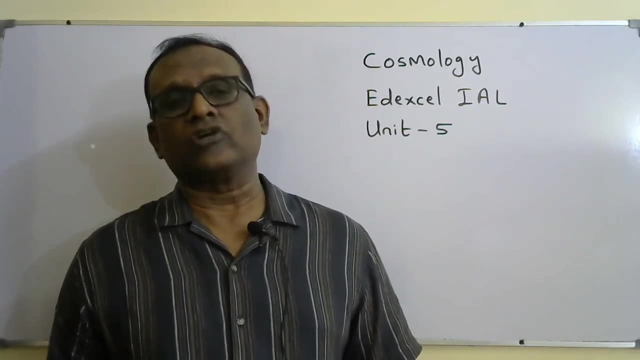 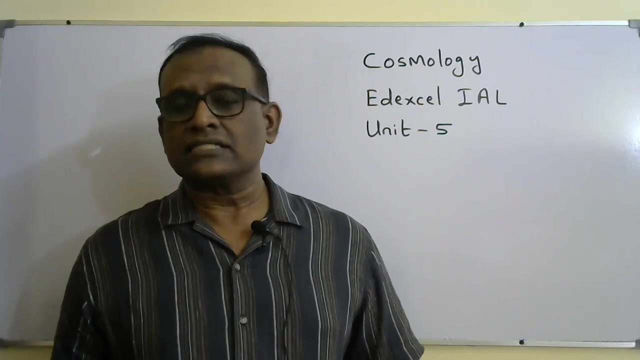 real world applications. but you know, all the study or complete studies related to cosmology depends on the light we receive from the star or star cluster galaxy. the light that we receive from these stars or star clusters or galaxies are older light. you know. the light from Sun takes almost eight. 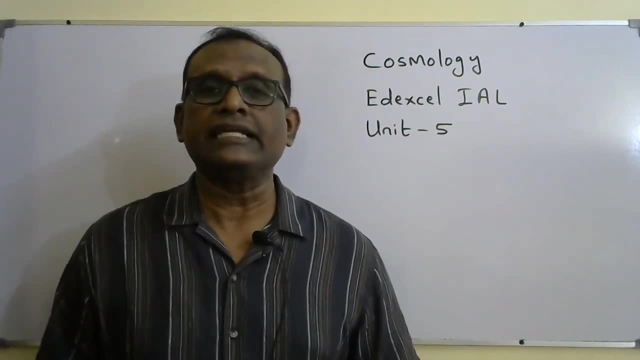 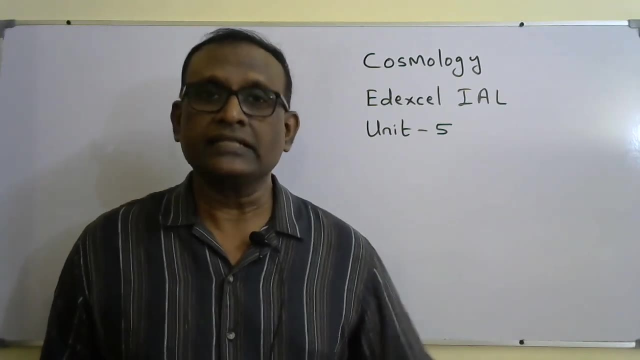 minutes to reach us. that means the light that you see now was emitted 8 seconds. Smart people know why. will light from day one reaches us? There are minutes ago, like that, the nearest star to earth other than the sun is the alpha century. but the light from the alpha century 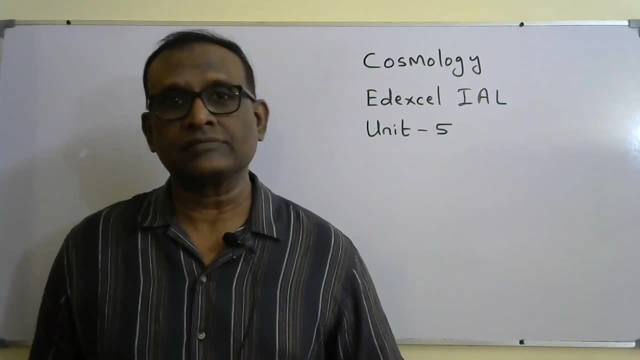 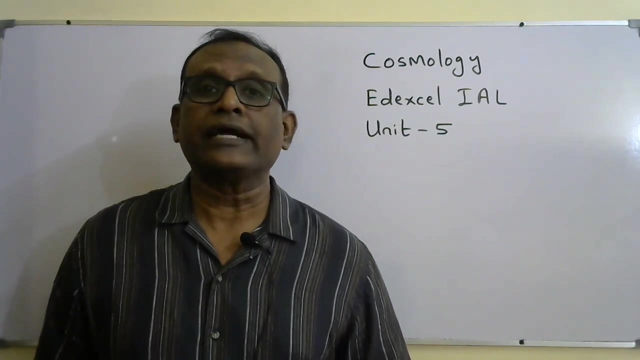 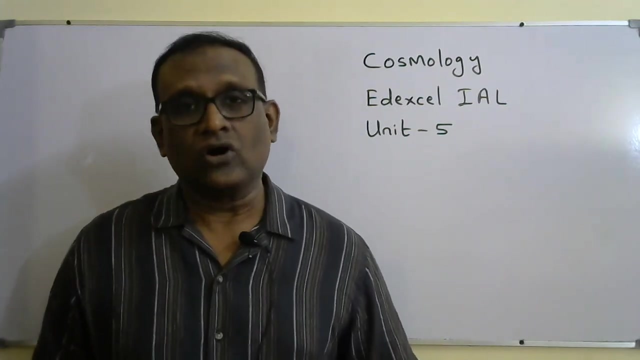 takes almost 4.35 years to reach us. so the light that you see now, which is was emitted from the alpha century, was emitted almost 4.35 years ago. by using very powerful telescopes, scientists are able to receive light or be able to see light from. 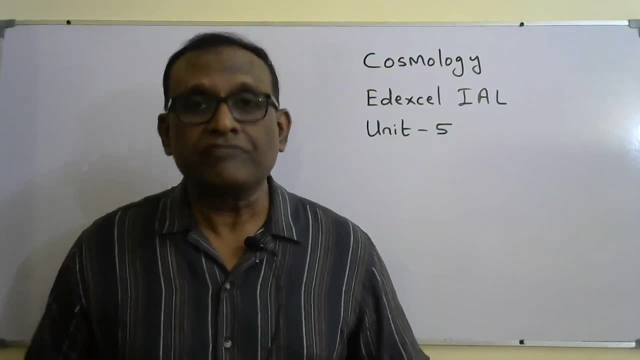 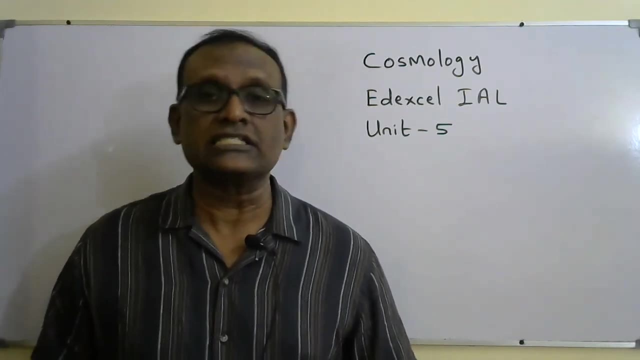 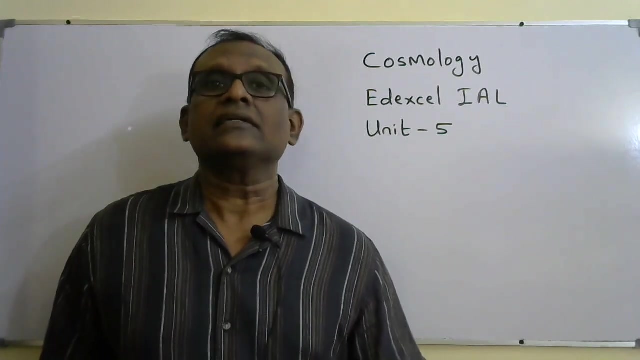 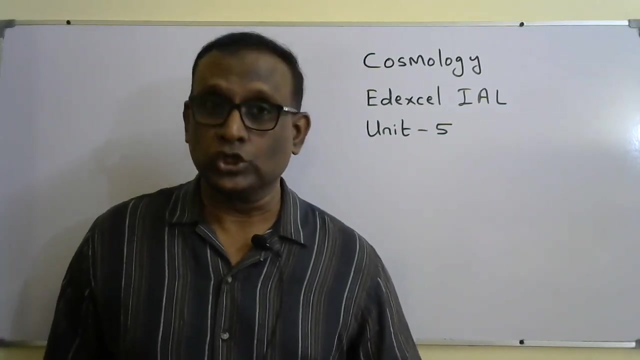 several billion light years away from us. light year means the light that travels during one year. the distance the light travels during one year is called light year. so if scientists can see stars several billion light years away, means that light was emitted billions of years ago. so by using the spectrum of these lights, 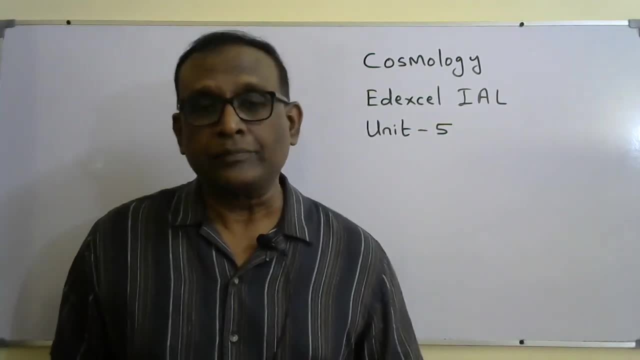 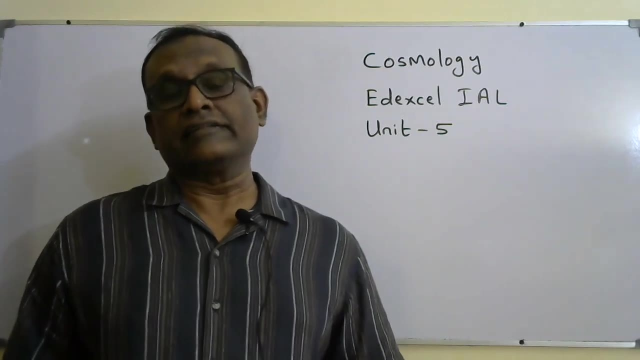 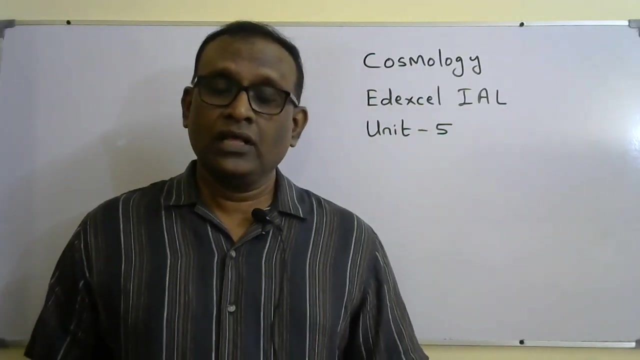 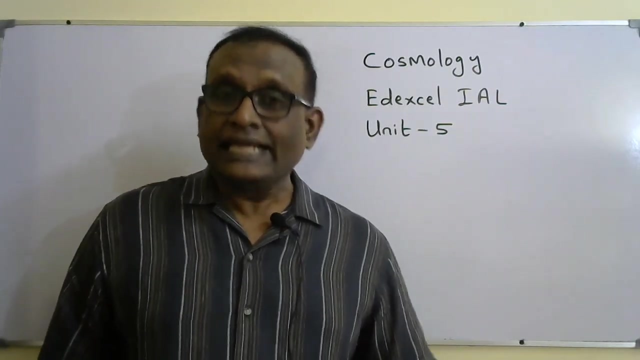 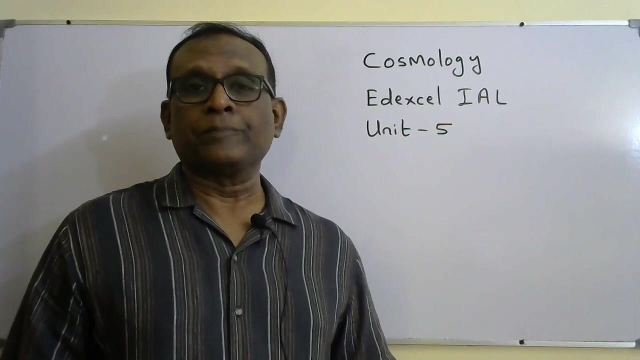 scientists are able to analyze what happened several billions years ago, how physics principles are involved in the creation of universe, how physics principles evolved or changed during several billions years ago. also, scientists can analyze how energy matter interacted during those periods, that is, several billions years ago, or you know that actually the 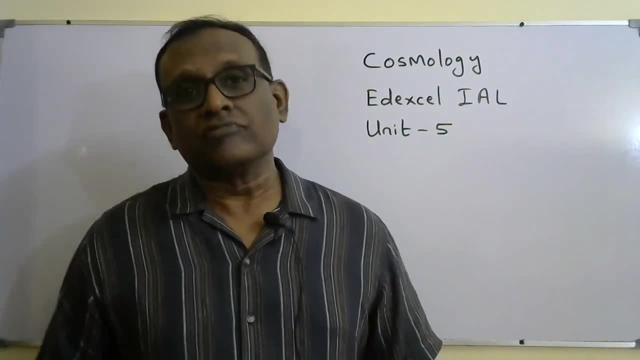 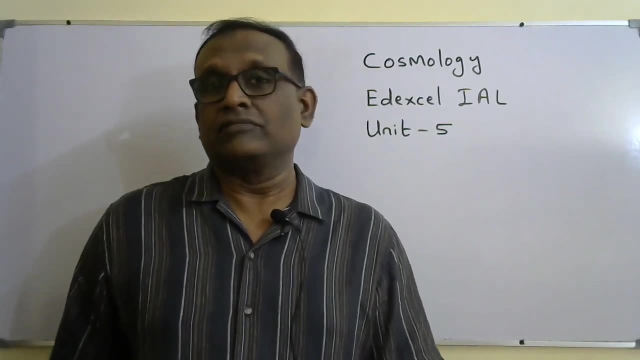 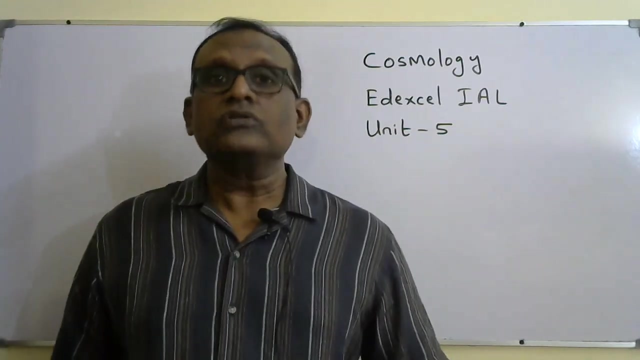 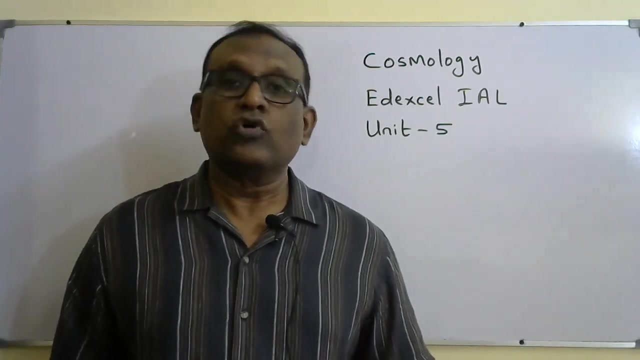 universe is a. actually it's a natural laboratory for scientists to test certain experiments. that means like a critical, like a very critical situations, like very high temperature, very high pressure, how these physical physics principles behave during these situations. so normally the laboratory we won't be able to create such very high temperature, very high. 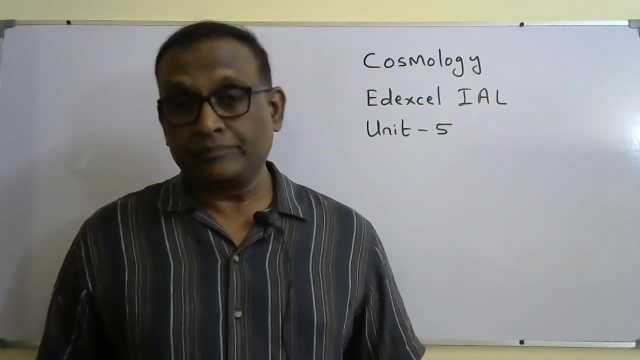 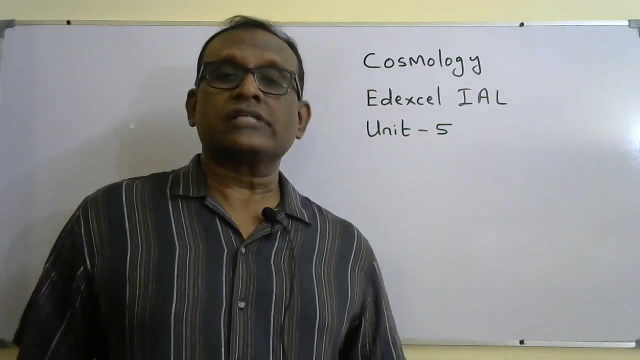 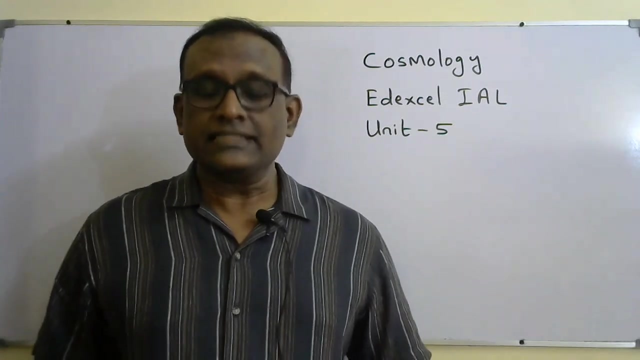 pressure, but naturally these physics principles are about basic level of, but naturally it exists during the Big Bang or even after the Big Bang. Also, scientists can predict what could happen in future, what could be the fate of the universe. So like this cosmology, actually something related to research in that 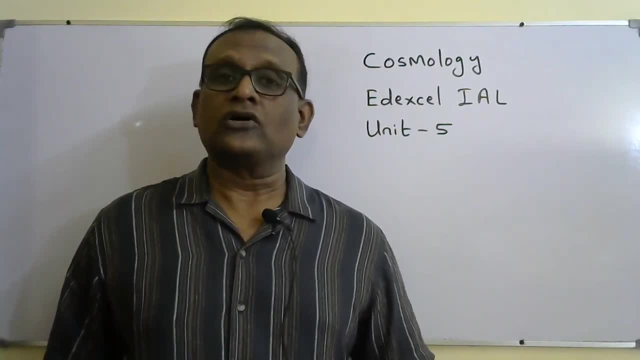 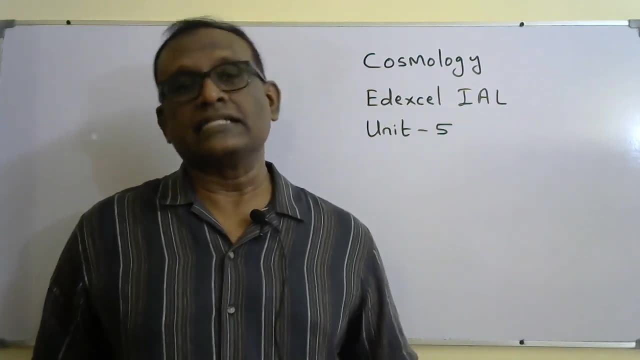 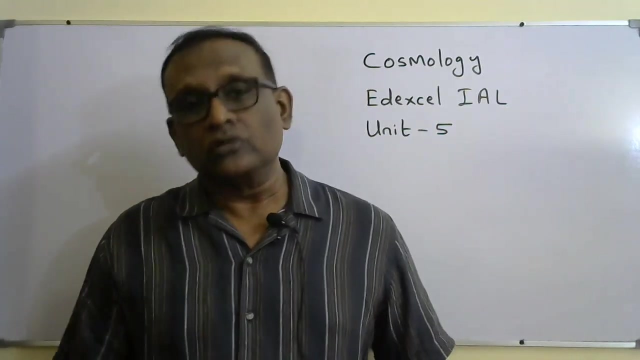 way. it's an important study because you know, all the physics principles were created after the Big Bang. So scientists are interested about how the physics principles are changing during several billions of years ago or how their physics principles could change in future. there are researchers going on. 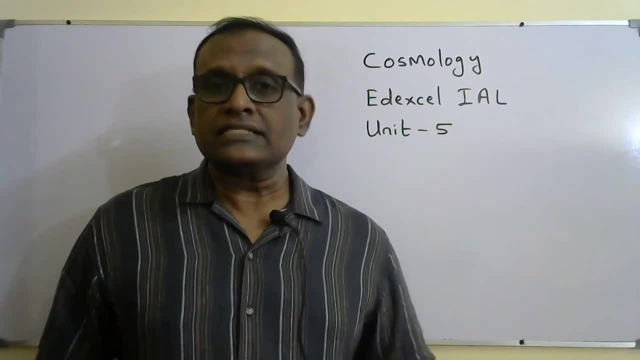 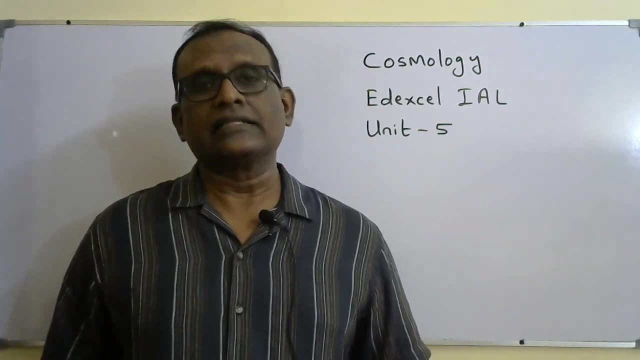 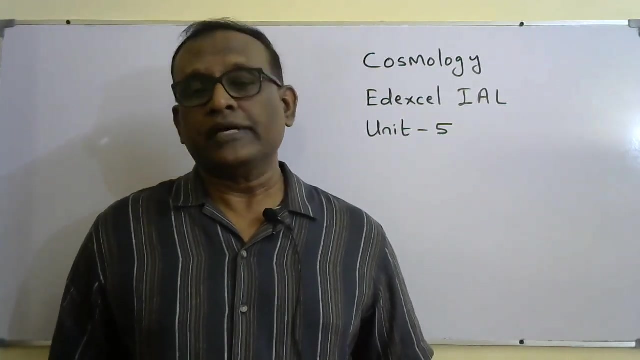 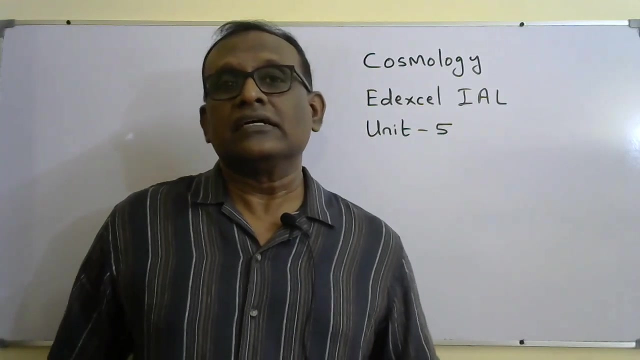 like that. So in taste about that is Unified syllabus. we mainly focus on measure of certain measurements. that means how to measure the temperature of a star, to measure the luminosity of a star, or how to measure the distance of different stars, galaxies, and how the lifespan of a star changes. those are the things we are going to learn, because 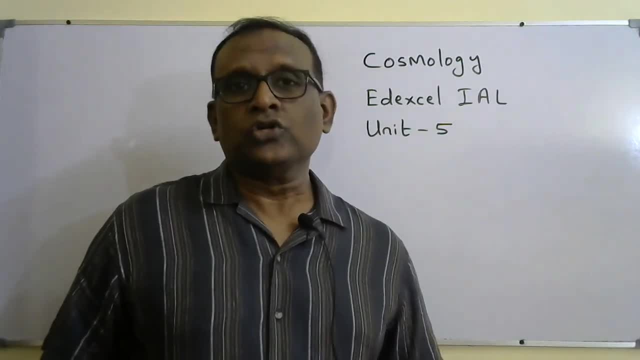 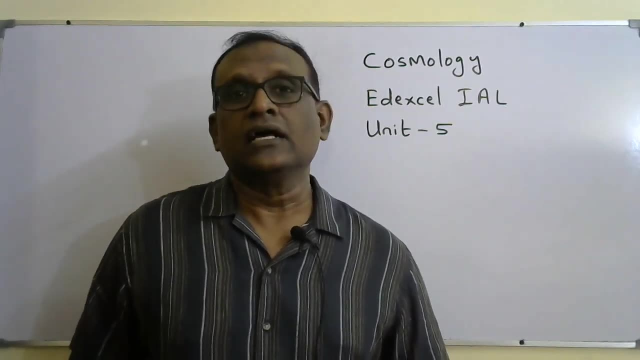 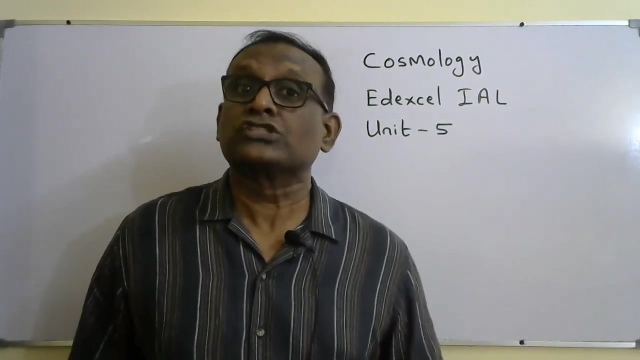 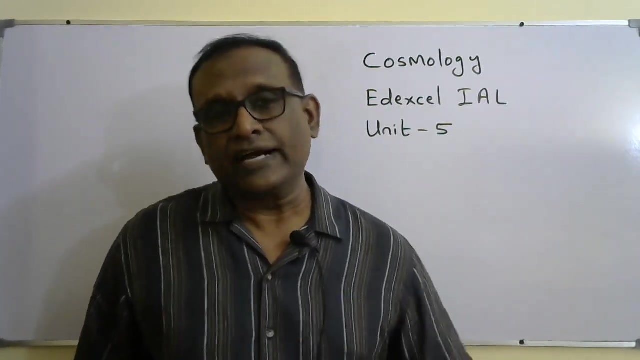 actually we are not going to learn the real cosmology. to learn the real, actual cosmology you should have very good knowledge in thermodynamics, special theory of relativity, general theory of relativity, then about electromagnetic wave theory, everything you should have. you should have good knowledge in those things, but in unit 5, syllabus you don't. 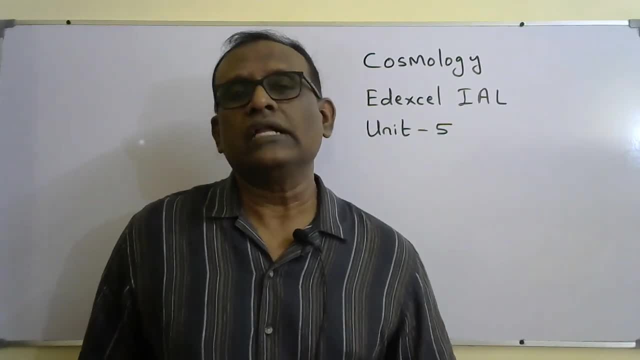 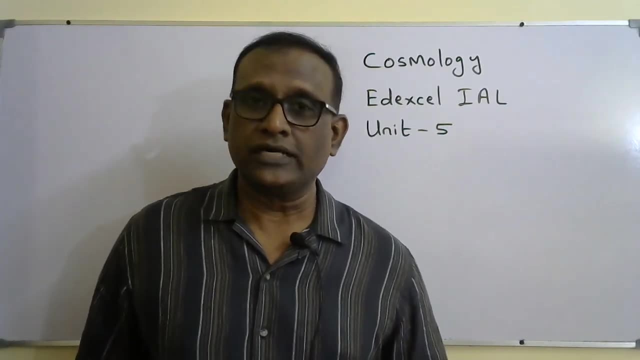 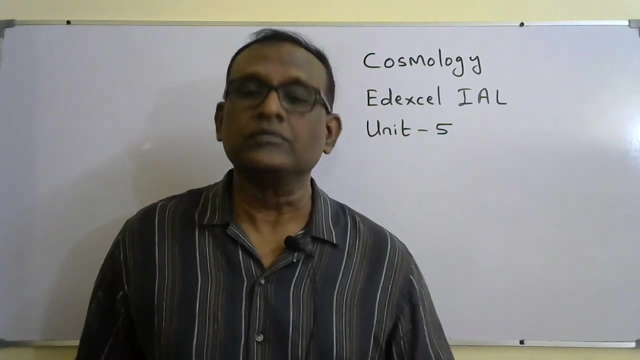 need to worry much. it's actually we are using only three laws and, uh, doppler, three laws means we are using stefan boltzmann law, wien's law, those two laws nothing related to cosmology. they are actually related to cosmology, actually to the Stefan-Boltzmann law and Wien's law. both are related to blackbody. 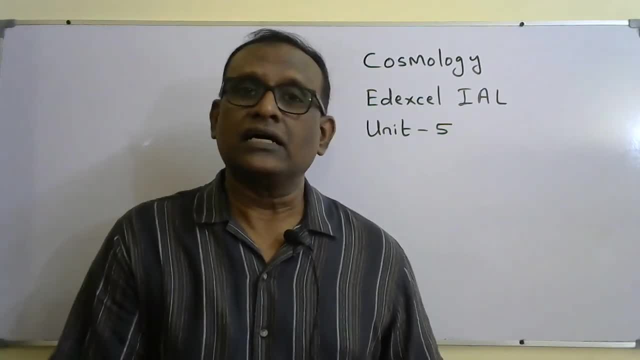 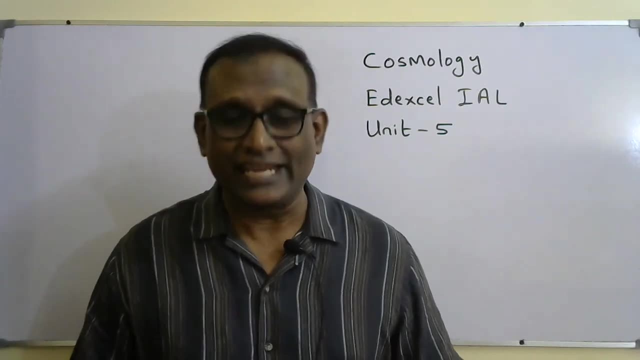 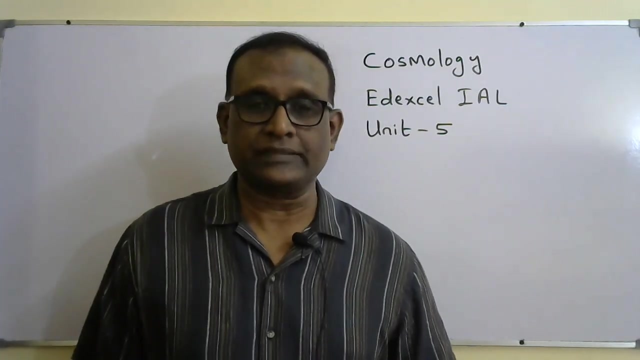 radiation- nothing related to cosmology. same way, Doppler effect or Doppler shift, that is that also nothing related to cosmology. that is related to waves, how the wavelength and frequency changes when an observer and the source has related motion. so only one law we are learning, related to cosmology, that is. 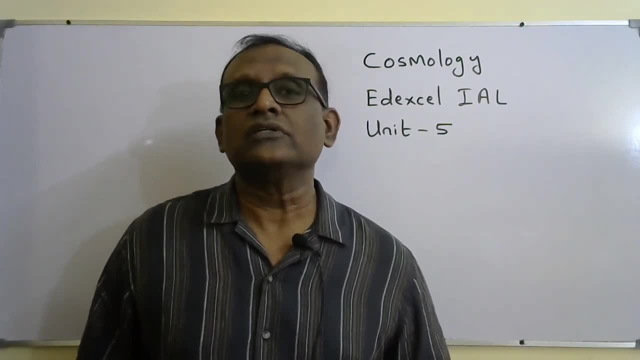 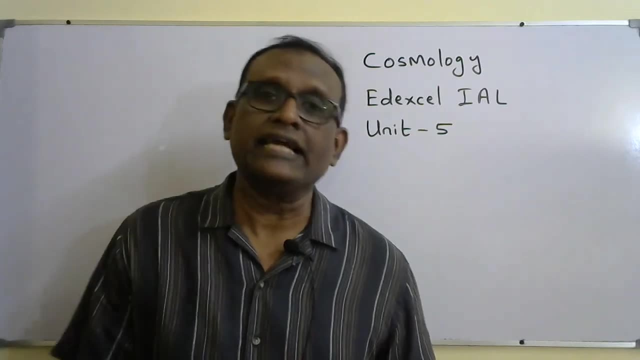 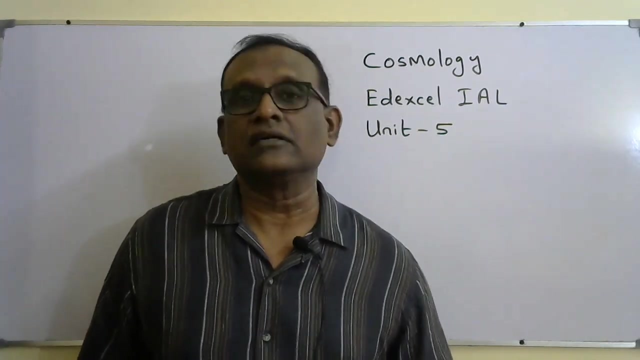 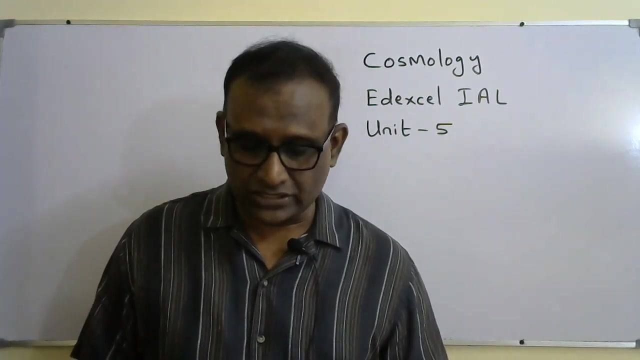 Hubble's law. other than that, we are trying to do certain measurements in unit 5 syllabus by using the physics principles or the laws they are related to some other, like some other physics principles like wave theory or something like blackbody radiation, so there's nothing to worry about cosmology. 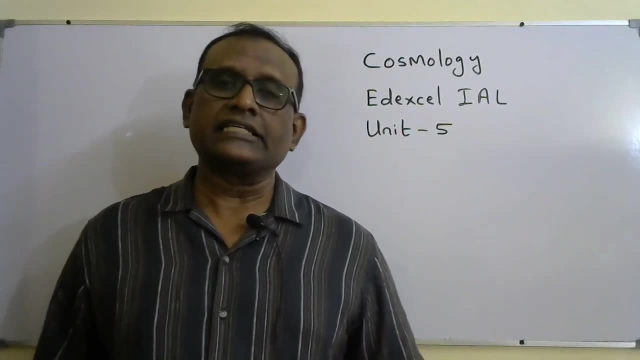 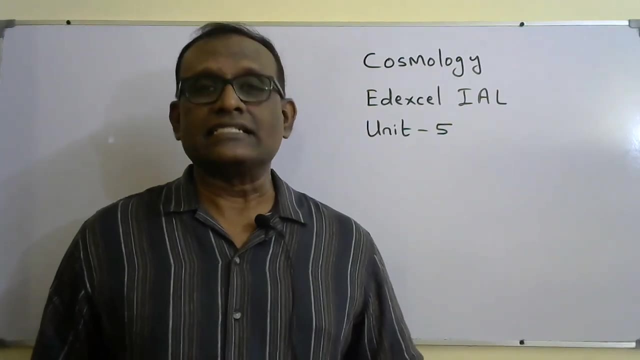 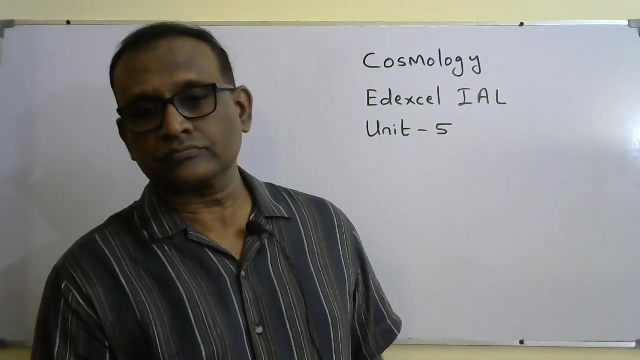 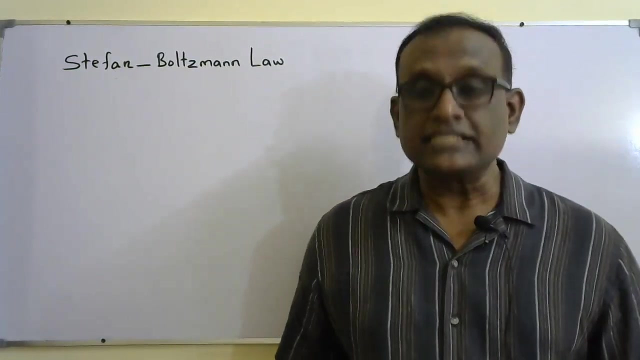 the questions are the calculations related to cosmology also based on only these equations? additionally, there could be calculations related to intensity. I equal L over 4 pi d squared, so that you already studied in unit 2. okay, so the first law that we learn in this topic in 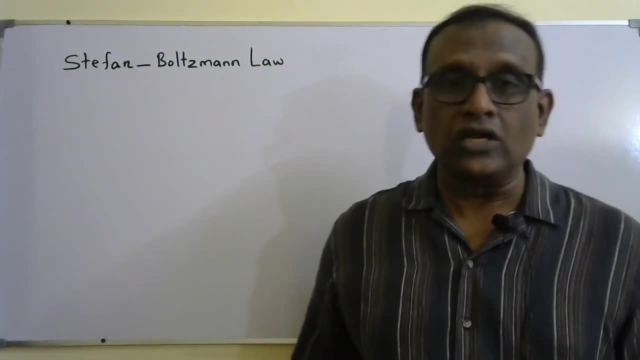 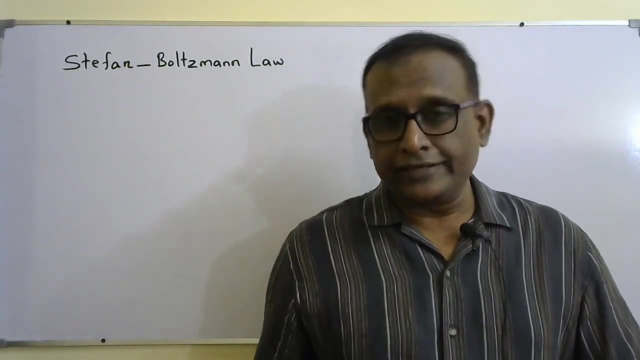 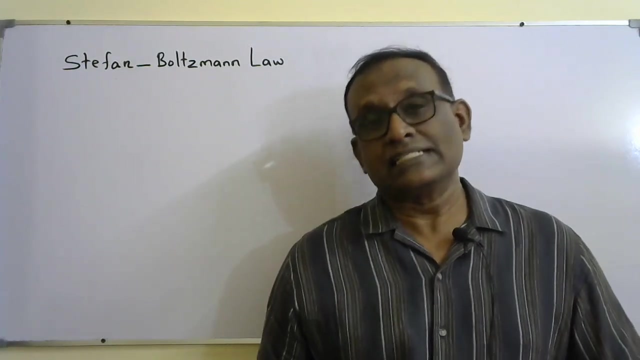 unit 5 under cosmology is Stefan-Boltzmann law. I already told that Stefan-Boltzmann law nothing related to cosmology, that is related to black body radiation. so what is black body? black body means it's a physical object or physical system or an object that absorbs all the. 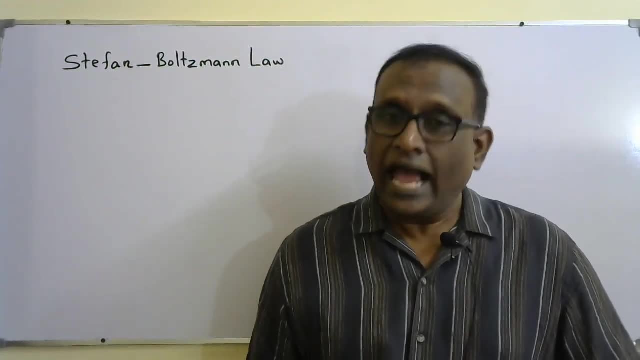 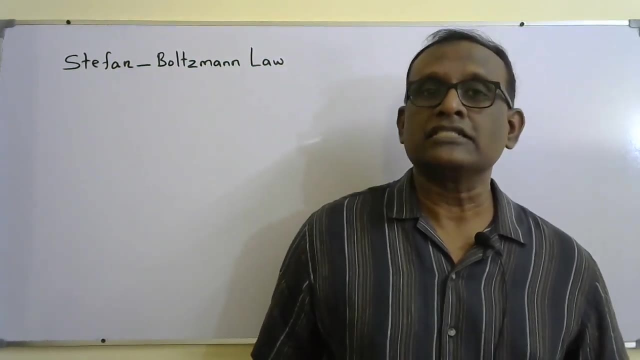 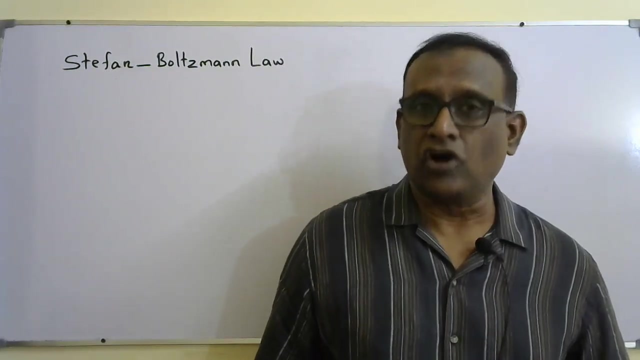 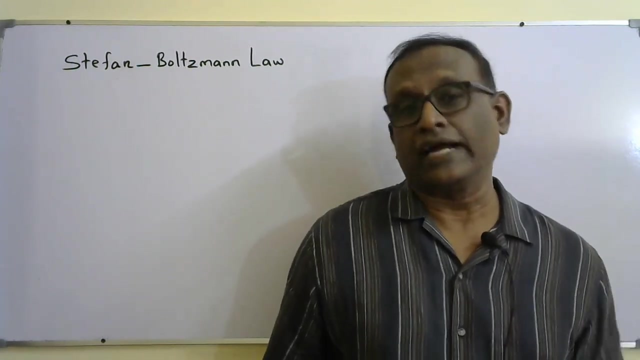 radiation- electromagnetic radiation- falling on it, and it emits radiation depending on its temperature. so black body is should be a perfect absorber. it should absorb all the chromatic radiation falling on it and it emits radiation in a wider range, with a wider range of wavelength, and the distribution of the radiation should be. 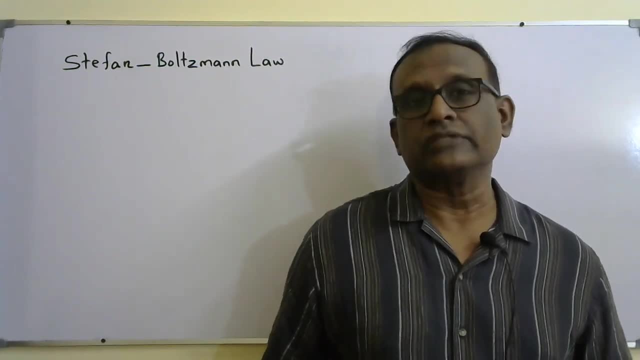 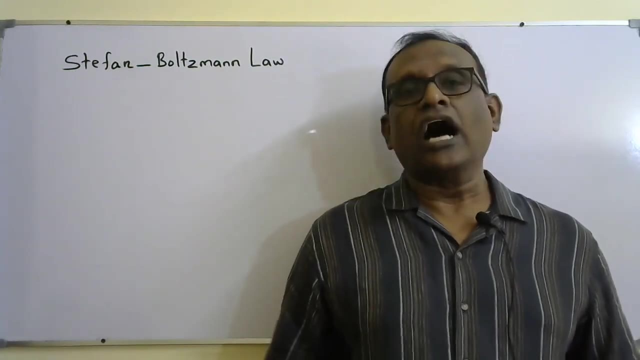 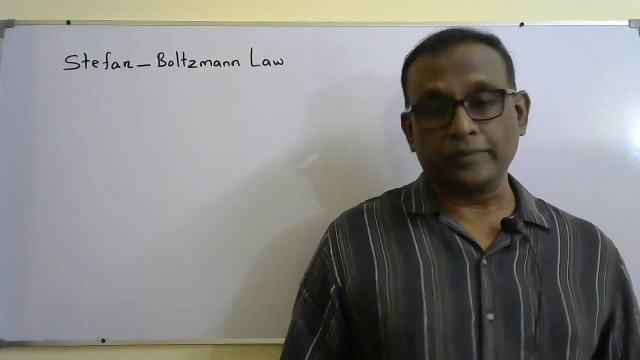 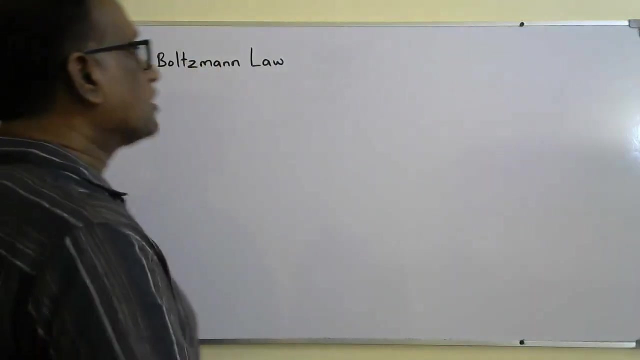 governed by the temperature. so that is the black body, right. so the stiff Boltzmann law relates the luminosity, how the luminosity of the radiation emitted by a black body depends on certain properties of the black body. so luminosity means power of the radiation is called luminosity, so luminosity is. 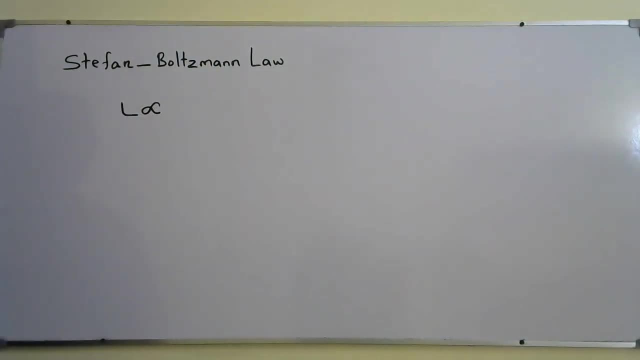 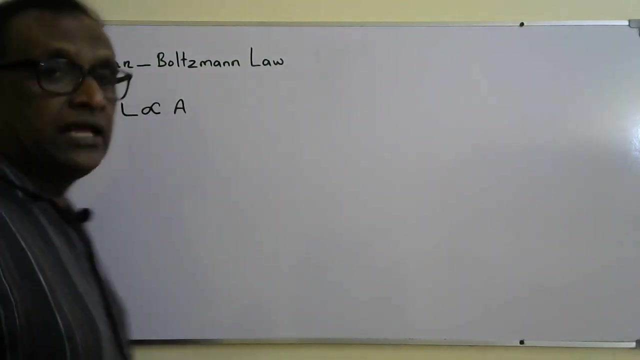 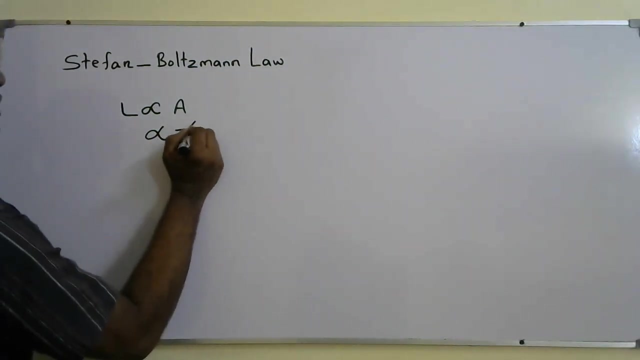 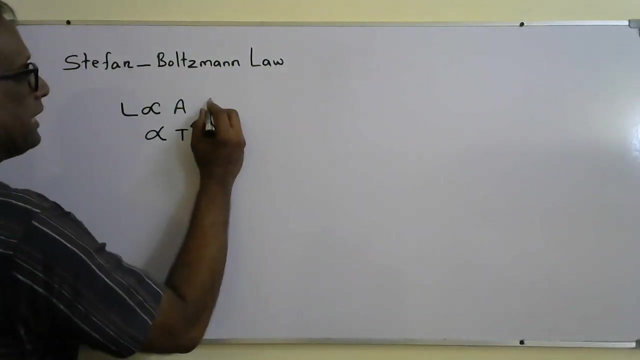 denoted by L. so luminosity. the Stefan Boltzmann law says that luminosity is directly proportional to the surface temperature of the sorry surface area of the black body. also it's directly proportional to the power 4 of the absolute temperature of the black body. so when we combine these two things it will become 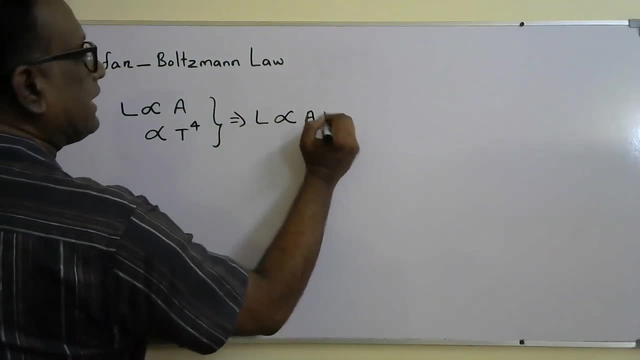 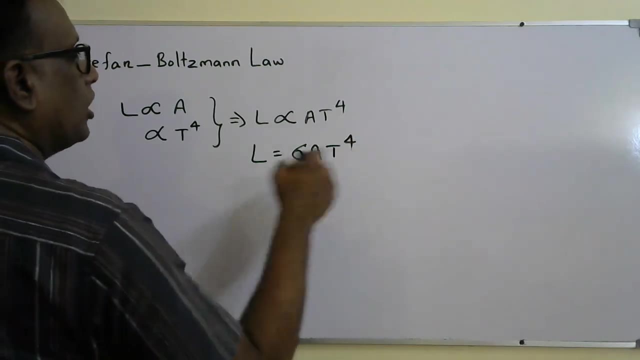 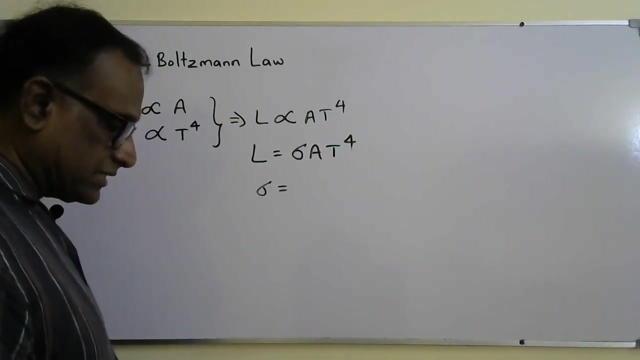 the luminosity is directly proportional to a t to the power 4. so when we convert this to an equation, L equal sigma, a, t to the power 4. where sigma is called Stefan Boltzmann constant, it has a value. the sigma value is equal to that's given in. 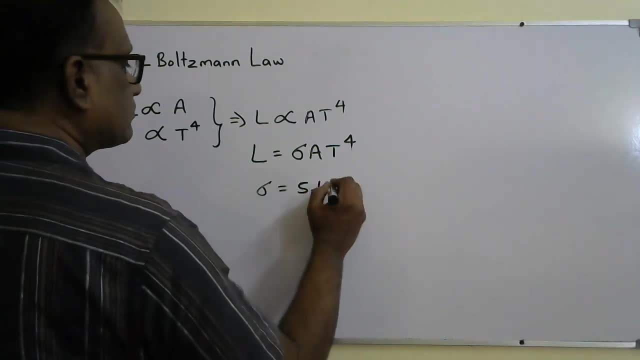 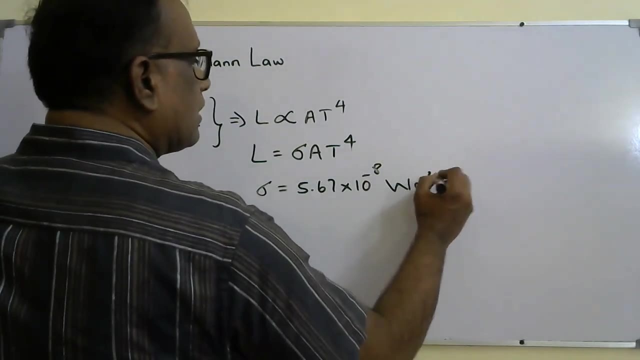 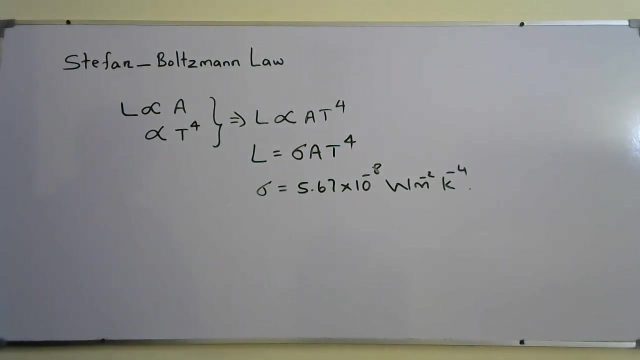 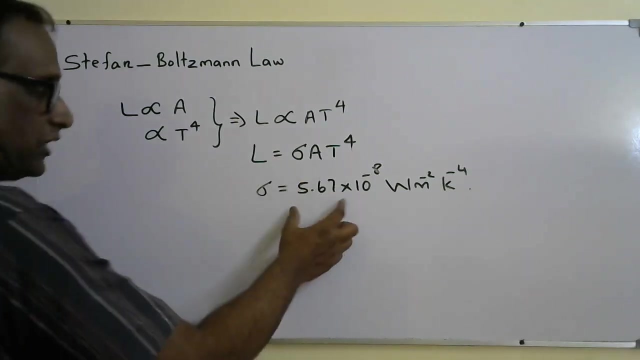 the data sheet. five point six, seven into ten to the power four. so this is the value of the value of Stefan Boltzmann, constant. so this is the first equation. so there were calculations based on this equation. so, sigma, we know that. so that's given in the 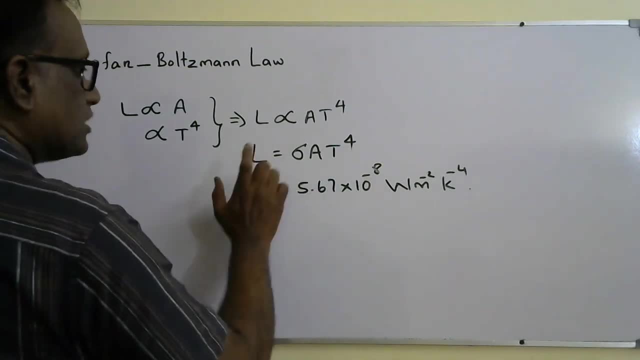 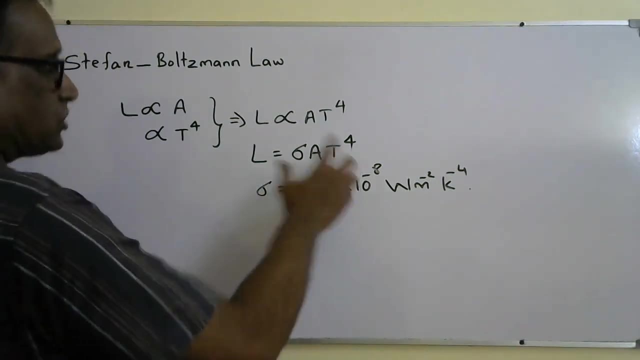 data sheet. so, other than that, there are three other quantities: luminosity, that's the power of the radiation emitted by the black body, A is the surface area, T is the temperature. So out of these three quantities, they'll give any two and they can ask the fourth one. Those 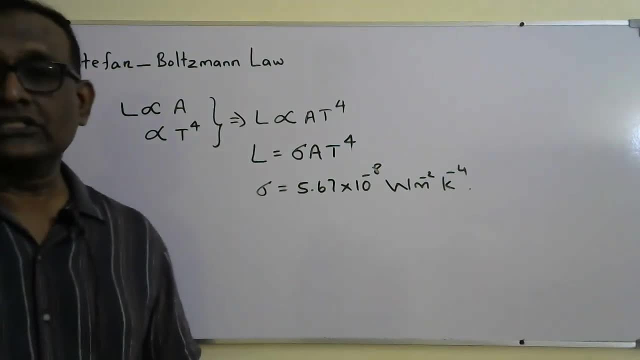 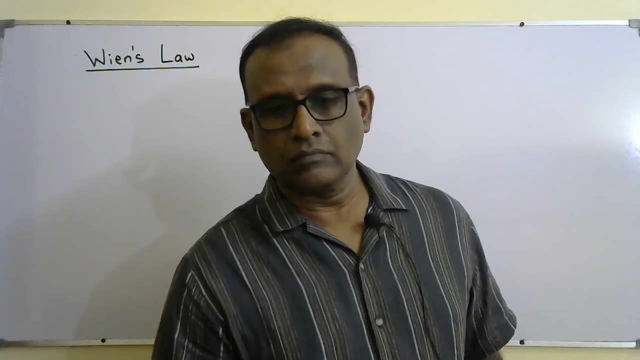 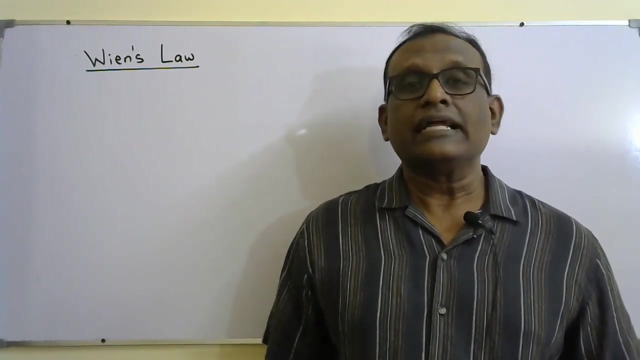 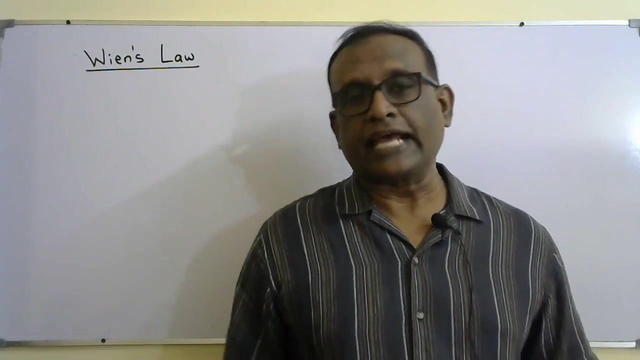 are the questions comes in the past papers related to calculation. Okay, so the next law is the Wien's Law. Wien's Law is also related to black body radiation, So I told that black body means it should be an object or system that absorbs all the. 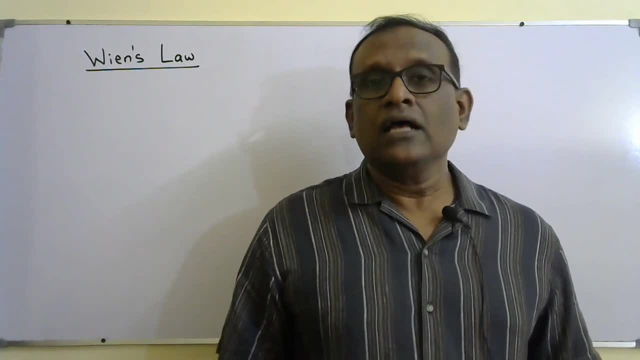 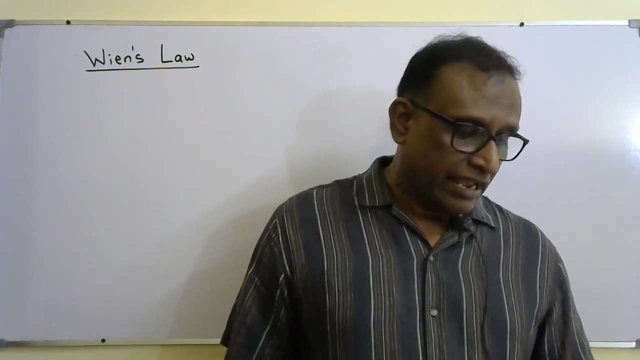 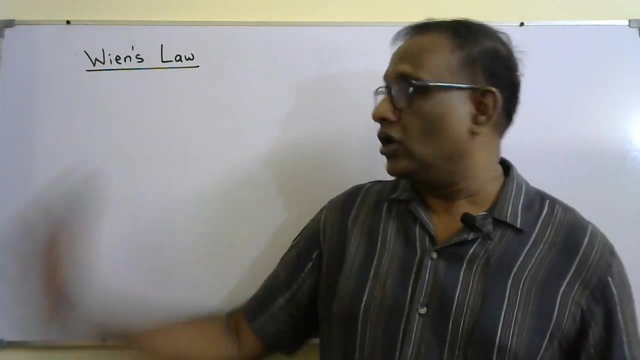 electromagnetic radiation falling on it. okay, Then it should emit radiation, electromagnetic radiation with a range ofzone of wavelength, and that wavelength should depends on the temperature. The emitted wavelength should be related to the temperature. So the Wien's law tells that. 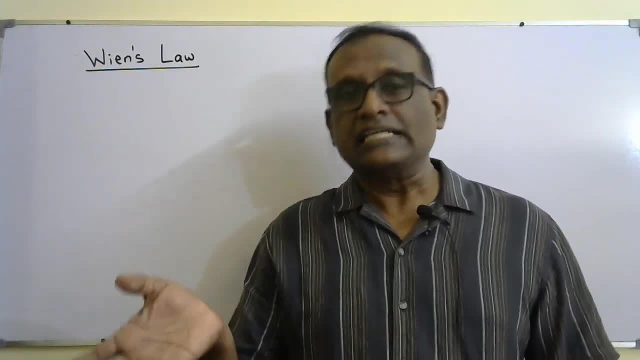 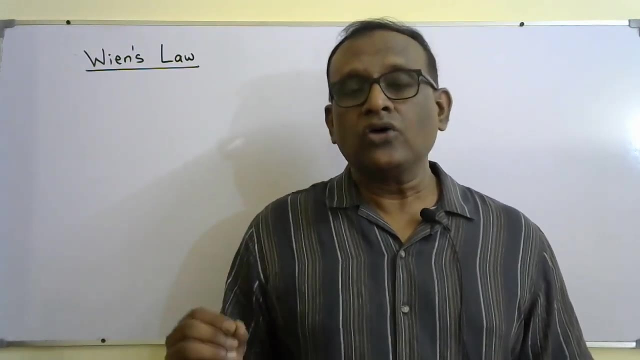 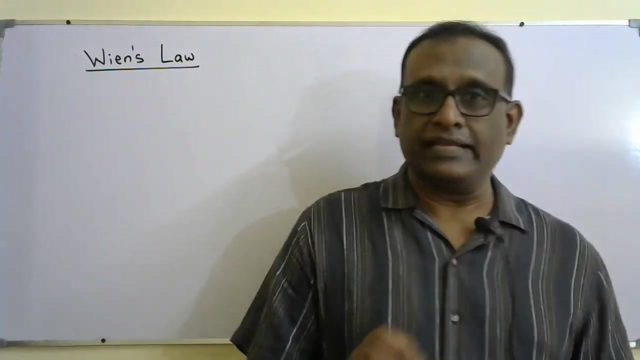 the luminosity of it's actually a curve. that's an equation, is there? but there's a graph. I'm going to show that. That graph shows that how the luminosity of the emitted radiation depends on the wavelength. Say, for example, at a 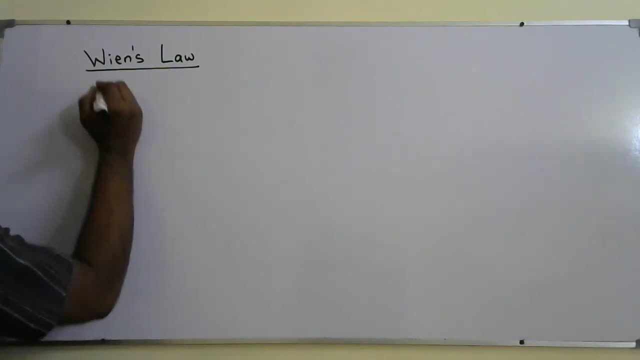 particular temperature if I draw a graph or luminosity against wavelength of the emitted radiation, so at a particular temperature the distribution will be something like this: So that means, at a temperature T1, the wavelength emitted by the blackbody, the electromagnetic radiation emitted by 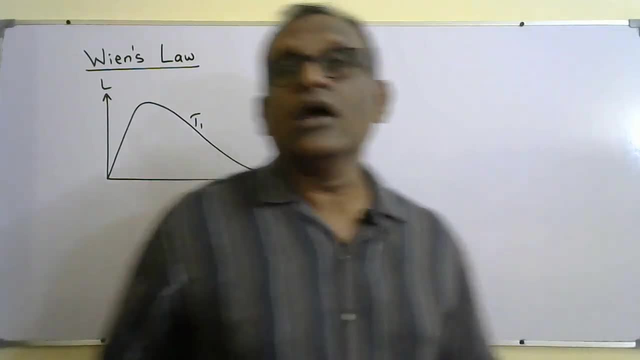 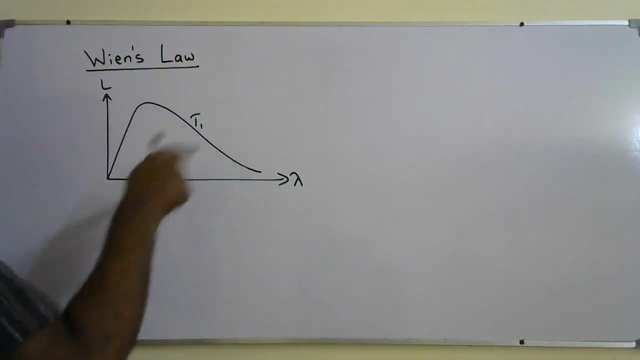 the black body will have a range of wavelength. All those wavelengths won't have the same wavelength. And that wavelength had a range of it must be luminosity. different wavelengths will have different luminosity, so this particular wavelength will have this particular luminosity. this wavelength. 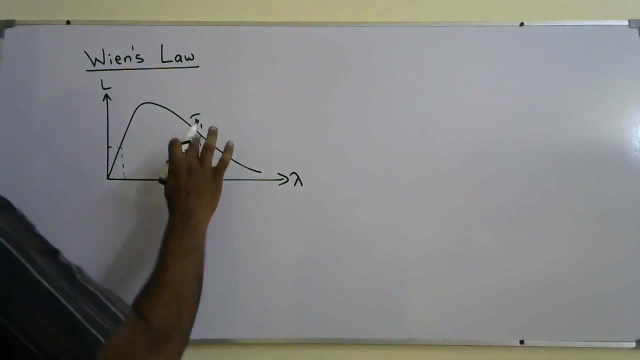 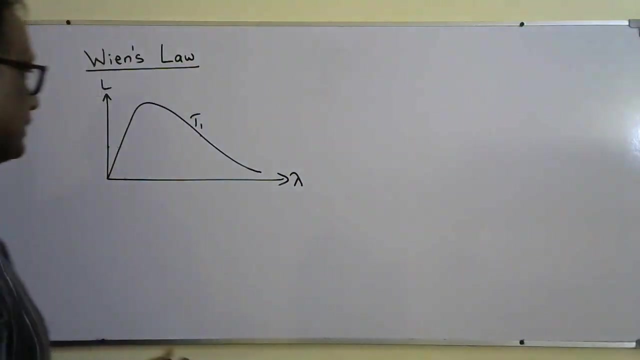 will have some other luminosity. so like that, the luminosity will be different for different wavelengths. also, it says that when the temperature decreases, if you have another blackbody that has lower temperature, what happens? the wavelength that correspond to the peak luminosity will increase. so in this 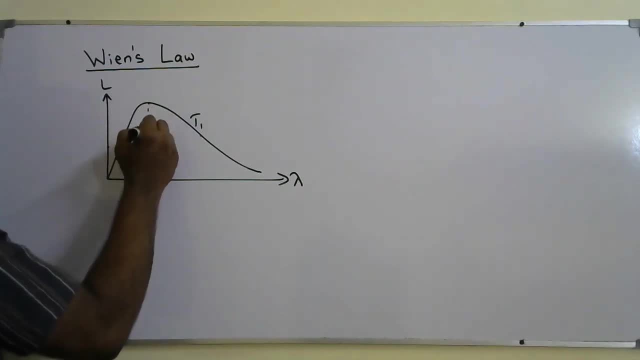 particular temperature T1. there is a wavelength, lambda 1, that gives the maximum luminosity at this temperature. but when the temperature decreases, the distribution curve will become like this: the distribution curve will become like this: so there, at this temperature T2, the blackbody is at a temperature T2.. At this temperature there is a peak luminosity, The wavelength that 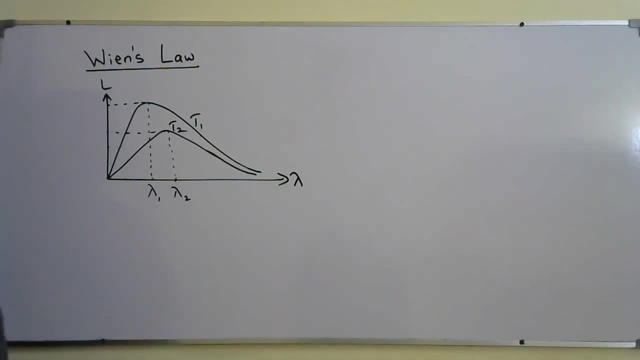 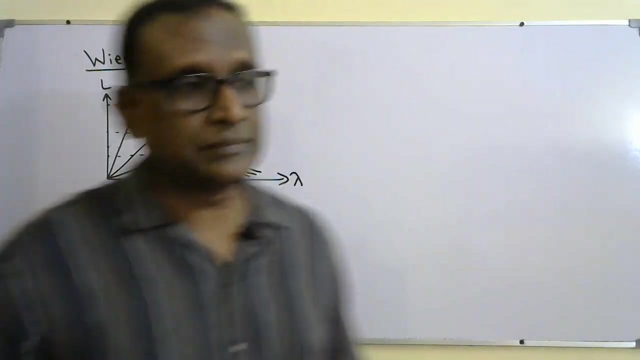 gives the peak luminosity is lambda 2.. So if I consider another temperature, T3, which is lower than T2, so there the diffusion will be like this: The wavelength lambda 3 gives the highest luminosity at temperature T3.. So like that it's a distribution curve. Wien's law tells about how. 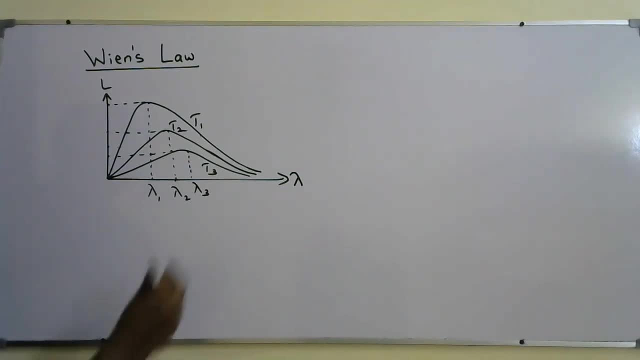 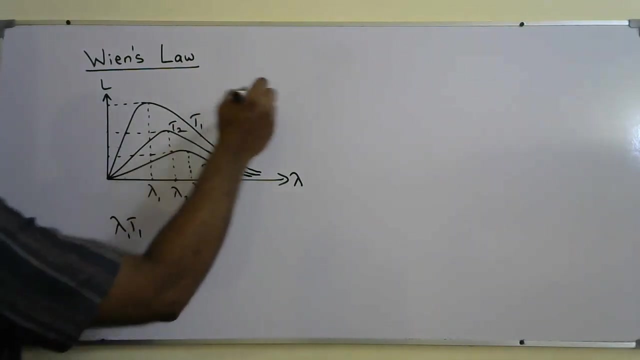 the luminosity varies with different wavelengths of the emitted radiation. So the Wien's law says that lambda 1 times T1, where lambda 1 is the wavelength that corresponds to the highest luminosity at temperature T1. So here temperature T1 greater than temperature T2, temperature T3. 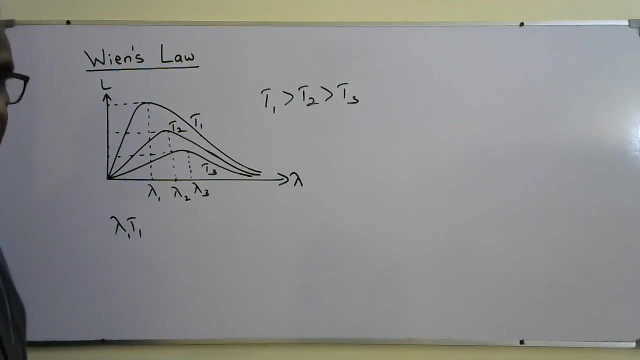 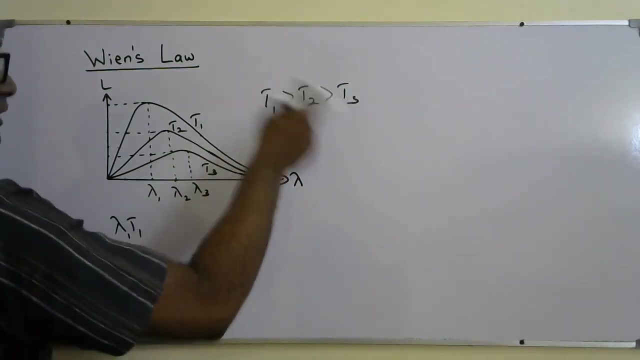 or temperature T3. So T3 is the lowest temperature. T1 is the highest temperature. When the temperature is the highest, the peak value of the luminosity will be higher. You can see the wavelength that correspond to the peak luminosity will become smaller from highest temperature. So when the temperature 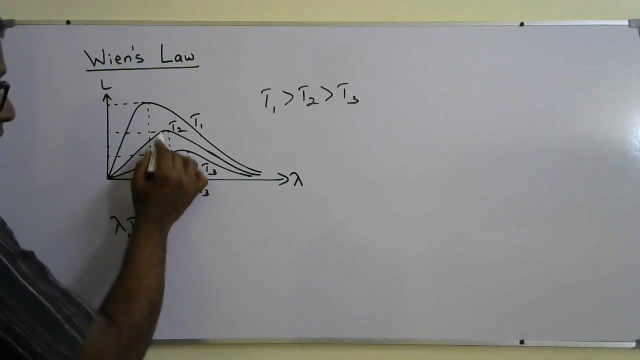 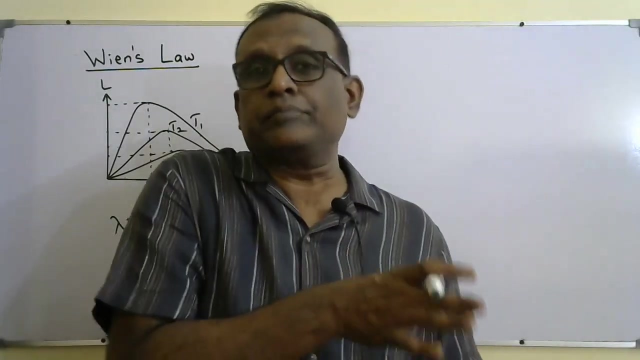 decreases, the peak luminosity will decrease. Wavelength that corresponds to the peak luminosity will increase. he found a relationship between the wavelength that correspond to the peak luminosity and the temperature of the black body. so he showed that lambda 1 t 1 is equal to lambda 2 t 2. 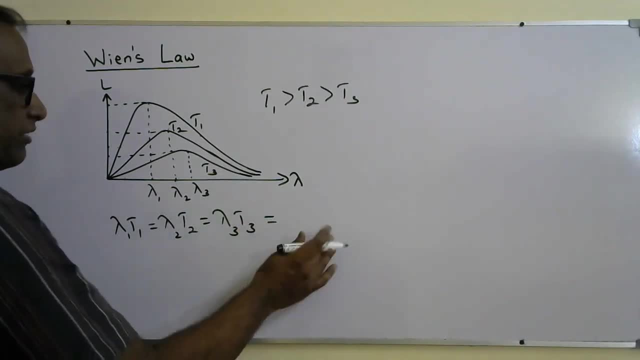 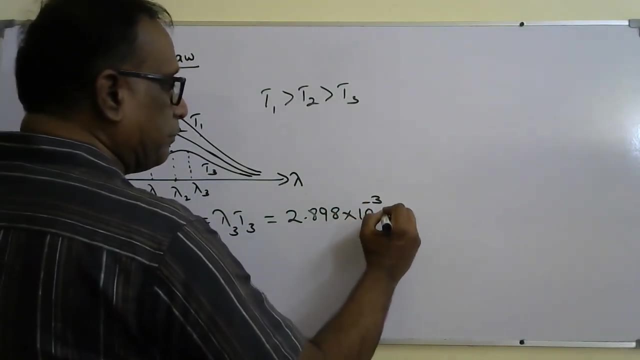 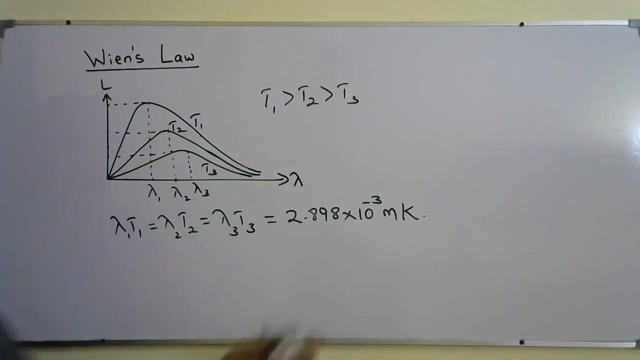 that is equal to lambda 3 t 3. so he found a constant that is 2.898, 10 to the power minus 3 meter. unit of lambda is meter. unit of temperature is kelvin, so meet kelvin. so this is called. this numerical value is called beans constant. okay, so generally we write this: 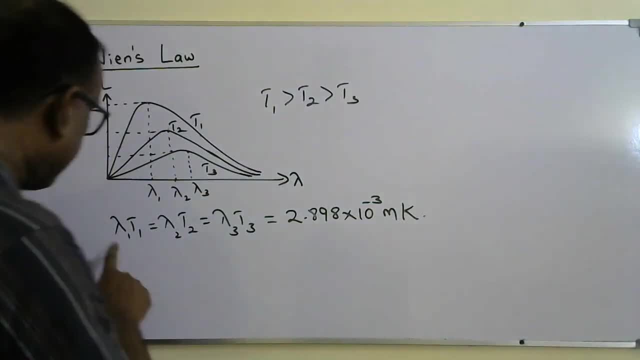 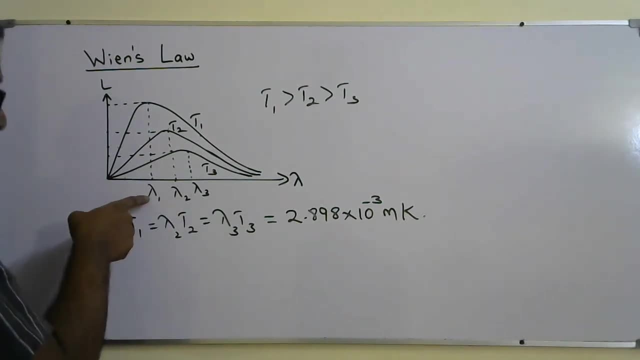 equation like this: so where lambda 1, lambda 2, lambda 3, they all correspond, related to or they are correspond to the wavelength which gives the highest luminosity at that particular temperature. so we write that lambda max. so lambda max does not mean maximum wavelength, the wavelength that correspond to the peak luminosity times. 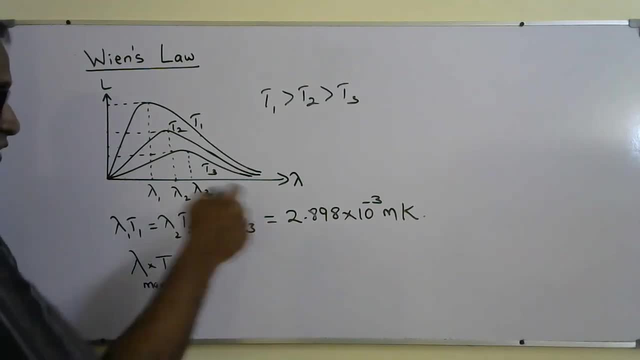 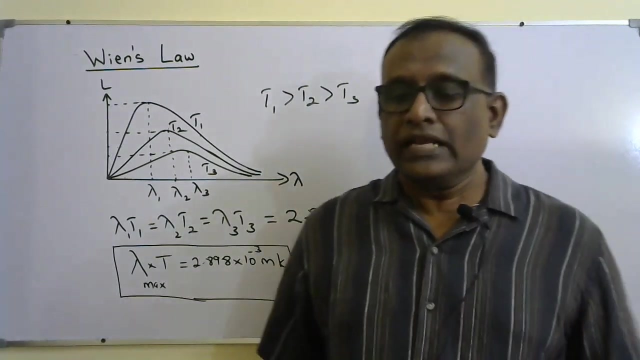 the temperature of the black body is equal to constant, which is two point eight nine eight ten to the power, minus three eta kelvin. so this is the wings law, this relationship is the wings law. so the two laws we learned just now- wings law and Stefan Boltzmann law- both are related to blackbody. 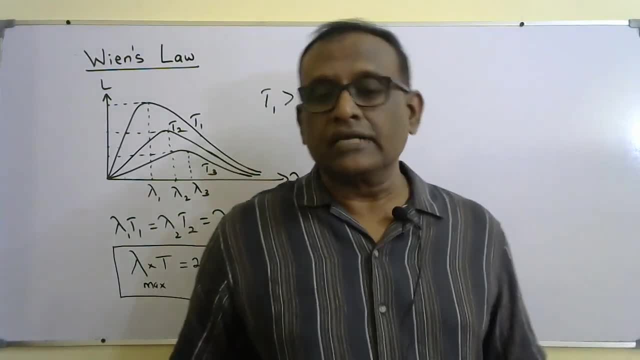 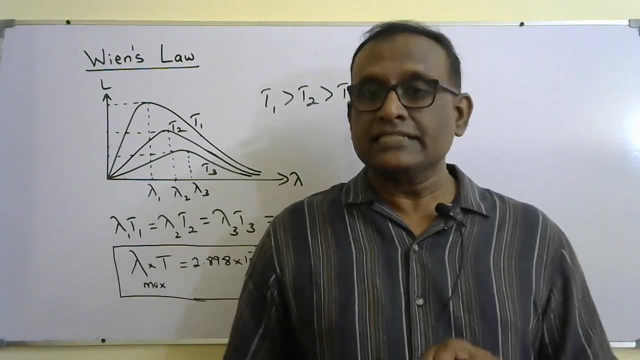 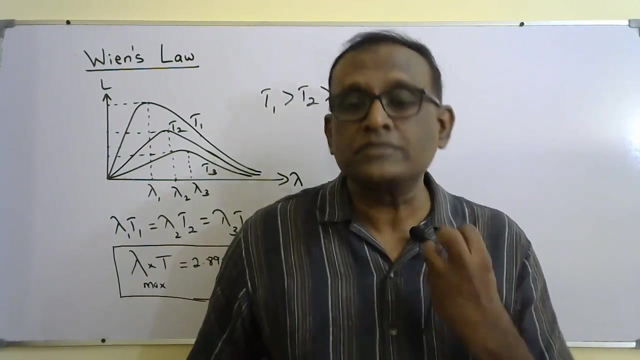 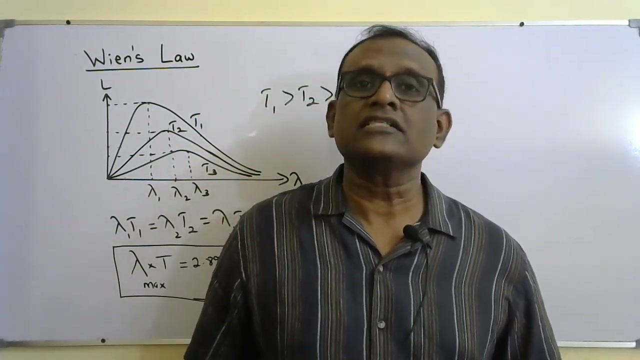 radiation. so can we use this path in cosmology? yes, we can use, because you know, even Sun is a star and many other stars. they behave as almost black bodies. so you know, the sun absorbs radiation. not only sun, even other stars they absorb radiation. so you can ask me: what is the experimental evidence to show that star? 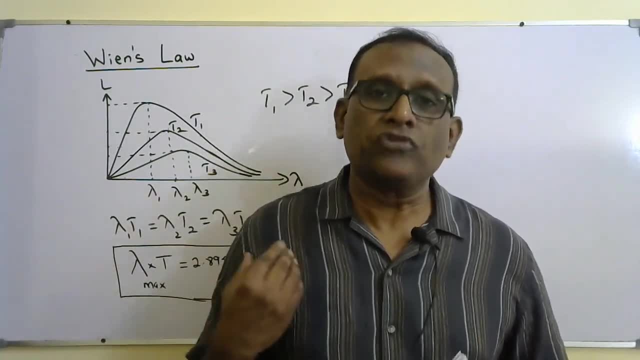 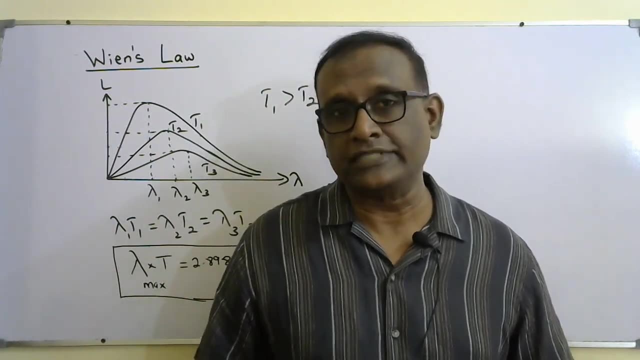 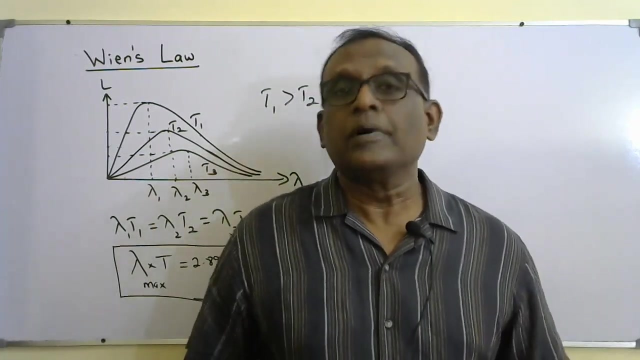 or sun absorbs radiation. okay, if you focus telescope to the sun and receive the spectrum, you know it's a very hot object, so it should give continuous spectrum. hot objects give continuous spectrum. that means all the colors should be there, from violet to red, but there are absorption lines. 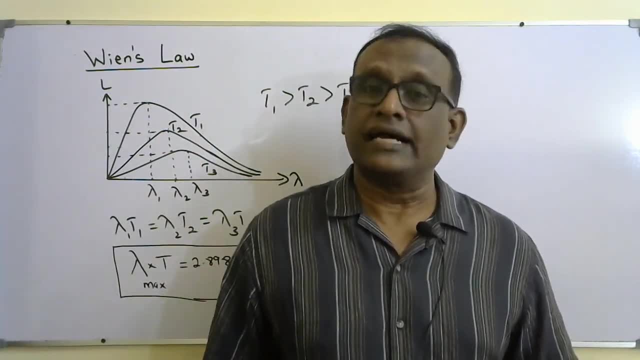 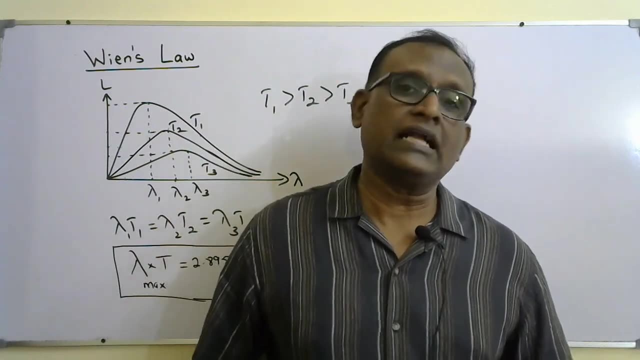 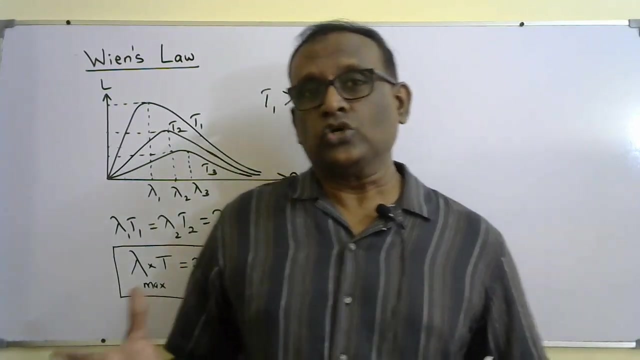 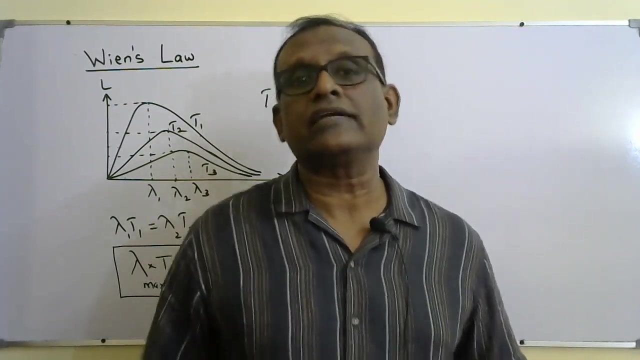 in the emission spectrum of the sun or even from any other stars. when you see the spectrum there will be absorption lines. so those absorption lines depends on the type of gas in the star. so that means that shows sun and other stars are absorbing certain rays of radiation, but they are not absorbing all the radiation, but they are absorbing certain wavelength. 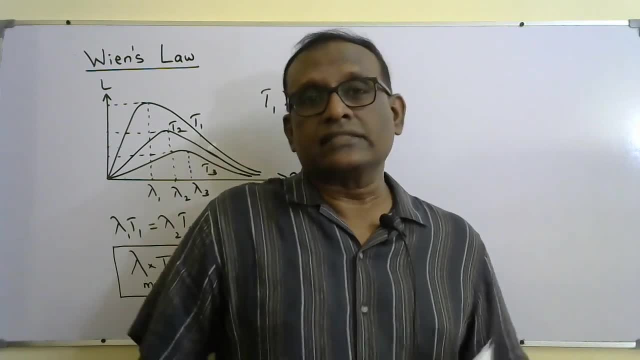 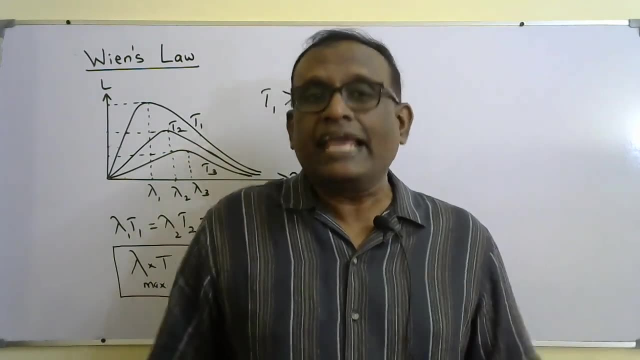 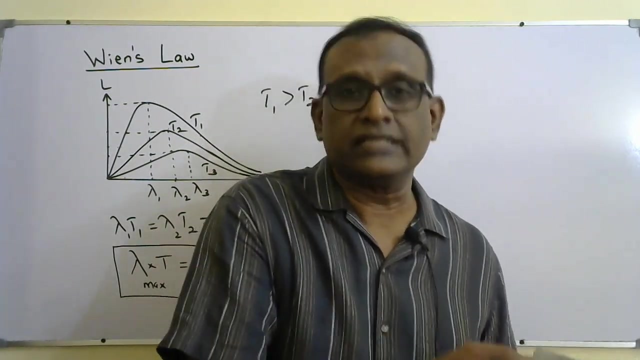 of radiations. so stars, including sun, are not perfect black bodies, uh, so they show certain behavior closer to black body so they are emitting radiation. their radiation emitted from the stars depend on the temperature, so in that way they are not perfect black bodies, but they show certain up. 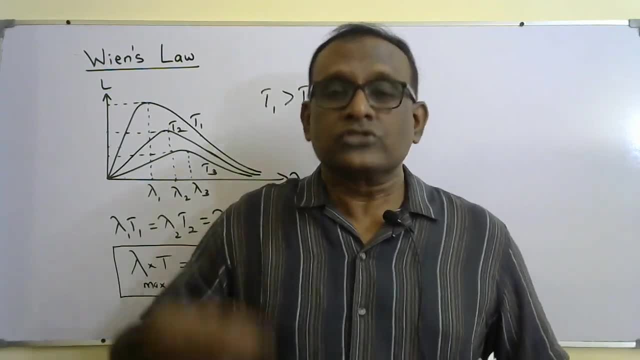 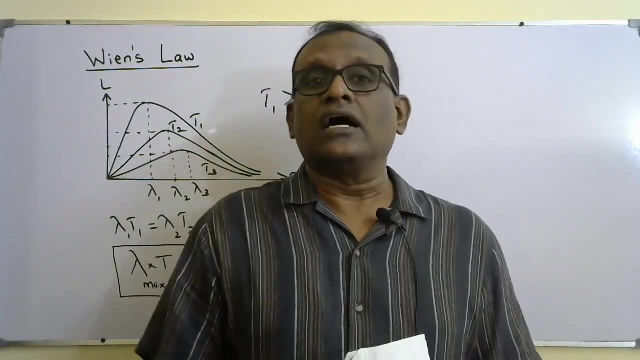 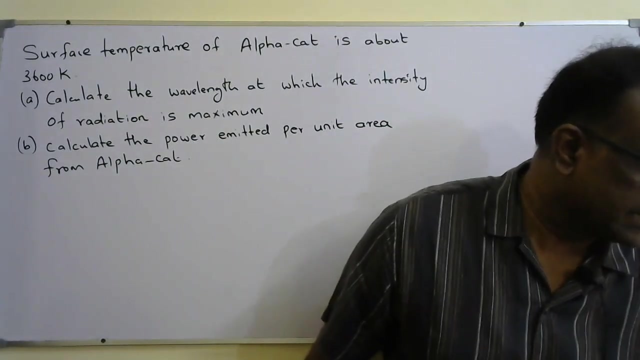 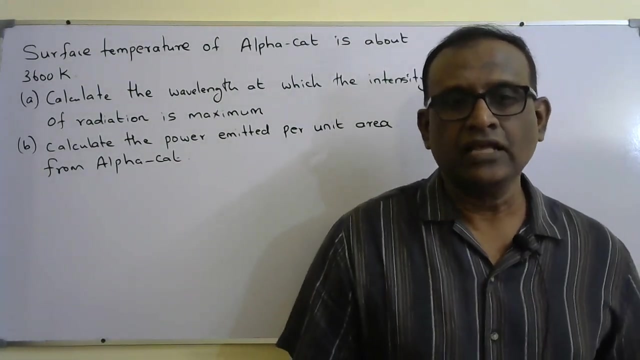 next end they show the behavior of black body. so that's the reason we use Stefan Boltzmann law and Wien's law for the stars, uh, in cosmology. okay, so simple calculations related to these two laws. the first one: surface temperature of alpha set is about 3600 kelvin. 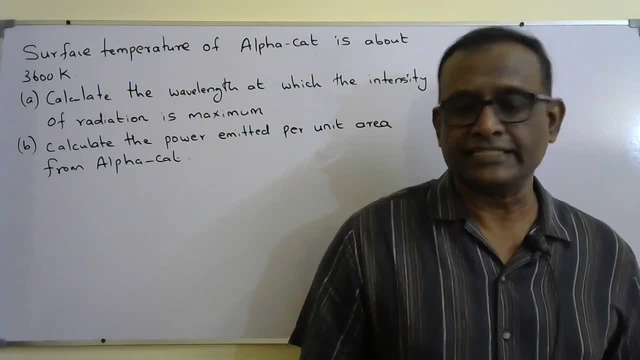 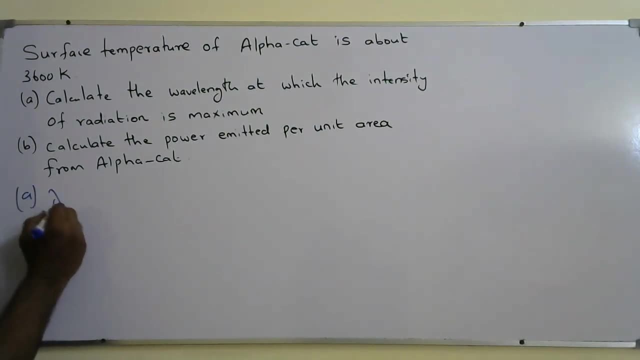 help with the wavelength at which the intensity of radiation is maximum. so to find the intensity of radiation we have to calculate the intensity of the radiation. so to find it we should use the Wien's law, the first part, a part. so i can say lambda max into t equal to 0.898, 10 to the power minus 3 meter kelvin. so i need to find the lambda max. 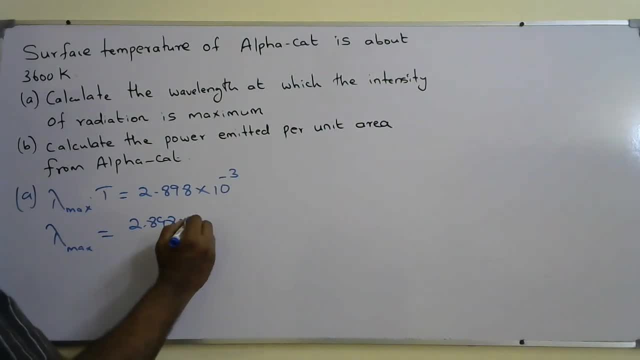 is going to be 2.898, 10 to the power minus 3 divided by the temperature, which is 3600 kelvin. so the wavelength will be equal to the, or wavelength that correspond to the peak luminosity, that will be equal to 8.05. 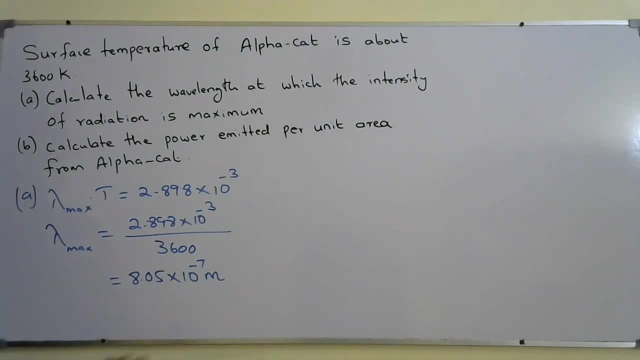 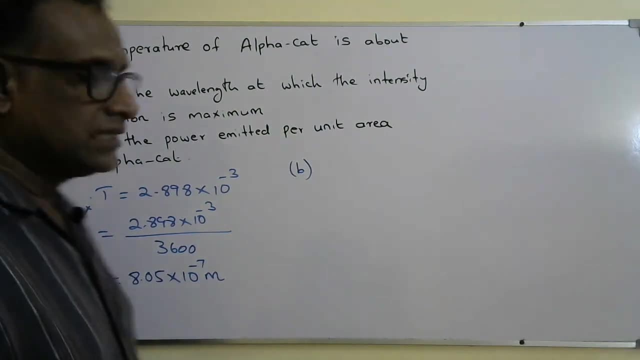 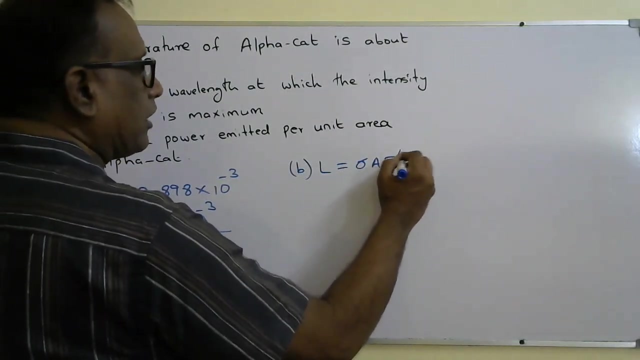 10 to the power minus 7 meter. okay, b part: calculate the power emitted per unit area from alpha set. uh. so that means you know power means luminosity, l equal sigma a, t to the power 4, but the question is: calculated power emitted per unit area, so l over a. 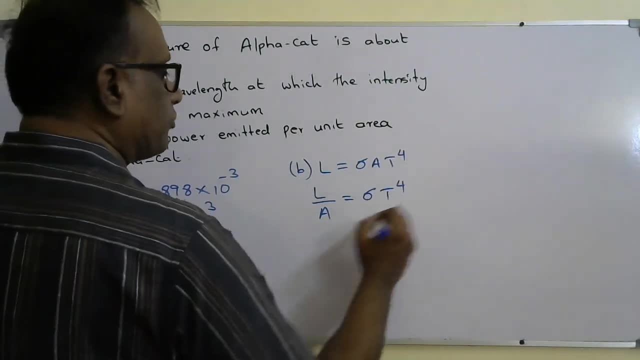 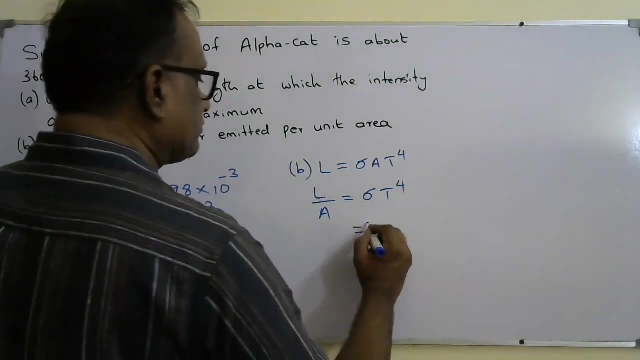 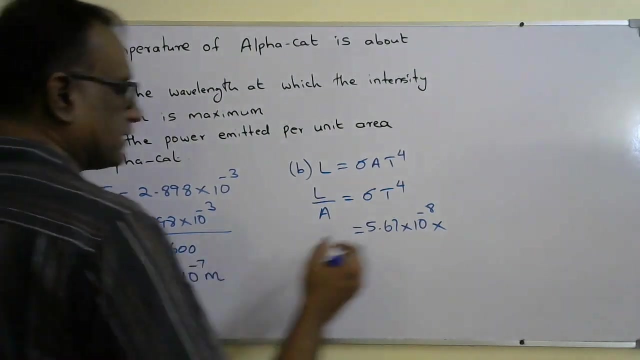 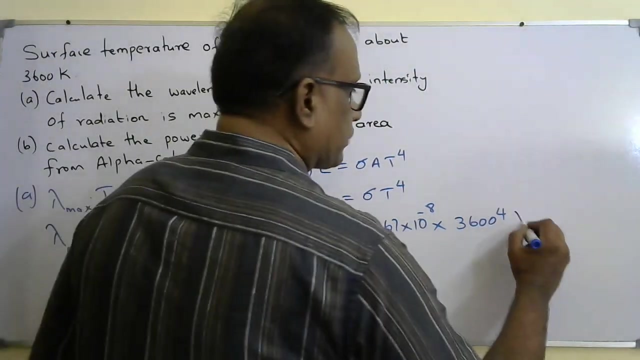 per area is sigma t to the power four, so we know the sigma Staphon Boltzmann constant. that is 5.67, 10 to the power, minus 8 times the temperature, 3600. so 3600 to the power 4, so this much of watts per meter squared. 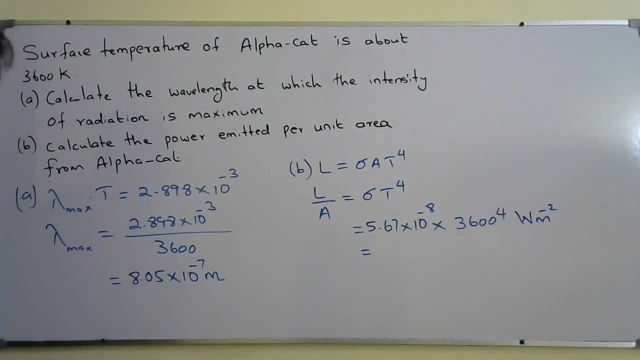 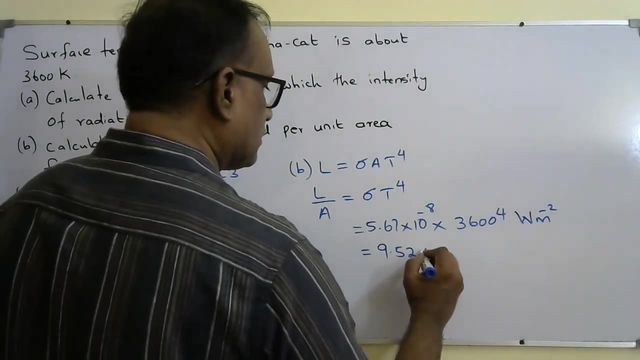 watts per meter square. so salt. we have to calculate the electrical temperature from furーい second medium energy, 3.67W tower camera, Carlson, Frank words. so what does the temperature range? And x etwa ç, you will get the answer. that will be equal to 9.5 to 10, to the power, 6 watts per meter squared. 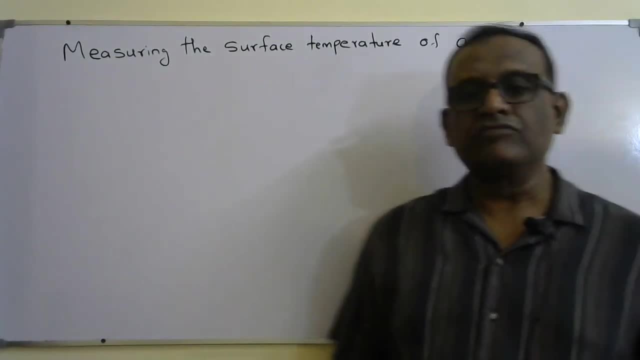 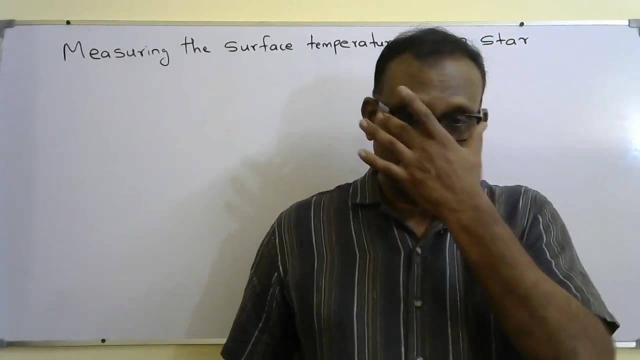 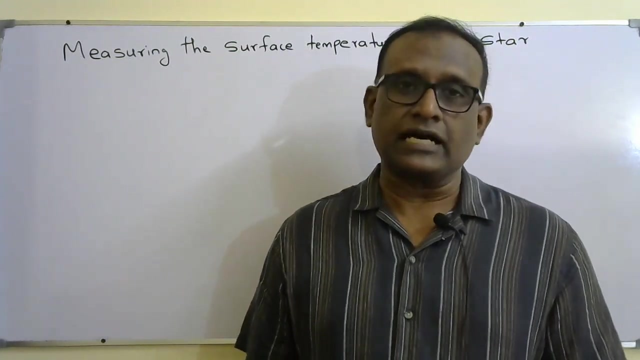 Okay, so how can we measure the surface temperature of a star by using these laws, what we learned? Okay, so it's simple. You must know this. They can ask in the exam. They earlier asked also. So how can we measure the surface temperature of a star? 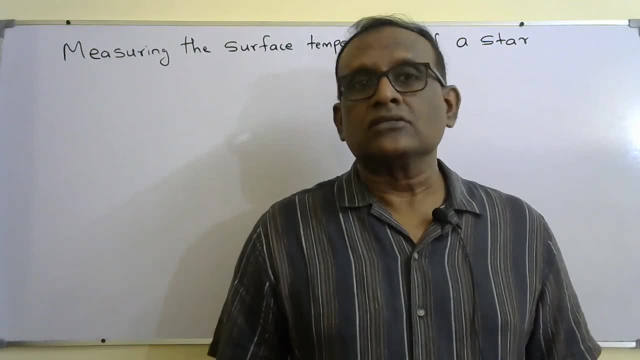 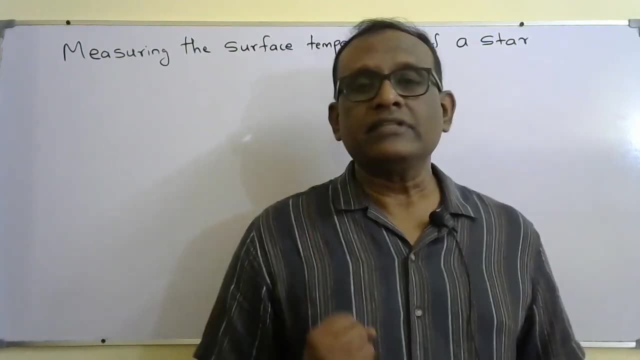 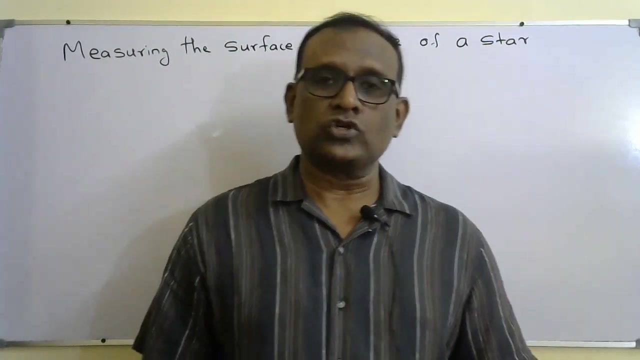 Okay, you know we assume stars behave as black bodies. So what we do? we use a powerful telescope to receive the light or radiation emitted from the stars. So it's better to use a satellite telescope. Satellite telescope means a telescope which is fixed on the surface. It's fixed on a satellite because if you try to receive radiation from Earth, the radiation from the stars- certain wavelengths could be absorbed or scattered by the atmosphere, So we might lose that radiation in our experiment. So to avoid this unwanted loss we can use a satellite outside the Earth's atmosphere which is fixed on a satellite. 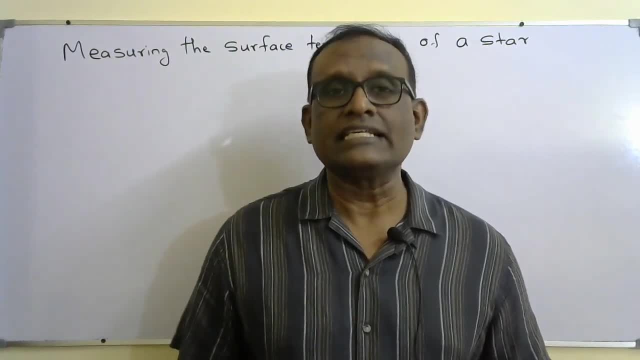 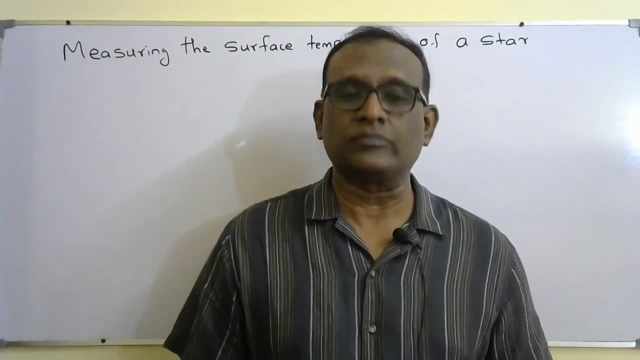 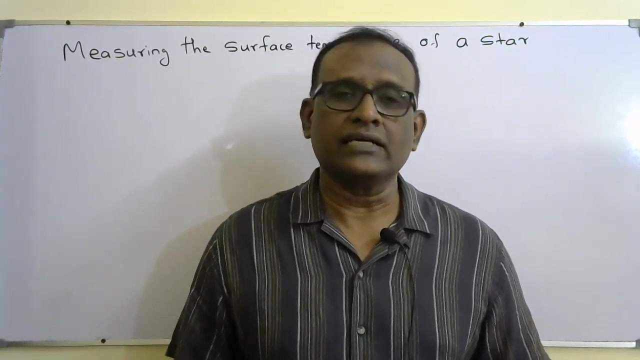 So, by using a satellite telescope, receive the radiation from the star. You are going to measure the temperature of that particular star. So receive the radiation from the star. Disperse the radiation into different wavelengths. In your syllabus you know that by using diffraction grating you can split the white light or split the radiation into different wavelengths. 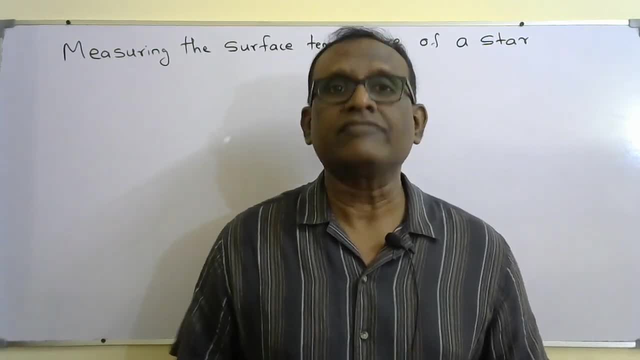 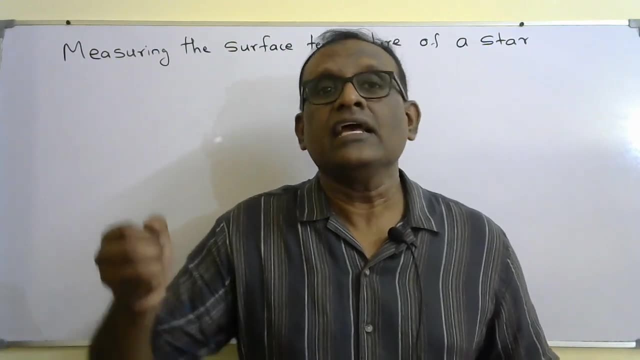 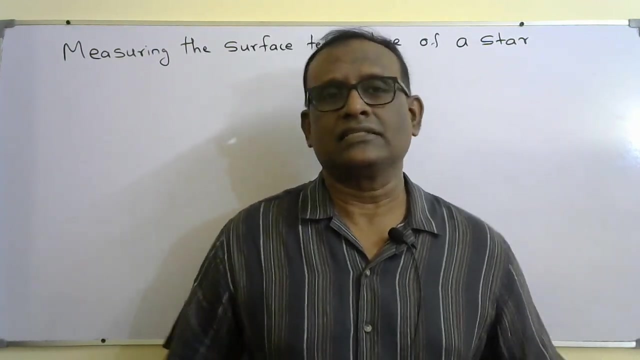 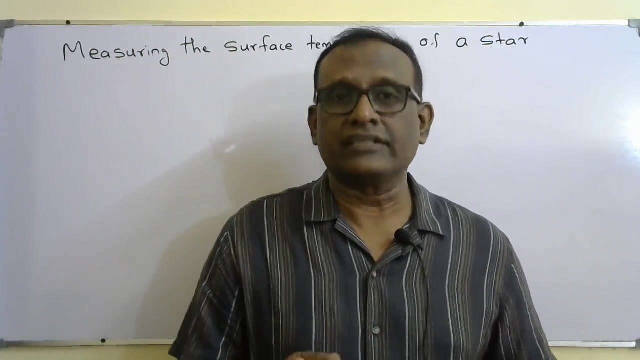 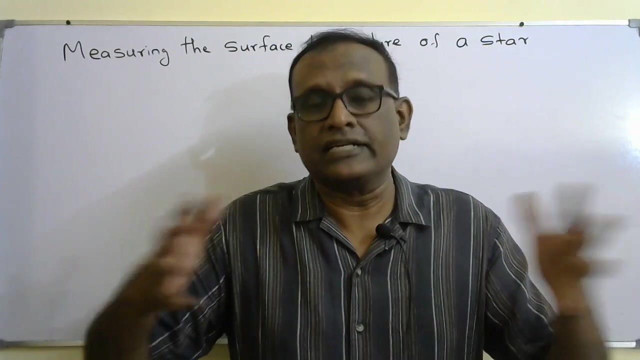 Something like that: Disperse the radiation received from the star into different wavelengths, Measure the intensity of each and every radiation. You can measure the intensity of each and every wavelength of the radiation that we receive from the star, after that radiation is split into or dispersed into different wavelengths. 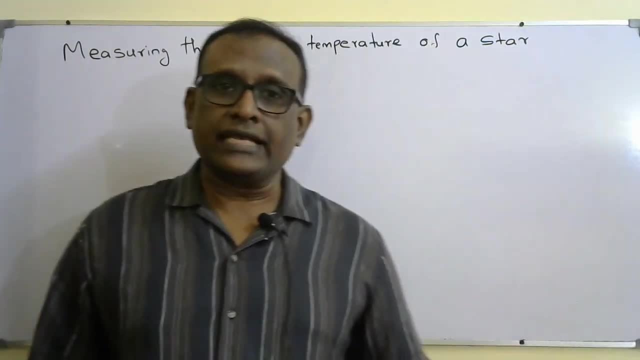 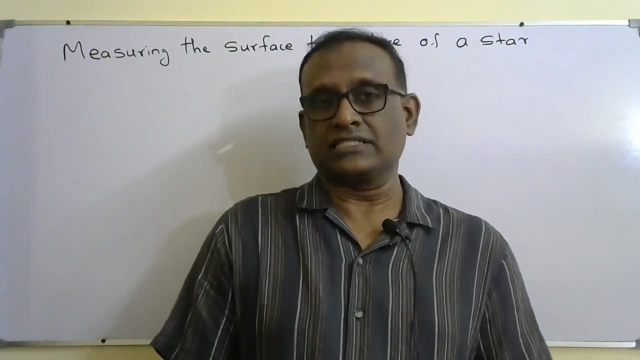 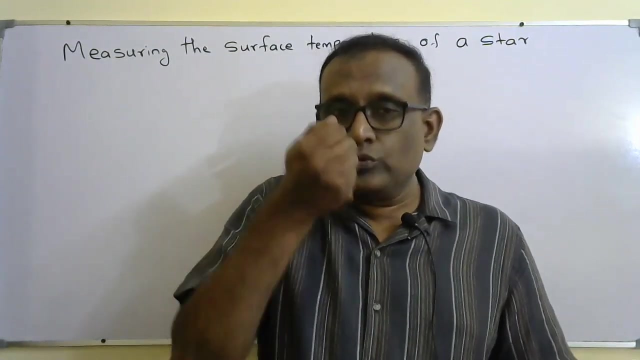 Measure the intensity of each and every wavelength. OK, Identify the most intense wavelength, So most intense radiation, first, So you know, when you are measuring the intensity of each and every wavelength, identify which radiation is giving the highest intensity, So that's the most luminous radiation. 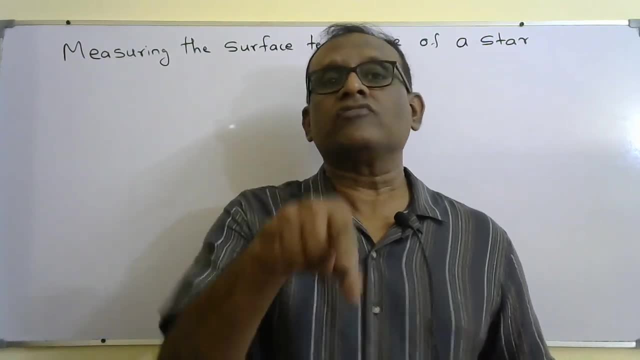 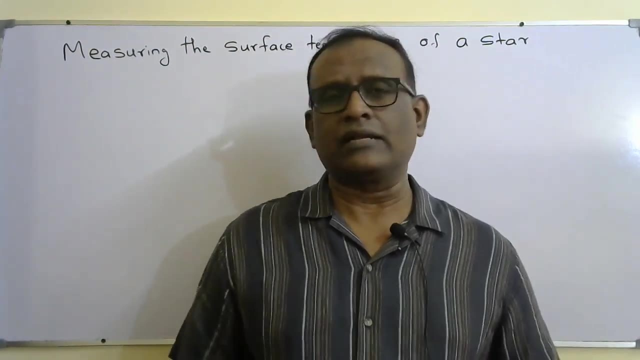 Then we should find the wavelength of that particular radiation. How can you find it In your syllabus? we can say by using double slit experiments. Simple: There are a lot of methods. There are Newton's rings, So there are many methods. 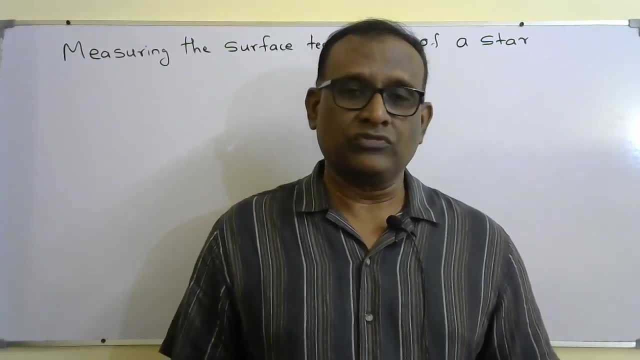 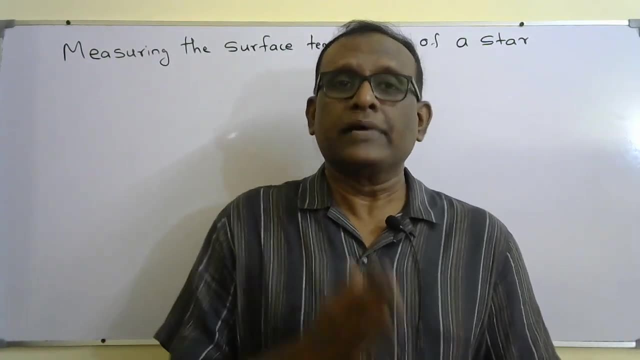 But in your syllabus you need two. We learned how to measure the wavelength. So by using double slit, So by using a method, find the wavelength of this particular most intense radiation. So you know the wavelength, That is the lambda max. 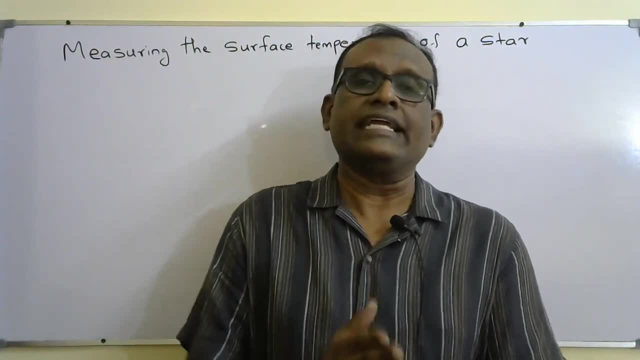 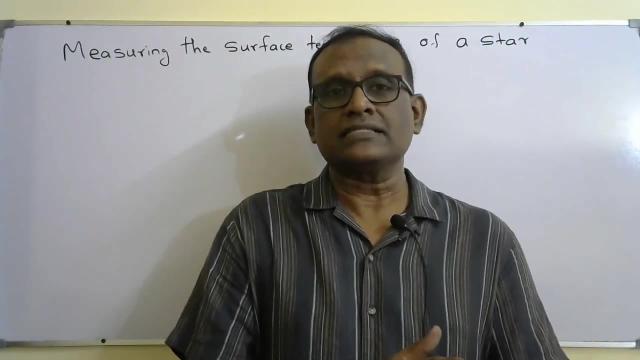 That is the lambda max, Because you are measuring the wavelength of the most intense radiation. So that is going to be the lambda max. You know the lambda max? Use the Wien's law: Lambda max into t, equal 2.8918 to the power of 10.. 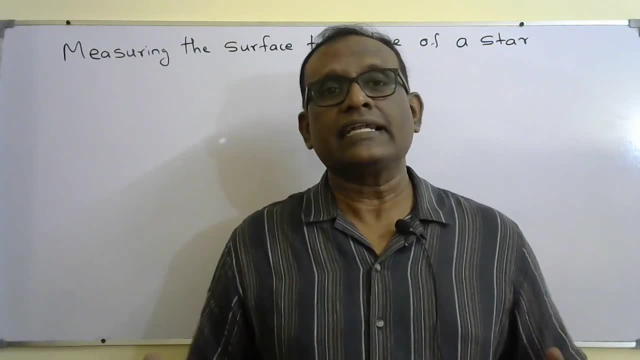 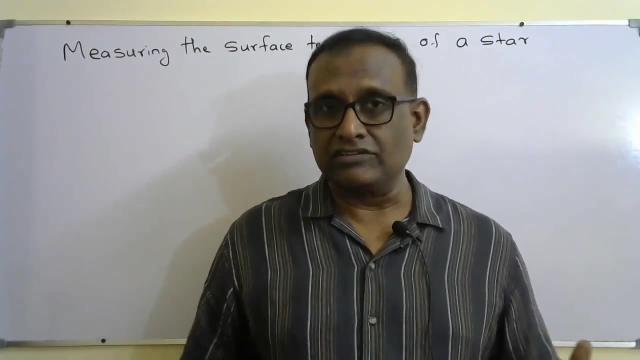 2.8918 to the power minus 3.. From that find the T, That is the surface temperature of the star. So by using Wien's law we can find the surface temperature of a star. I'll repeat it again. 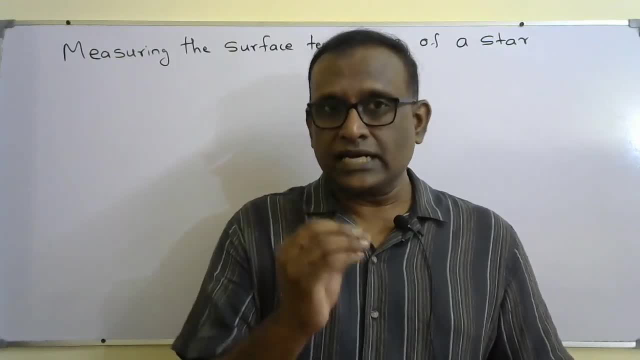 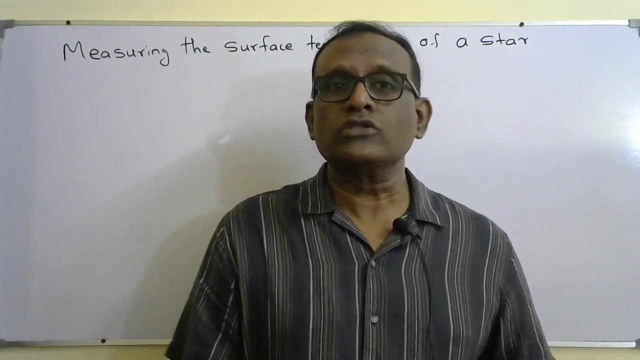 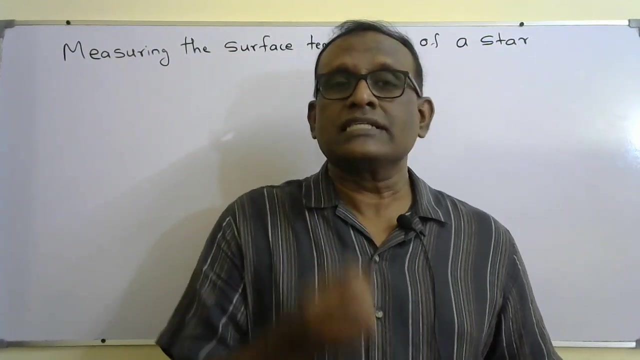 Focus a satellite telescope to the star. Receive the radiation from the star, Disperse it into different wavelengths And identify the most intense radiation after dispersion. Measure the wavelength of this wavelength, The wavelength of this most intense radiation, That is, lambda max. 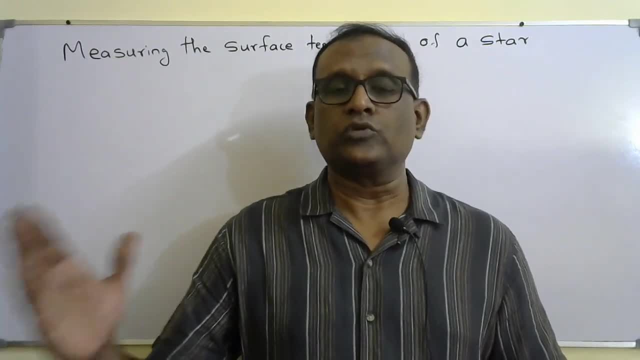 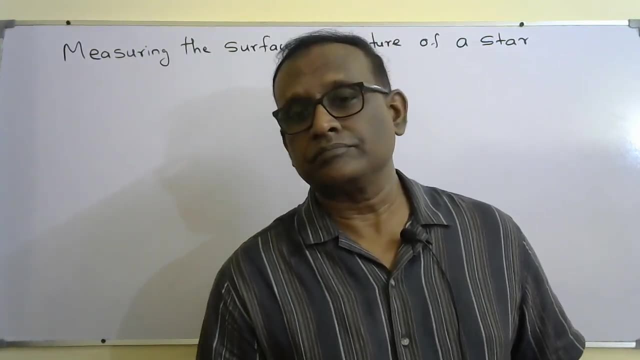 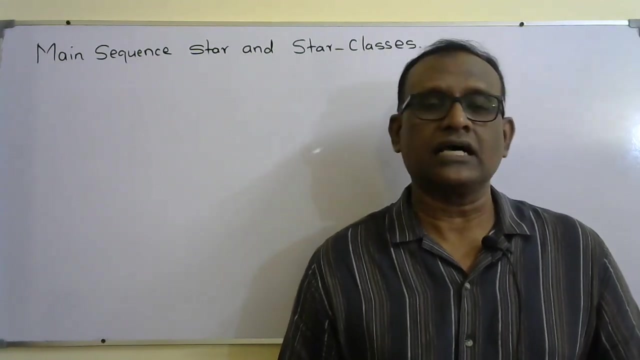 By using Wien's law, Lambda max into t equal 2.8918 to the power minus 3.. Find the T That is the surface temperature of the star. So the next thing you should know, The main sequence, star and star classes. 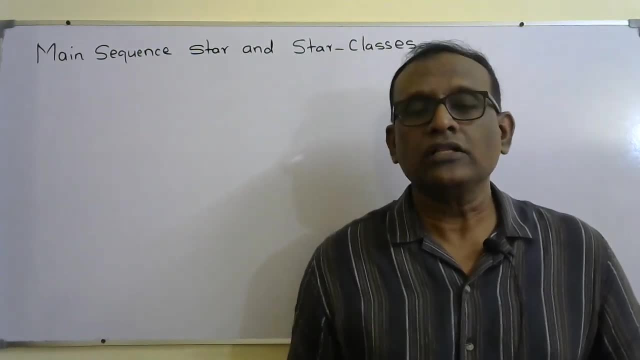 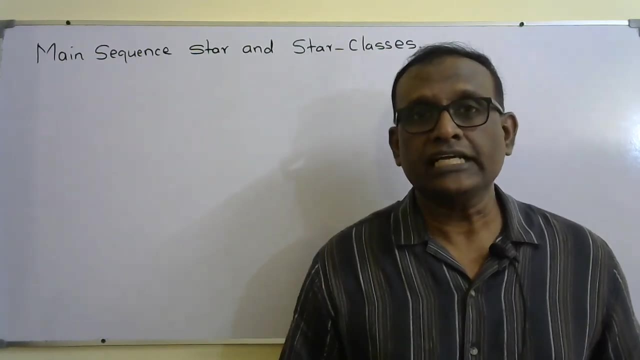 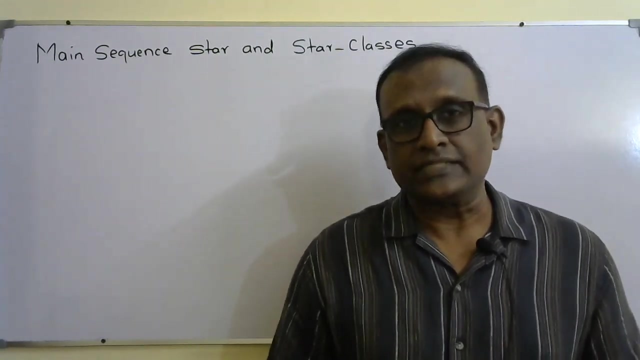 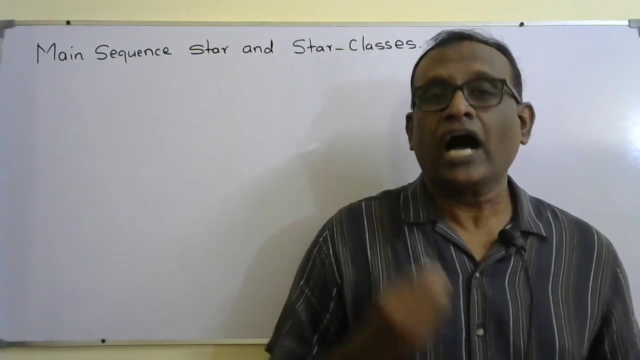 So what is meant by main sequence star? You know all the stars, including sun, emit radiation Or emit heat and energy due to nuclear fusion reaction. So in all stars nuclear fusion is happening. So main sequence means, or main sequence star means, If there is a significant amount of hydrogen fusion. 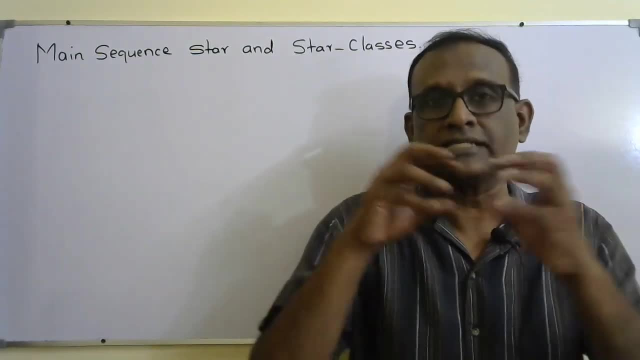 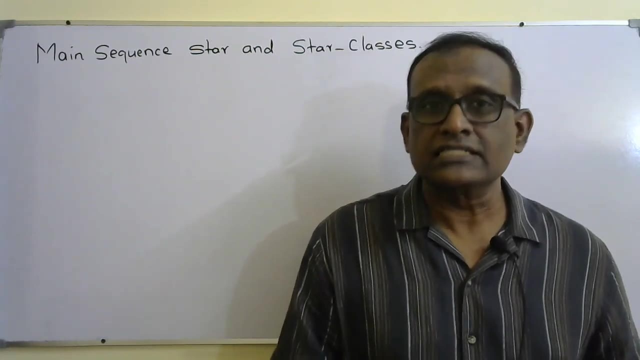 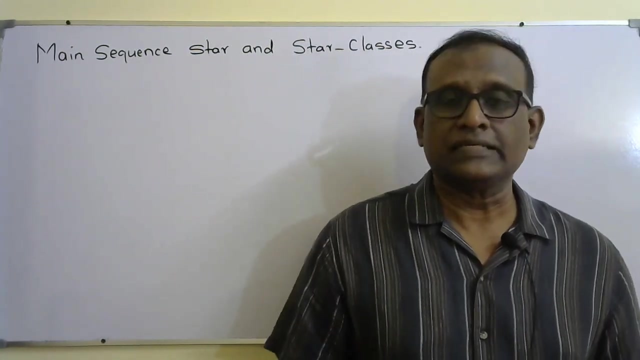 Happens or occurs in the core of the star. Core means the central part of the star. So when there is significant amount of hydrogen fusion Occurs in the core of the star, Then that star is called main sequence star. You know, when you think about after the big bang. You know, initially plasma were created, Then fundamental particles were created After certain amount of years, Later, hydrogen nuclei were created. So the hydrogen nuclei or hydrogen atoms. They attracted each other due to the gravity of the star And when they hit each other. 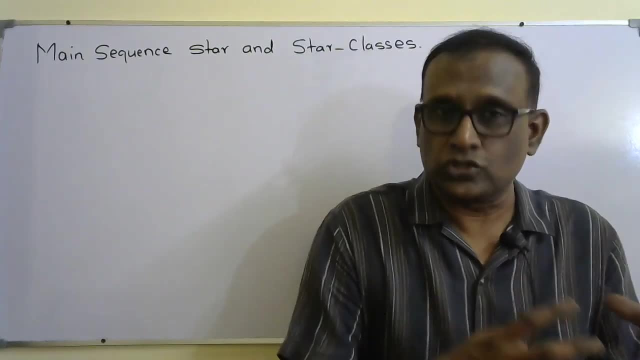 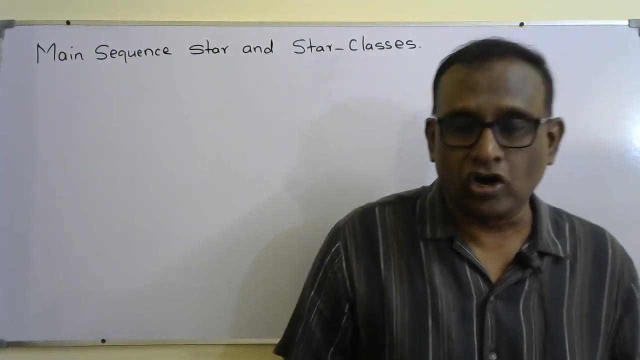 Hydrogen fusion started. So that is the protostar. When I tell you the life span of the star, I will tell you again. But that is the way the stars are formed, Due to hydrogen fusion. So main sequence: star means: 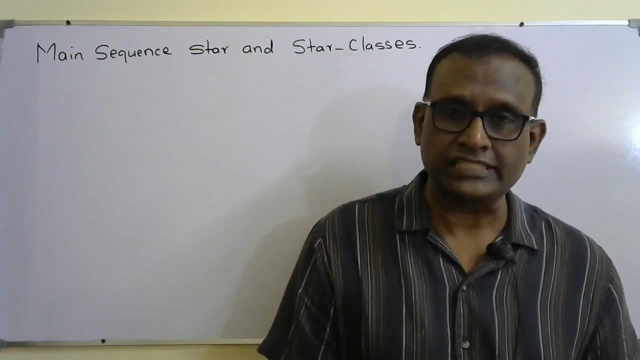 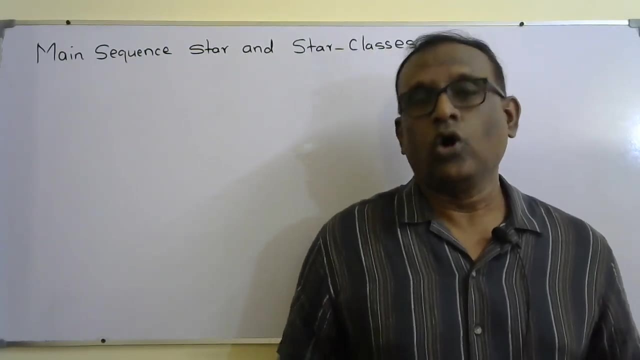 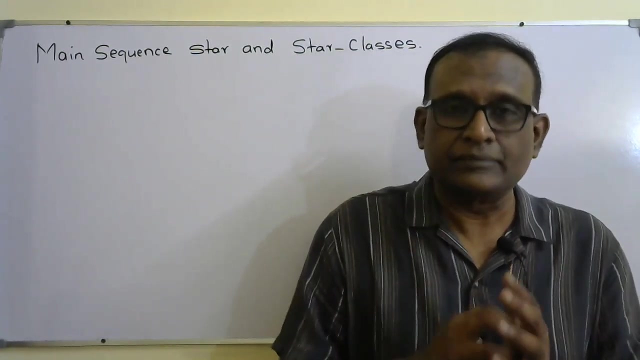 A star that has significant amount of hydrogen fusion In its core- The word core is important In its core- is called main sequence star. Okay, So when a star is in main sequence- So you know the meaning of main sequence- We have significant amount of hydrogen fusion. 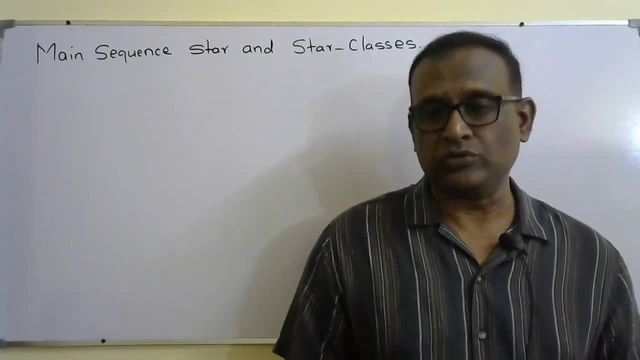 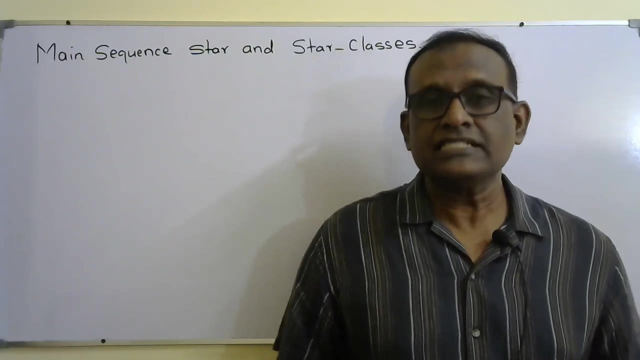 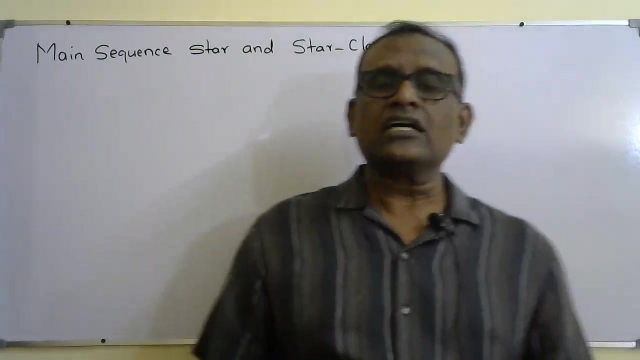 Occurs in the core of the star. When a star is in the main sequence, The star experiences two different types of pressure. We can say The first is due to inward gravitational pressure. The first pressure is called inward gravitational pressure Because, you know, a star consists of huge, tremendous amount of gas. Mainly the hydrogen In its core. So there will be very large gravitational force Acting on all the gas particles. That causes very large amount of inward gravitational force, And force per unit area is the pressure. So that is called inward gravitational pressure. 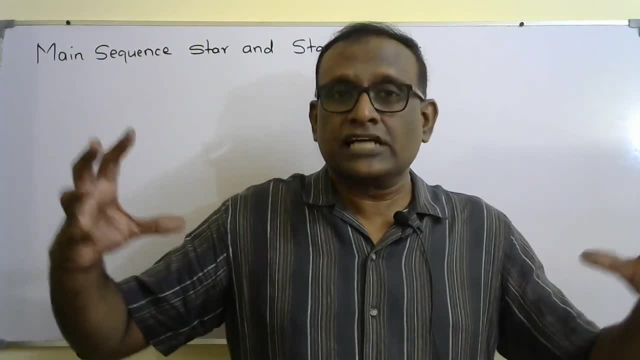 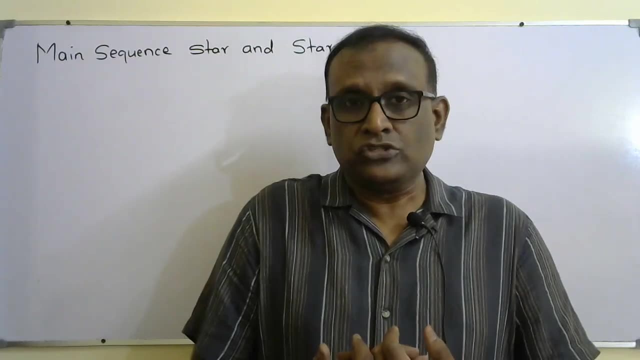 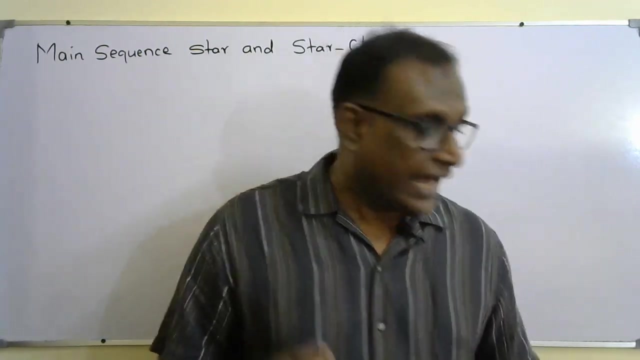 So, due to this inward gravitational pressure, The star should string and burst, But that never happens When the star is in the main sequence Because, due to hydrogen fusion, The star is emitting radiation In the form of photons. You know, photons carry momentum. 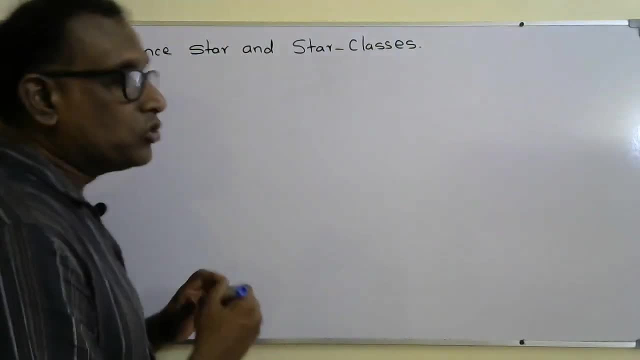 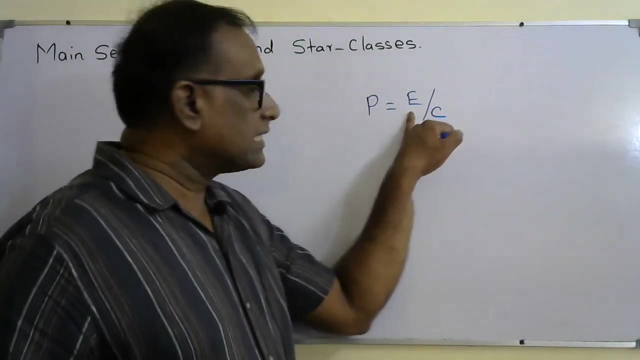 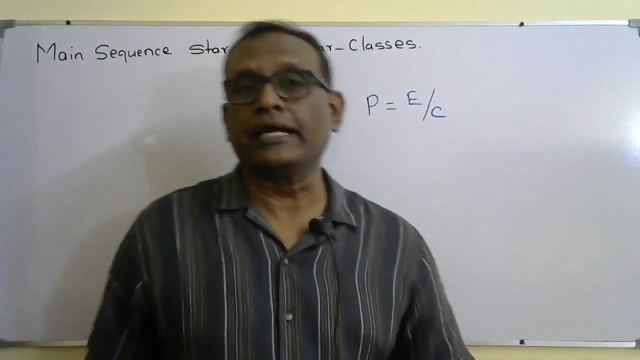 I told that in unit 4.. Momentum of a photon is given by P, equal E over C. Where P is the momentum of the photon, E is the energy of the photon, C is the speed of light. So, due to the momentum carried by the photons, 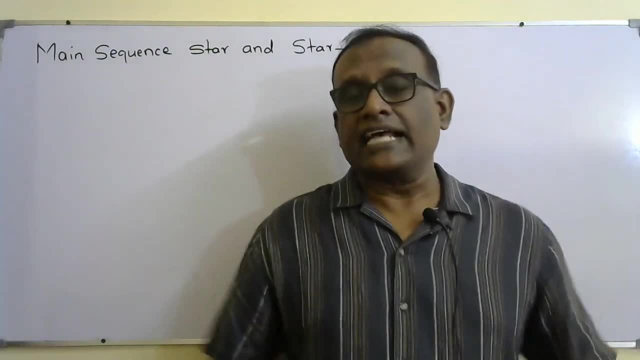 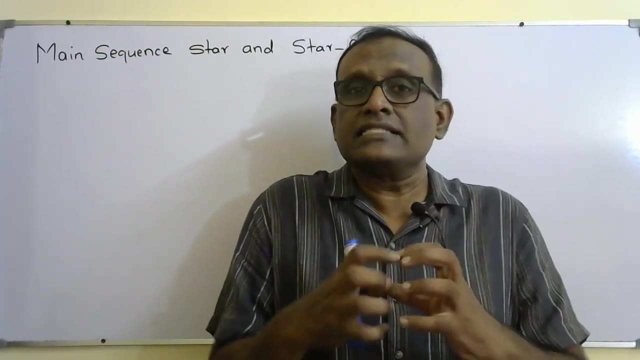 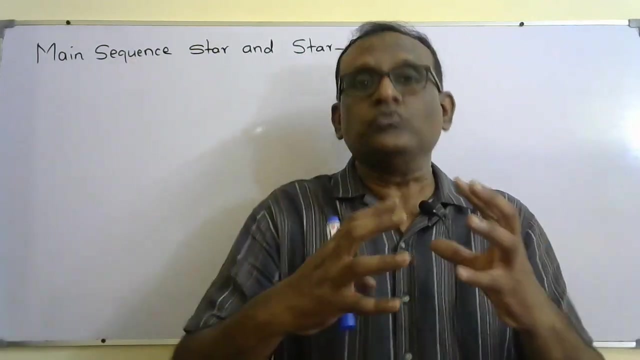 They exert force On other gas particles In outward direction. That is called outward radiational pressure. So when a star is in the main sequence state It experiences two different types of pressures. One is the inward gravitational pressure And the other one is outward radiational pressure. 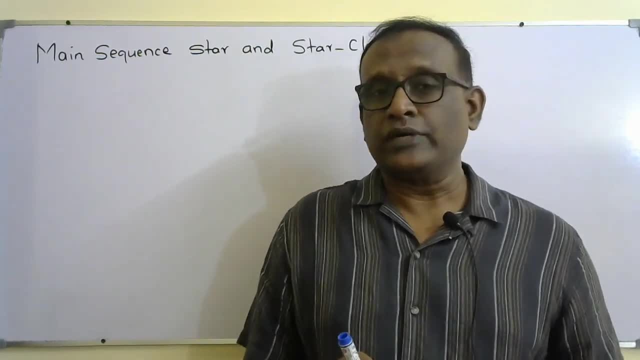 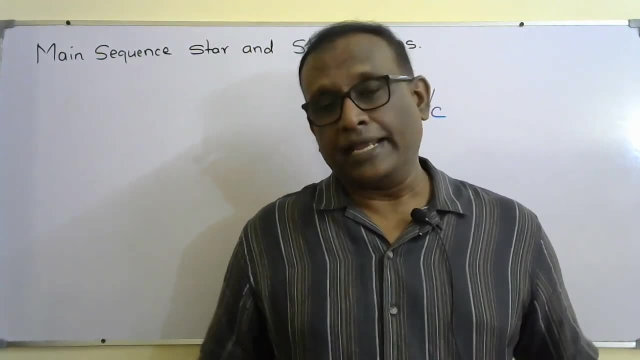 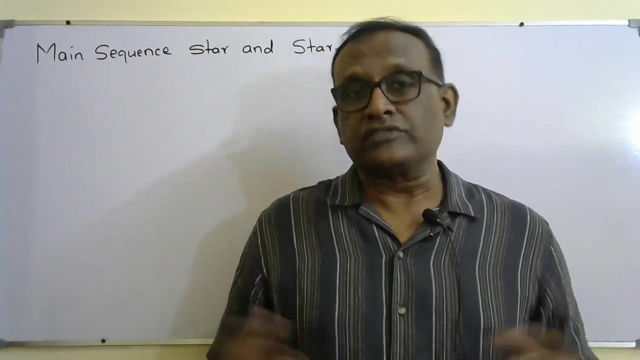 So when the star is in the main sequence, These two pressures balance each other, So the star will have a stable state In its main sequence. Okay, So depending on the mass of the star, The temperature of the star varies. Say, for example: If the star has very large amount of mass- Say, for example, We compare it with the mass of the sun, Which is called solar mass. If the mass of the star is much greater than 4 times the solar mass, What happens? It will have very large inward gravitational pressure. 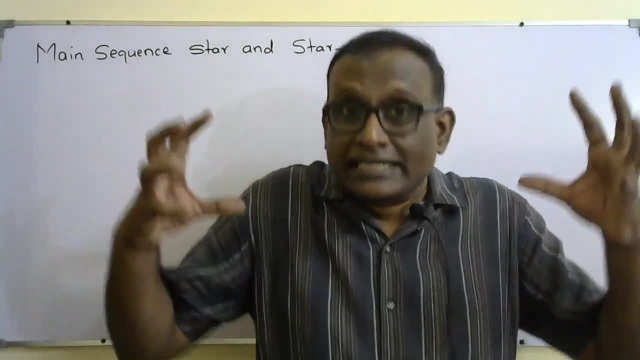 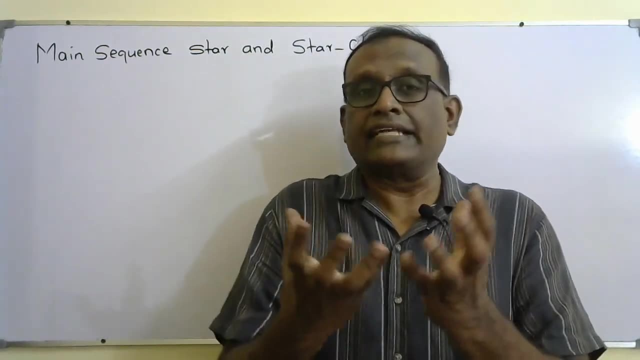 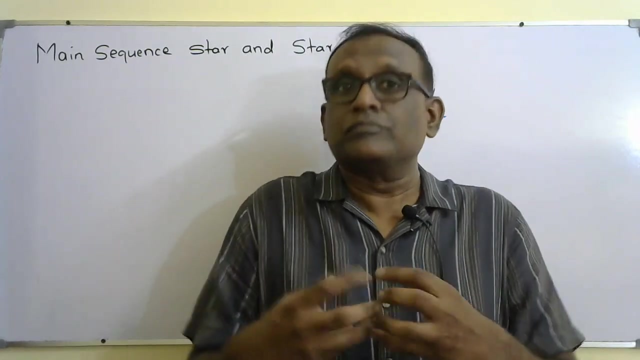 So, due to that, core will have very large density. The hydrogen molecules, or hydrogen atoms, inside the core Will be compressed a lot Due to the inward gravitational pressure, Which even by a huge amount of mass. So what happens? The density will increase. You know that To sustain or continue The hydrogen fusion, The collision among the hydrogen particles, Or hydrogen molecules, should be at very high rate. So due to the very high density The rate of fusion will be very high. So for massive stars, The rate of hydrogen fusion will be very high. Why? The reason is Much larger inward gravitational pressure Will cause the density of the core to be very high, So the rate of fusion will increase. When the rate of fusion increases, What happens? 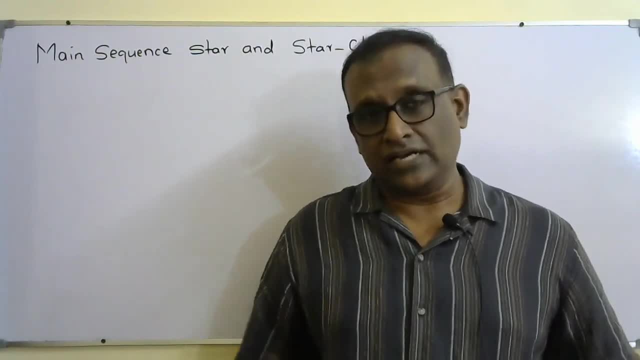 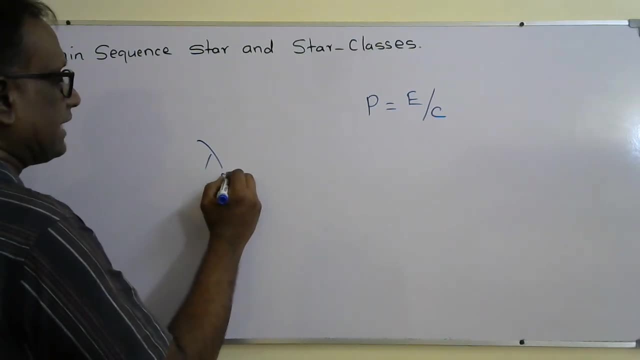 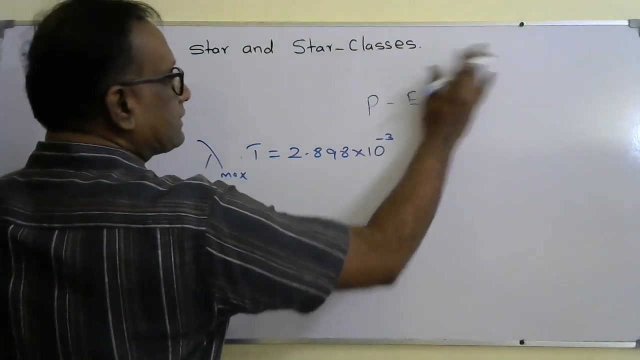 The temperature of the massive star will be much larger When the temperature is much larger. According to Wien's law, Lambda max T equals constant. When you consider that way, 2.898.. 10 to the power minus 3.. When we consider this equation, 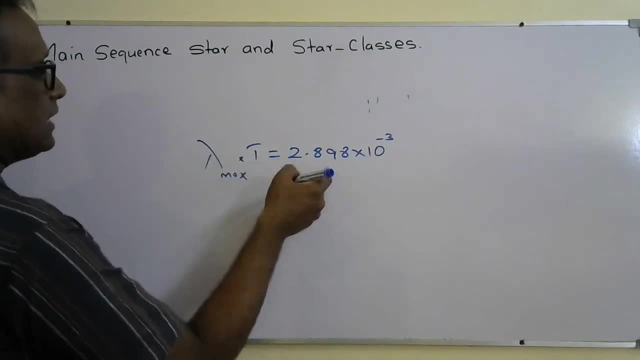 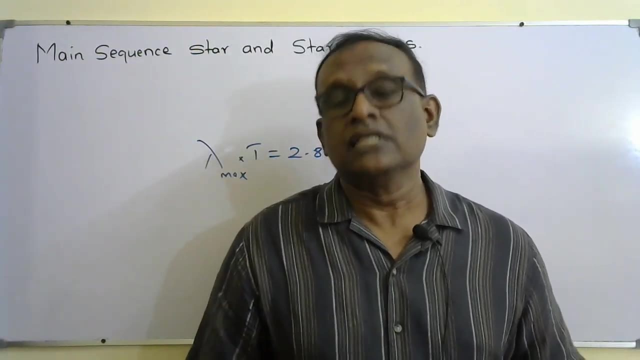 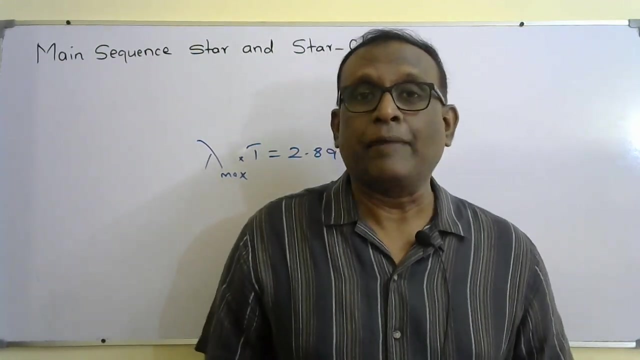 So these massive stars have much larger temperature. So the way Lambda max, The wavelength that corresponds to the peak luminosity, Will be much smaller. So you know, in the visible spectrum The lowest wavelength is almost blue or violet, So massive stars will appear bluish. 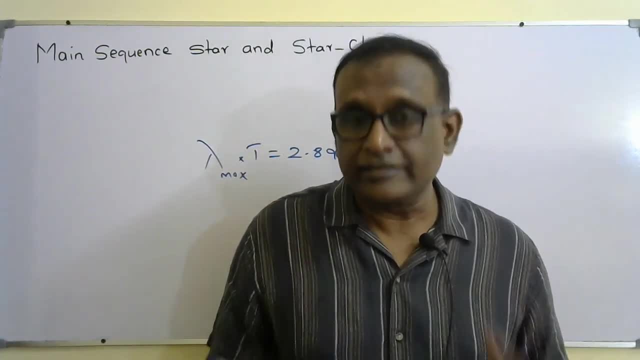 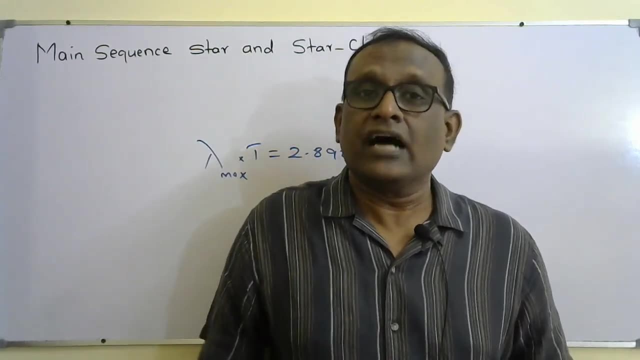 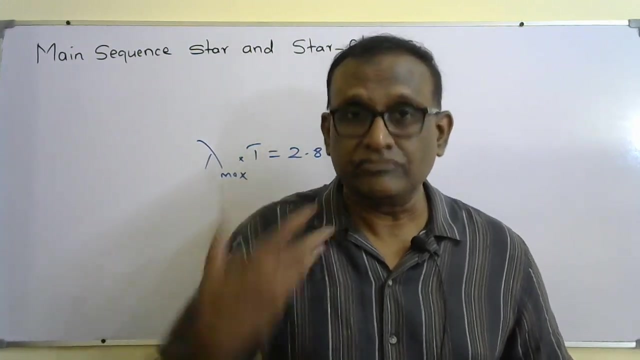 Massive stars will appear bluish. The reason, Again, I will tell you. Massive stars have much larger mass. That causes very high amount of Very high, significant amount of Inward gravitational pressure. That causes very high density Rate of collision among the hydrogen fusion. 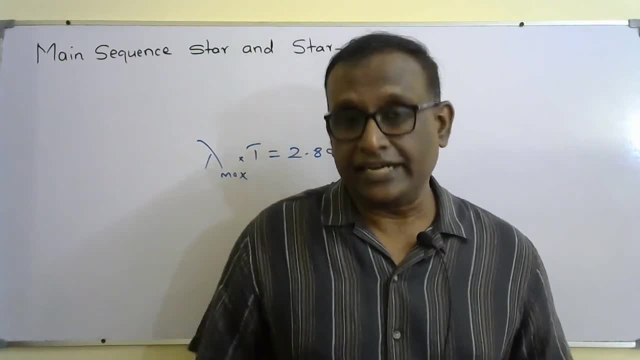 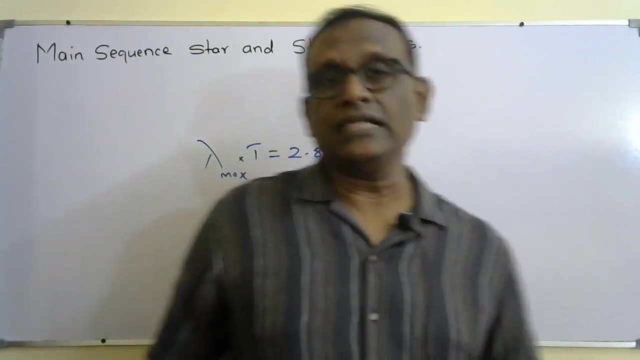 Particles will increase. That causes high rate of fusion. Due to high rate of fusion, What happens? The temperature will be very high. So due to the higher temperature, Lambda max becomes very small, The wavelength that corresponds to the peak luminosity. 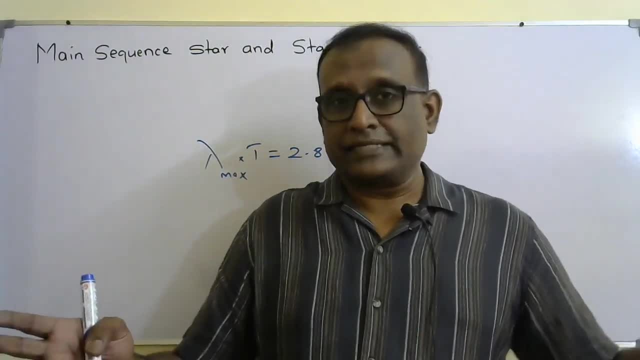 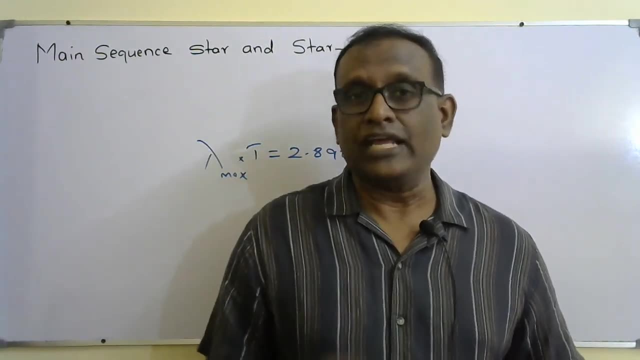 Will become very small. That is, in the visible spectrum, Closer to blue color. So massive stars appear Bluish. Same way low mass stars. So if the mass of the star is Much smaller than 4 times the solar mass, 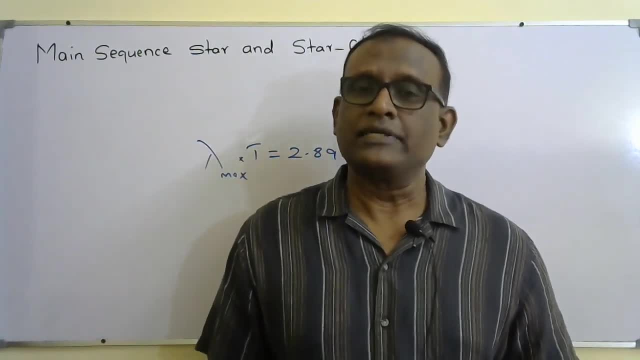 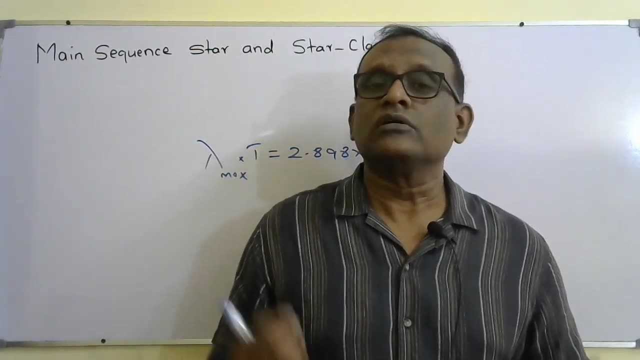 Much smaller than 4 times the solar mass. What happens? The density of those stars, Even when they are in the main sequence, The density of those stars will be much lower. So density lower means. Rate of collision will be lower. So rate of collision lower means. 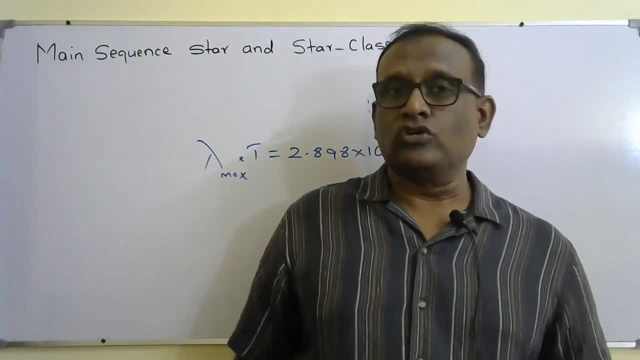 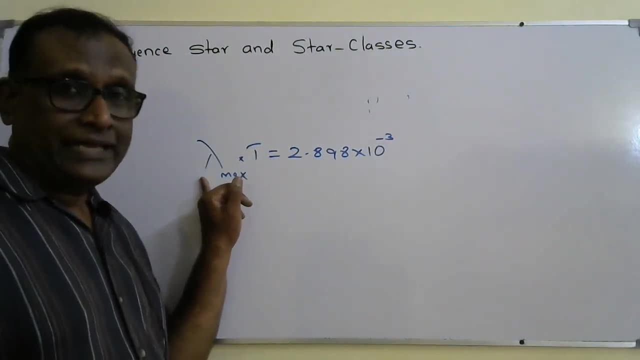 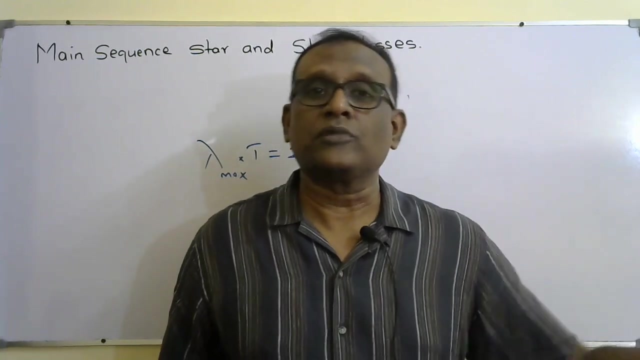 Rate of fusion will be lower. Rate of fusion lower means Temperature will be lower. So temperature lower means Lambda max, The wavelength that corresponds to the peak luminosity Will be larger. In the visible spectrum The highest wavelength Corresponds to red color. 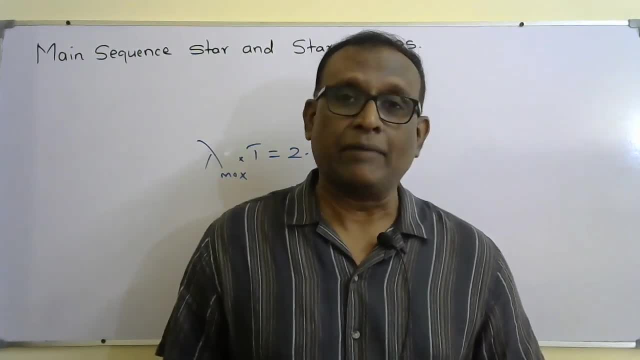 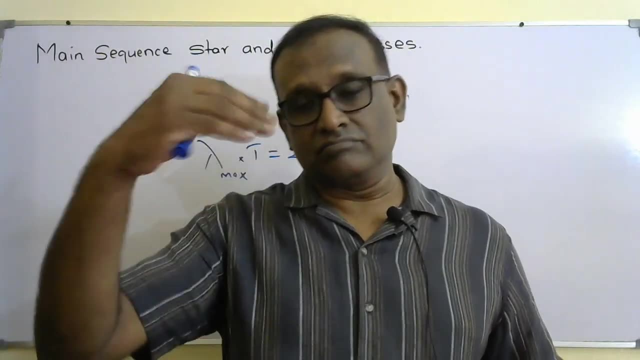 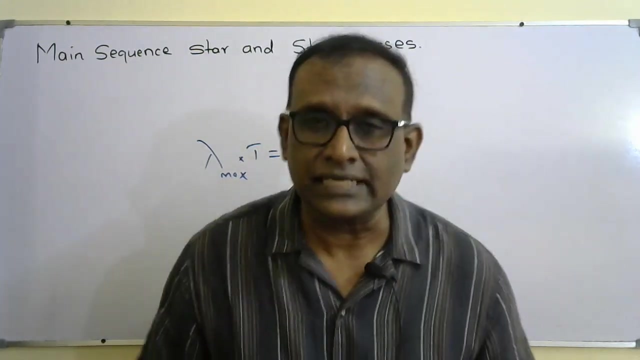 So these low mass stars Appear reddish. There will be other stars In the range between blue and red. There will be different color stars there. You know, sun looks little bit yellowish, So it's somewhere in the middle, Okay. 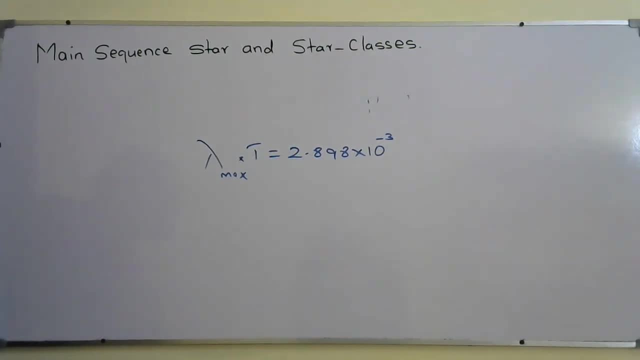 So, depending on the mass of the star, All the stars exist- Are classified into 7 classes. So the 7 classes are, You don't need to remember that. So these are the 7 classes: O class, V class, A class. 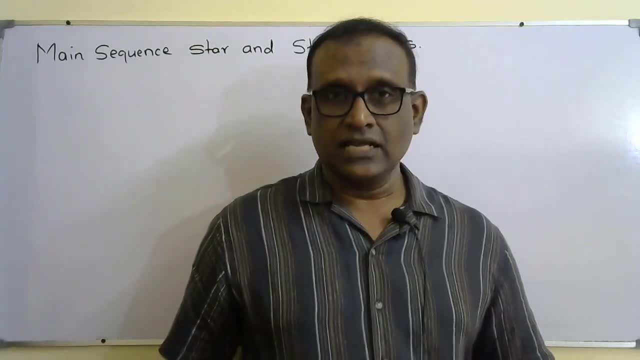 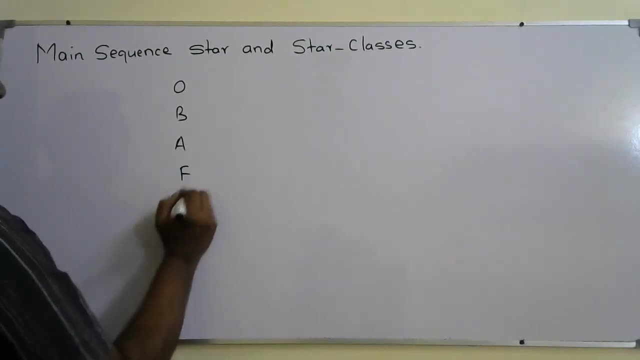 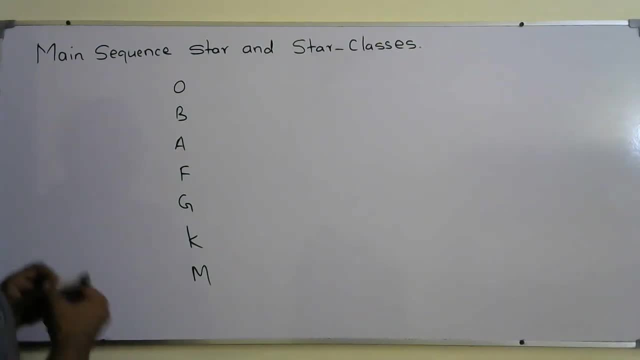 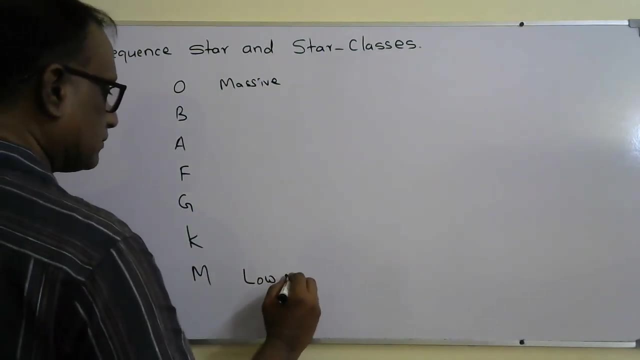 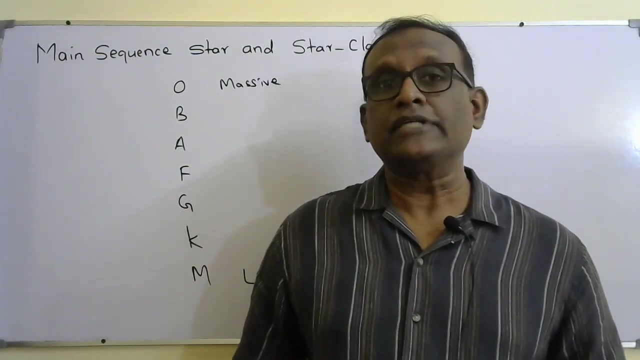 E class Class m, 1 class and m class. These are the 7 classes. O class stars are the massive stars. These are low mass star. So, as I explained, Massive stars appear bluish. You must be able to explain why those stars appear bluish. 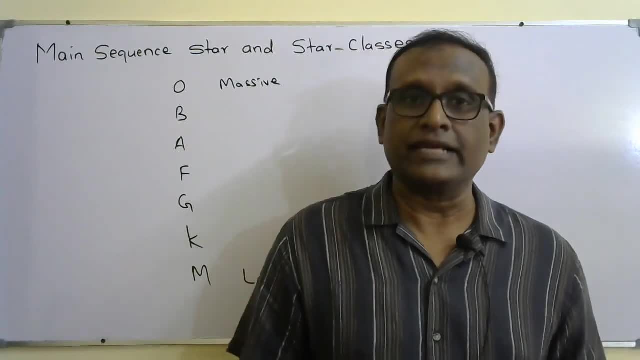 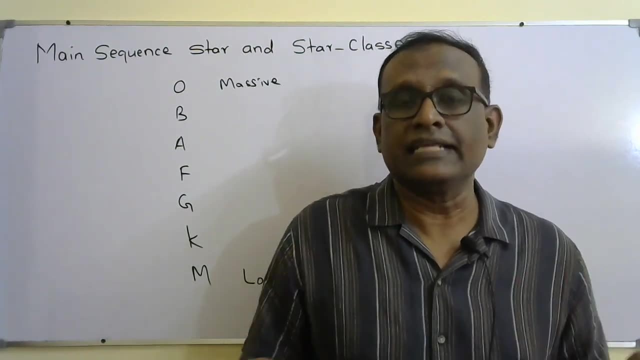 You know that Large inward gravitational pressure That caused by the huge amount of mass, The rate of collision increases Because density will be much higher. much higher rate of collision increases means rate of fusion is higher, so the temperature will be higher. so according to vane's law it becomes: 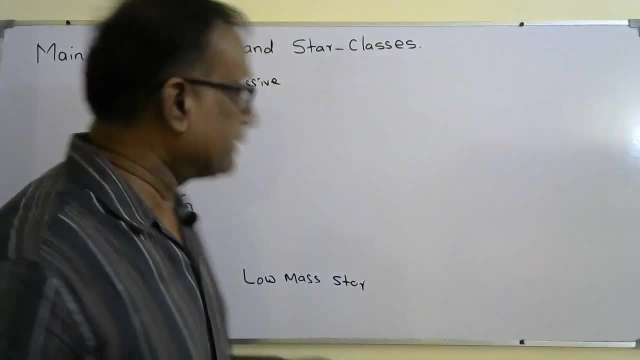 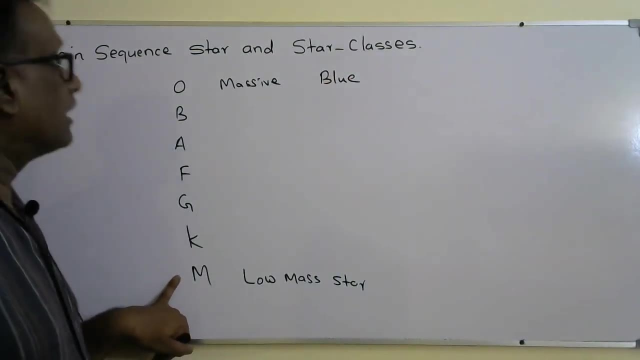 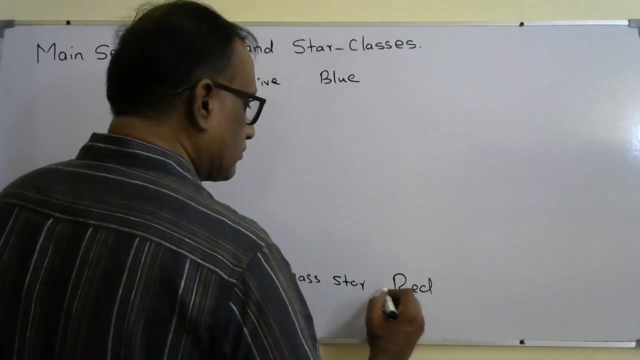 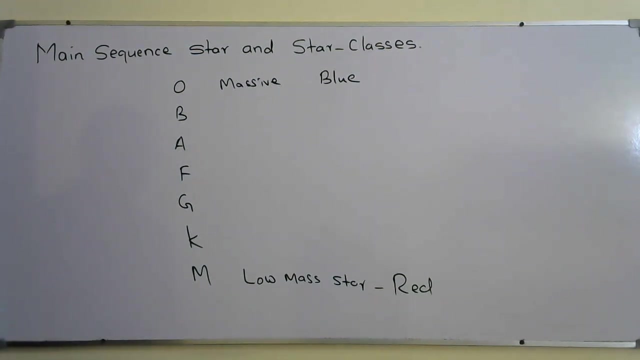 a blue color because lambda max will be lower. i already explained that. so the massive stars appear blue color. low mass stars: they also means main sequence stars. m class stars are low mass stars. they appear red color. low temperature, high temperature. so other stars fall in between o and m class stars. 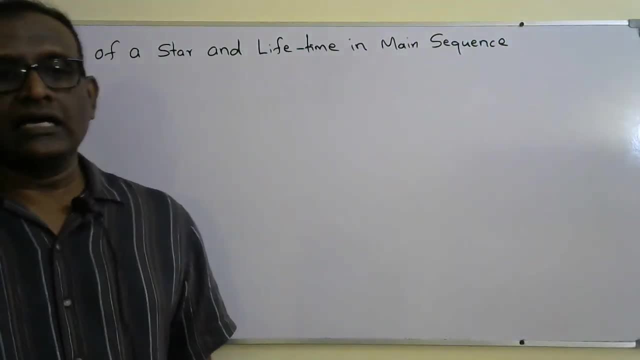 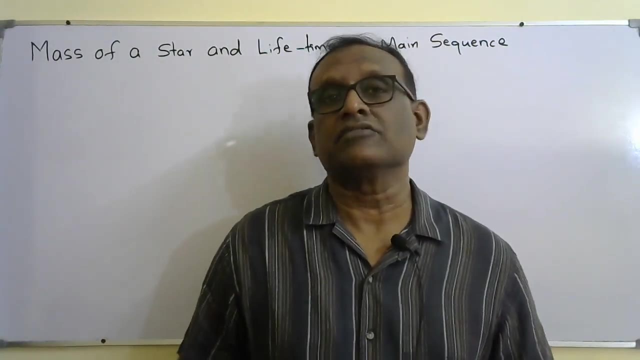 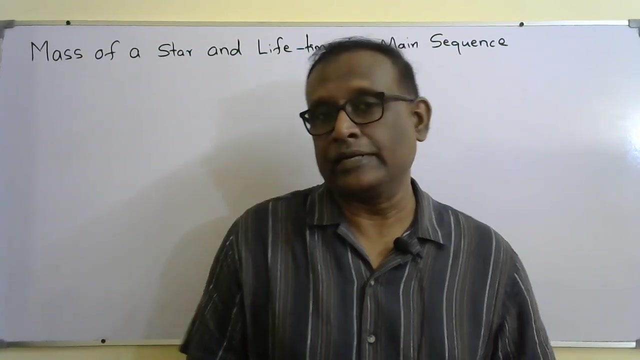 okay. next thing is about mass of a star and, uh, lifetime, in main sequence. okay, we know that o-class stars are massive. their mass is very high. it consists of huge amount of hydrogen in its core, but o-class stars are sorry. i mean o-class stars are massive and they consist of 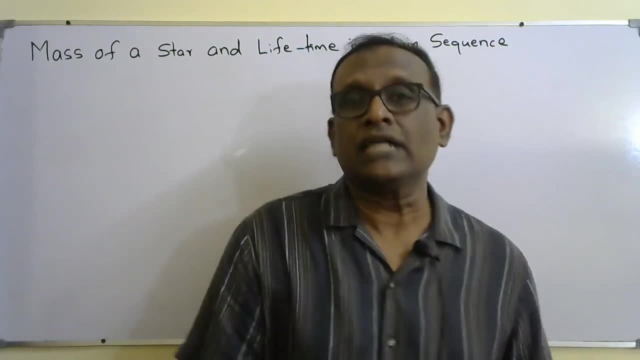 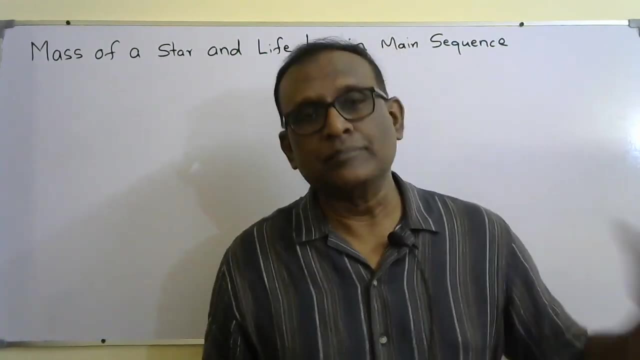 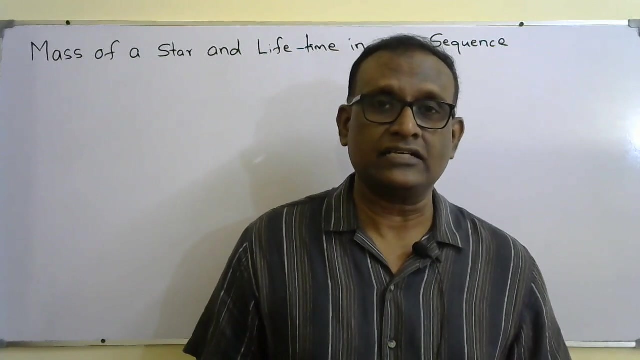 huge amount of hydrogen uh in their core. but m-class stars are low masters. they have less amount of hydrogen in the core. so which of these two stars- i compare only the o-class stars and m clusters- which of these two stars will remain in the main sequence state for longer time? you? know actually, uh, o-class stars have very high mass. but even they have very high mass. their lifetime in the main sequence is much lower compared to m-class stars. the reason is due to much larger inward gravitational pressure. the rate of fusion will be very high in o-class stars. due to higher, much higher rate of fusion, the hydrogen will be fused during shorter periods. so shorter periods means the o-class stars will remain in the main sequence for several millions of years. but m-class stars have lower rate of fusion. so lower rate of fusion means they will keep the hydrogen in their core for. longer periods. so they will remain in main sequence for billions of years. o-class stars can remain only for millions, millions of years. so the lifetime in the form of main sequence scale is much lower for o-class stars. the reason: due to their massive mass, the rate of fusion is very high because 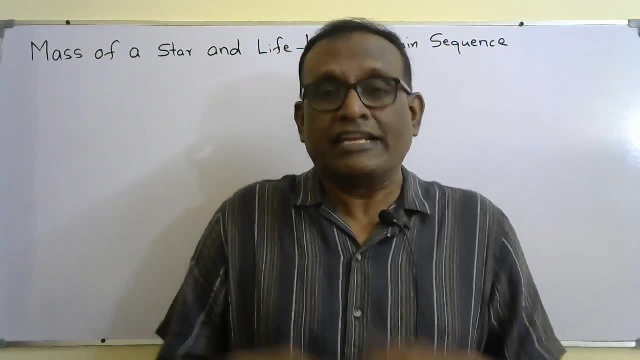 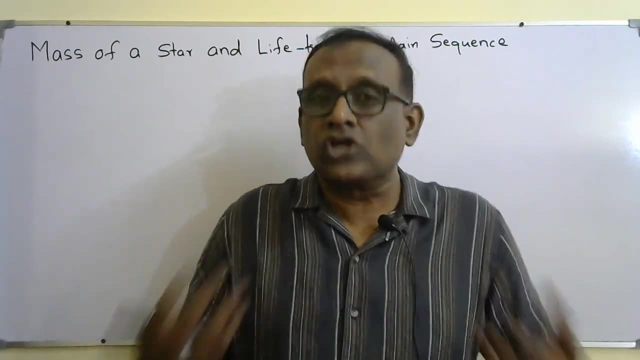 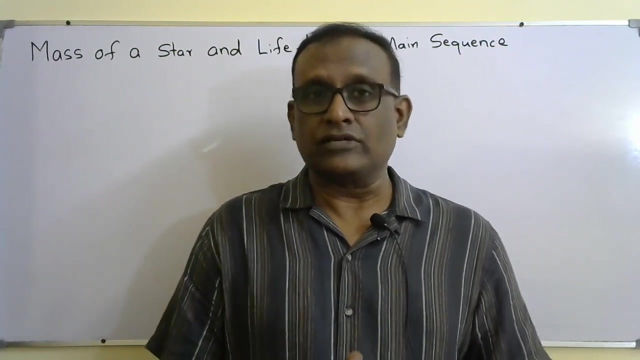 of inward gravitational pressure. you know it supports or influences them. hydrogen fusion by giving sufficient amount of density so the hydrogen will be used up in a shorter period. so they can uh be in the main sequence, uh, m-class, o-class stars. they can be the main sequence only for a few millions of years. but 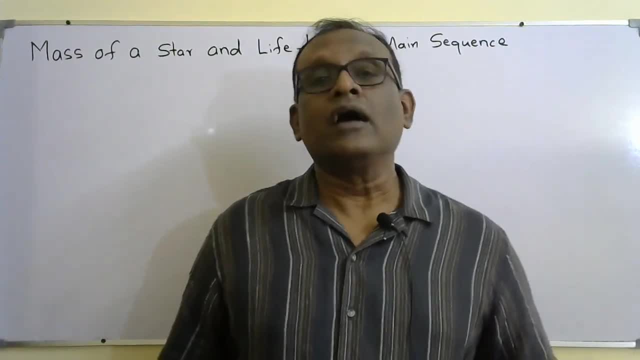 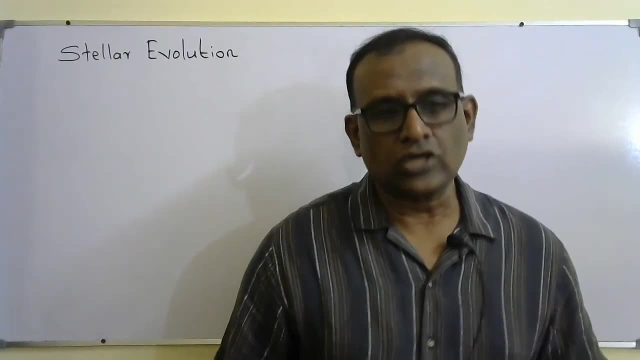 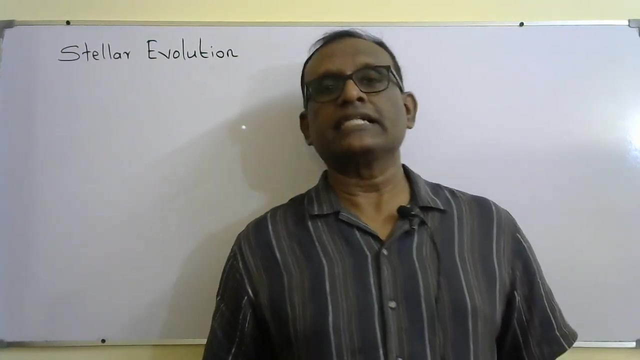 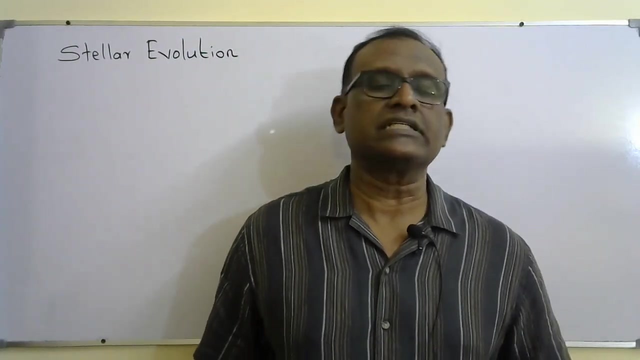 m-class stars can be in the main sequence of several- uh millions or billions of years. okay, so next topic about stellar evolution. stellar evolution means how the uh star changes during its lifetime. okay, so we classify this into two groups. normally, the stable stellar evolution is classified into two- uh different types. 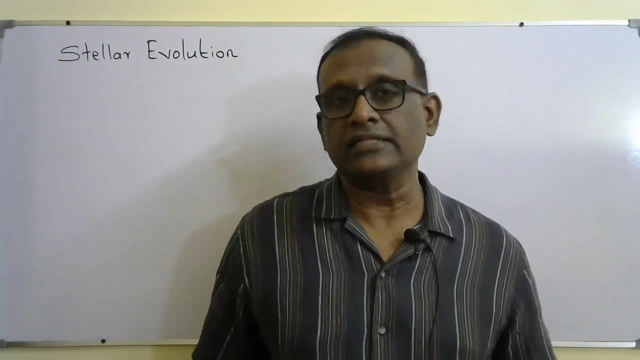 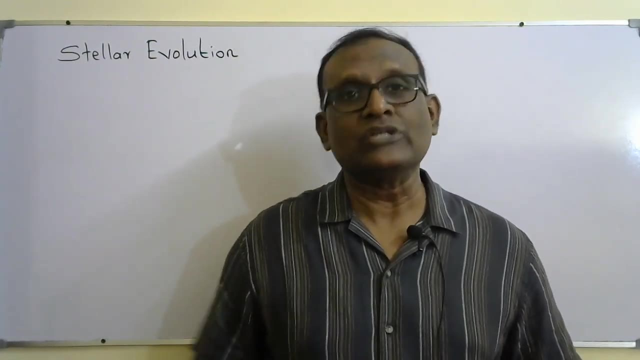 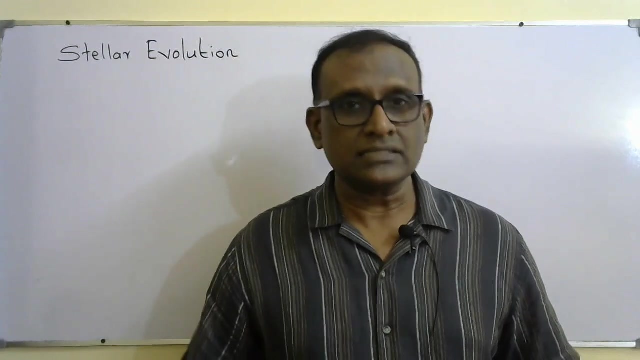 one is called lifespan of low master, the other one is called lifespan of massive star uh, as i told earlier, stars are classified into eight classes. but in terms of that is uh, depending on the uh color and the mass, we classify them into eight classes, but here the depending on the stellar. 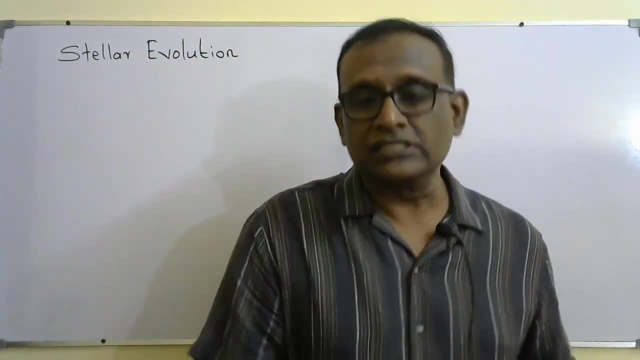 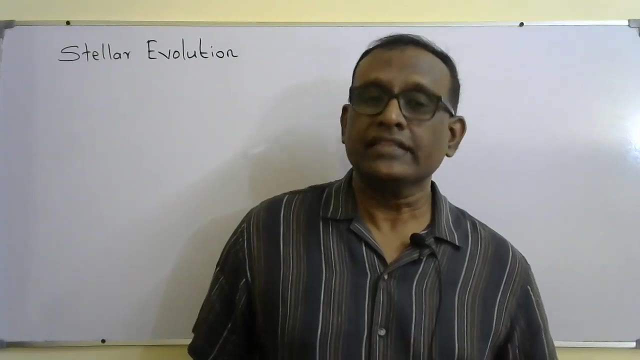 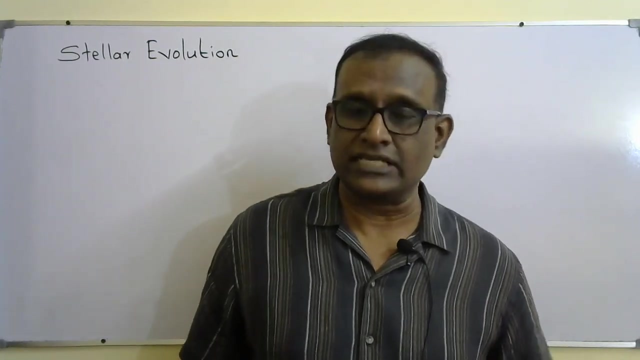 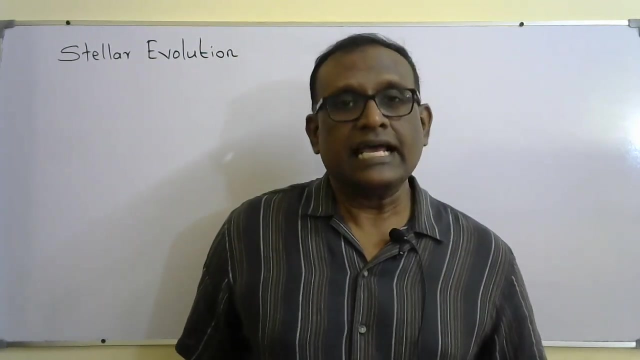 evolution, how they are, uh, how the stars changes during their lifetime. depending on that, they are classified into two groups. they are, like we call that, stellar evolution of low master and cell evolution of massive star. so what do you mean by low master? low master means if the mass of a star is less than or equal to four times of the solar mass. solar mass means mass of the sun. so if the mass of a star is less than or equal to four solar mass, then that type of star is called low master and its lifespan is a particular type. same way, if the mass of a star is more than, 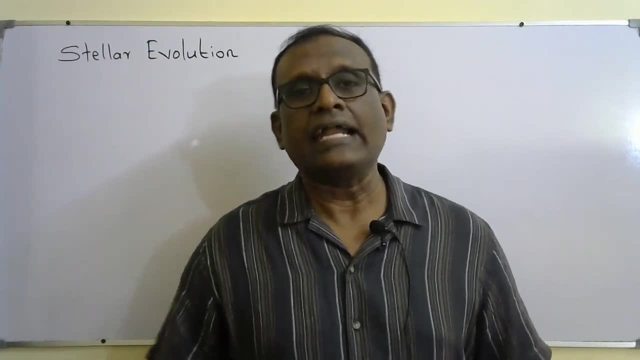 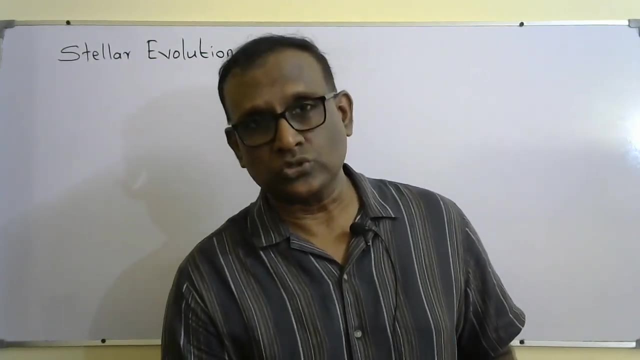 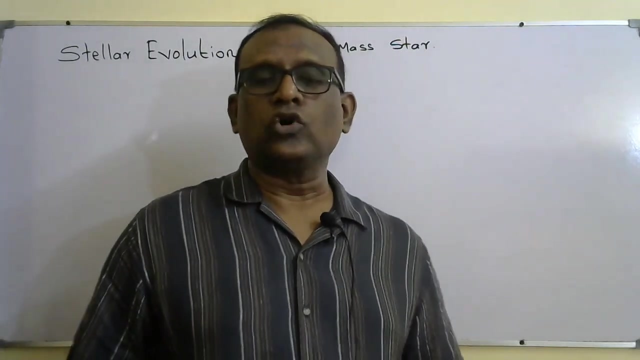 four times the solar mass. that is called massive star and its lifespan is different compared to lifespan of low master. so we are going to analyze these two different types of lifespans. so okay, so stellar evolution of low master. low master means if the mass of the star is less than or equal to 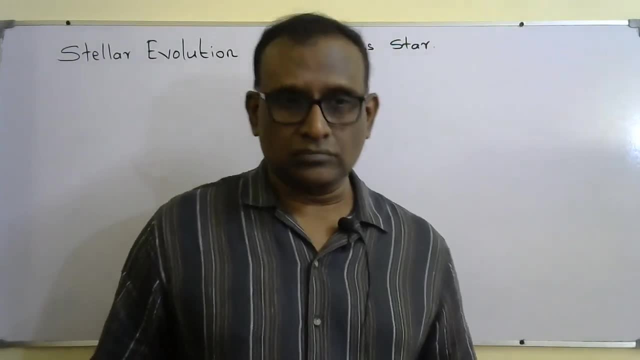 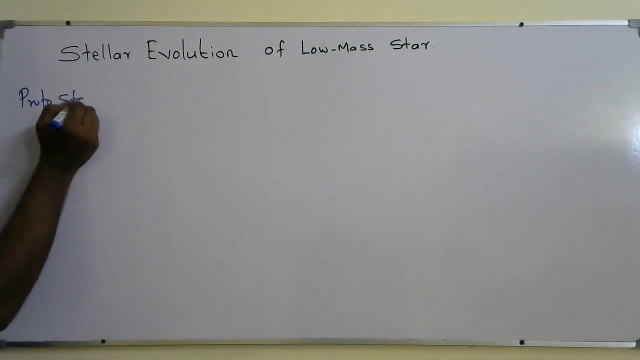 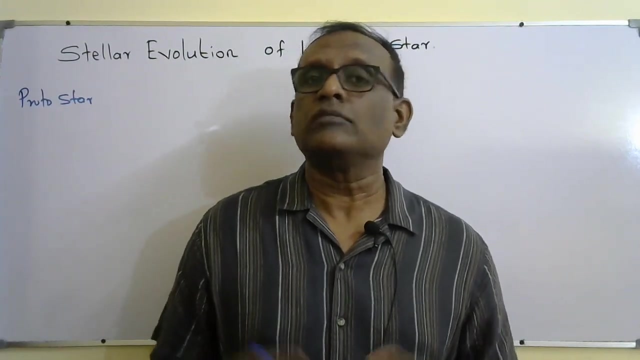 four times of the solar mass. that is called low master. okay, so initial first stage is protostar. so protostar means where the hydrogen molecules have started the fusion, so that is called protostar. when the high, when it collects more and more hydrogen due to gravitational pull. 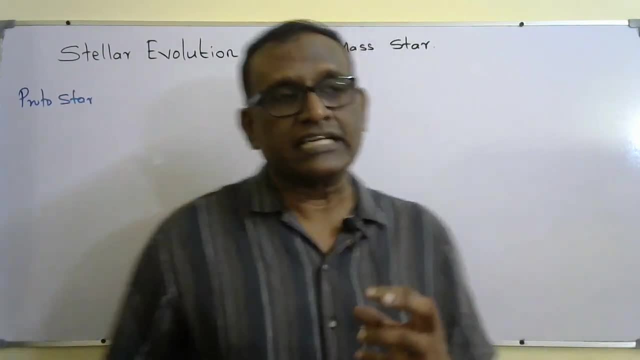 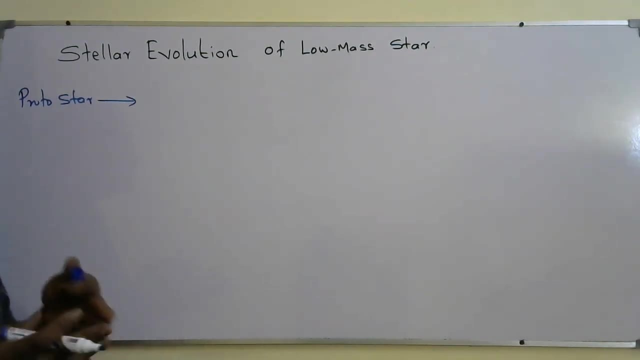 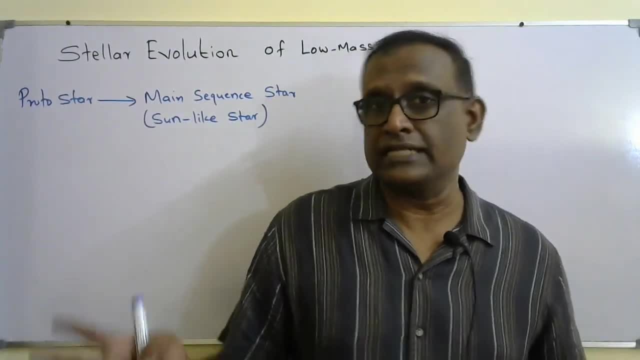 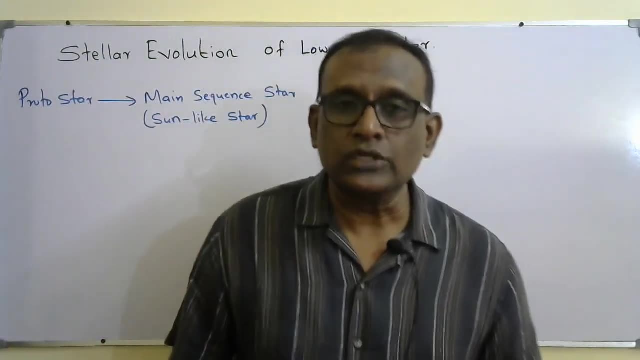 could be in several millions years or few millions years, depends on the mass. so that means depending on that. okay, so what happens when it is in the main sequence star? it experiences, as i told earlier, two different pressures: outward radiational pressure due to the momentum of the 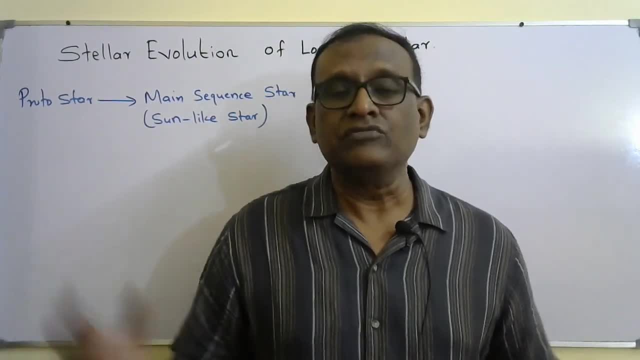 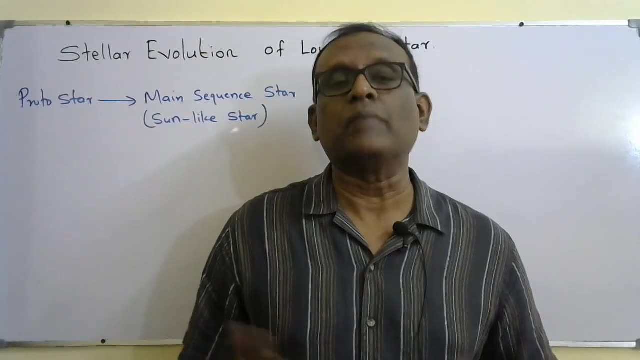 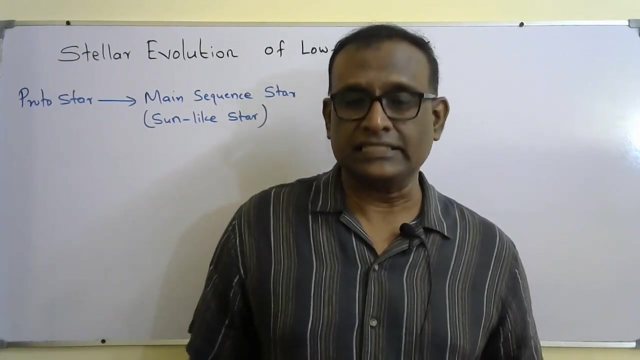 photons emitted from the fusion and the inward gravitational pressure due to the mass of the star. these two force. these two pressures will balance each other. so remember that when a star is in the main sequence, these two pressures will balance each other. so the star will stay in the 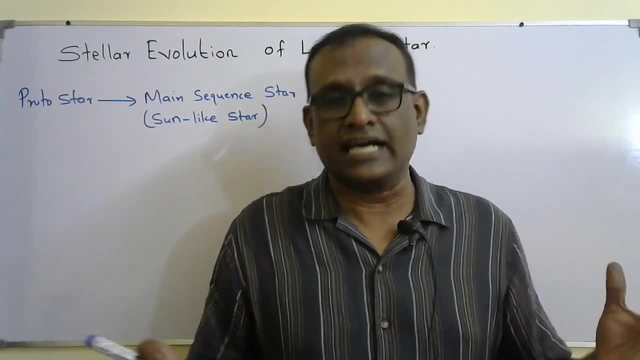 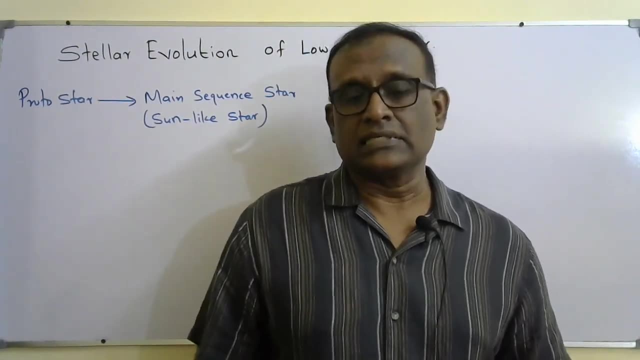 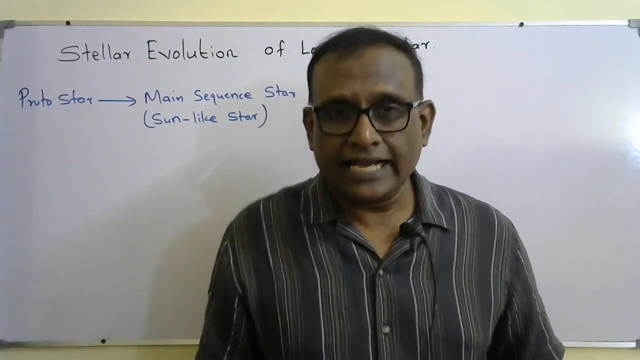 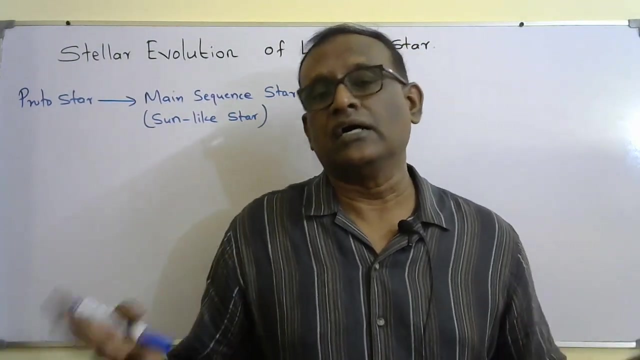 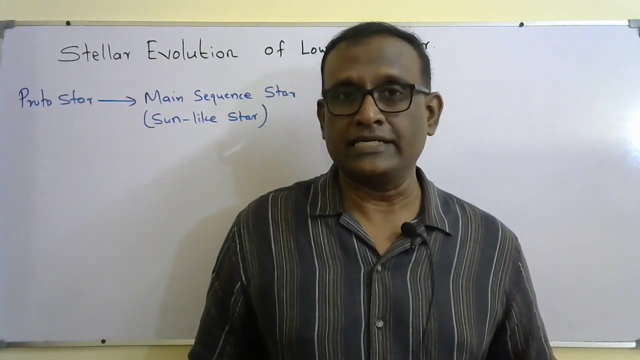 main sequence, without any change in its size or other properties. the temperature also will remain almost the constant. then what happens when the star, you know, the co-hydrogen fusion occurs? when the hydrogen is fused, the outcome or the product will be helium, so gradually the hydrogen molecules in its core will decrease. and when the hydrogen is exhausted, what happens? 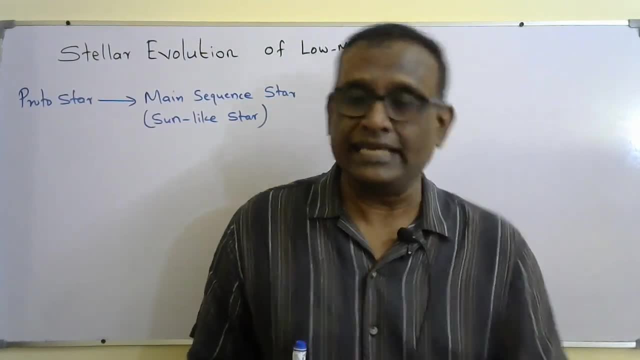 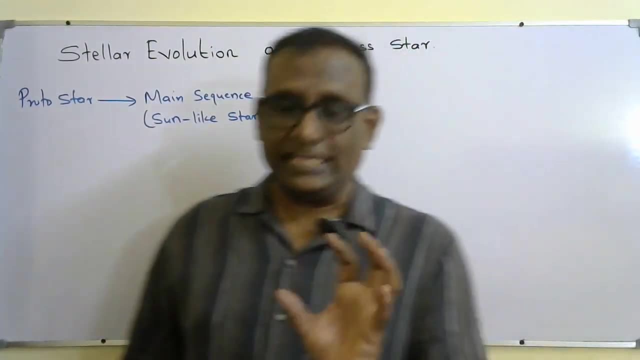 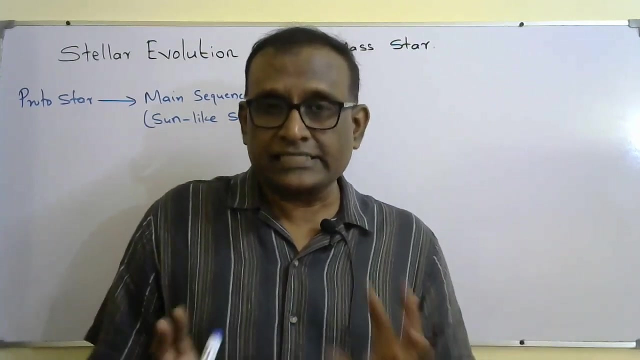 the core will be mainly occupied by helium. there could be a little bit of hydrogen in the outer layer of the core, but core will be occupied by helium when the hydrogen is exhausted. so there's no much further outward radiational pressure inside the core. so the core will 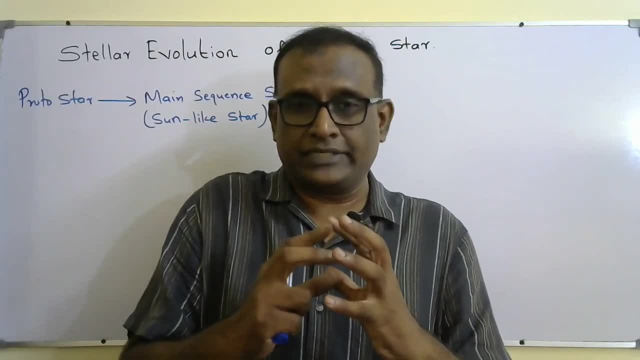 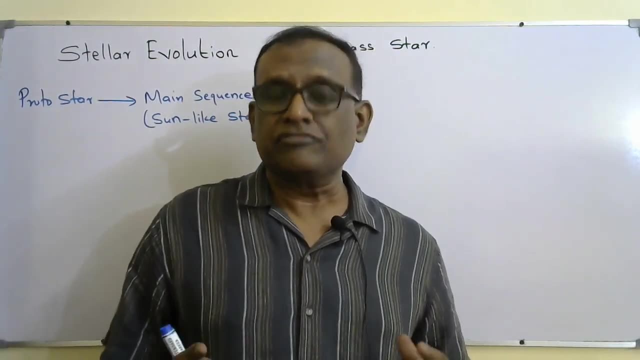 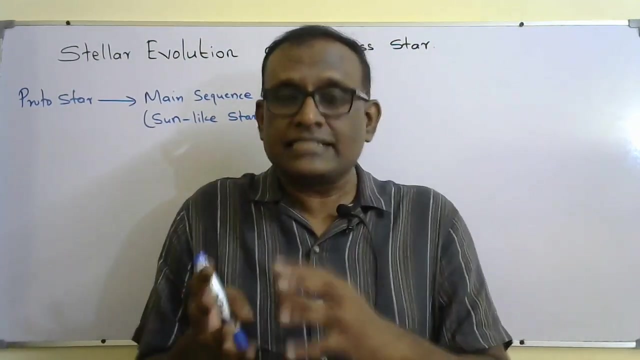 shrink. when the core shrinks, what happens? the temperature of the core will increase and the rate of fusion becomes less so. this, since the rate of fusion becomes less, the star, the temperature of the star, will decrease. so that means in this state, the star is leaving the main sequence. so until 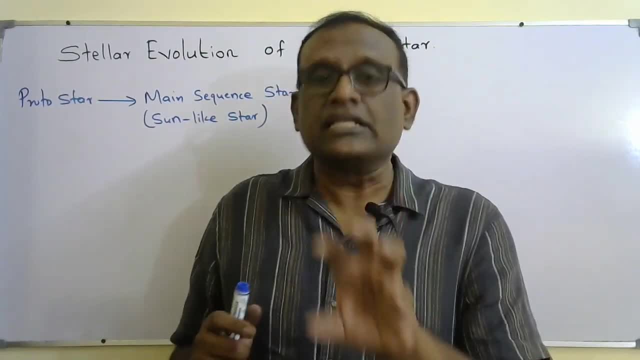 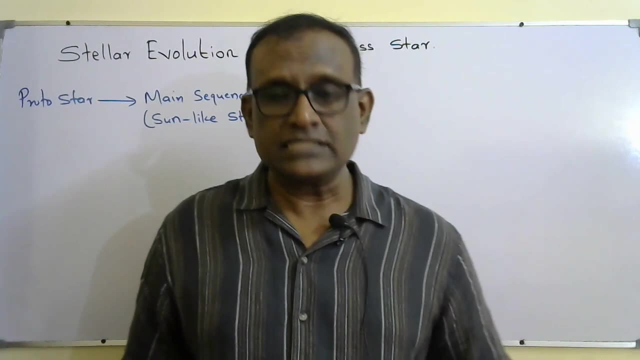 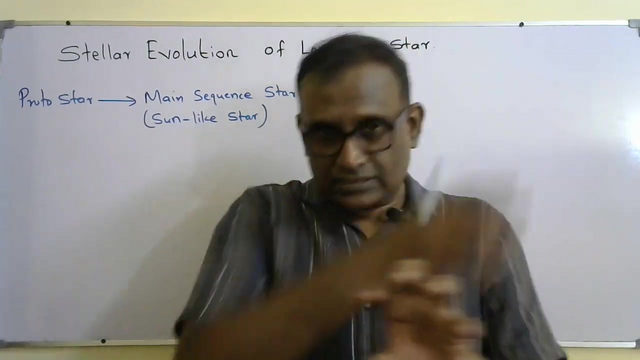 hydrogen occupies in the core and the significant fusion in the core is hydrogen. the star will be in the main sequence. so when the hydrogen is exhausted, core will be occupied by helium. there could be a certain amount of hydrogen in the outer layer or next layer of the 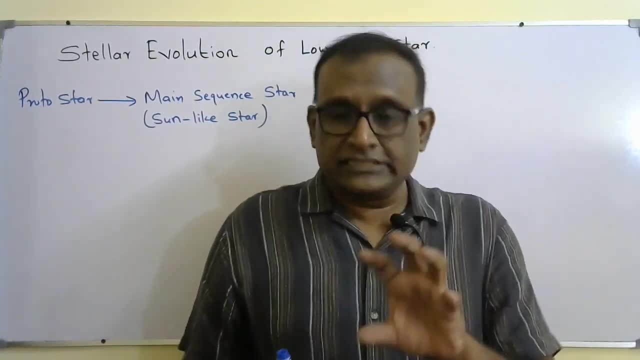 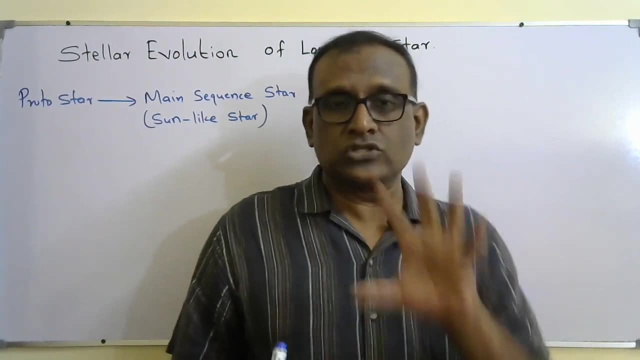 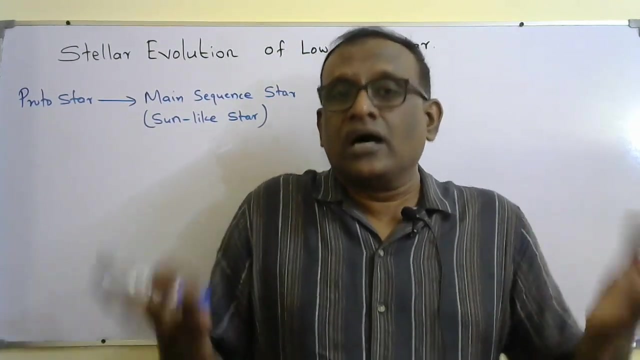 core. but inside the core there won't be any hydrogen fusion and helium fusion not yet started. so what happens? there is no outward radiational pressure, so the core will shrink due to the inward gravitational pressure and due to the less amount of radiation, the temperature of the star will decrease. when the temperature of the star decreases and 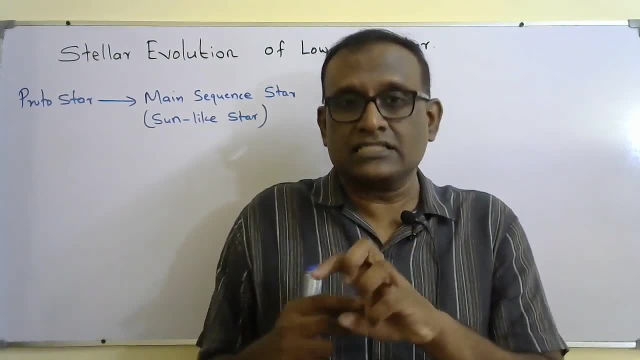 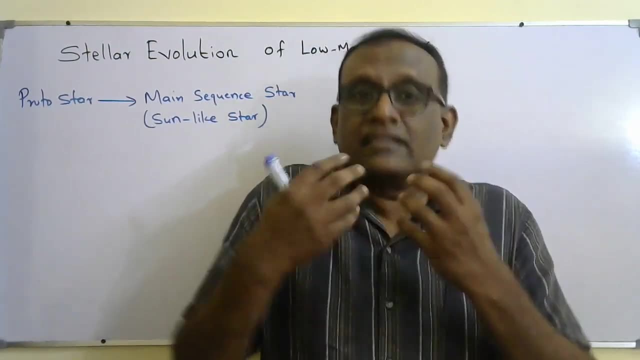 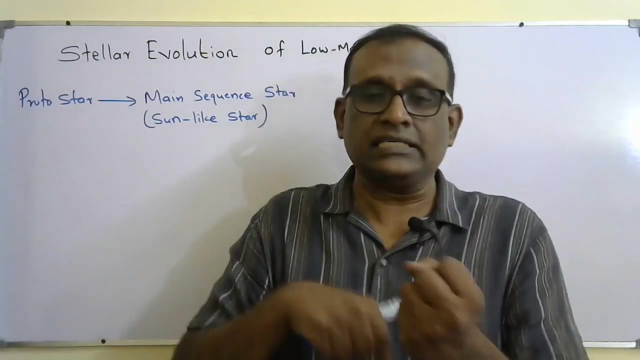 the core will shrink. when the core shrinks, you know, whenever a gas is compressed like that, when the core shrinks again, the temperature will increase and that temperature will fuse the hydrogen gas in the outer layer of the core. due to this hydrogen fusion happening in the outer layer, what 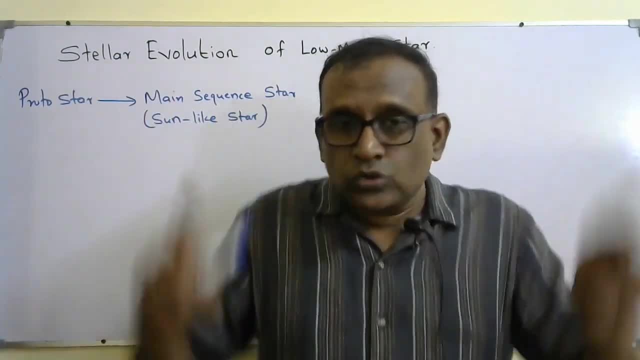 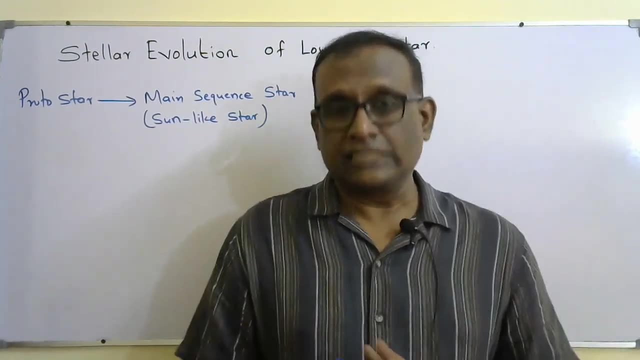 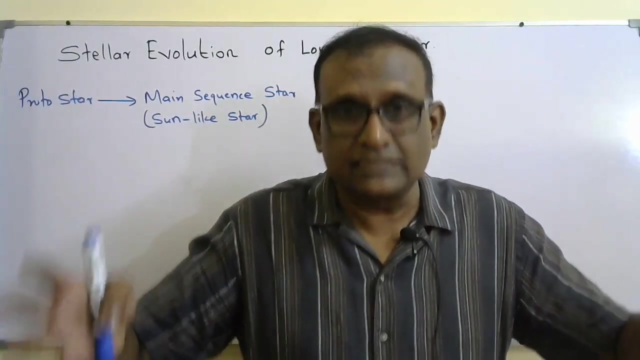 happens, there will be output radiation pressure from the outer layer, which is outside the core. due to that fusion- hydrogen fusion- outward radiation pressure will be emitted. that will make the outer layer to expand and the star will become giant. that is called red giant. okay, so when the star becomes red, 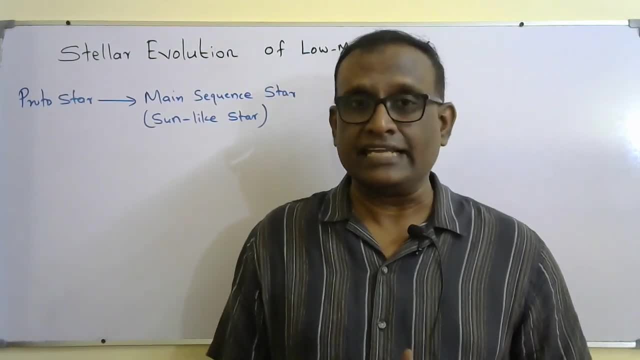 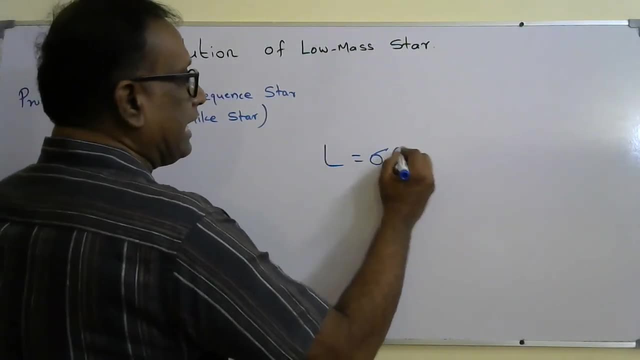 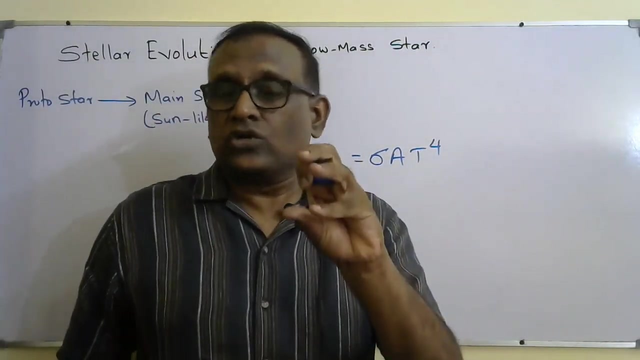 giant. what happens? the amount of increase in surface area will be very large. therefore, according to Stefan Boltzmann law n equals sigma a, t to the power 4. the temperature will decrease. I told that the hydrogen fusion inside the core is not much enough. so the star? there could be a little bit of hydrogen fusion in the outer layer when. 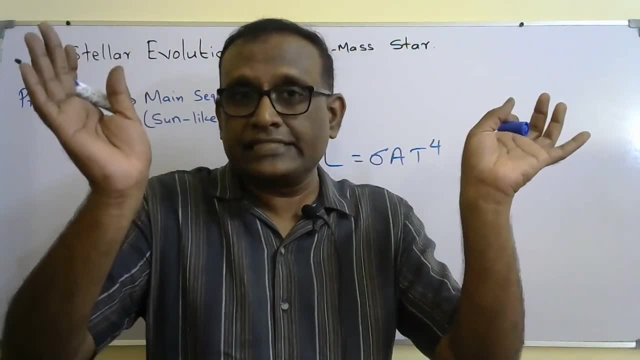 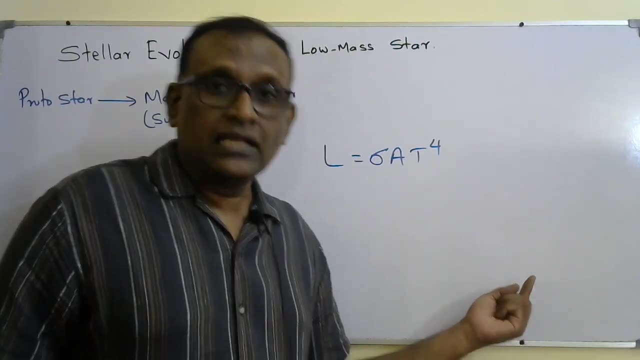 the core shrinks, it emits radiation. it emits temperature. that temperature will be used, or heat will be used in the outer layer. when the core shrinks, it emits radiation. it emits temperature. that temperature will be used, or heat will be used to fuse the hydrogen in the outer layer. because of that hydrogen fusion in the outer layer. there will be outward radiation pressure that will cause the outer layer of the star to expand, so the star will become much larger. the increasing surface area is very high. very large amount of increase happens in the surface area. because of that, luminosity will increase. temperature is. 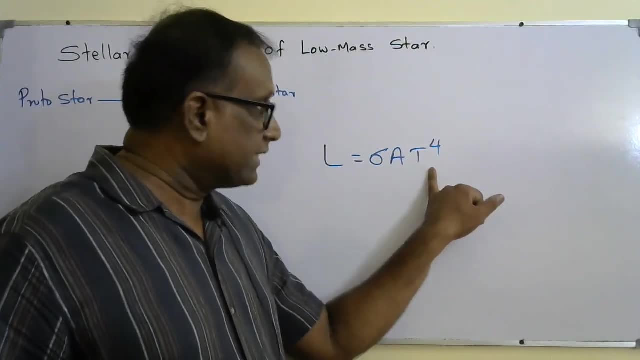 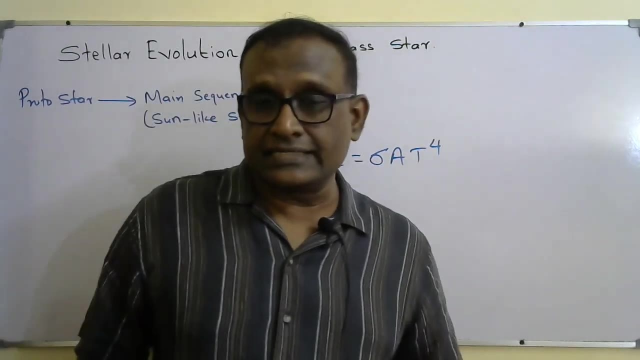 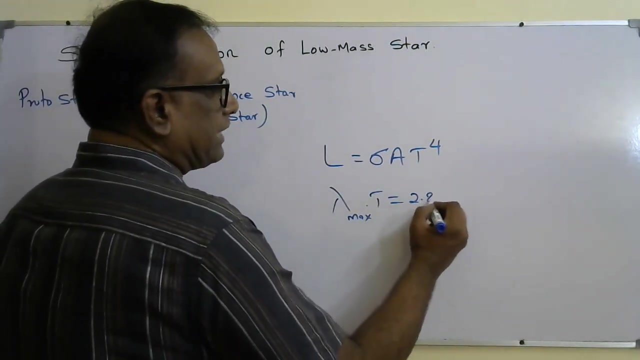 decreasing surface area increases is increasing temperature. decreasing surface area, increasing luminosity also will increase, Since the temperature is decreasing. according to Wien's law, the constant that is 2.898, 10 to the power minus 3 according to Wien's law. what? 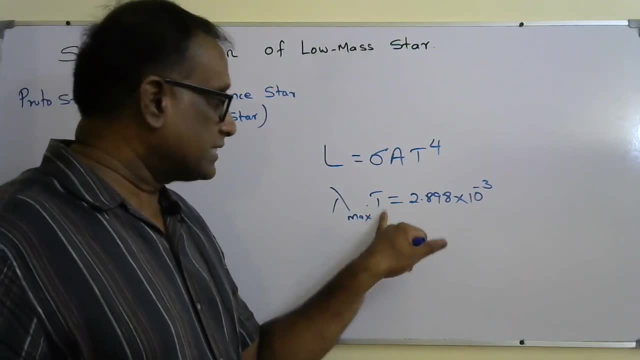 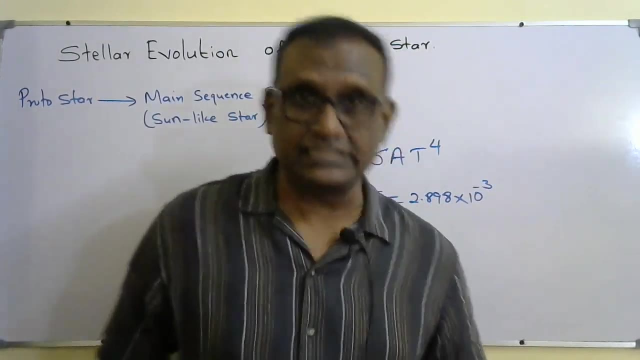 happens, The lambda max will increase because T is decreasing. the star will become more reddish. the star will become red color. we call it as red giant. so after the wien's sequätt state, the star will become red giant. So when that happens. red giant state occurs when the core is occupied by helium and inside the core there is no hydrogen fusion. so core is shrinking but there could be little bit of hydrogen fusion in the outer layer. When the core shrinks, the temperature of the core will increase and heat will be radiated. that heat will fuse. hydrogen in the outer layer and there will be outward radiation pressure from the outer layer of hydrogen in the outer layer. that will cause the outer layer to expand. that's the reason the surface area of the star becomes much larger. so when the surface area becomes larger, luminosity 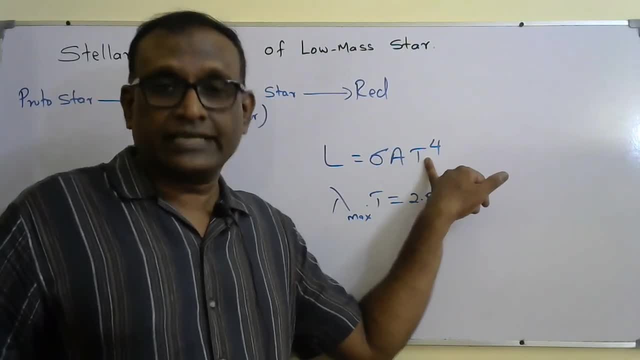 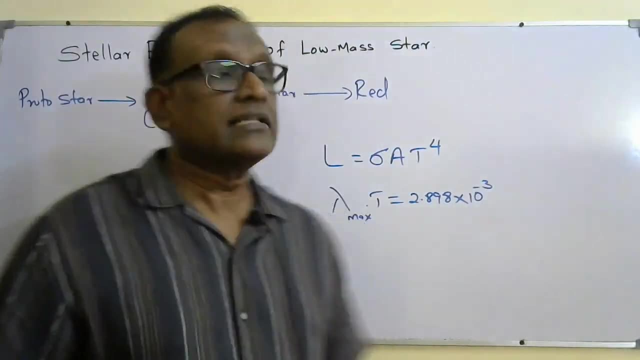 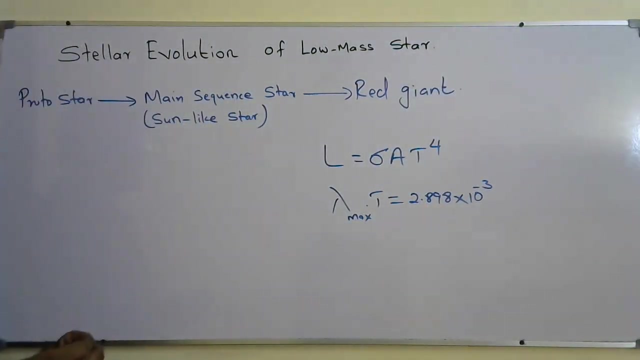 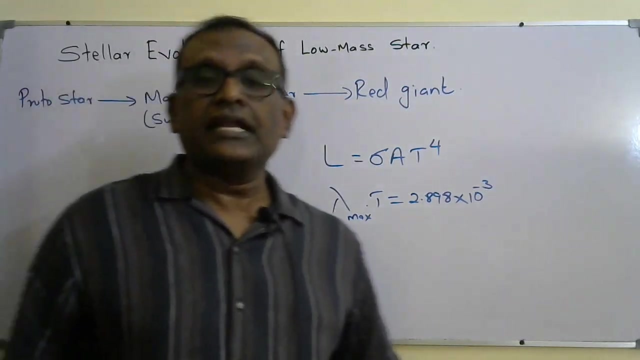 becomes much higher the temperature I told already decreasing. so the temperature reduces, lambda max increases. star will become red and very big. that is called red giant. okay, so it could be in millions of years in the state of red giant. now what happens now inside the core? I told that core is shrinking. Heat produced. the temperature increases heat produced. That heat will be able to fuse the helium. so when the helium fusion becomes Significant inside the core, the outward radiation pressure will become very large and the outer Layer of the core will be thrown away Into the space and that will cause planetary nebula. So When the helium fusion becomes significant in the core, the amount of energy radiated due to Helium fusion is very high. outward radiation pressure becomes very large and that Throws away the outer layer of the star. So the outer layer will be thrown away into the space and that will form planetary nebula. 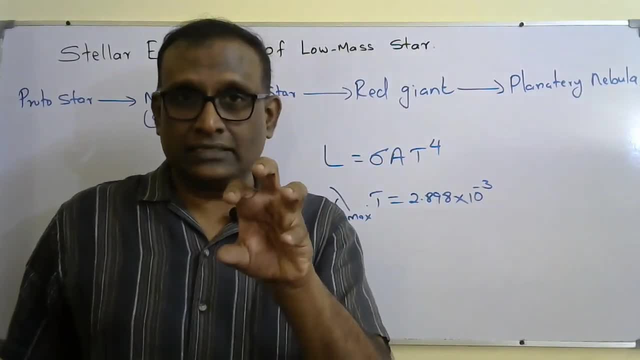 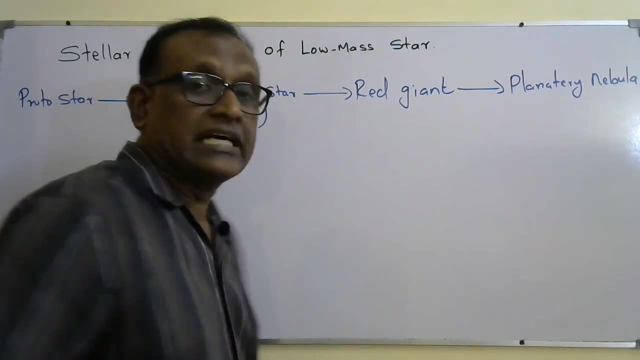 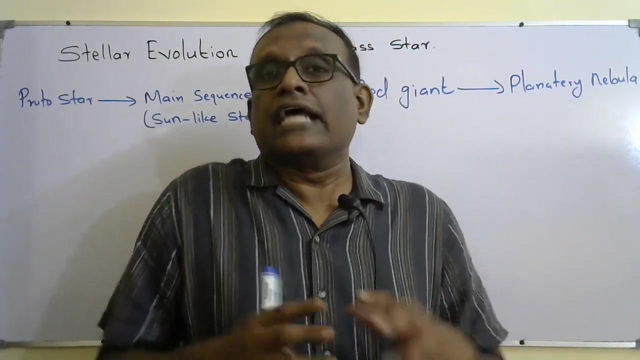 So after that only the core will remain. Now, when the core remains after throwing the outer layer, The core has not enough mass to continue the fusion, So the fusion inside the core will be sustained, no further fusion. So there is no outward radiation pressure from the core. when it comes to the planetary nebula state, 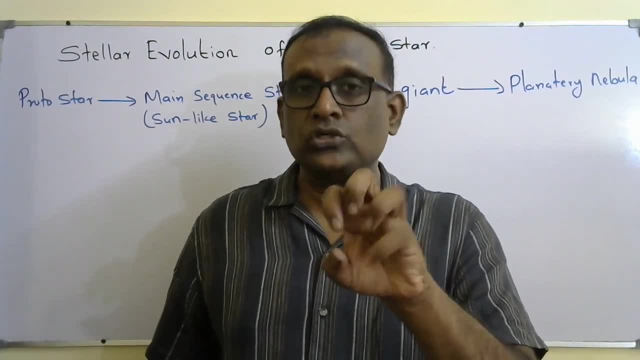 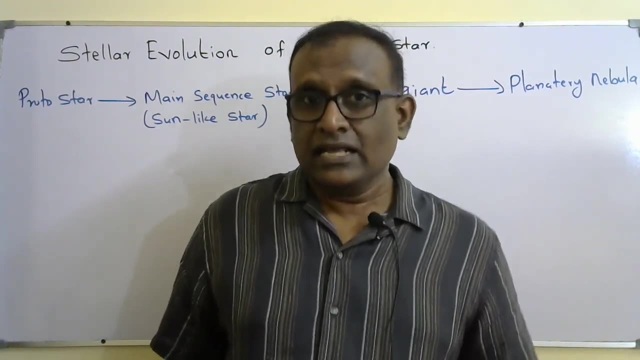 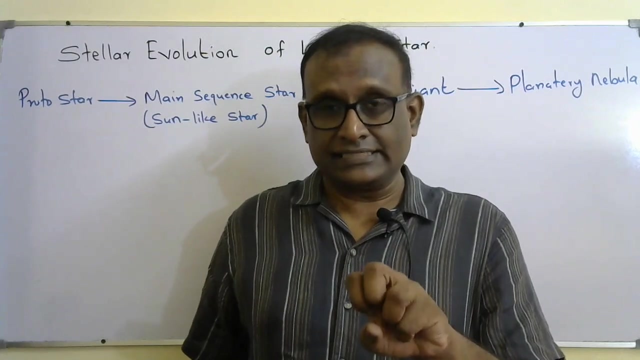 No outward radiation pressure, the core will shrink due to much larger inward gravitational pressure. So when it shrinks, what happens? the temperature will increase and it will become white color. So it will become white color much smaller due to inward gravitational pressure. So that is called white dwarf. 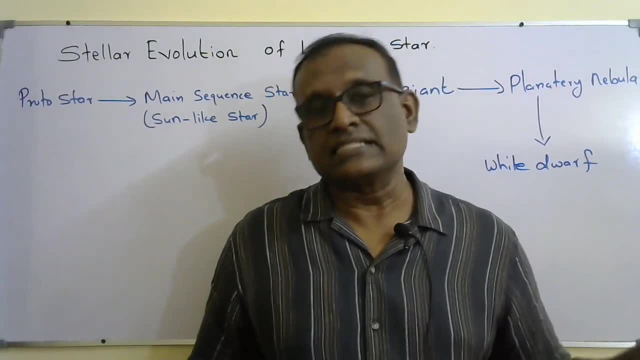 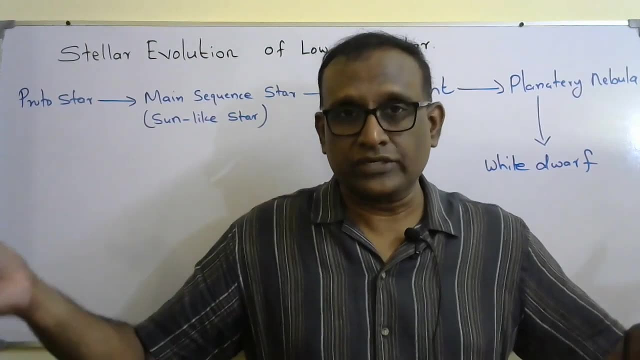 Okay, so when the star becomes white dwarf, that is the final state. but it will emit radiation Due to the temperature to the surrounding. so no further fusion reaction. due to the temperature, it appears like a fainted white color. Due to the temperature, it appears like a fainted white color. 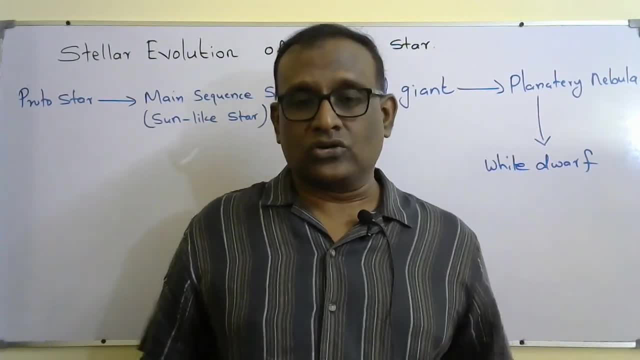 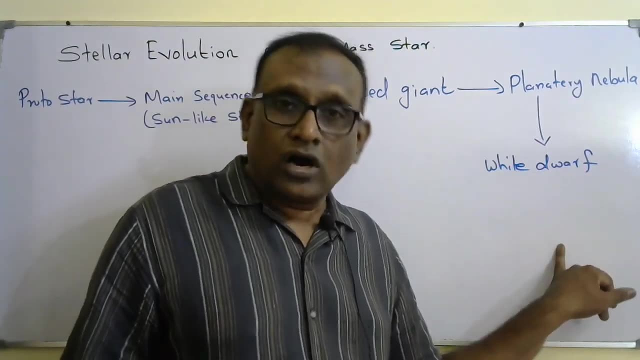 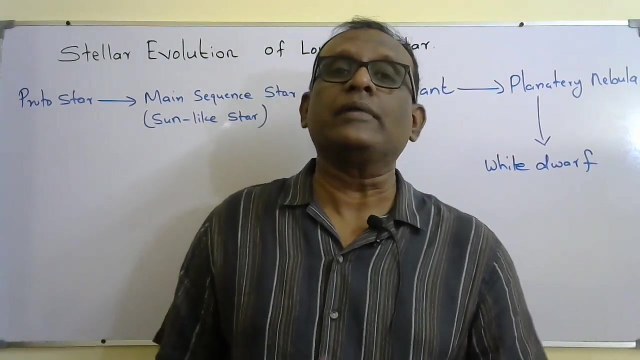 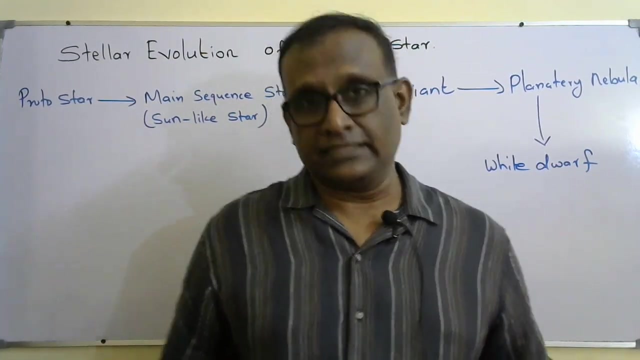 but gradually, When it lose heat to the surrounding, the intensity of that white color can decrease And later the white dwarf will become brown dwarf and finally become black dwarf. So theoretical Model says the time required to become black dwarf is more than The current age of the universe. so there are no black dwarfs in the universe. 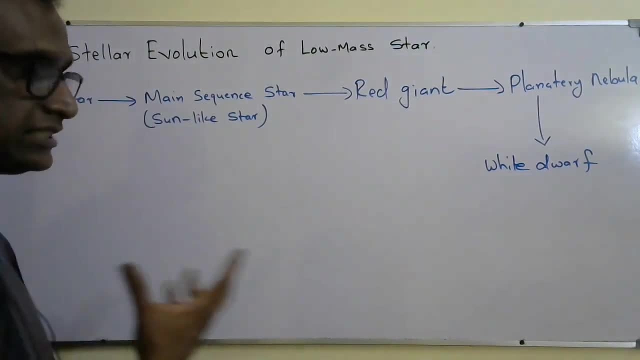 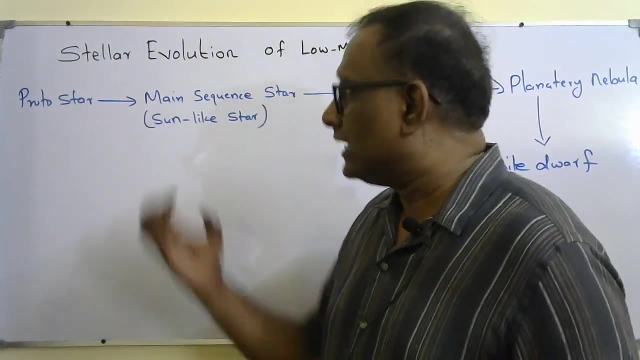 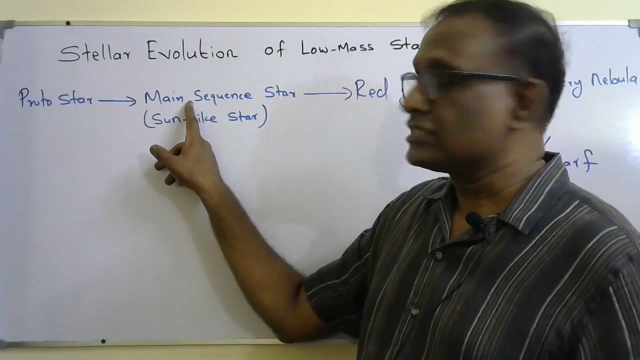 Okay, again, so quickly we'll compare. this is the initial stage of the star where the hydrogen fusion is Starting. when it accumulates more and more hydrogen nucleus, the mass will increase and there will be significant hydrogen Fusion in its core. that is the main sequence. It could be in the main sequence for several millions of years, depending on the mass. It could slightly, it will vary. 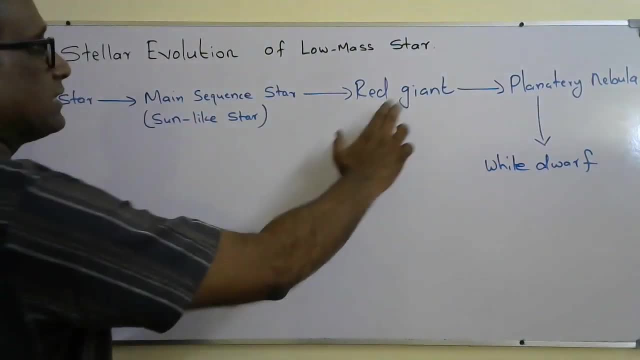 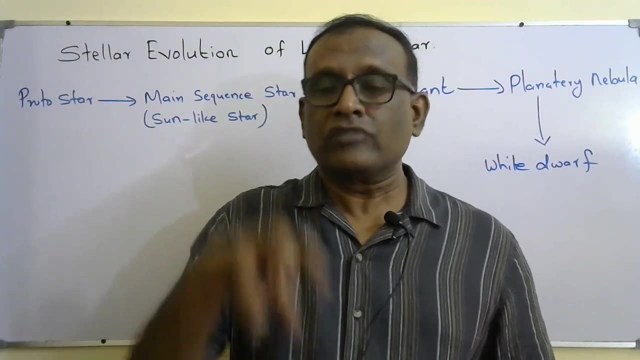 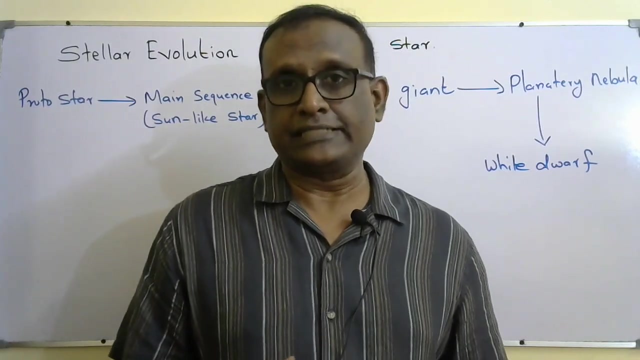 Okay, so then the red giant star occurs. What's the difference between red giant star and main sequence star? So when a star is in the main sequence, significant amount of hydrogen fusion occurs in its core. Outward radiation pressure will be balanced by inward gravitational pressure. 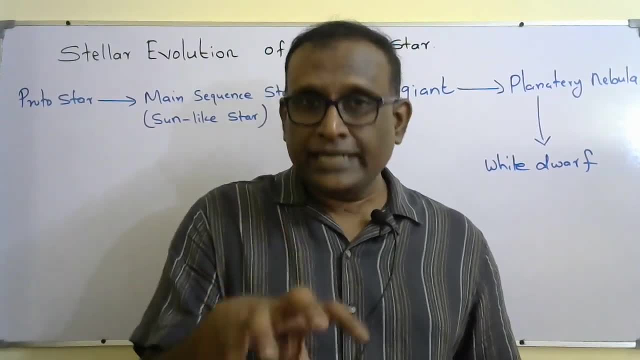 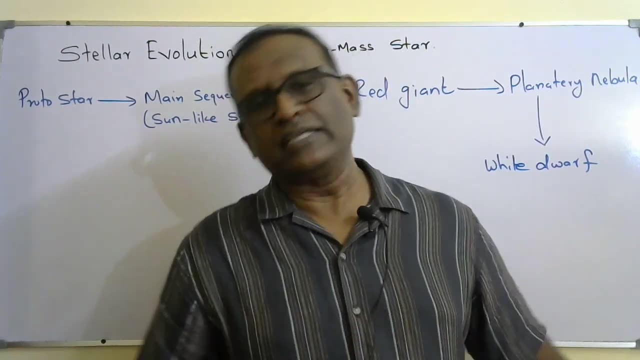 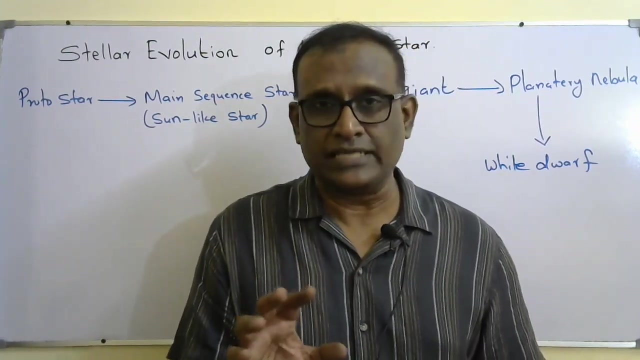 So when it is in the main sequence the state will remain same. the property of the star will remain Unchanged. its luminosity, temperature, all will remain unchanged. But when we consider millions of years there could be slight difference variations. But generally we can say: when a star is in the main sequence, it properties remains unchanged. 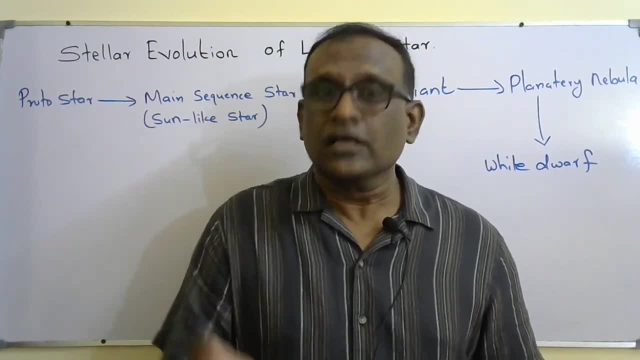 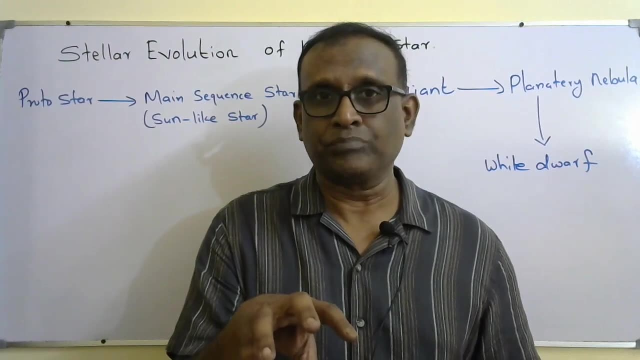 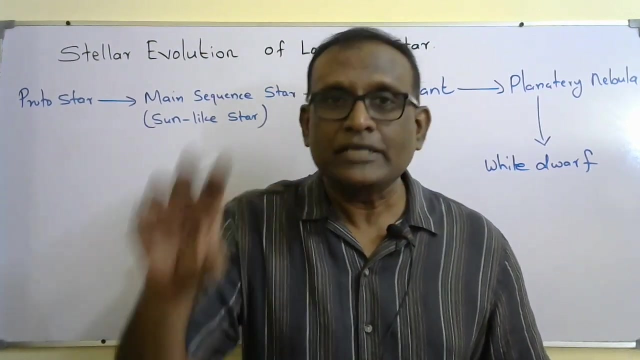 So when the hydrogen is exhaust- You know, when hydrogen is fused- helium will be produced. when the hydrogen is exhaust, core will be occupied by helium. there could be little amount of hydrogen in the outer layer of The core. there could be little bit of hydrogen. fusion occurs in the outer layer. So in case, 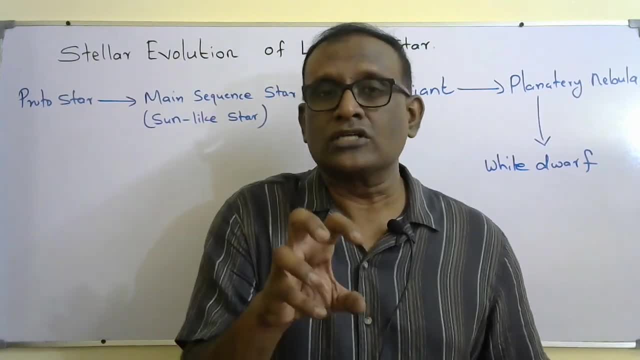 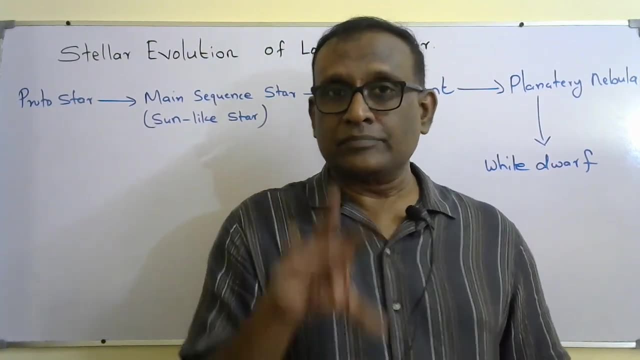 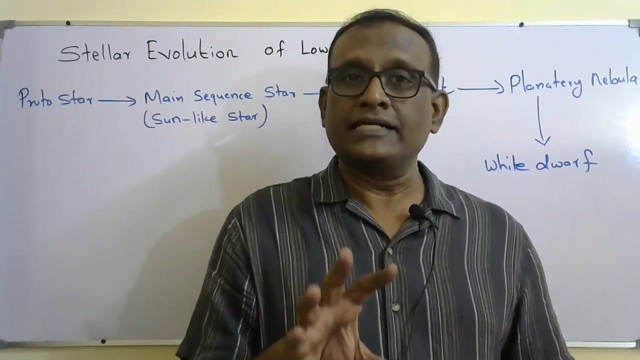 That time what happens? the core will shrink. because the core has no fusion, no outward radiation pressure, but it has Large amount of inward gravitational pressure. So the core will shrink due to inward gravitational pressure. when it shrinks, when a gas is compressed, What happens? pressure increases. that will cause the temperature to increase. so temperature of the core will increase. 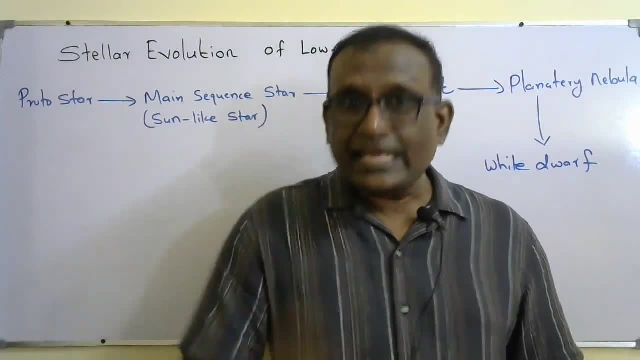 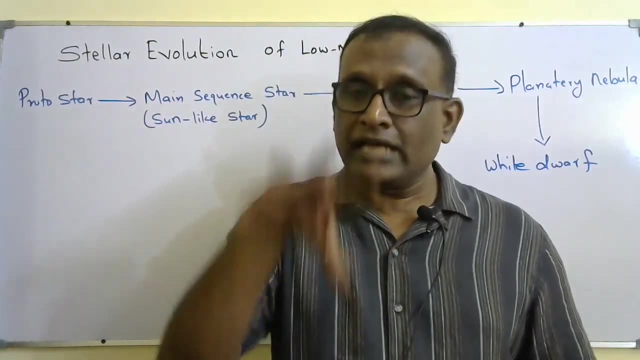 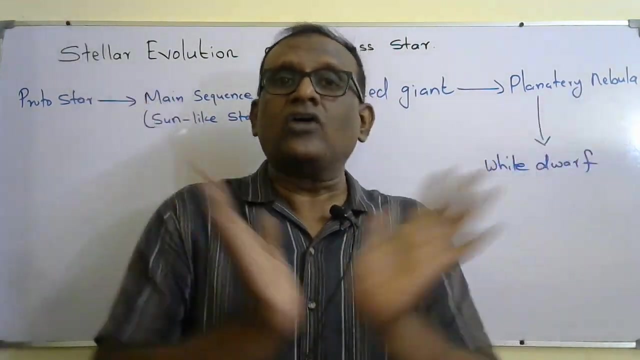 But the temperature of the core increases, it will radiate heat and that heat will support the hydrogen fusion In the outer layer of the core. so there will be hydrogen fusion is outer layer of the core, So that hydrogen fusion in the outer layer will give out outward radiation pressure and exert force on the outer layer. 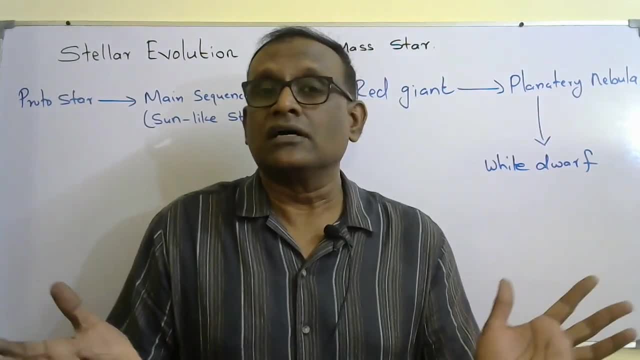 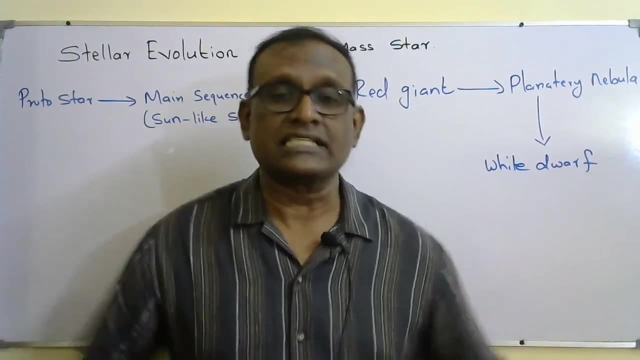 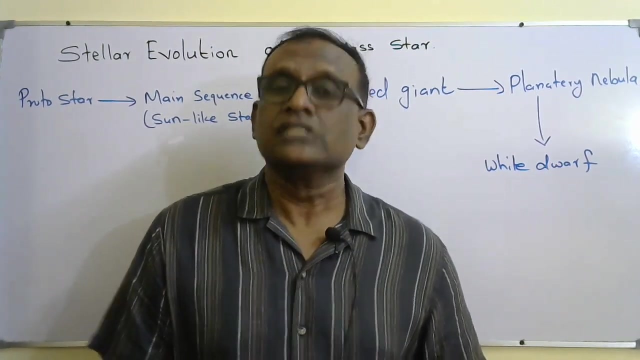 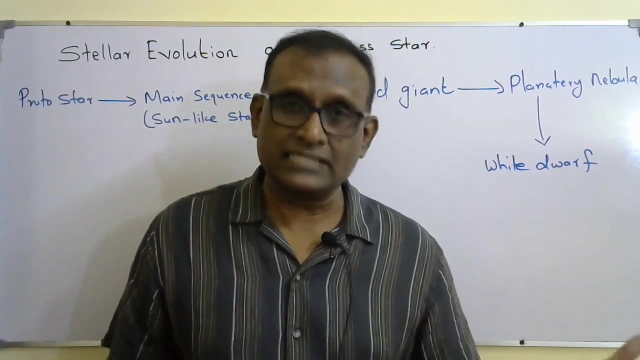 of the gases. then what happens? the outer layer will expand, weather layer expands. it will becomes giant, huge surface area. but the temperature is low because there is no significant amount of hydrogen fusion and helium fusion not yet started, so it will become red giant. so when it becomes red giant, what happens? the luminosity will be higher because surface area is higher. 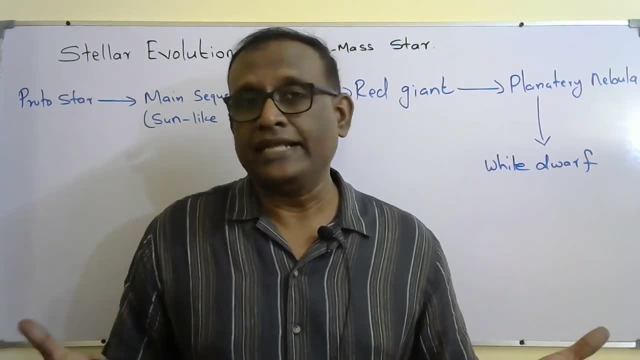 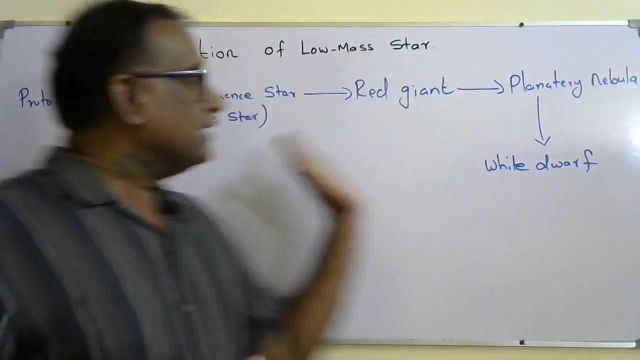 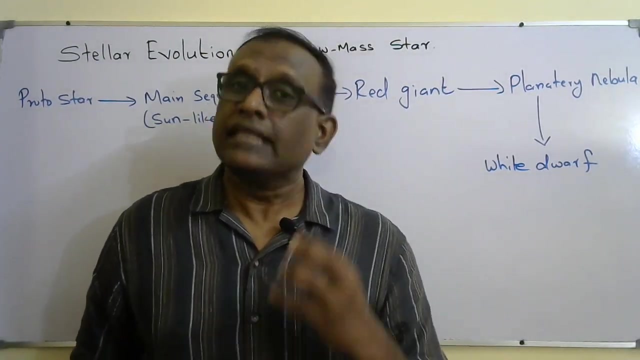 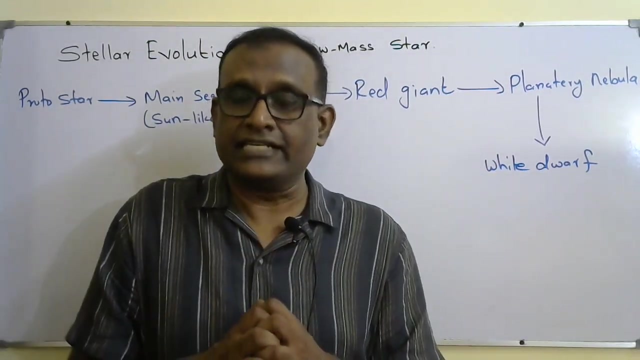 temperature becomes less, so the account of Wien's law lambda max will become larger. it becomes reddish, so it will be leaving the main sequence. but when it becomes red giant state, perfectly red giant state, what happens inside the core? there will be helium fusion, because star will continue, the core will continuously shrink and the temperature increases, and that will support the helium fusion. but when the helium fusion becomes significant, the outward radiation pressure becomes much more, because the energy released during helium fusion is much more compared to hydrogen fusion. so when the core is occupied mainly by helium and when the helium fusion becomes significant, the outward radiation pressure will become. much more compared to inward gravitational pressure. so what happens? due to the large outward radiation pressure, the outer layer of the star will be thrown away into space and that will form planetary nebula. after planetary nebula is formed, the total mass of the star is decreased because outer layer has shrunk. and the outer layer has shrunk. 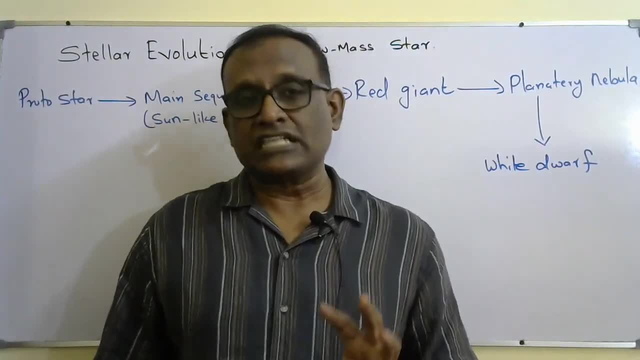 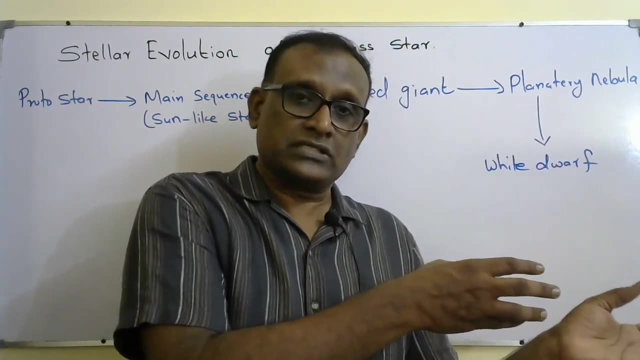 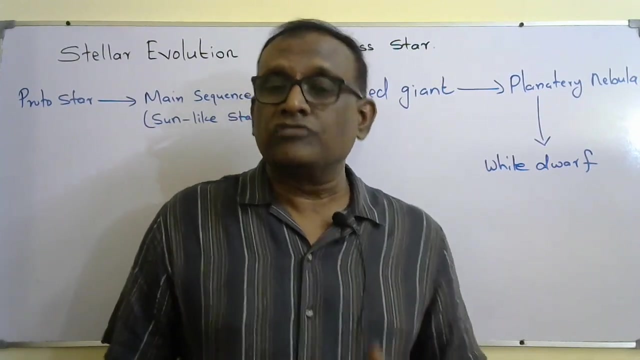 gone, has thrown out. so the mass of the core is not sufficient to produce further fusion of helium. Helium fuses will produce carbon, so there will be carbon also, but it can't fuse the carbon because temperature is not enough. So what happens? there is no further fusion in the core, but there. 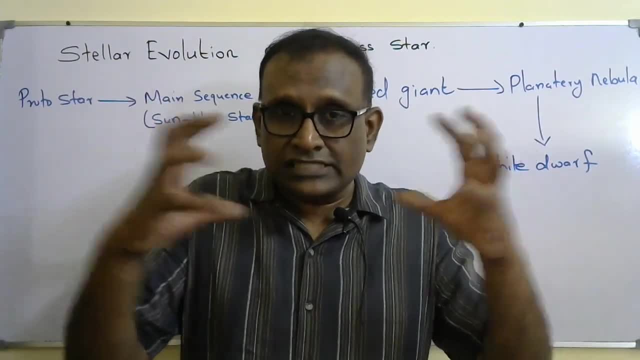 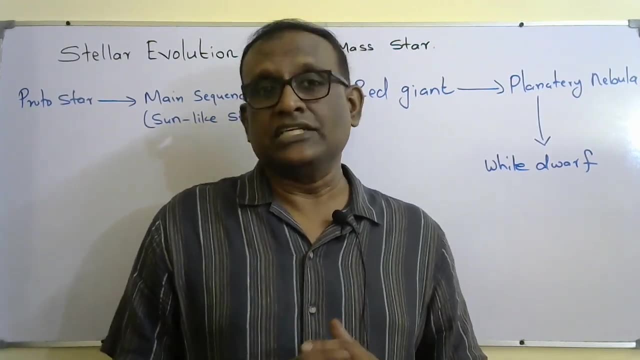 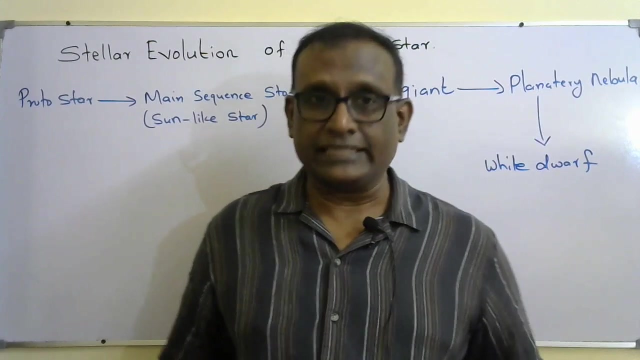 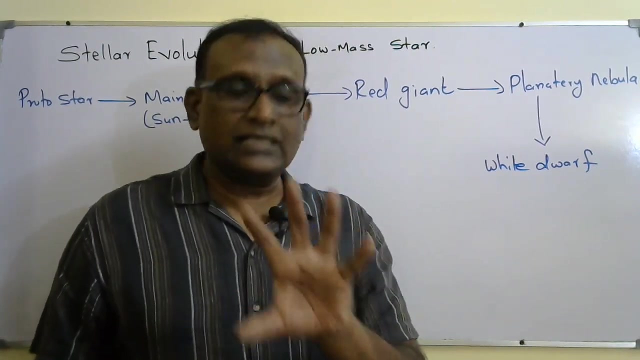 is inward gravitational pressure. the star will shrink. whenever gas shrinks, temperature will increase, so it will become white color. that white color is due to the temperature only, not due to fusion. it's due to the temperature it becomes white color. it emits almost several radiations, so due to that radiation it will become fainted white color. that will become white dwarf. So the 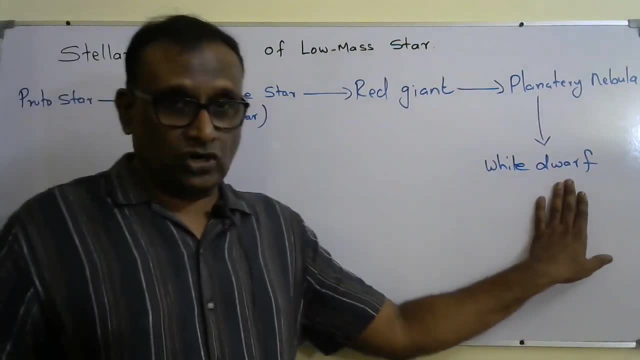 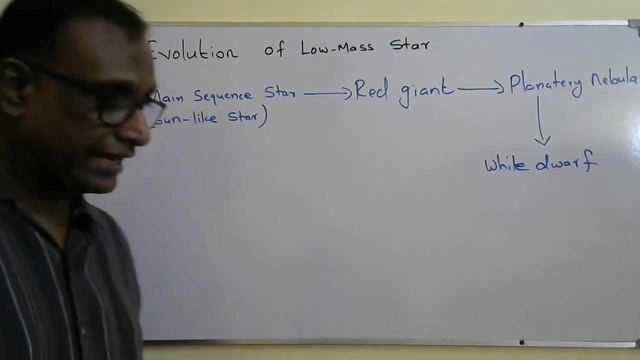 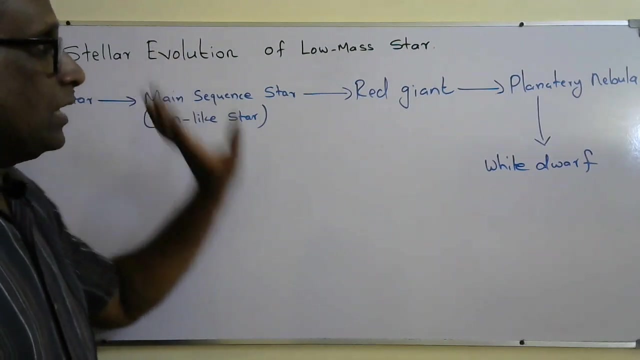 temperature. when you compare the temperature, temperature of the white dwarf is more than temperature when it is in the main signal could have. You can see the chart diagram later. so temperature of the white dwarf is normally more than temperature of the main sequence star. Luminosity of the white dwarf is much lower compared to main. 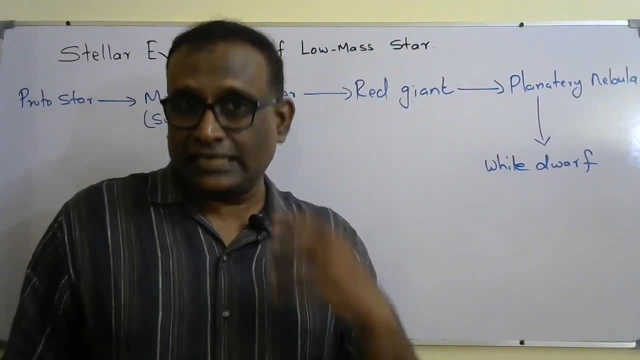 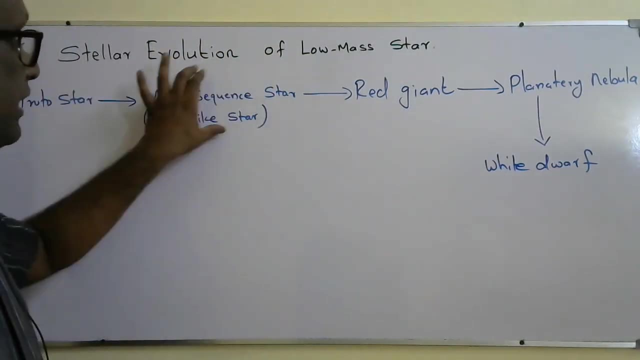 sequence star because the faint light will be emitted. that light is only due to the temperature. So temperature of the white dwarf will be more than temperature of the same star when it was in the main sequence, but the luminosity will be much lower compared to to when it was in the main sequence. When you compare red giant and white dwarf, the 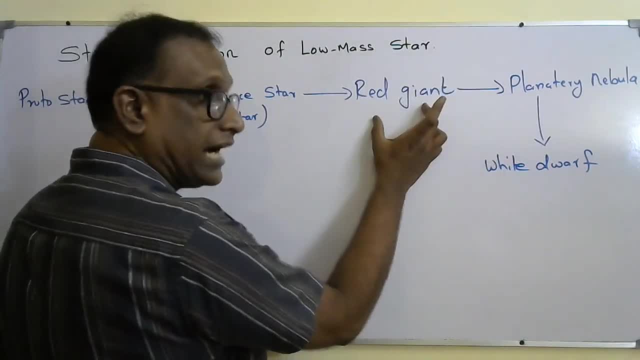 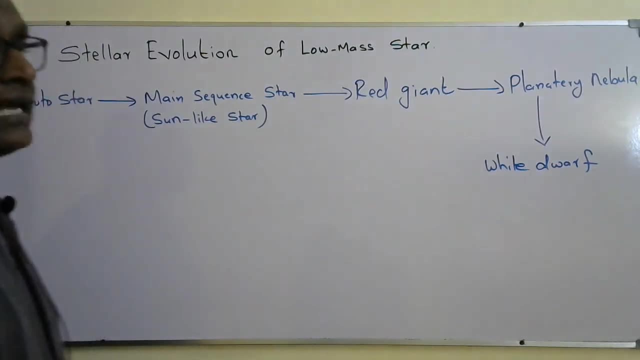 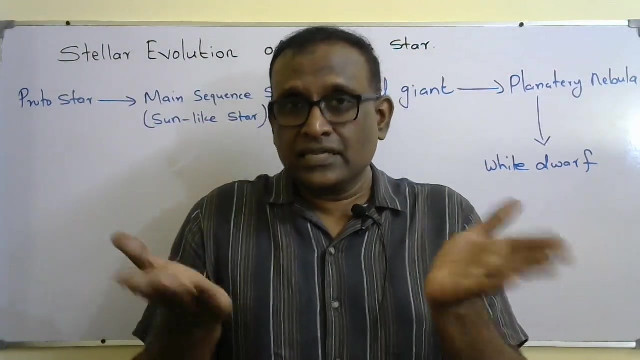 surface area much larger, much smaller surface area. much higher luminosity. much lower luminosity. much lower temperature, much higher temperature. They can ask: what's the similarity between main sequence giant and red giant? Similarity, you can say both have hydrogen fusion. but difference: Hydrogen fusion occurs in the core. 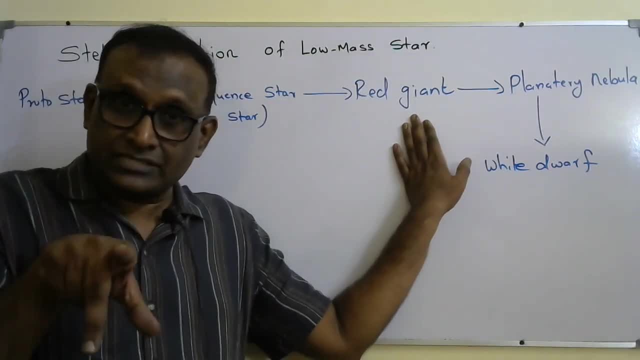 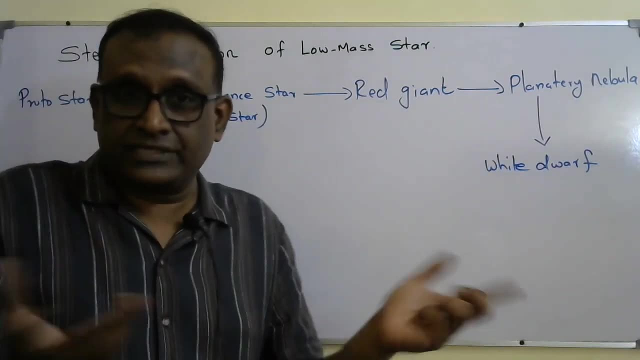 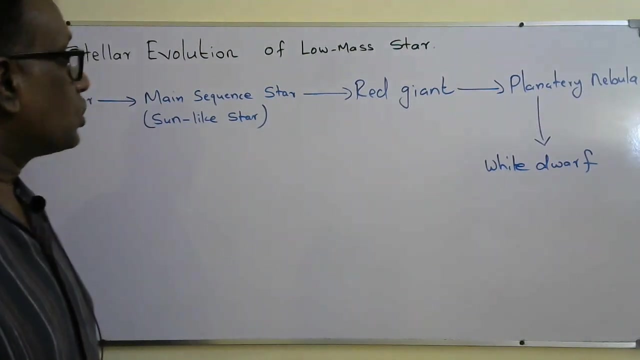 hydrogen fusion occurs in the outer layer. Careful, the difference means Similarity, means both have hydrogen fusion. But where the hydrogen fusion occurs is the difference. here the hydrogen fusion occurs in the core, here hydrogen fusion occurs in the outer layer. So those other 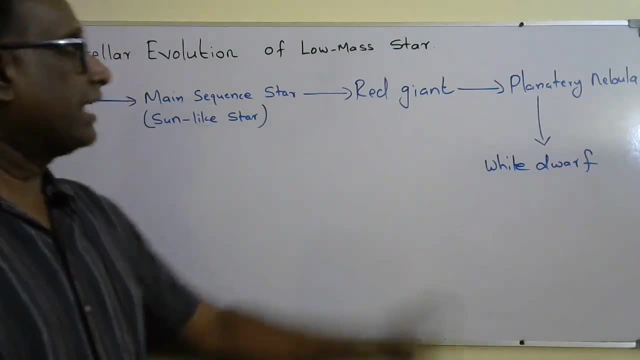 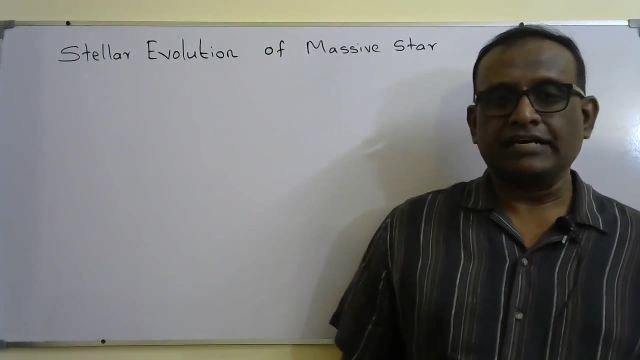 similarities and differences between main sequence And the red giant. Okay, so next thing is about Stebbler Evaluation of Cross-Chipphynologyowed Picture and Injection massive star. that also, you know. massive star means if the mass of the star is more than 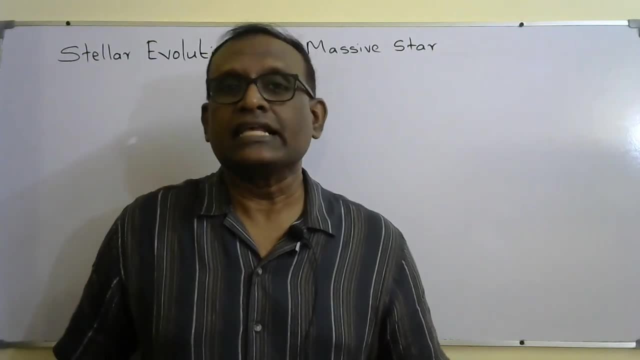 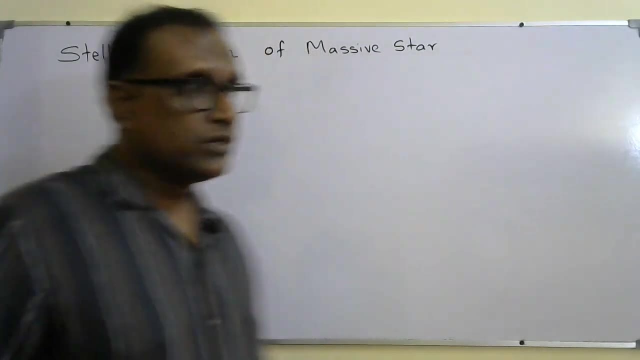 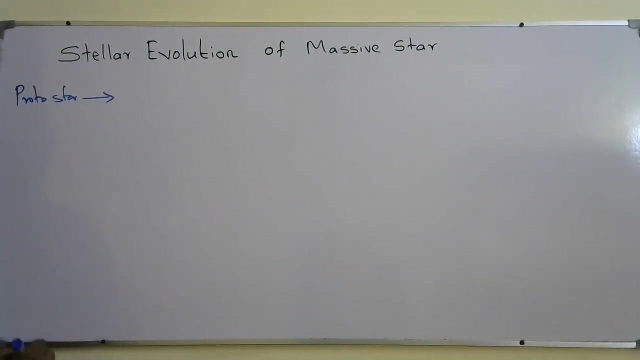 four times the solar mass. you know what's the specialty? they are the invert. gravitational pressure will be much higher, so the rate of fusion will be much higher. right, so here also, the initial state is the protostar, so when it gets more and more hydrogen nuclear, it will become main. 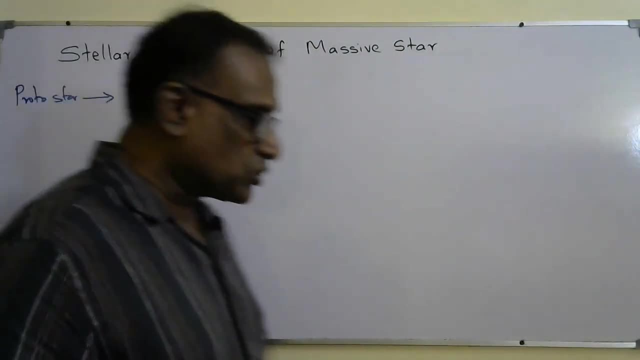 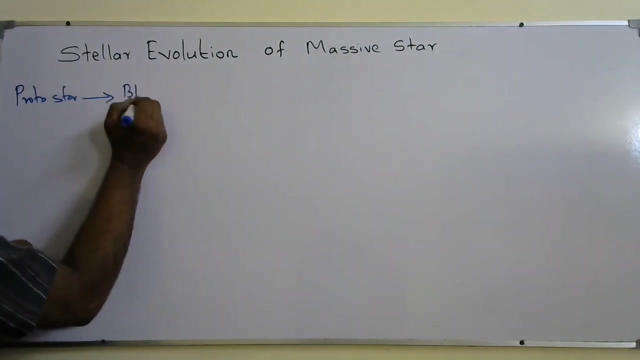 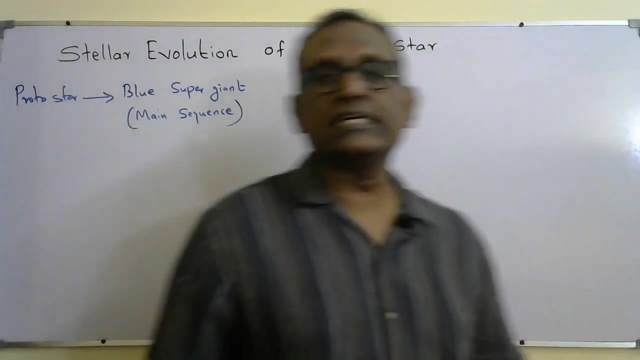 sequence star. so the main sequence star is called blue supergiant. is called blue supergiant because massive and much larger, so it's called blue supergiant. so that is the main sequence star. so in this state, here also inside the nucleus, there will be a significant amount of hydrogen. 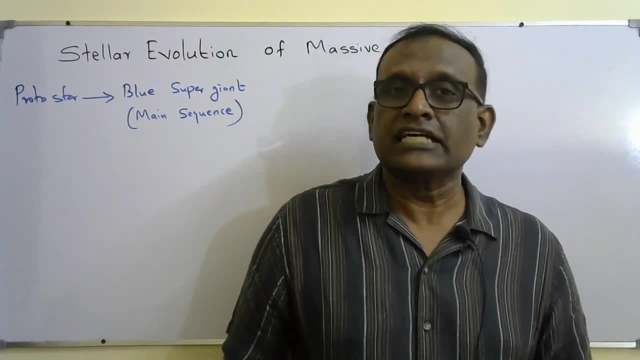 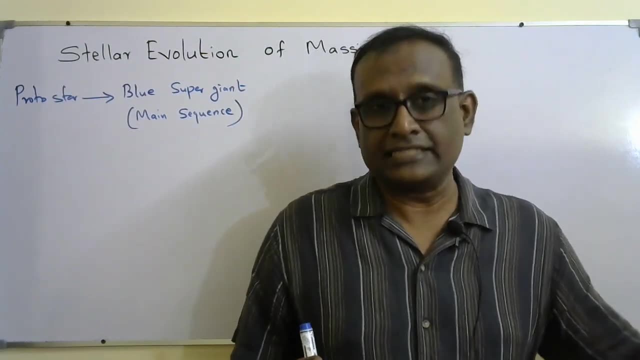 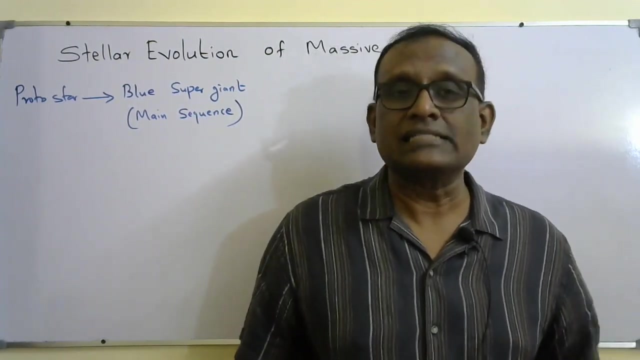 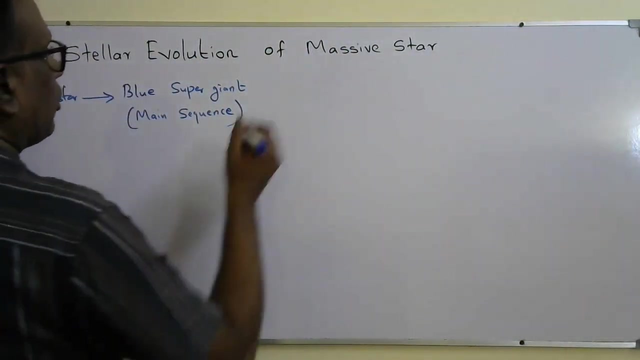 fusion occurs. but when the hydrogen fusion is completely used up or exhaust, helium will be occupied. the star will leave the main sequence. so, as i explained in the loma star, when it becomes, when it leaves the main sequence, it will become red giant. same explanation. so red giant means here we call some books, they call 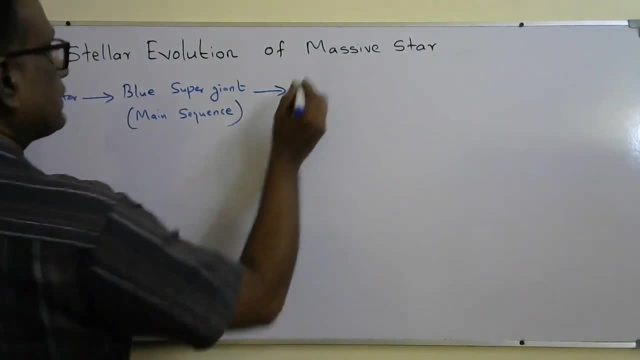 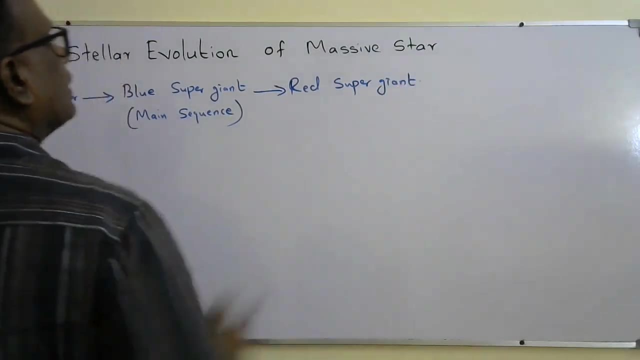 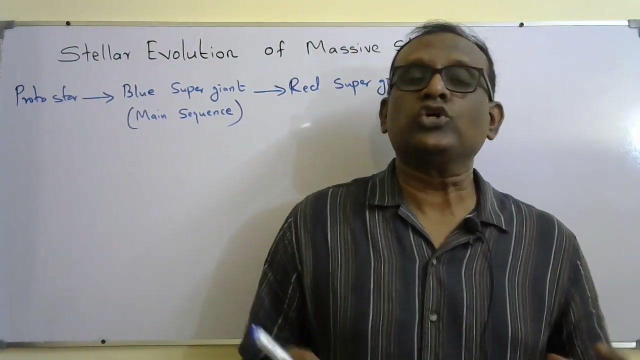 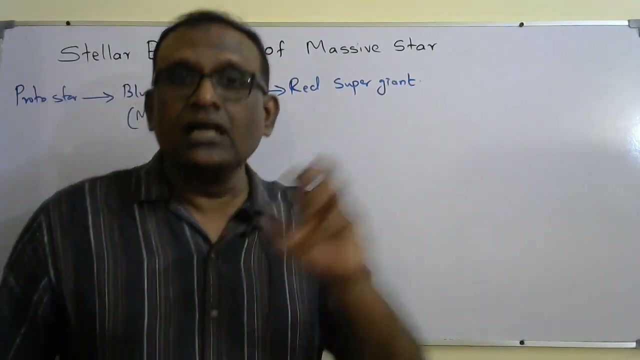 red supergiant or some books they call red giant. okay, but here the difference is the star has very high mass, so it could be in the red supergiant state inside the core until iron is formed. you know, when hydrogen is fused it will become helium. 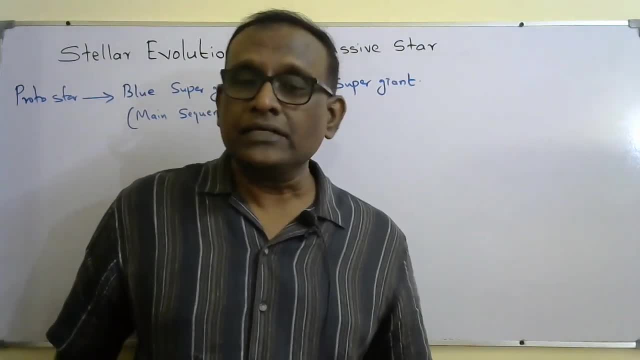 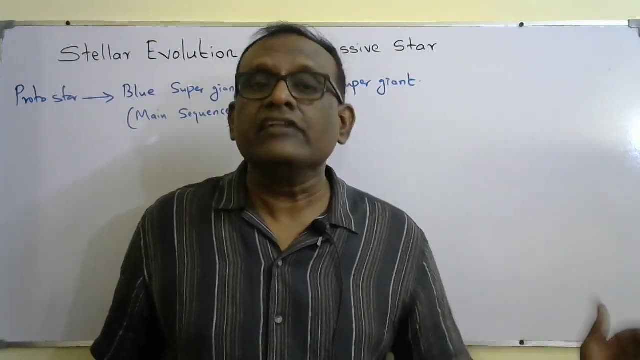 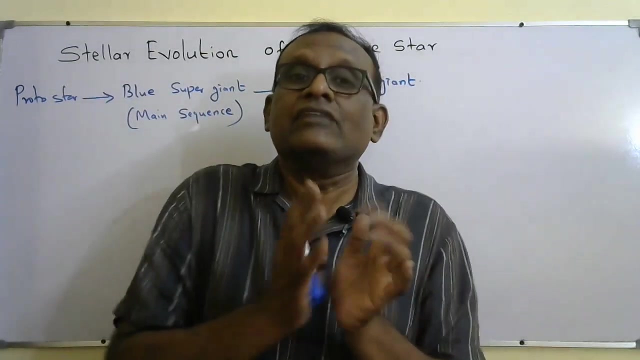 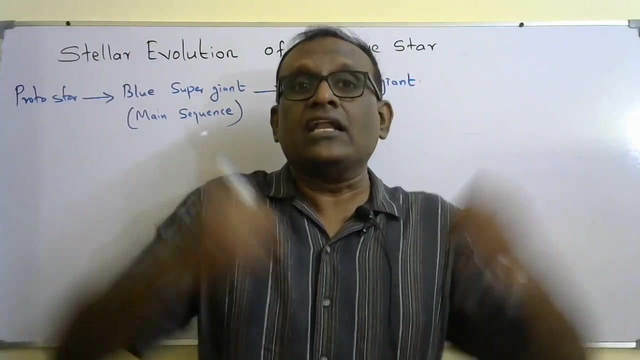 when helium is fused, it will become carbon, like that when carbon is, you don't need to remember. like all the outcomes of fusion, right? the? finally, iron will be formed. until iron is formed, the red supergiant can withstand even very high amount of outward radiation pressure. it can withstand because it has very large 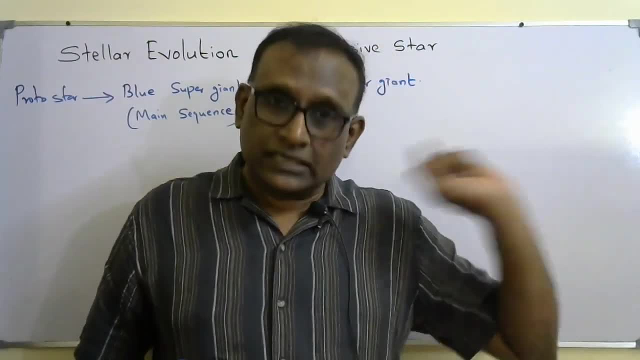 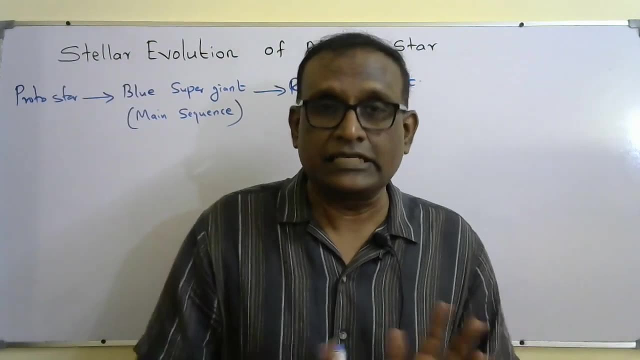 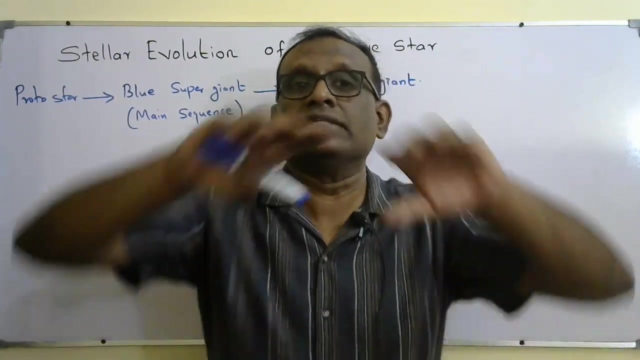 inward gravitational pressure. but when you compare the super red giant of low master, it was unable to withstand for the outward radiation pressure given by amount of helium fusion from the core. it was unable to withstand. so that's the reason it threw away the outer layer and formed planetary nebula. i'm talking about the low master, but in 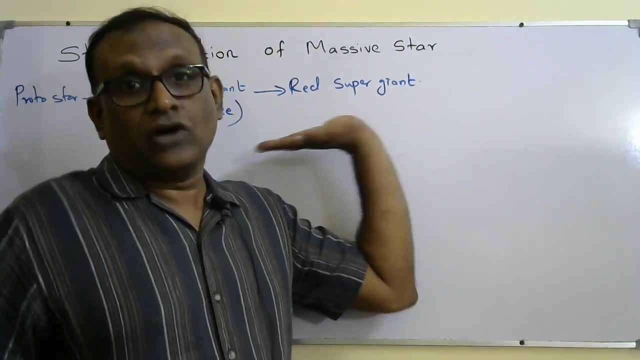 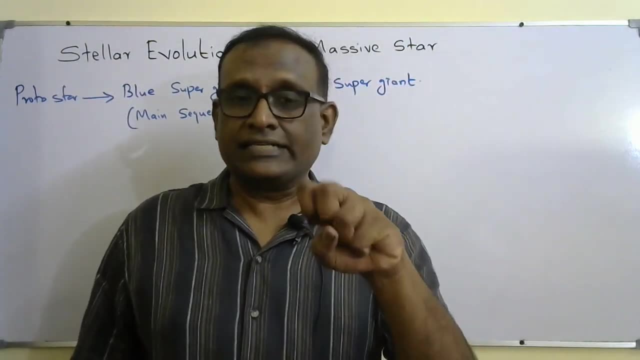 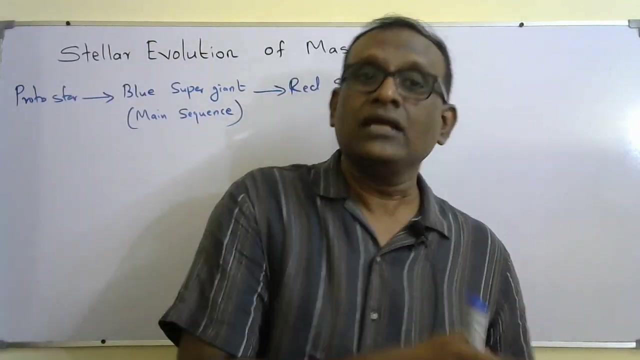 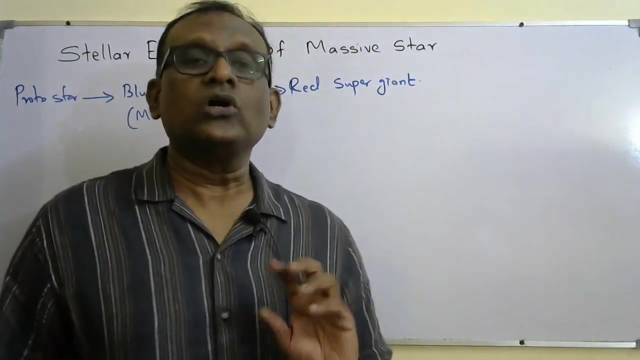 massive star. the star could be or will be in this state of red supergiant state until iron is formed because its inward gravitational pressure is very high and it can withstand to very large outward radiation pressure given by different types of fusion reaction. When ion is formed, what happens, You know, in the radioactivity you would have. 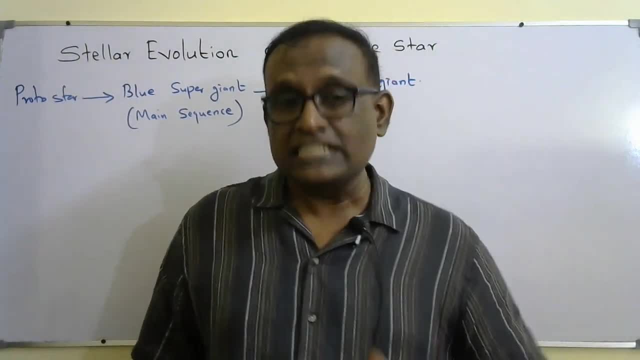 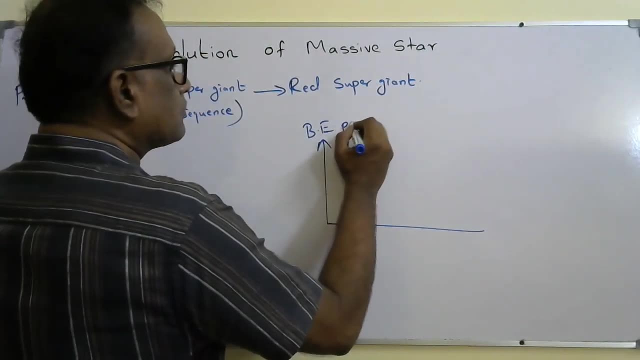 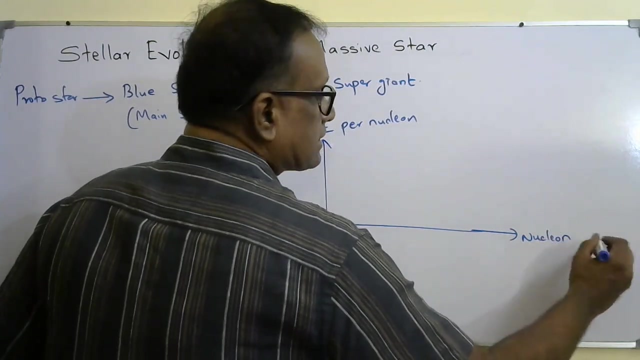 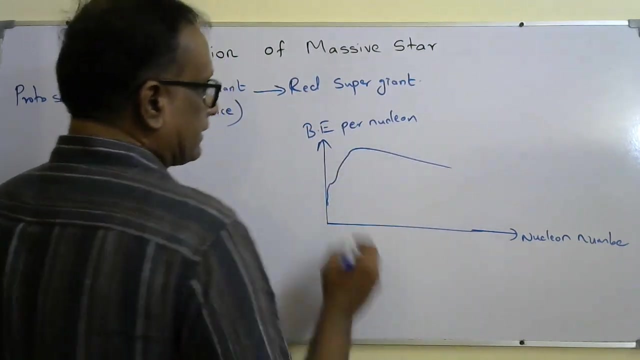 learned. when you think about binding energy per nucleon against mass number- graph- When you think about the binding energy per nucleon against nucleon number or mass number, the graph is something like this and it goes like this: So the highest binding energy per nucleon occurs for: 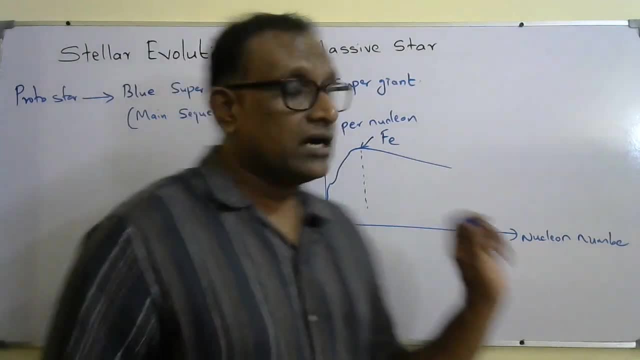 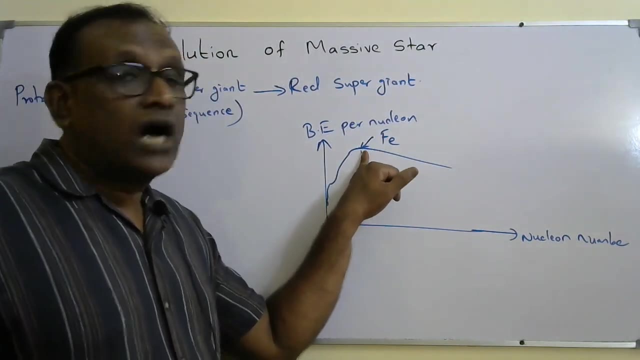 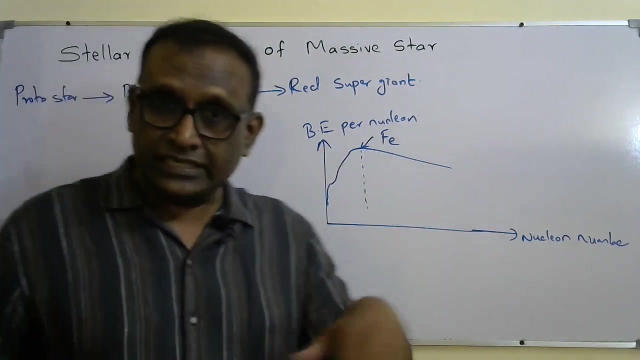 ion. So that means you know the binding energy per nucleon indicates the stability That means when ion is formed you can't fuse ion further because if you are fusing the ion the product will be on the right side. You know, during fusion the nucleon number increases for the product. 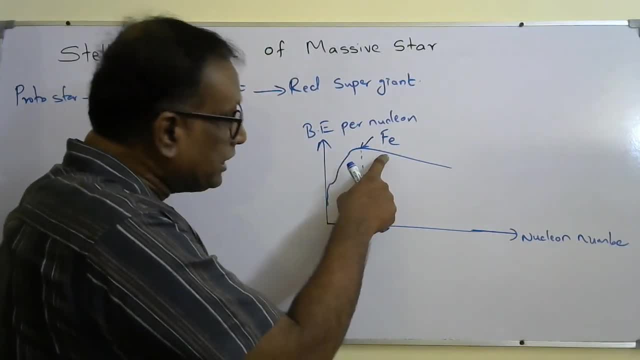 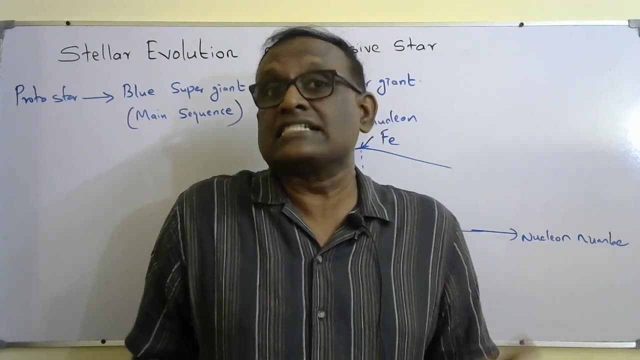 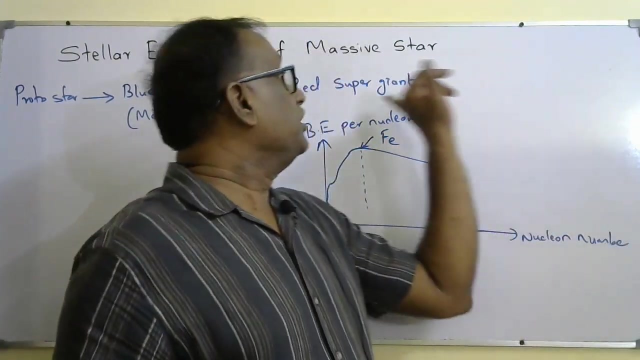 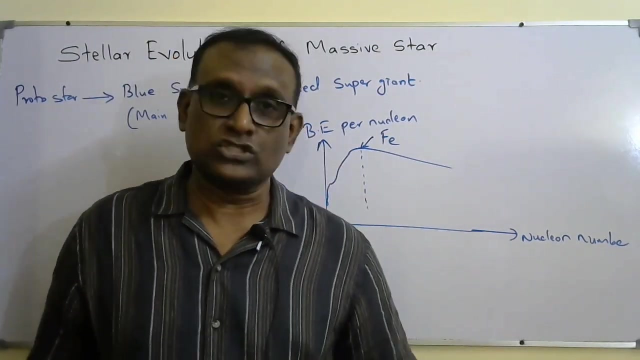 So if the ion is fused the product will have larger nucleon number but it has lower binding energy per nucleon. Lower binding energy per nucleon means its stability is lower. So that means iron cannot be fused inside the core of red supergiant. So when iron is formed inside the core of the red supergiant there, 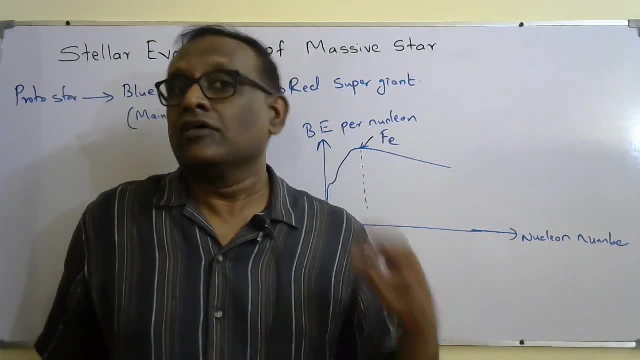 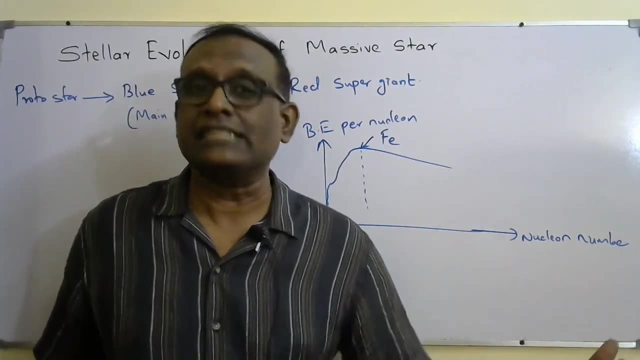 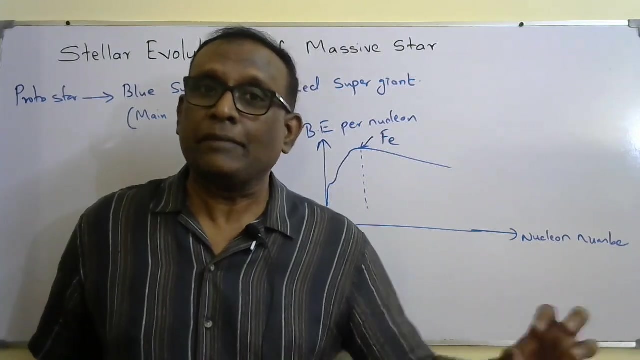 won't be any further fusion reaction because iron cannot be fused there At that particular temperature. it's not possible because outcome is unstable, so energy will not be released. You would have learned that in radioactivity. So if the outcome or the product becomes stable, only energy will be released. So to have a fusion reaction in which the product is unstable means you need to supply energy to have such fusion. So here energy is not released because the product, if you fuse the iron, the product will have low binding energy per nuclear. it's unstable, so the fusion will not happen. 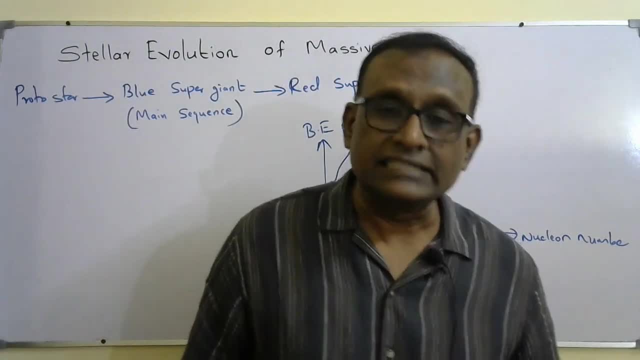 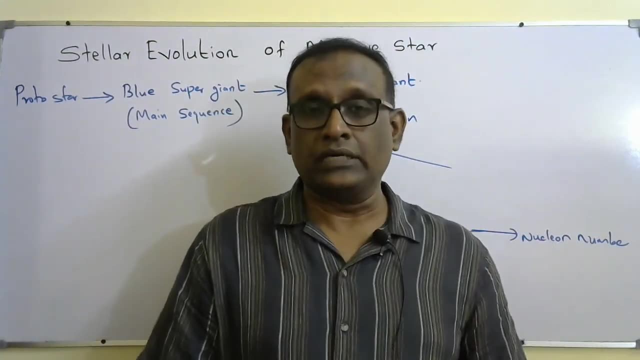 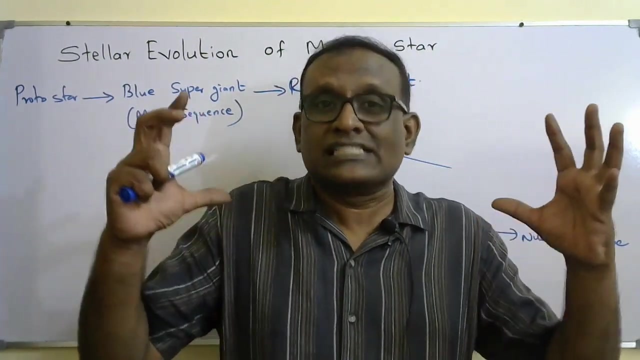 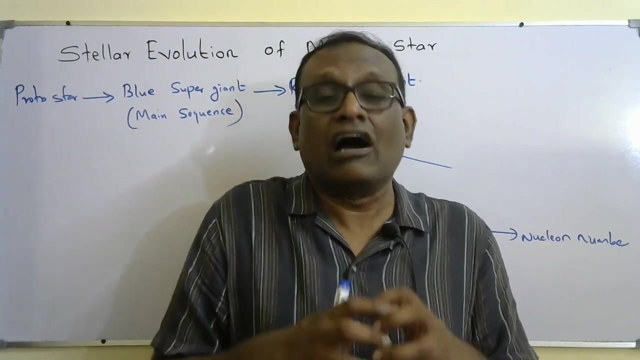 and energy will not be released. so if there's no further energy released, what happens? the outward radiation pressure won't be there or will become significantly lower, but inward gravitational pressure is huge. so due to inward gravitational pressure, the core will shrink heavily. and suddenly, when the core shrinks, pressure increase and there will be explosion. that explosion, 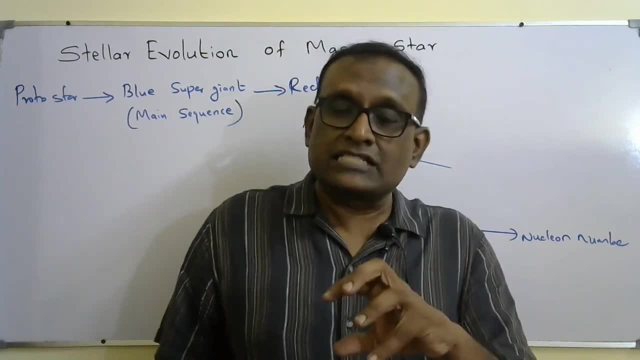 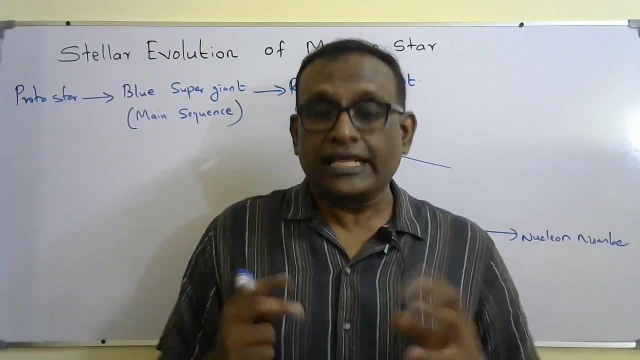 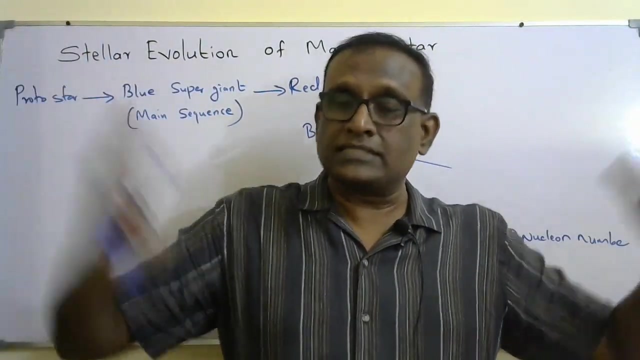 is called time to supernova. so here the explosion happens due to sudden shrink of compression in the core. that causes the explosion, but in plantar nebula formed when the output radiation pressure throw away in low masa, throw away the outer layer. here no further fusion, no outward radiation, so on and so forth. my friends, that's it for the Atheist theory. 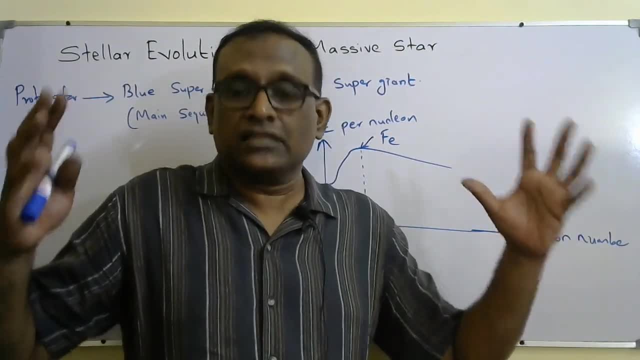 It will be a very helpful video. if you like my video and would like to see it in this video, then request a donation to my patreon. radiational pressure. so the star, the core, will shrink due to inward gravitational pressure and when it shrinks the pressure becomes very high. 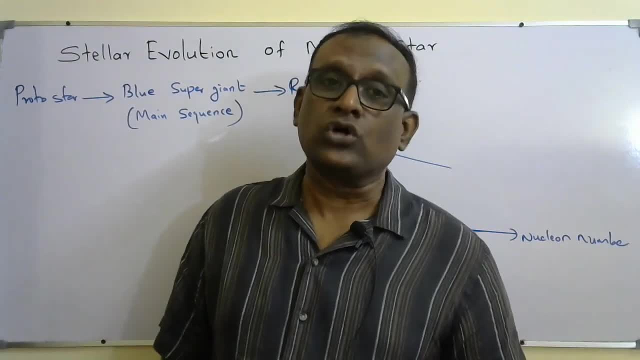 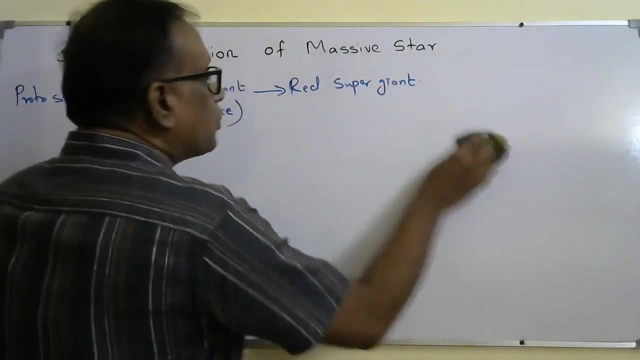 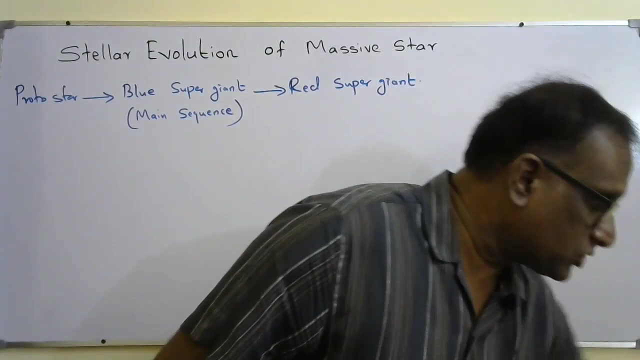 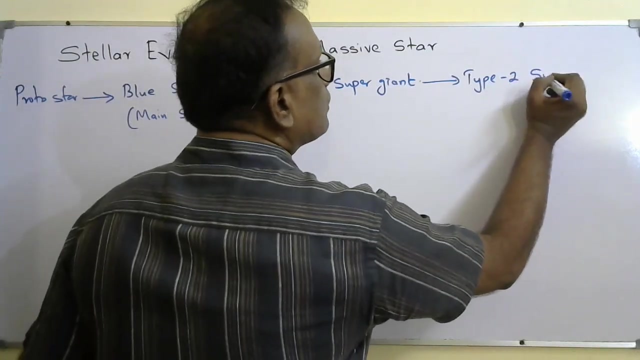 and the core will explode and that is called type 2 supernova. so after the explosion the most of the mass will be thrown out. so the core retinant will become, or could become, two different stages after the explosion. so the next stage I can say is red supergiant will become type 2 supernova during type 2. 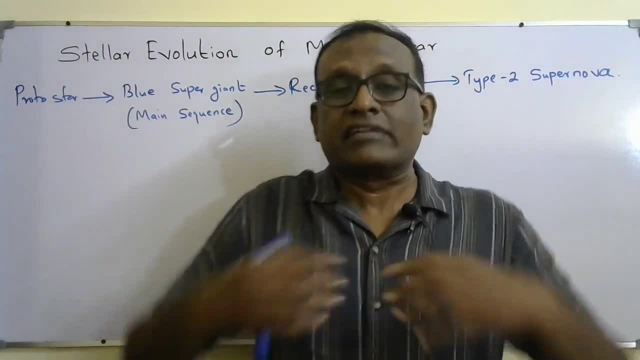 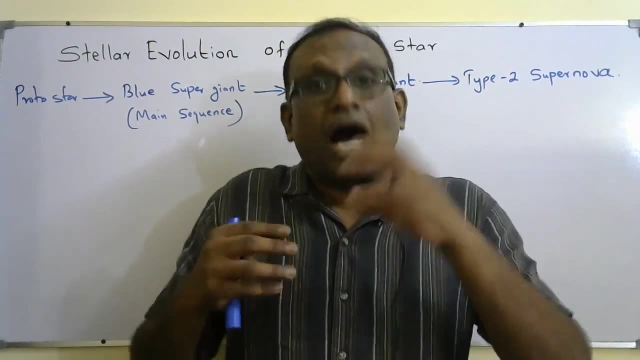 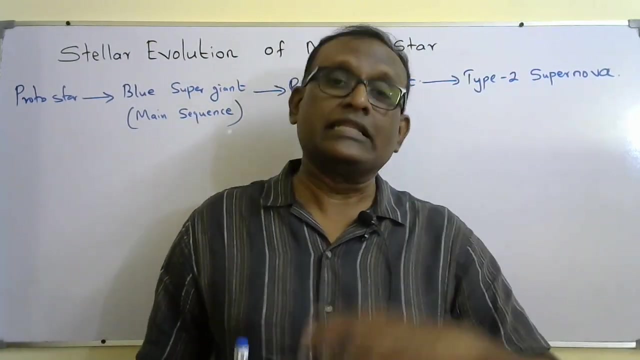 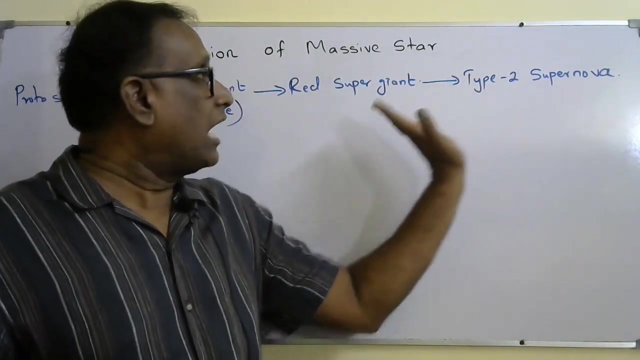 supernova. yes, iron can be fused because the energy released during that explosion is very high. that energy can fuse even iron, not only iron, beyond iron also the fusion will happen. they are saying that's the way other elements in the periodic table are being fused, created during supernova. okay, so this type 2 supernova will be there after the? super red supergiant, there will be explosion called type 2 supernova. then, after the supernova, the core mothers could become three or two different types. if the mass of the core goat is lower than three times of the solar mass, it will become new trans star. further. mass of the core remnant of the type 2 supernova is less than 3 times of the solar mass, it will become Newton star. It consists of full of neutrons. If the mass of the core remnant after the type 2 supernova is more than 3 times of the 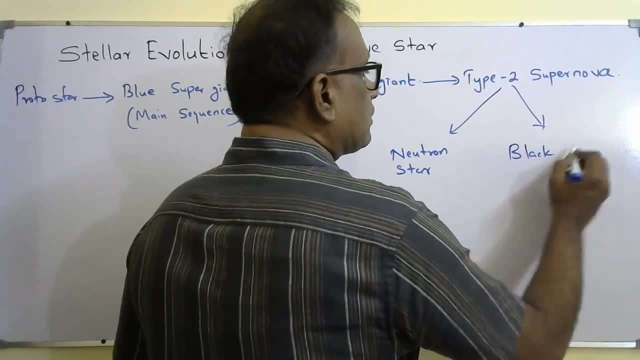 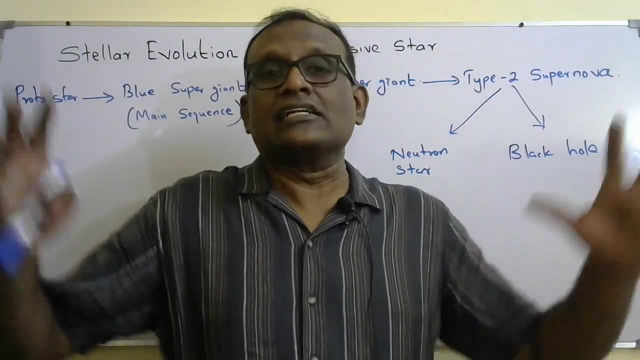 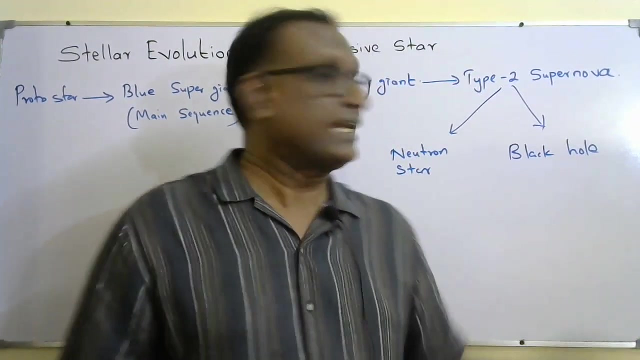 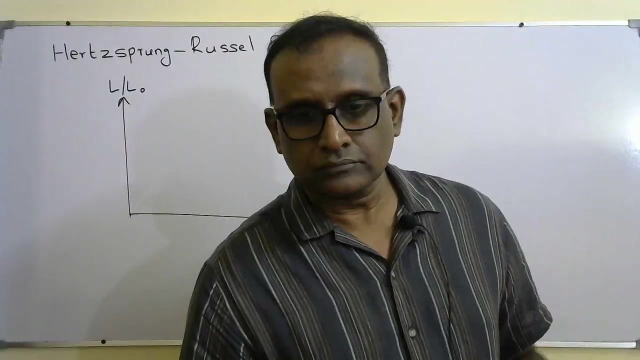 solar mass, it will become black hole. So black hole means it has huge amount of inward gravitational pressure. it will shrink a lot and the density will become very high. it can act at even light. That is the black hole stage. Okay, so next topic is Hertzsprung-Russell diagram or HR diagram. 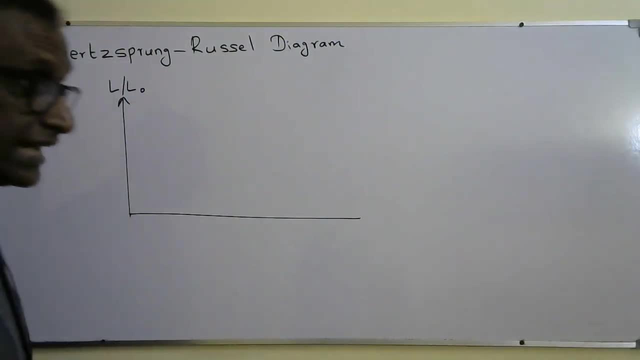 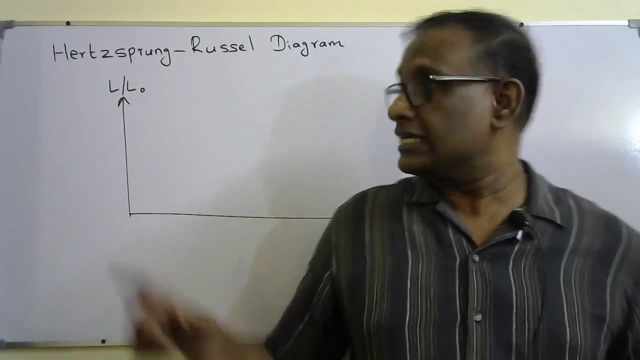 So it's actually a plot. Y-axis indicates relationship between black hole and black hole. Y-axis indicates relative luminosity. Relative luminosity means luminosity of a star or star cluster relative to luminosity of the sun. So L over L0, L0 is the luminosity of the sun. 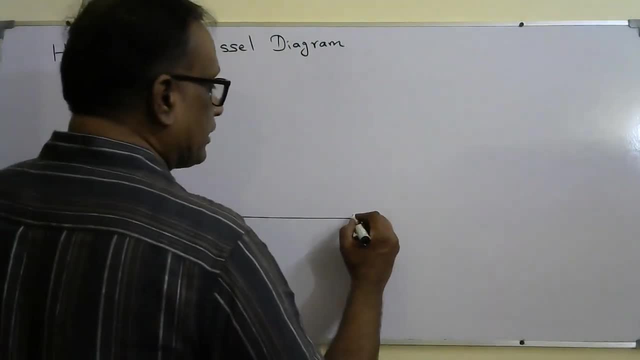 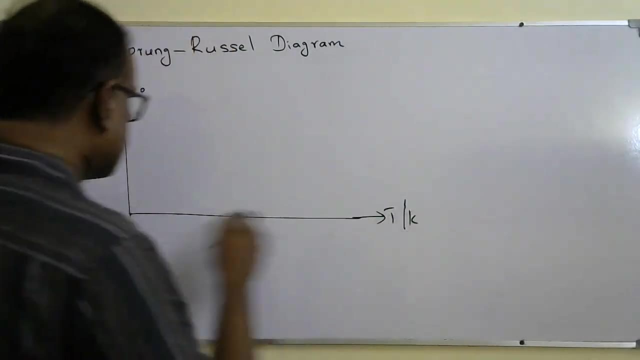 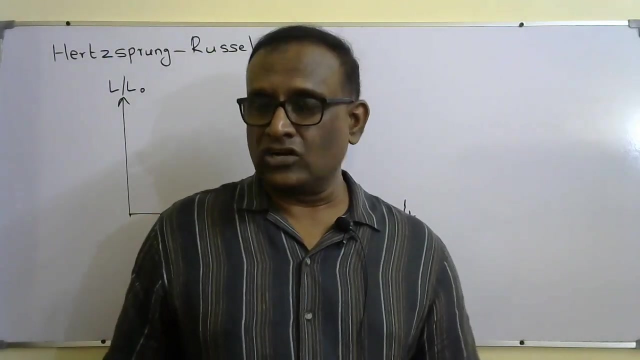 X-axis is the temperature in Kelvin. So here the temperature, the X-axis is marked in a different way. Normally in graphs we start from lower to higher, but here it's marked with higher to lower. It normally starts with 40,000 or 60,000.. 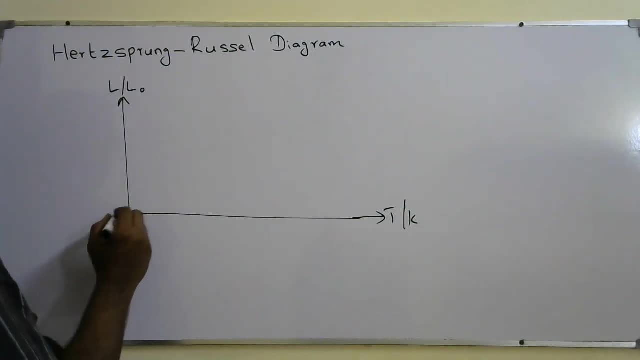 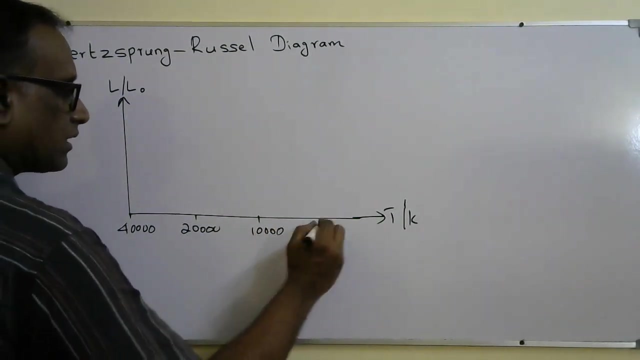 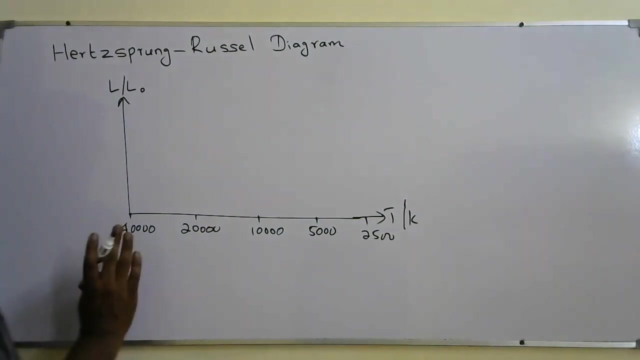 With equal ratio. it's marked, not equal intervals, equal ratio, so careful. so it's 40,000 Kelvin, Then 20,000, difference is 20,000, here 10,000, then 5,000 and 2,500, or you can start with. 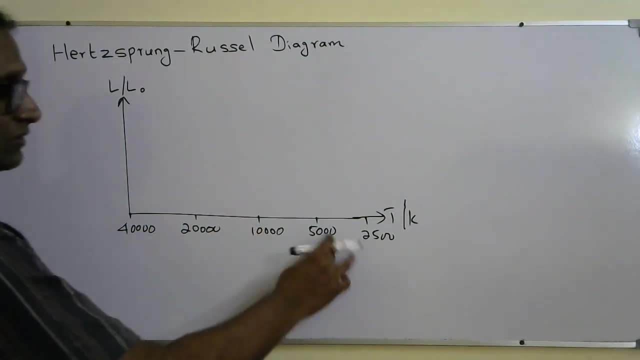 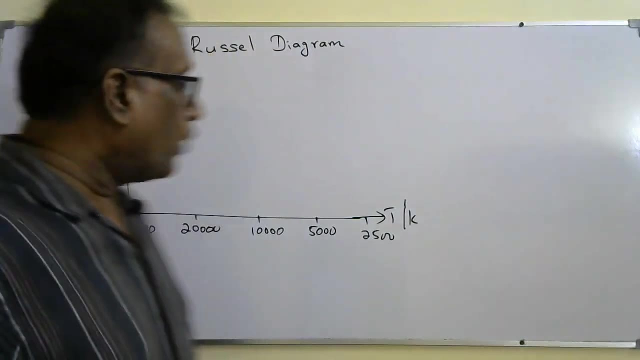 60,000, 30,000, 15,000, 7,000, find like that You can. This is the ratio And with the same ratio, mostly the ratio is taken as half. Y-axis is the relative luminosity. 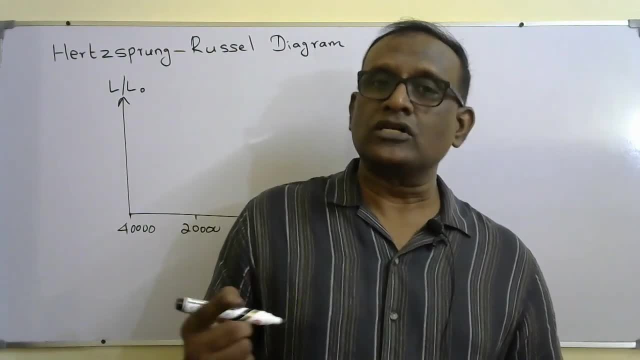 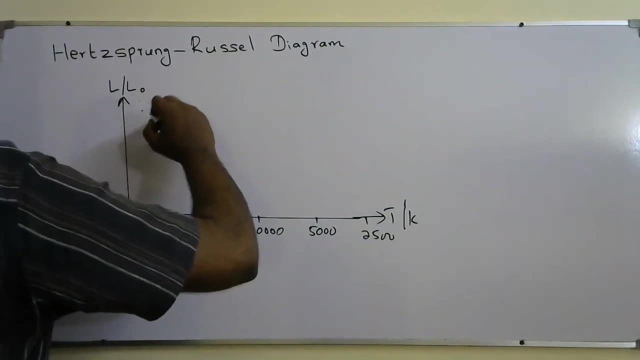 So relative luminosity of the sun is 1,. luminosity of the sun divided by luminosity of the sun is 1.. Okay, the main sequence I already explained. that is marked along the diagonal and this way, from left, top to bottom, right. 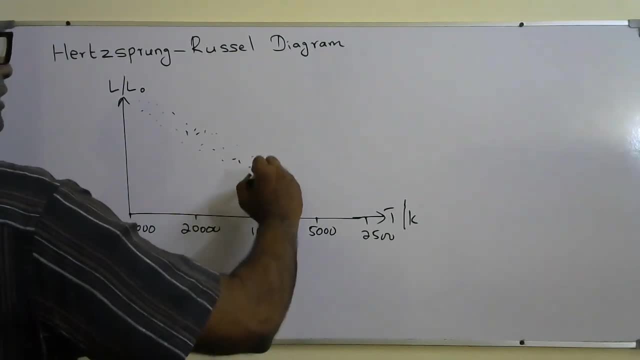 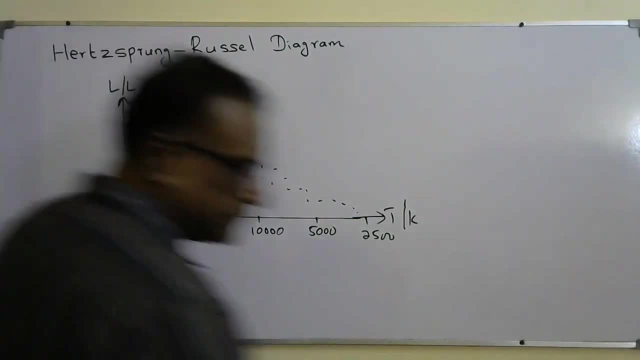 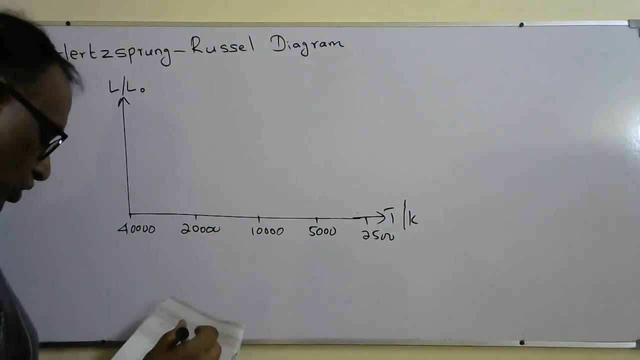 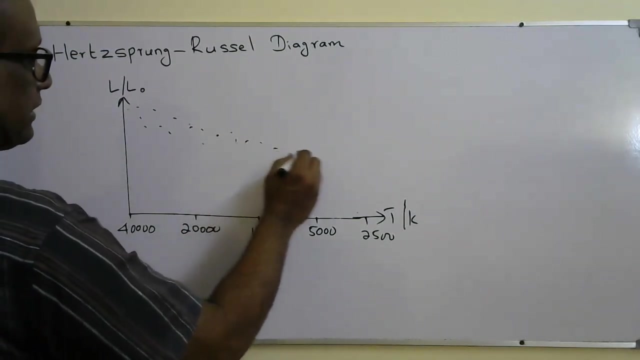 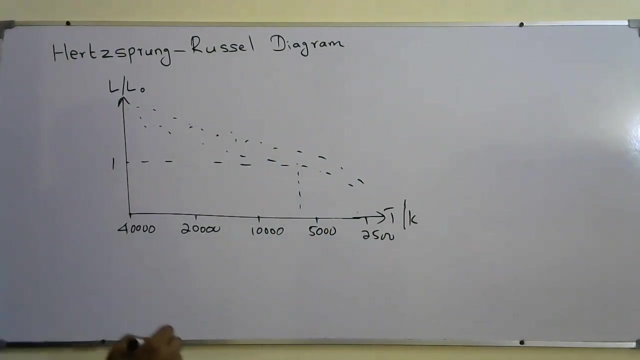 They won't ask to draw. they never ask like that. But you should be able to mark the positions of different things like: so sun is somewhere here, so this could be 1.. Sun temperature is almost 5,600, 5,800 Kelvin. 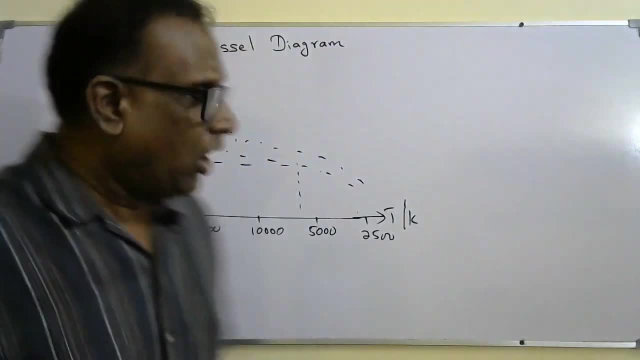 So sun is somewhere here, so this could be 1.. Sun temperature is almost 5,600, 5,800 Kelvin. So sun is somewhere here, so this could be 1. Sun temperature is almost 5,600, 5,800 Kelvin. 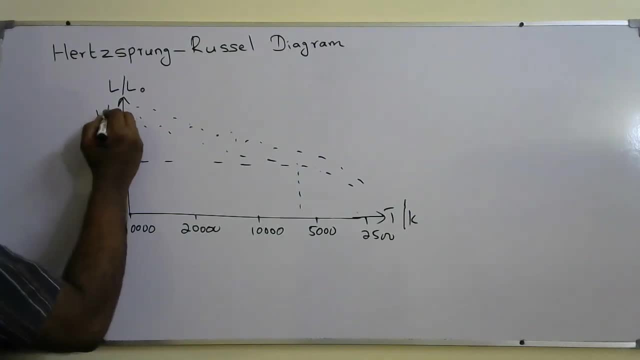 Okay, so this is 1, this is 10 to the power 2, 10 to the power 4, so here 10 to the power minus 2,, 10 to the power minus 4. here also that those are given with the ratio, right. 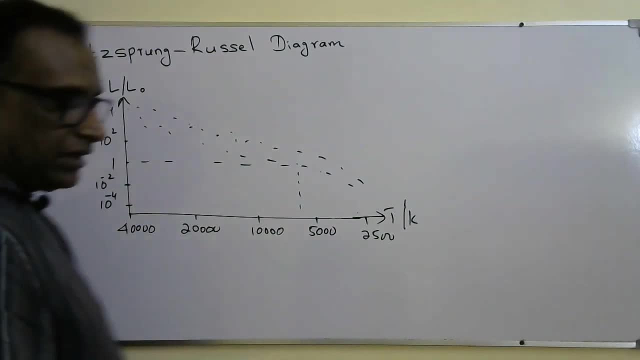 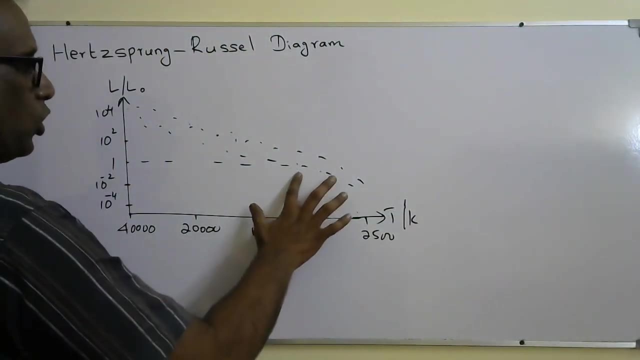 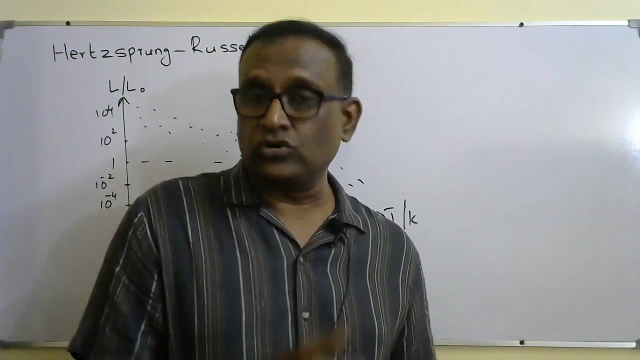 So you can see where to mark the main sequence. I already marked it. So where to mark the white dwarfs? I told white dwarfs temperature will be low, higher when it was in the main sequence. So if you think about our sun, when the sun becomes white dwarf, the temperature will be. 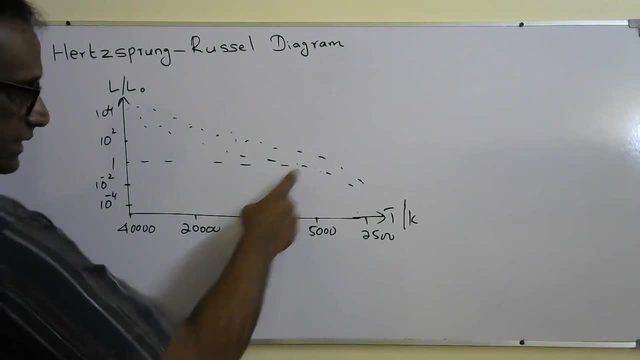 more. The temperature of the sun is somewhere here- 5,600, so it will be more when it becomes white dwarf. We can mark the white dwarfs up to around 18, 20,000, so these are the white dwarfs. 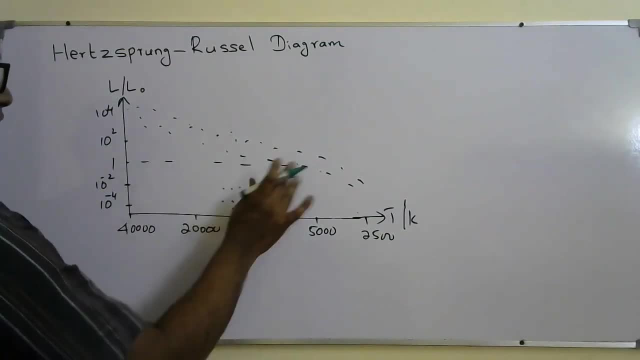 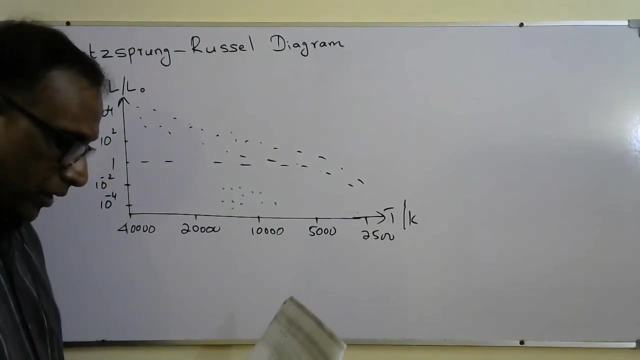 Yeah, luminosity is lower, much lower compared to luminosity of sun. So the luminosity will be 10 to the power minus 2 or 10 to the power minus 4, order: 10 to the power minus 4.. 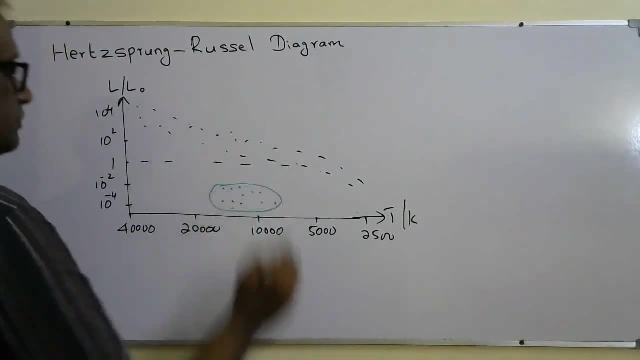 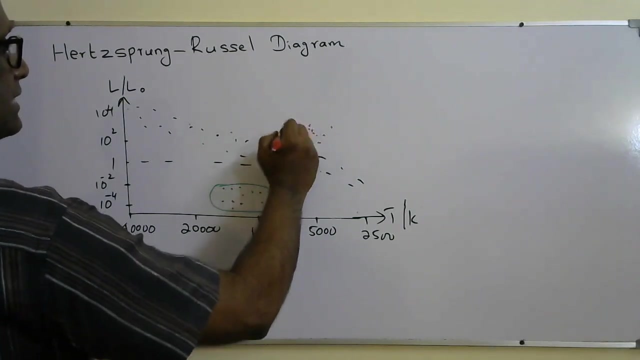 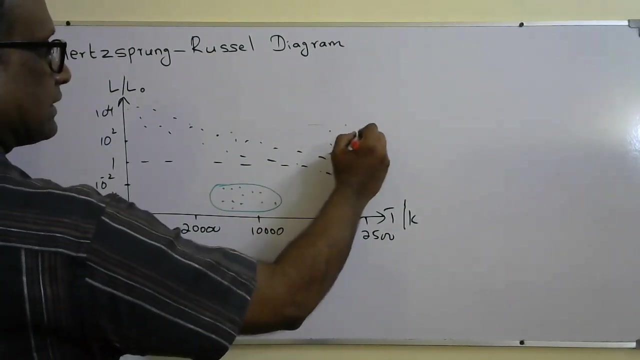 These are the white dwarfs this stage. Okay, red giant we have to mark. red giants have higher luminosity but lower temperature, so they will be towards right somewhere here. red giants will be in this position So little more further towards right, more than 5,000, so somewhere here. 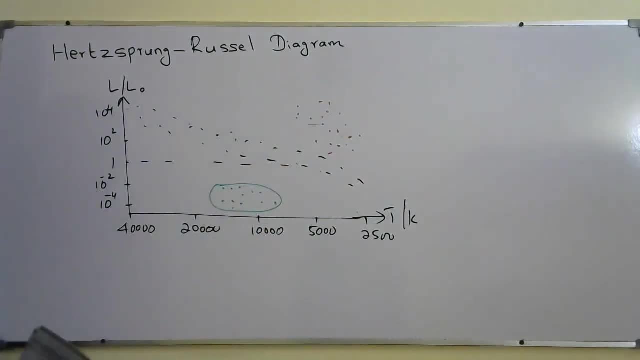 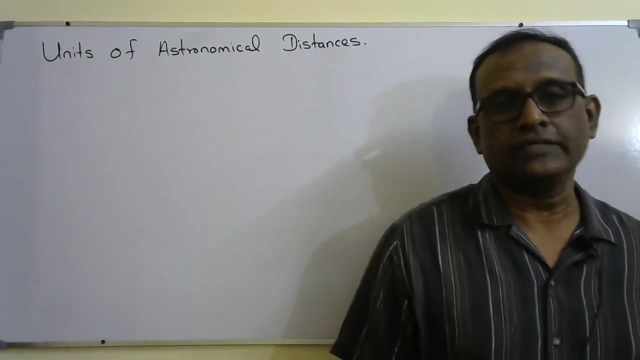 Super red giants could be somewhere here. So these are the red giants. So this is the white dwarf, red giants, main sequence. You should be able to mark them on a chart diagram that you should know that. Okay. so next thing about measurement of distance of a star or galaxy. that's very important. 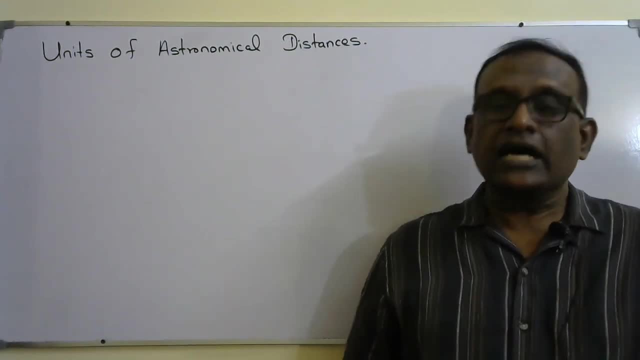 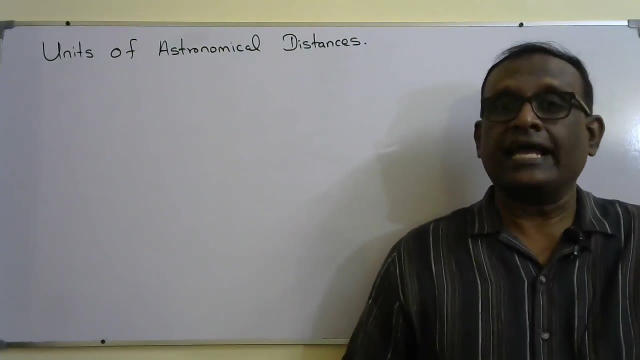 here it is levels, So different units are used when we talk about distance, of distances of different galaxies and stars from us. us means from earth, We don't give it in kilometers. So there are three different units we introduce in your syllabus. 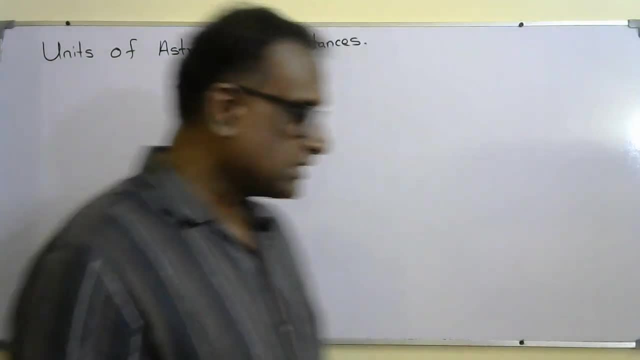 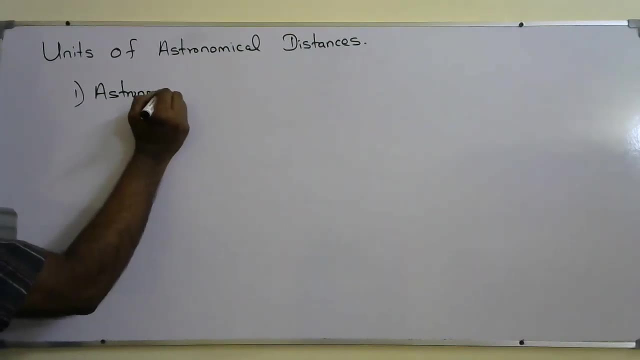 First one is called astronomical unit. The first unit is called astronomical unit, So it's denoted by Au, So kilometer denoted by Kf, like that it's denoted by capital, A capital, U, So what it means. 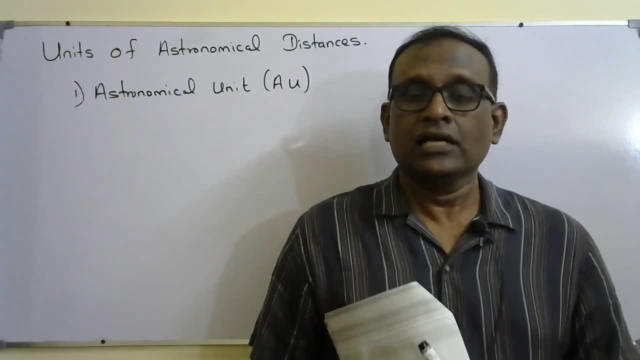 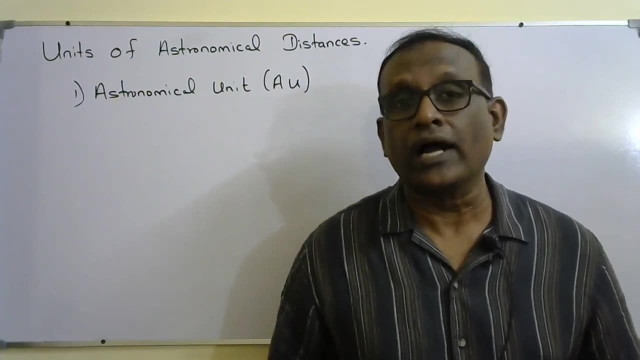 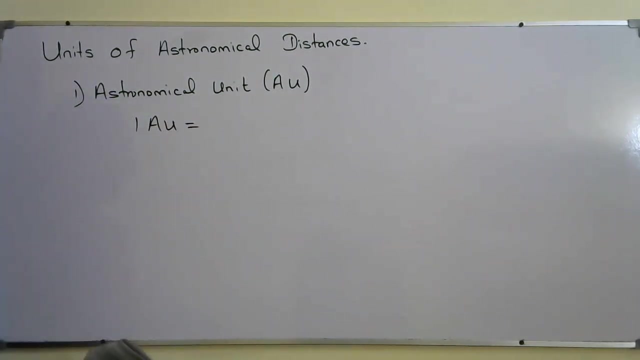 Astronomical unit. How do we define astronomical unit? So it's defined as the average distance of the earth from the sun is defined as one astronomical unit, So one astronomical unit has a value in kilometers, that's average distance of the earth around. 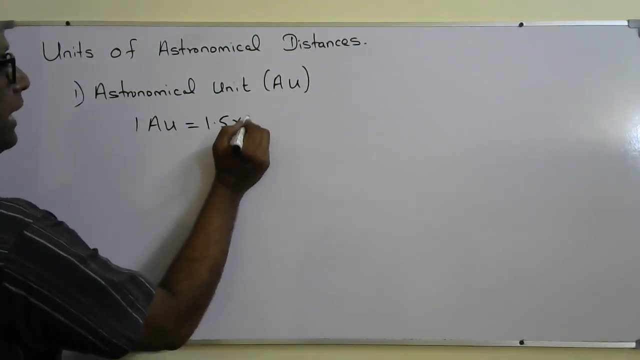 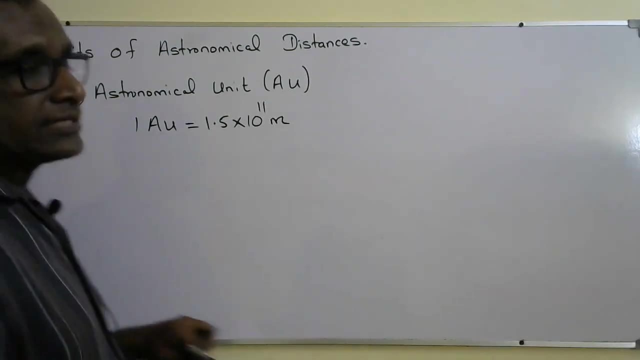 the sun, that is 1.5 into 10 to the power, 11 meters. that is called one astronomical unit. So we can find two astronomical units: 1.5 astronomical unit, anything you can find. If you want you can convert to meter. 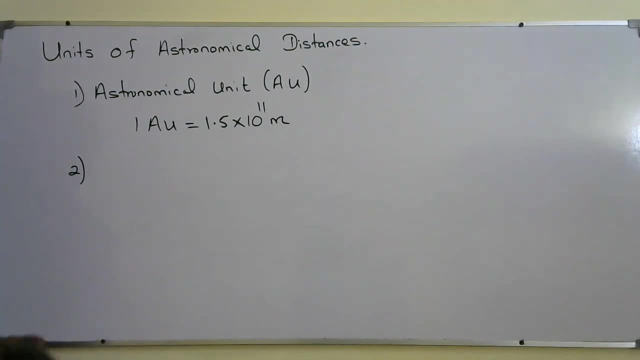 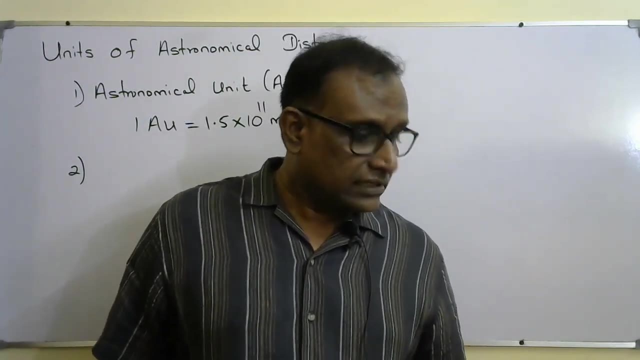 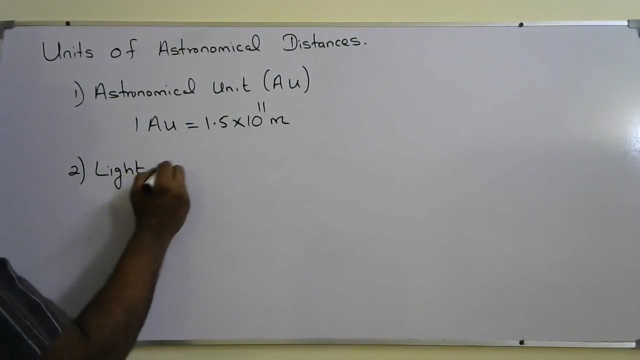 Okay, the second unit we use in your syllabus to measure the astronomical distances. astronomical distances means whatever the distance measured in astronomy, right? So second unit we use is light years. So what is light year denoted by Ly? So what is light year denoted by Ly? 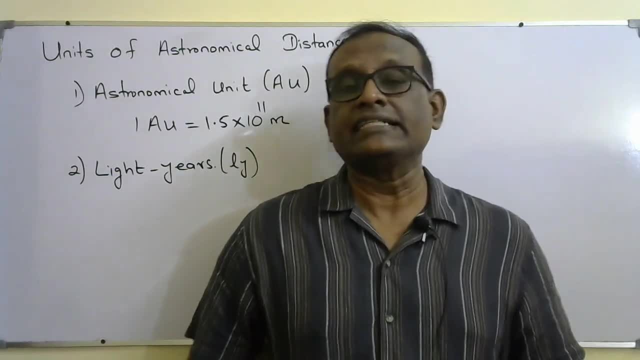 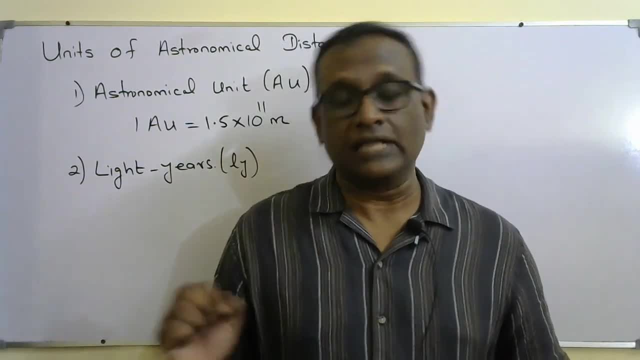 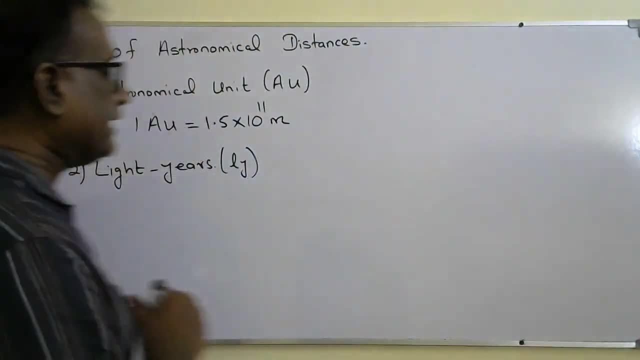 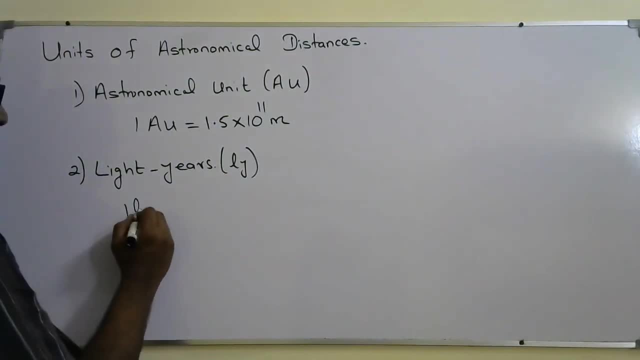 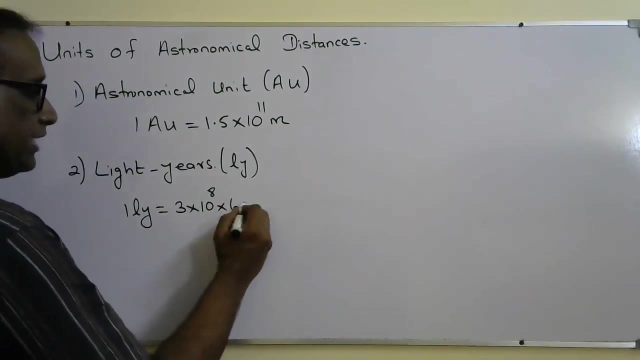 So what is light year denoted by Ly? one light year means the distance the light travels during one year. So during one second it will travel 3 into 10 to the power 8. During one minute into 60.. During one hour During. 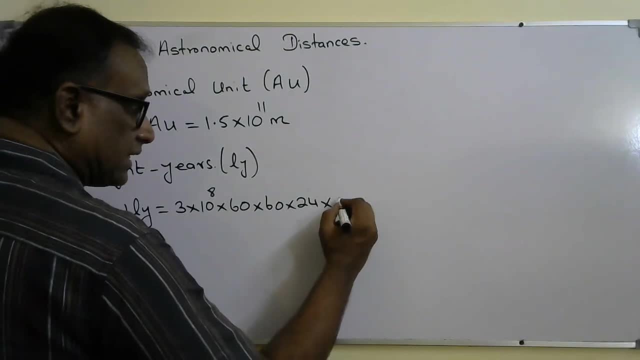 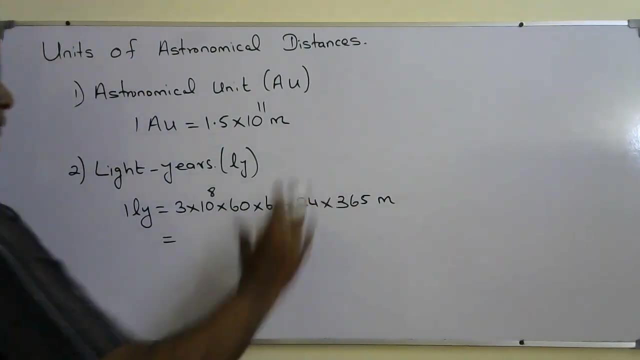 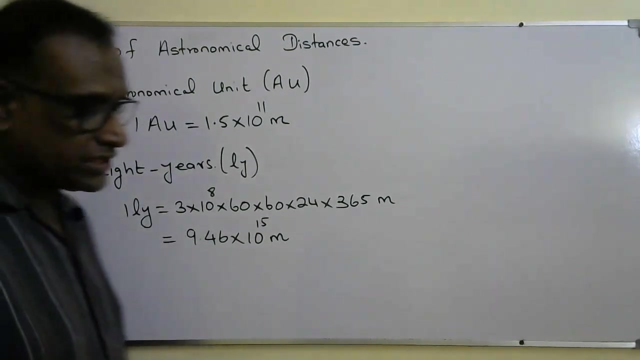 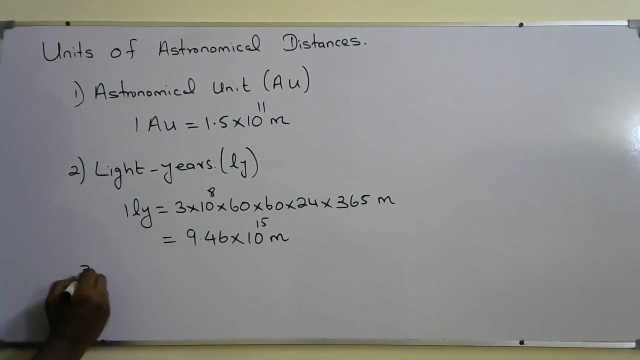 one day, During one year, 365 meters, So solid, you will get the amount, the magnitude of one light year. So that will be equal to 9.46, 10 to the power, 15 meters. Okay, so the third unit, what we use in your syllabus, is called parallax. second, The third unit in your syllabus: 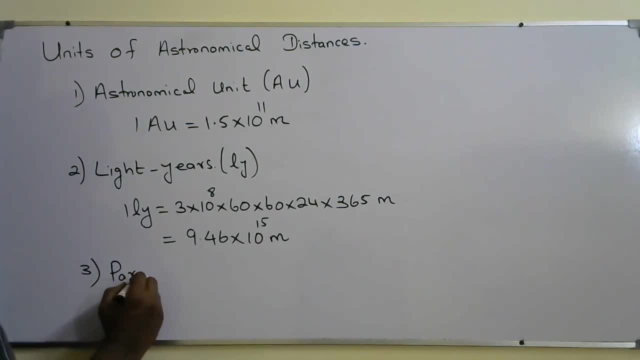 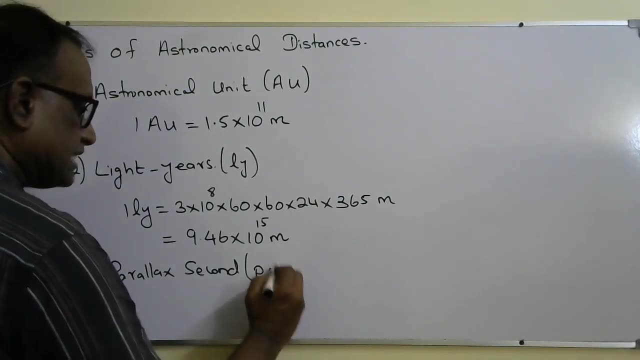 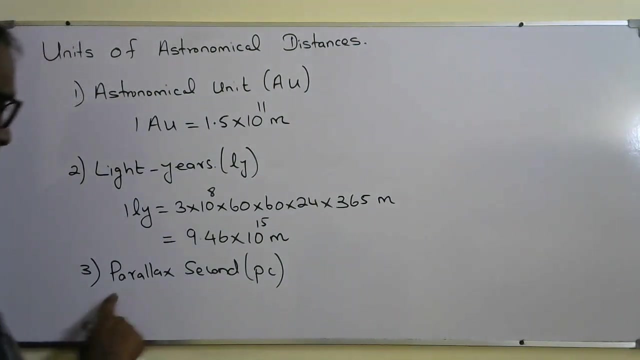 is called parallax second, Denoted by PC, Symbol P, Symbol C, Shortly it's called parsec. Parallax second, Shortly it's called parsec. The notation for parallax second is PC, Light year, LY, Astronomical. 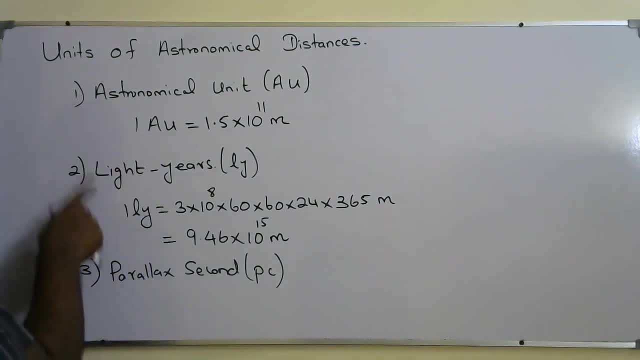 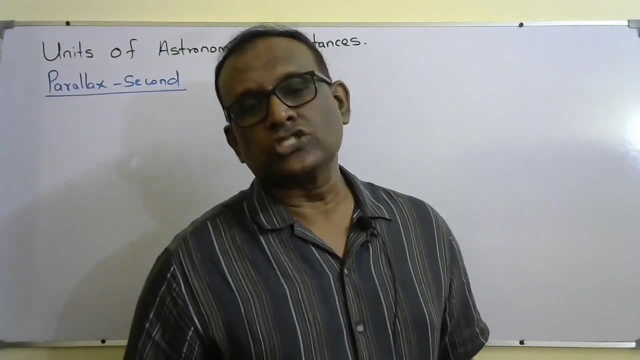 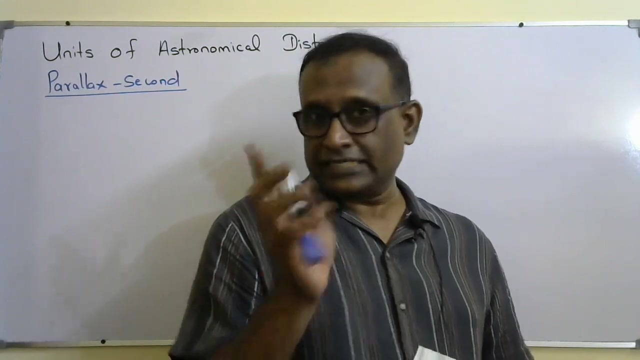 unit, AU. I defined the meaning of astronomical unit and light year. So how do we define parallax second? Okay, I'll define it now. Okay, so before defining parallax second, you should know that one degree in protector- but it's not much, but one degree. 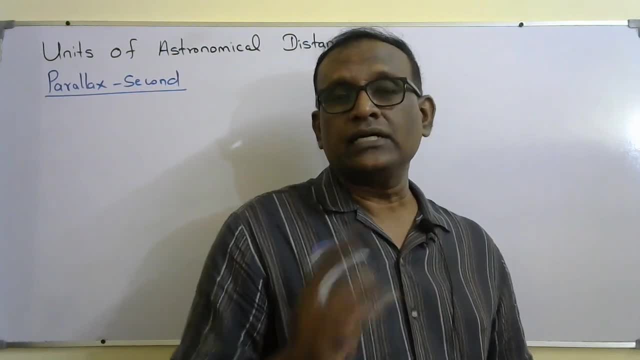 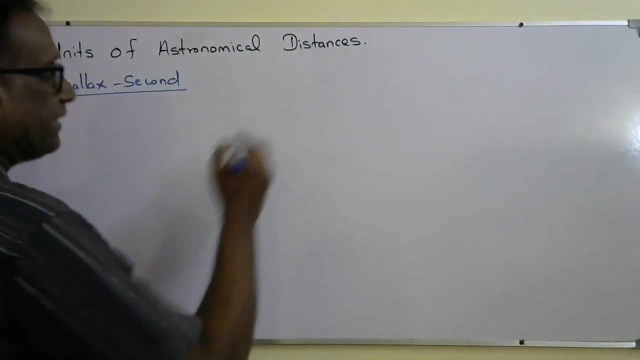 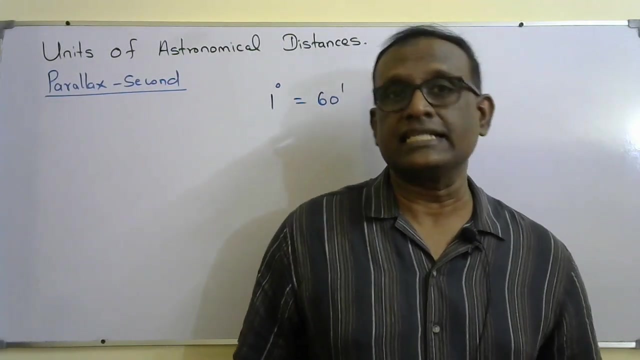 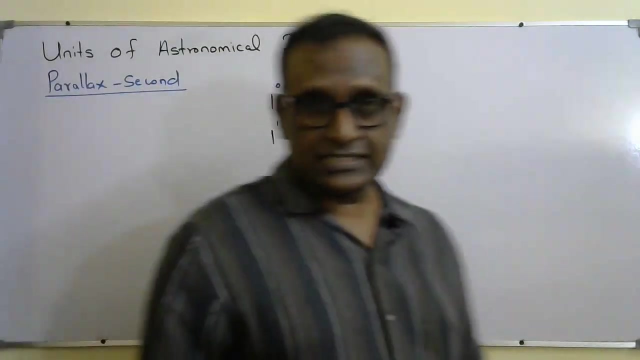 could be divided into equal 60 divisions and each division is called one minute. So that means one degree is equal to 60 minutes. One minute means 1 over 60 degree. Same way, one minute is divided into equal 60 divisions and each division is called second, So that 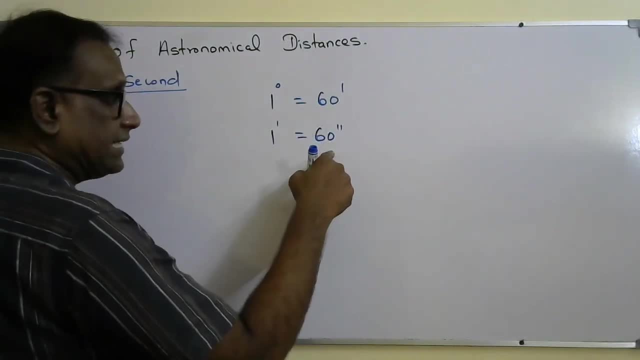 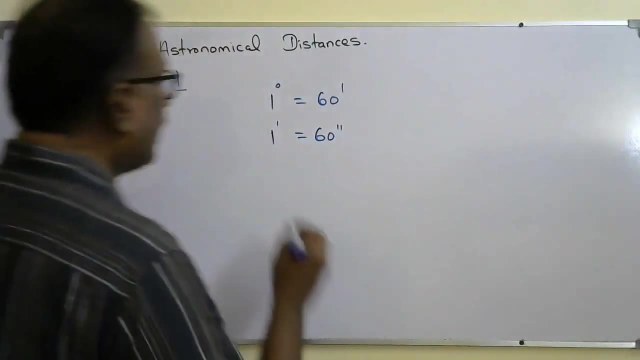 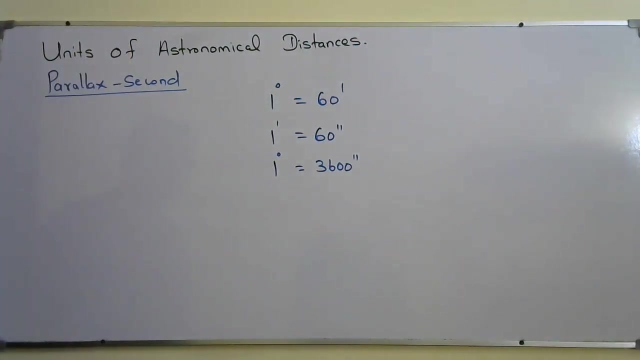 is 60 second. So that means one second is equal to 1. over 60 minutes. That means one degree is equal to 3600 second. One degree is equal to 3600 second. This is the notation for second. This is the notation for second. So that means one degree is equal to 3600. 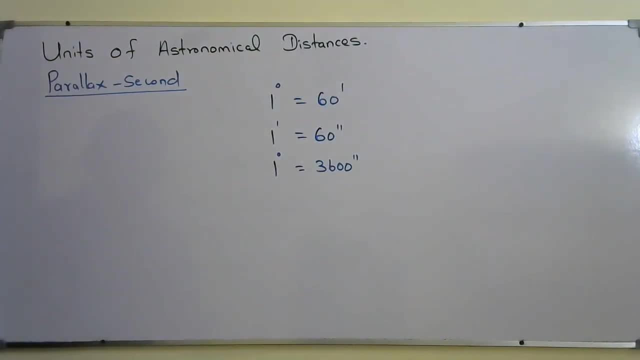 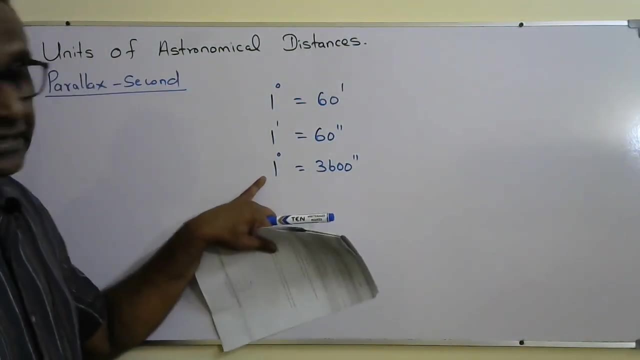 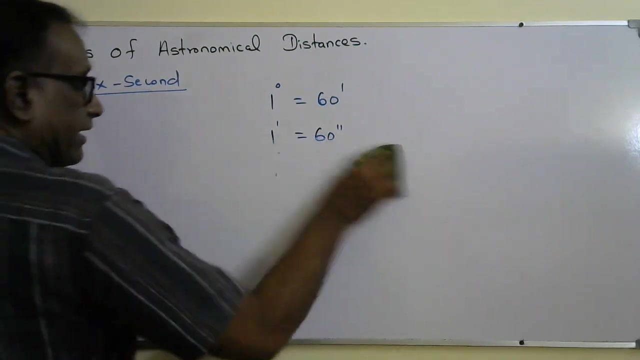 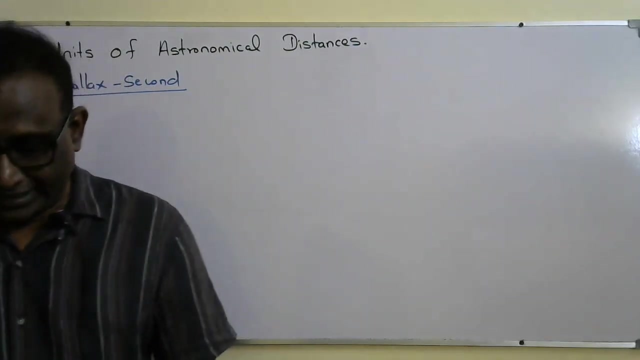 second. This is the notation for minute. Okay, so you must know this Right. So how do we define? So? one second means 1 over 3600 degree. One second means 1 over 3600 degree. Okay, so how do we define one parallax second? Okay, so we define parallax second like this: We: 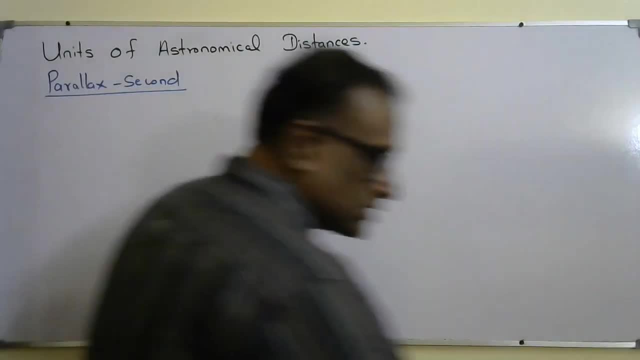 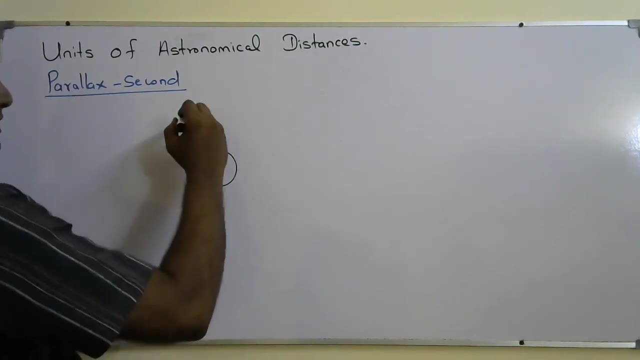 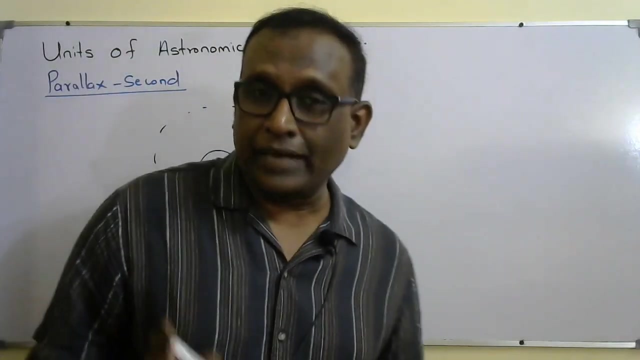 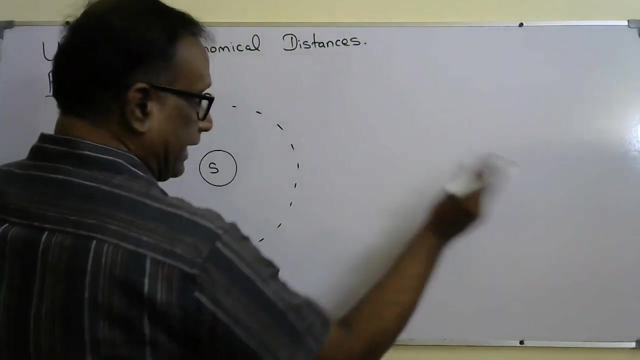 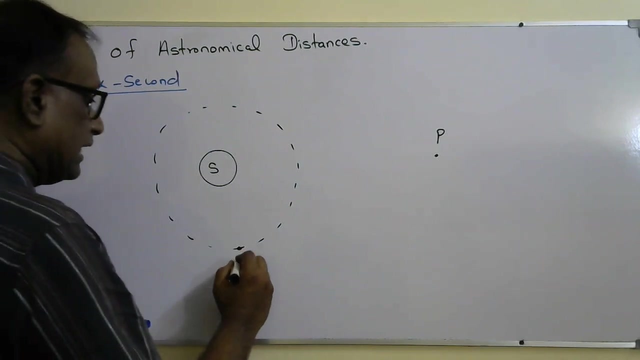 know that earth is orbiting the Sun, so this is the Sun, earth is orbiting the Sun. so how do you define one PC or one parallax? second means now, if, if we could find a point in space, if it would find a point P in space, such that the ether, this is the. 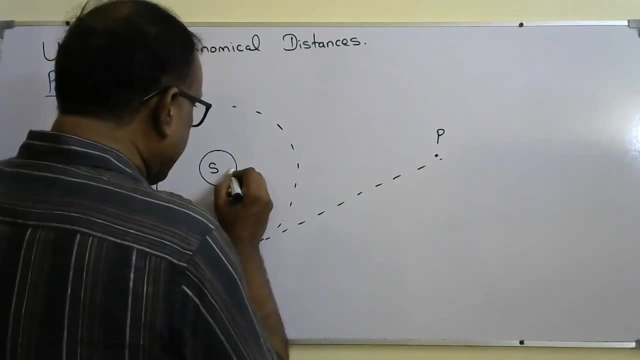 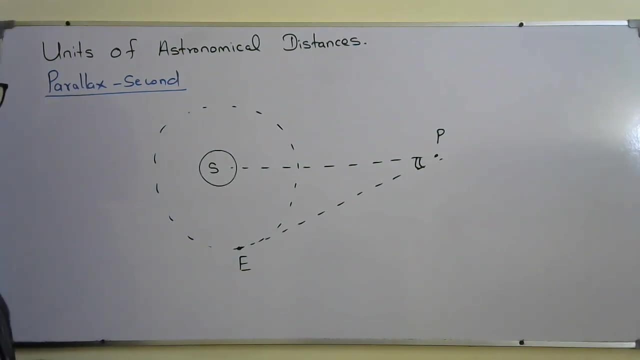 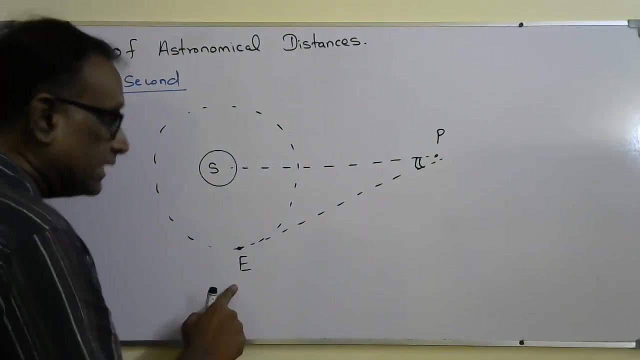 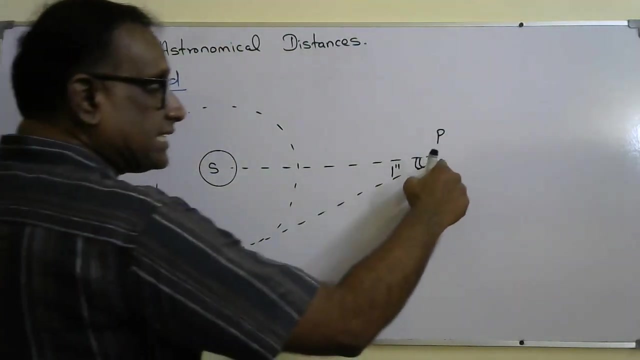 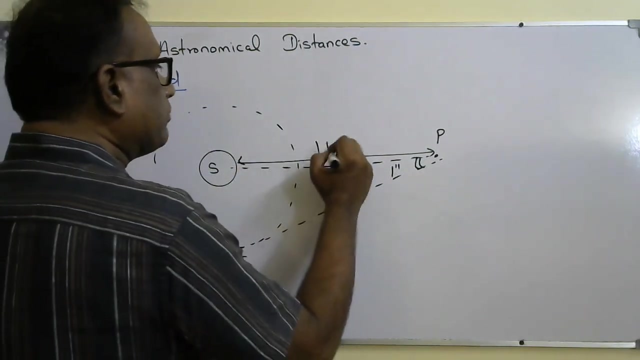 earth, the point P sun. this angle we should be able to imagine that you can find the point light. that but we imagine like is there could be a point P in space, such that the angular earth point P- Sun becomes David one second. if that happens, distance of that point p from the sun is called one pc. i hope you. 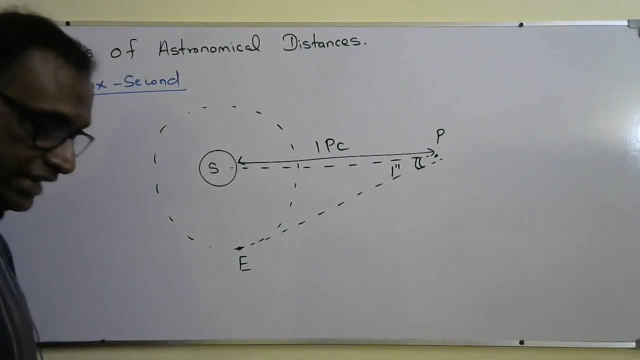 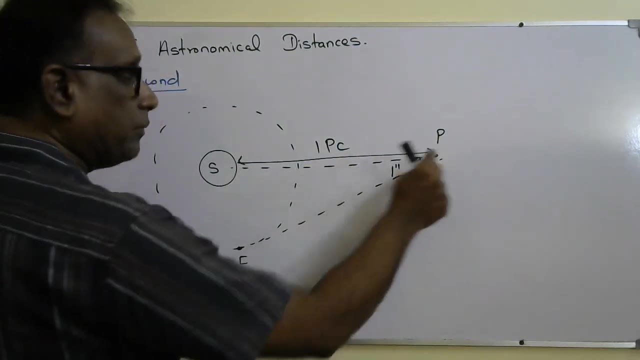 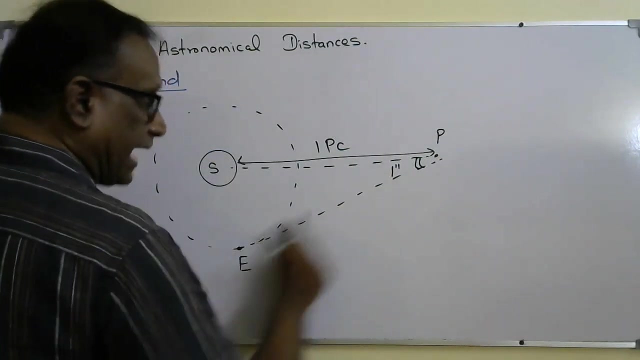 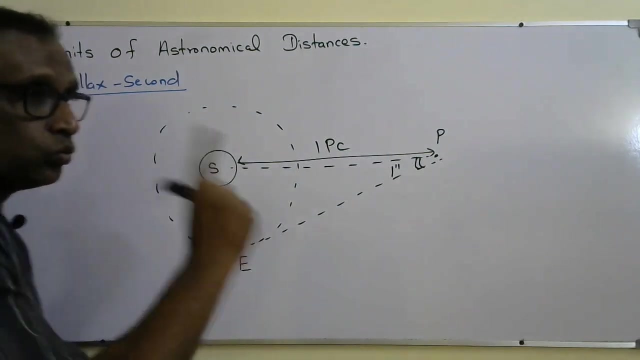 understood. how do we define in space? we imagine a point p such that the distance, sorry the angle, earth, point p- sun becomes one second. if we find a point p such that the angle become one second, then the distance of the point p from the sun is defined as one parallax second. 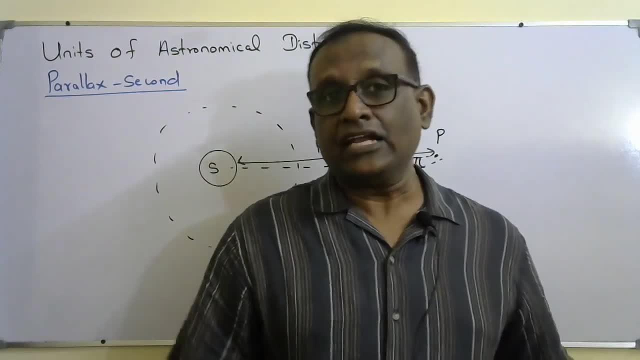 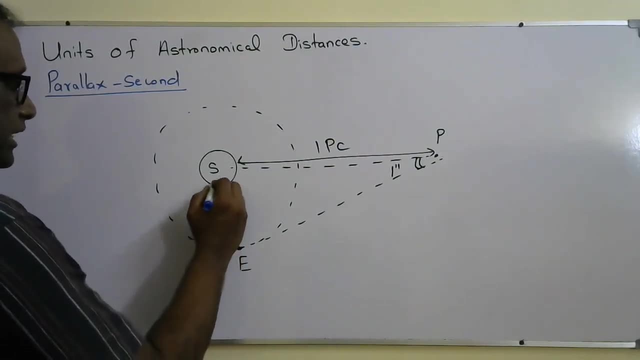 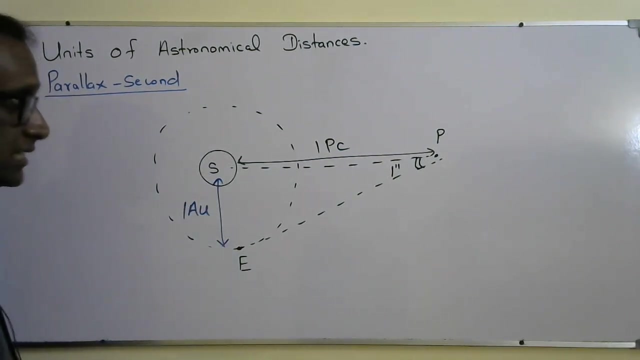 so by using this definition we can get a numerical value for one parallax second. so we know that average distance of the earth from the sun is one astronomical unit, one au. i already define it, and we know how much is one au in terms of meters. so here you can say tan. 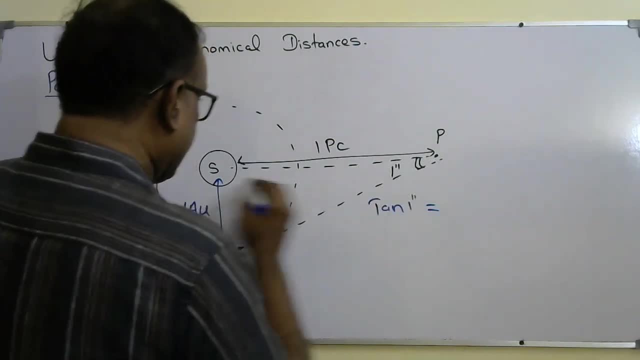 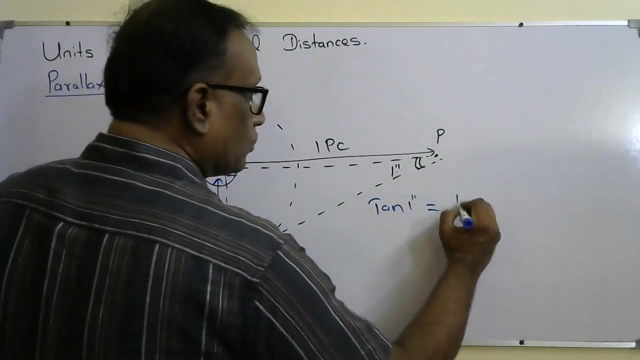 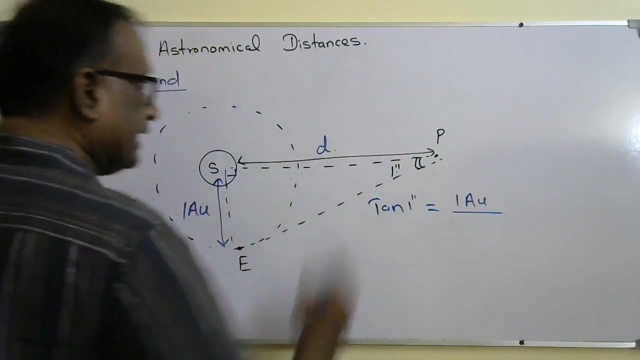 one second in this right angle triangle. in this right angle triangle, what tan one second is equal to opposite, that is, one au over this distance. so this distance is going to be one pc. i'll call it as d over d, so d is going to be one. 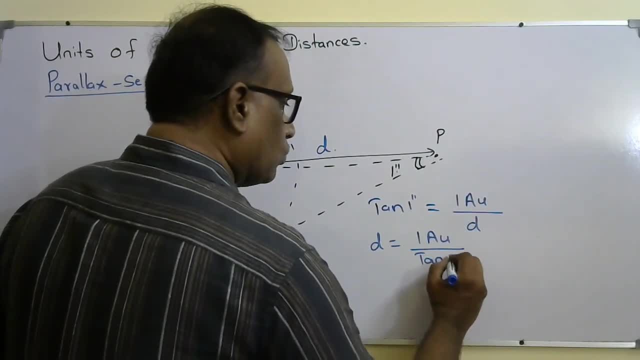 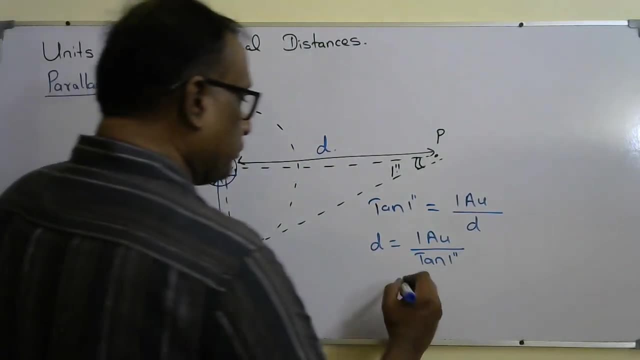 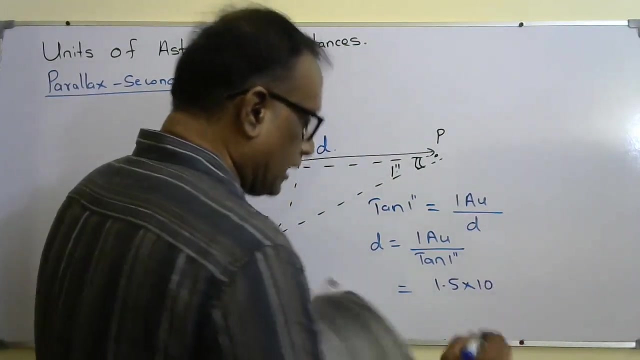 Au over tan 1 second. So you know that 1 second is equal to 1 over 3600 degree and we know 1 Au in meters. that is 1.5, 10 to the power, 11 meter divided by tan 1 second means tan. 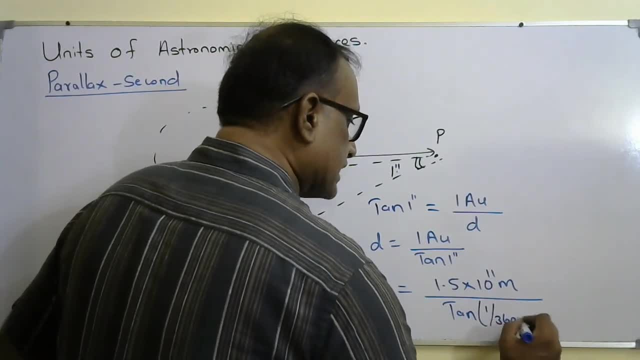 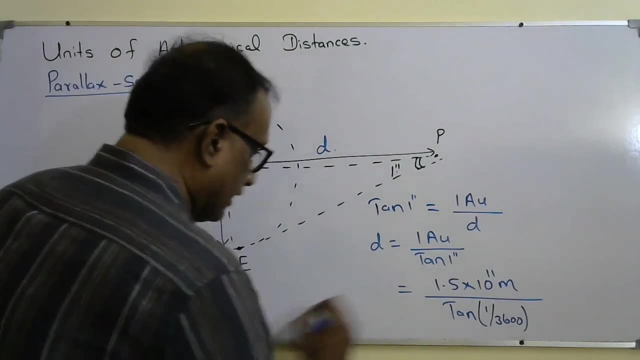 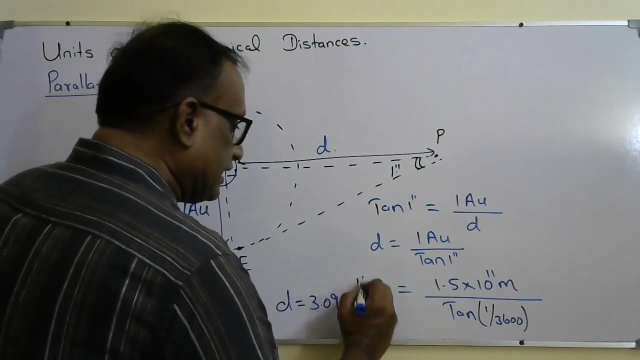 1 over 3600 degree. Solve it. When you solve you will get 3.09. so here you will get. I write it here: d is equal to 3.09 into 10. to the power: 16 meter. that is the distance. d that makes this angle. 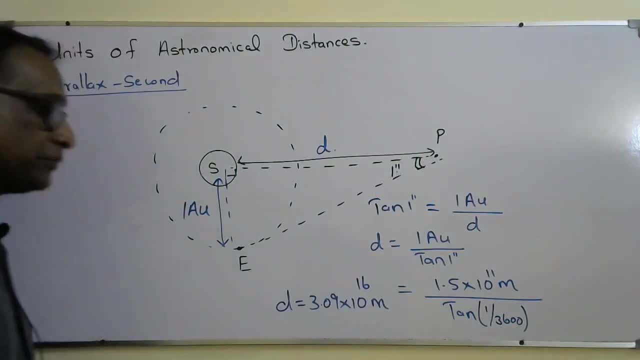 1 second, which is 3.09, 10 to the power. 16 meter, This distance, this distance is equal to 3.09.. So you know that this is a distance: d is equal to 3.09, 10 to the power. 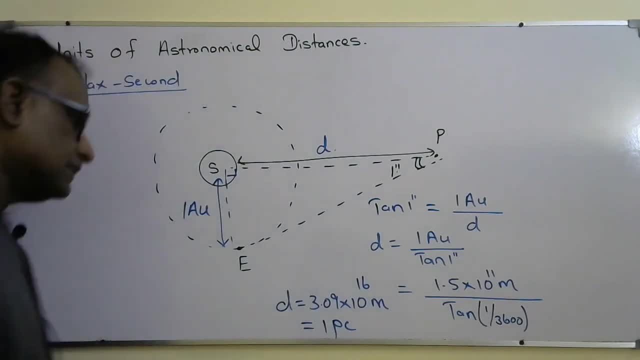 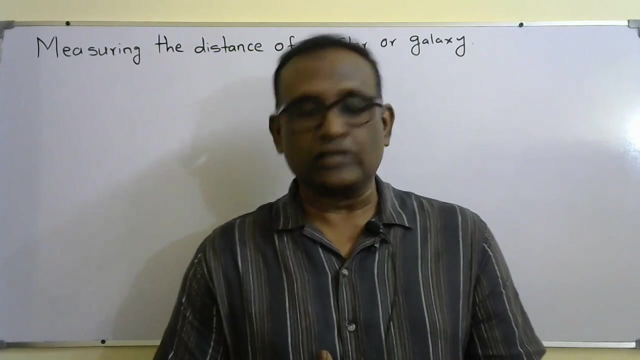 distance is defined as 1 parsec. This is defined as 1pc. So that means 1pc equal 3.09, 10 to the power, 16 meters. Okay so next topic is measuring the distance of a star or galaxy, That is one. 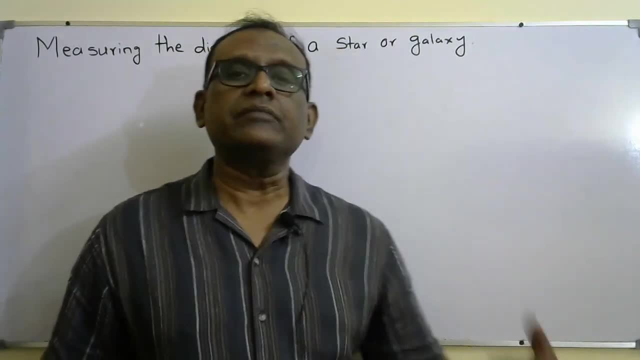 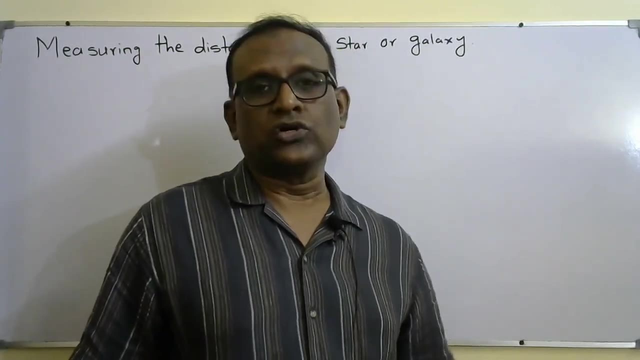 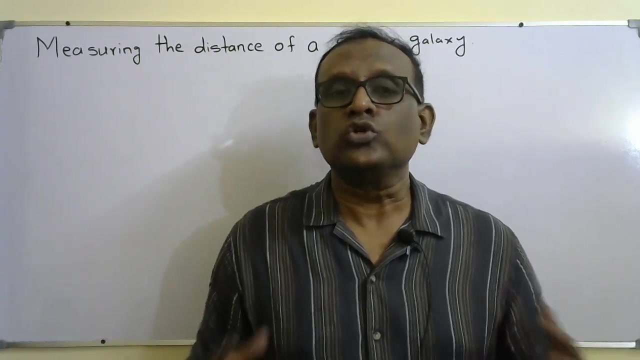 of the important topic in your syllabus. Okay, so different methods are used to with different accuracies. Say, for example, there's a method first we are going to learn called trigonometric parallax method. That method is suitable to do measurements up to a star at a distance of 100 parsec or 100. 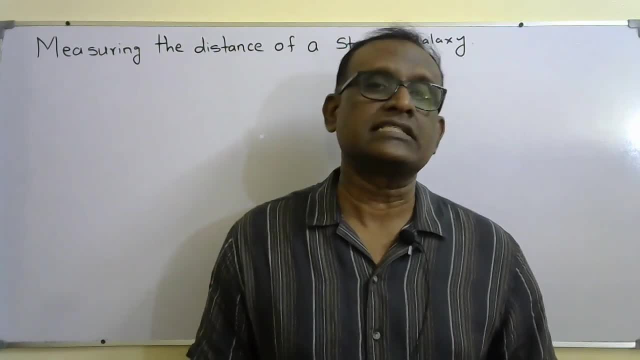 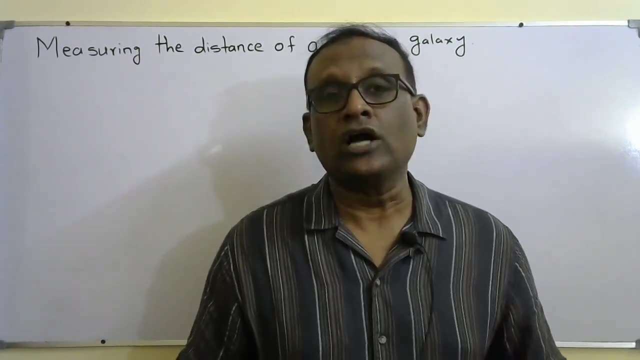 parallax second. You can't use that method if the distance of a star is more than 100 parallax second. So I'll let you know after explaining the first method. we call it as trigonometric parallax method. So it has actually it's a much better method compared to other methods. I am 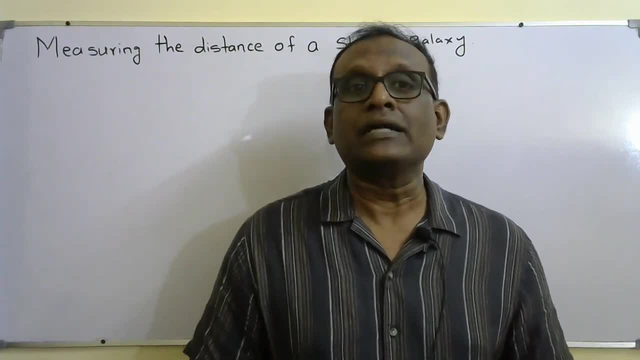 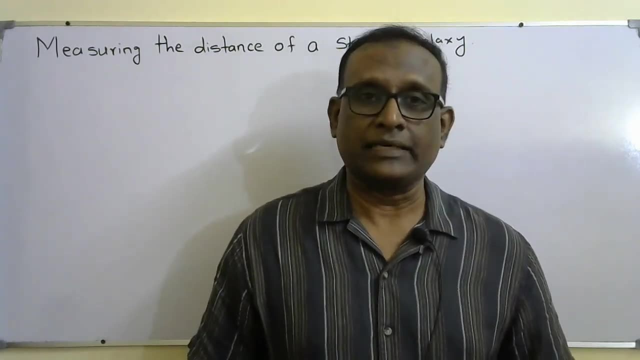 going to tell. but it has good accuracy, but it's limitation is shorter. You can measure, or you can use that method which is called trigonometric parallax method, only up to a distance of 100 parallax second. So I will explain that method now. 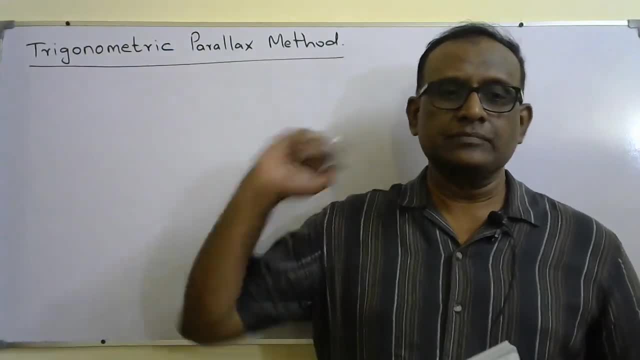 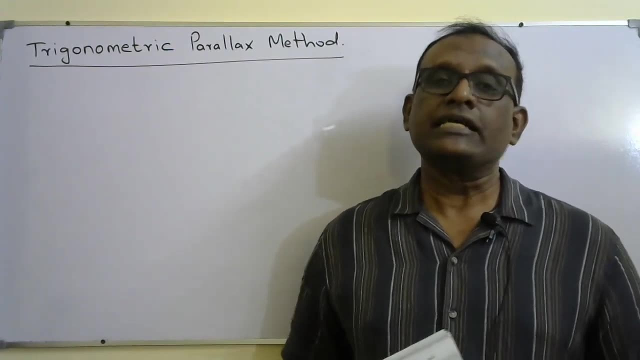 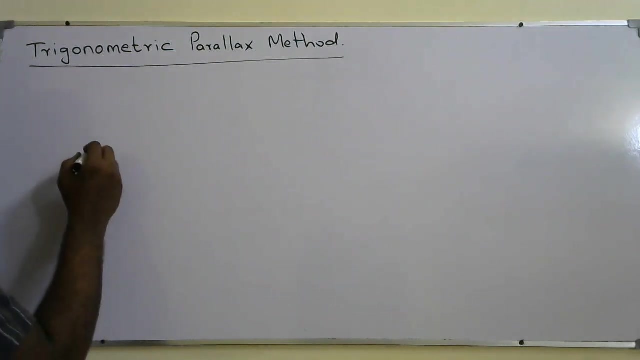 Okay, so normally we say this method, called trigonometric parallax method, is used to measure the distance of a star, measure the distance of nearby stars. nearby stars means up to a distance of 100 parallel second. okay, you know that the method how do you use here? this is the sun. 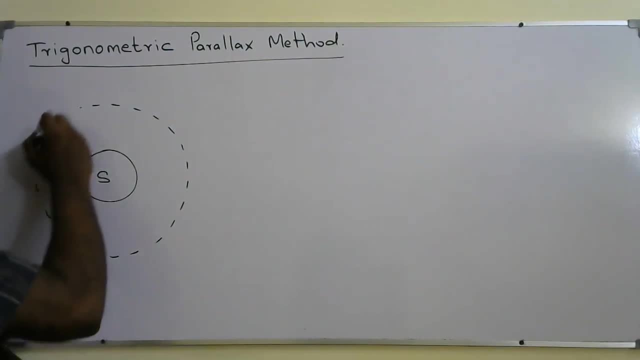 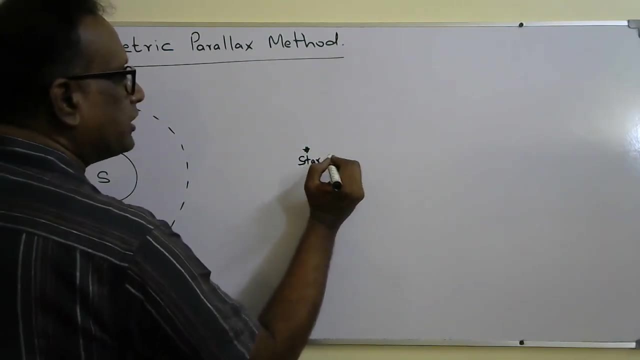 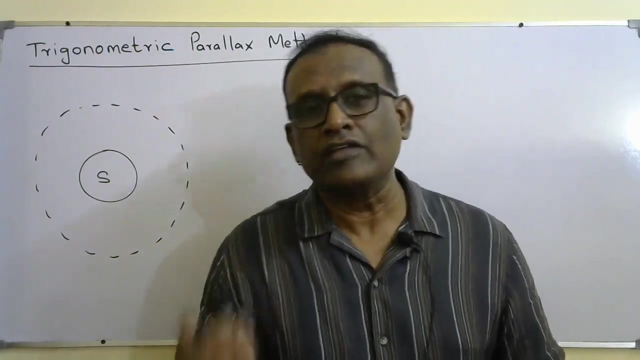 earth is orbiting the sun almost a circular path. so we are going to measure the distance of a nearby star. so this is the star, its distance we are going to measure. okay, so when we are taking measurements, mainly here, we are going to measure the angle. so when you are measuring an 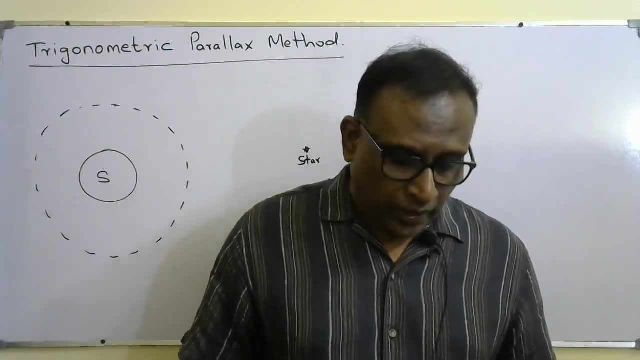 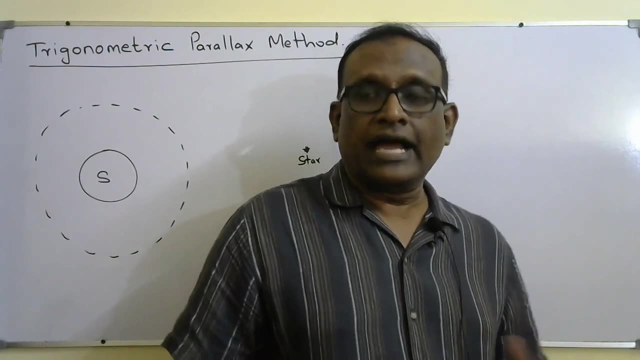 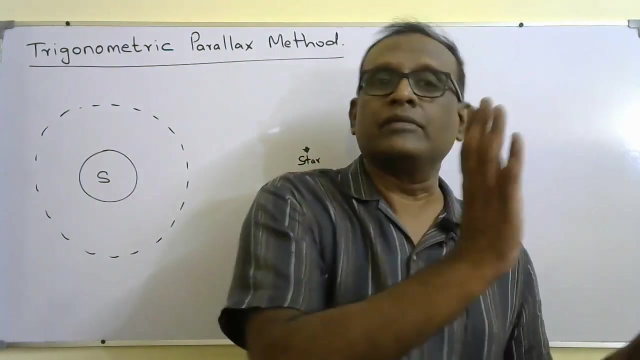 angle. we need a reference point, okay, so what, uh? how do we take reference point? you know, uh, normally you would have noted when you walk, uh, and when you see a far distance object, or maybe when you, in the night, when you see moon, and when you walk, you feel the moon is coming with you. 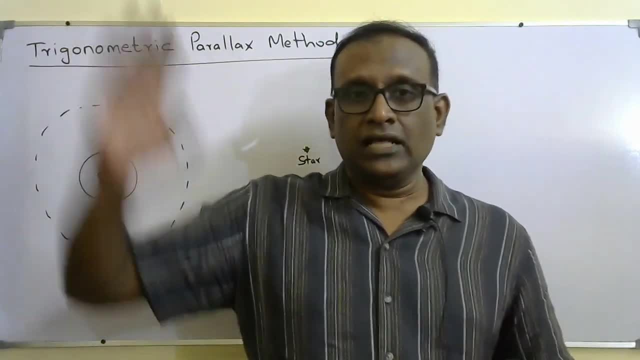 so the thing is, when the distance becomes much larger, the change in position, your change in position, won't change the distance of the star. so when you are taking measurements- mainly here- we are going to measure the angle. so when you are measuring an angle, we need a reference point. okay, so what? how do we take the reference point? you know, normally you would have noted, when you walk and when you see a far distance object, or maybe when you, in the night, when you see moon and when you walk, you feel the moon is coming with you. so the thing is, when the distance becomes much larger, the change in position, your change in position, won't. 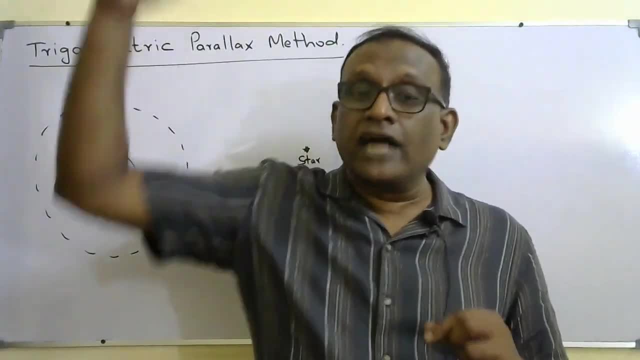 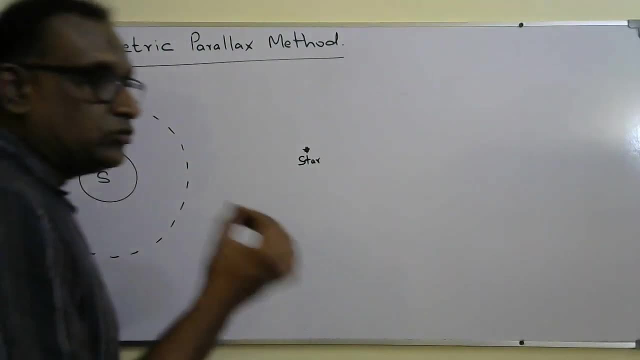 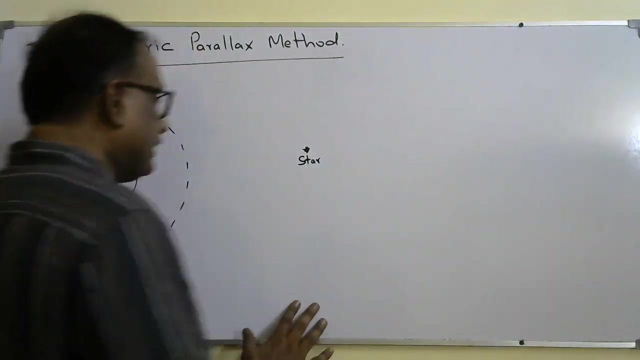 change in position won't affect the position of the far distance object. so here what we do in this method. we need a reference line to measure the angle we take. light from far distance stars, say, for example. there could be a star much far away somewhere. here the light from far distance star when the earth is here. 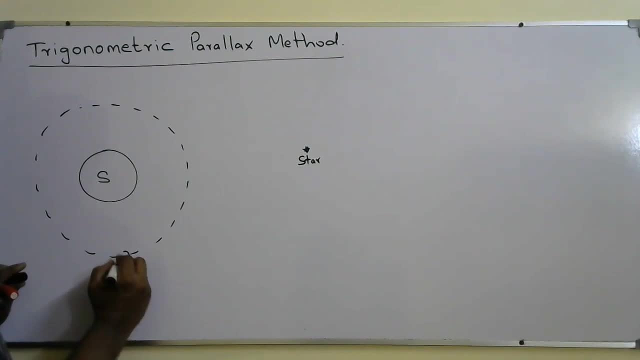 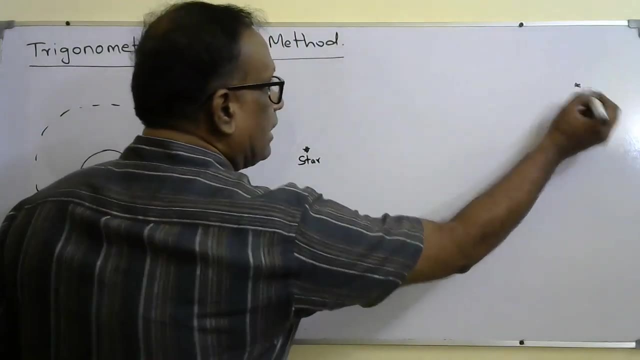 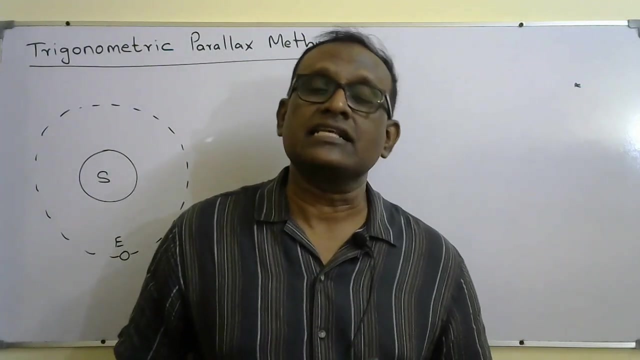 you observe that star, maybe the earth is here. when the earth is here, we see the star. light from a far distance, star somewhere here. so light from this star when we see that light will be taken as the reference line when we are taking the measurements of angles. so what? 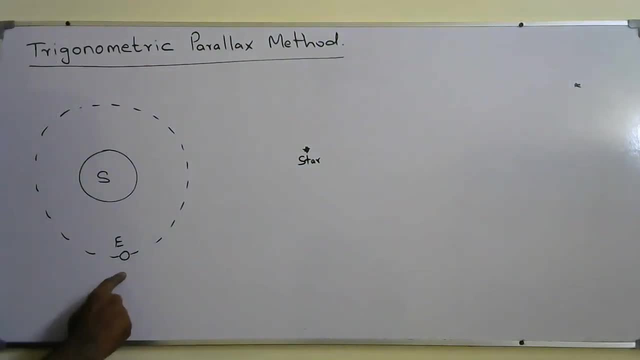 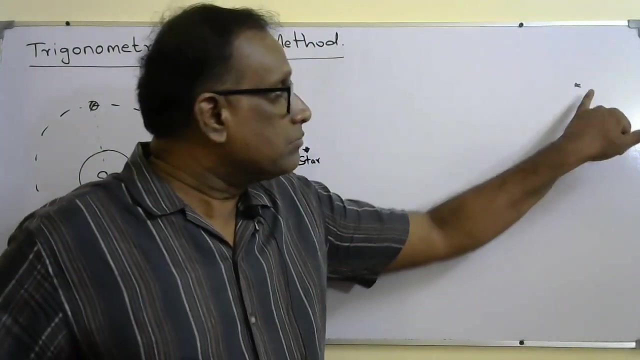 the method. first, i tell the method what we do. when the earth is here, we measure the position before the telescope to the star and we take a particular measurement. then after six months the earth will be exactly in opposite side here. there also, we take the measurement for the nearby star by using the same star, the light from the 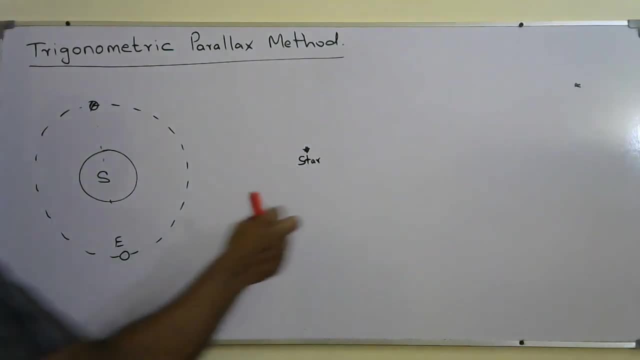 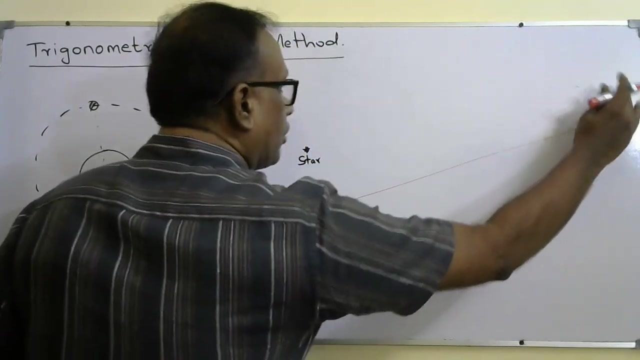 same star. so, for example, if the light from the star which is much far away, when it reaches earth, whether here or here, it looks like parallel. so if you draw a line from here to that part, something like this, maybe this I take, this I couldn't draw here. if I take this as the far, distant star somewhere here. 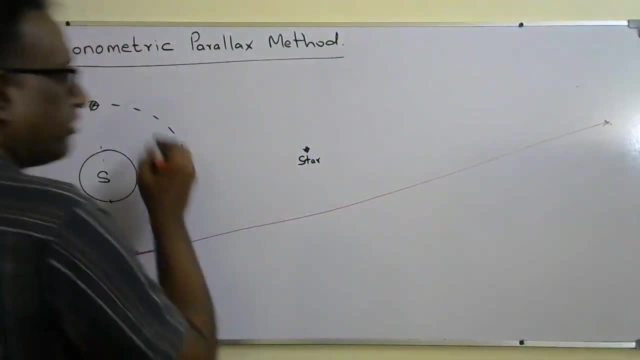 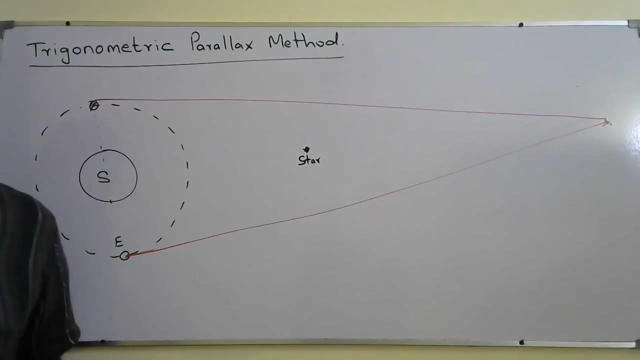 and this is the far distant star, same star. okay, now when I erase this part, when I erase this part, you see that these lines appear. okay, now, when I erase this part, you see that these lines appear almost parallel. so light from far distant star appears almost the same. 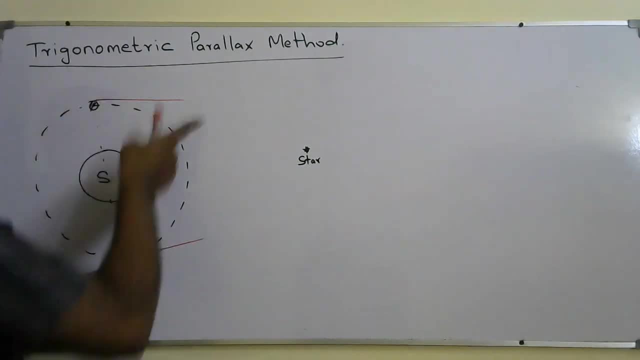 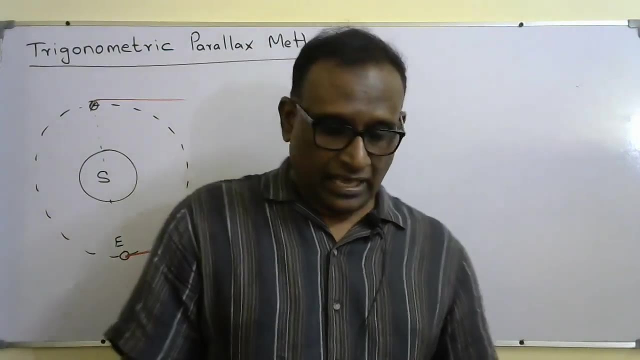 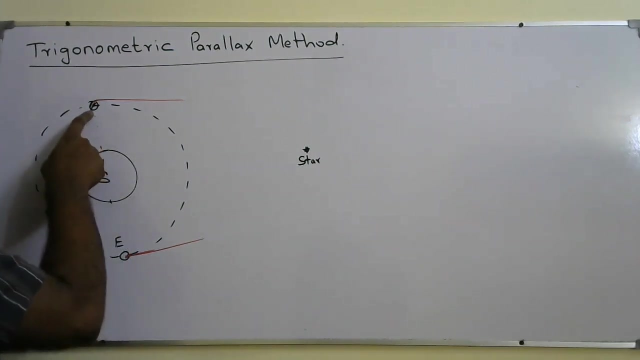 alignment, even when the position of the earth changes. so we use that light- light from far distant star- as a reference light and we measure the arc difference. so we take a measurement when the earth is here. after six months we take another measurement relative to the light from the far distant star. 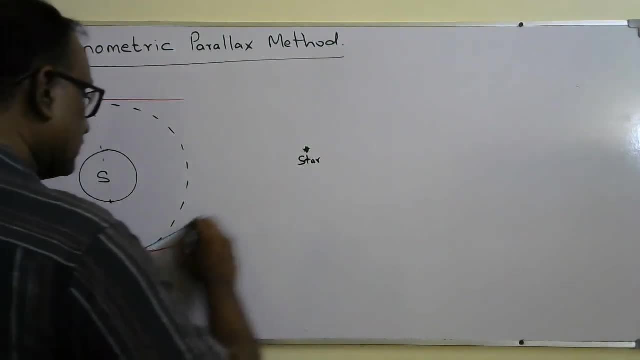 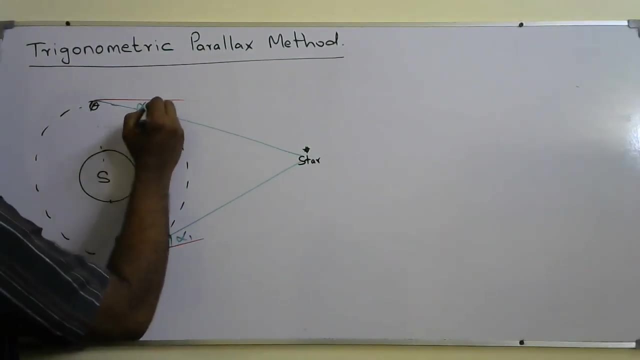 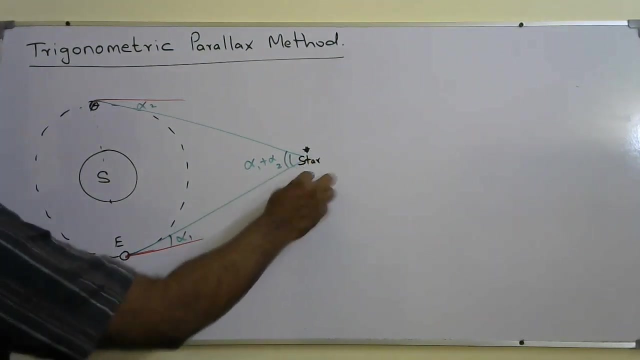 so we measure this angle. we measure this angle. alpha 1 could be alpha 2, so this angle will be alpha 1 plus alpha 2. that is called change in angular displacement or difference of the nearby star during six months period. so we can measure this. 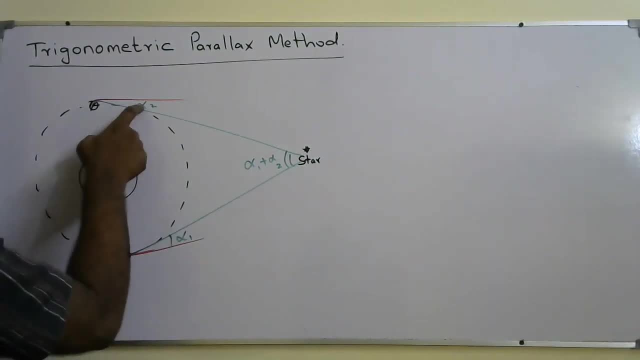 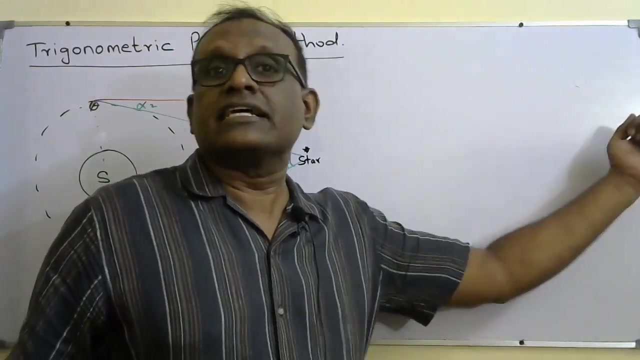 angle: alpha 1 plus alpha 2. alpha 1 is this one, alpha 2 is this one. so this angle will be alpha 1 plus alpha 2 because these two red color lights- red color lights indicates the light ray from far distance star. the light from the far distance star is taken as a reference line, so related to that. 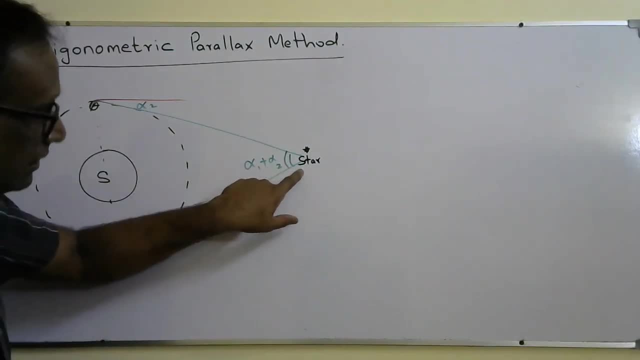 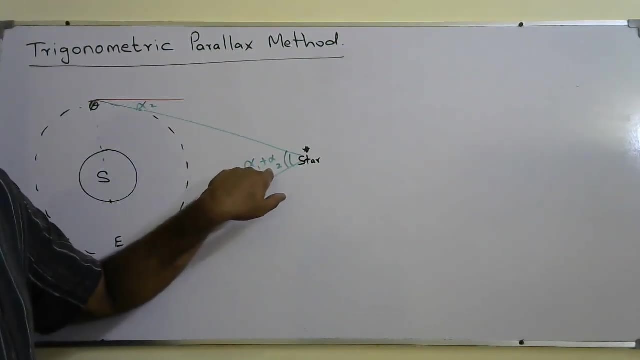 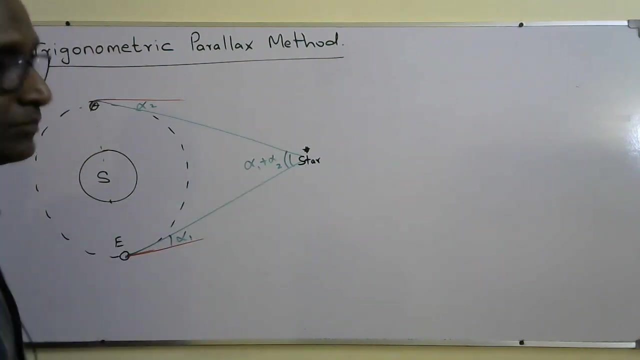 line. we measure these two angles. so the angle earth, star, earth during six months period. this is called arc difference or angular displacement of the star during six months. so if i know this angle, we measure this angle during six months, alpha 1 plus alpha 2. i know this distance, this. 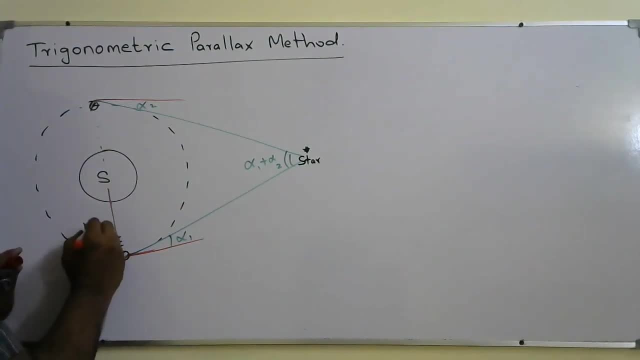 is one astronomical unit, one aeo. so now i can use trigonometry to find the distance of the star from the earth by using- we don't need to do any calculations, so we can find the distance of the star from earth during six months, or even distance of the star from sun. there is no big difference. 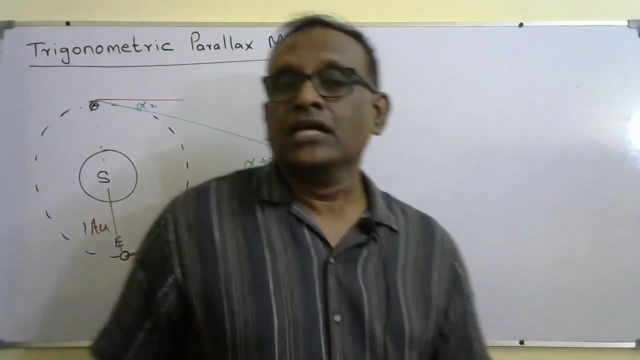 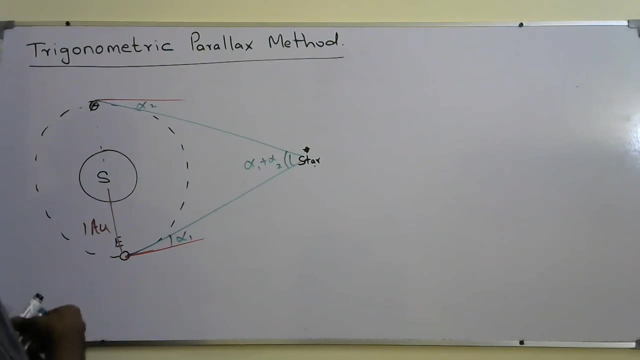 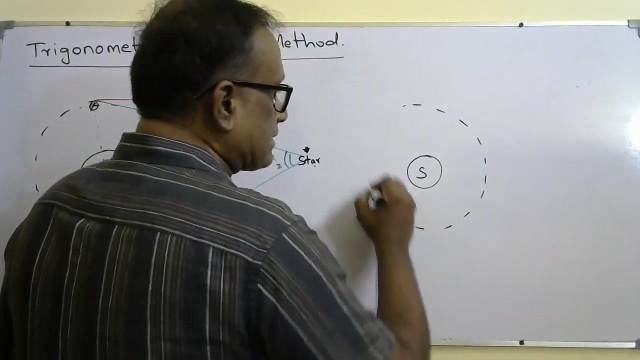 because these angles are very small, less than one degree normally. so we can measure the distance of the star by using trigonometry. okay, so if the simple diagram i can draw, the sun is here, earth is orbiting like this. so imagine simple diagram: earth is here, exactly here the star is. 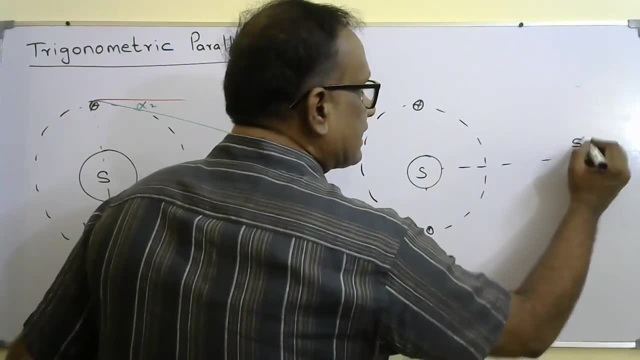 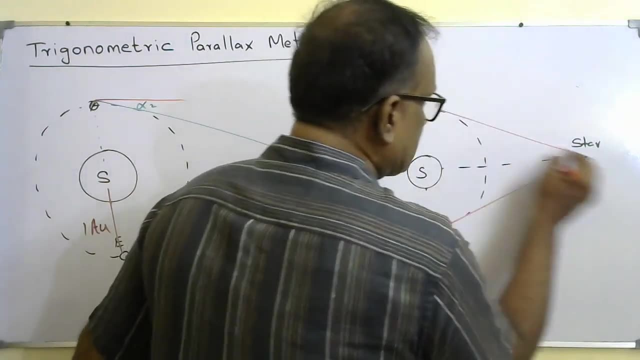 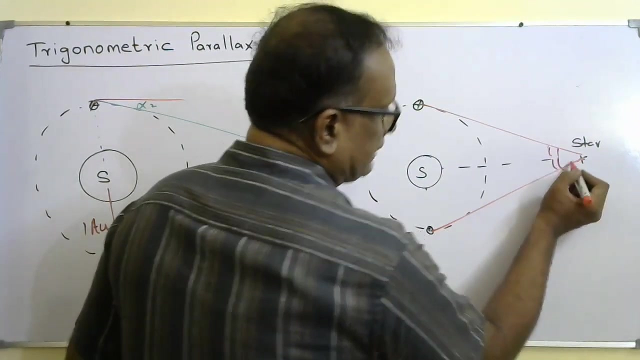 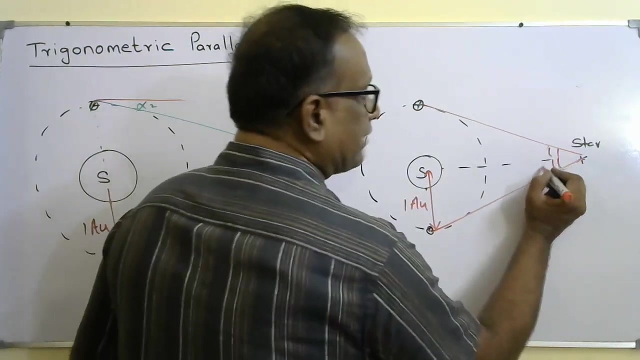 exactly here, but that won't happen. so if the star is here, i can measure this angle. so this angle, we can measure symmetrical nature. so this angle will be bisector, this line will be bisector. so if i know this angle, this will be half of it, this line, one astronomical unit. so simple. i can say tan theta, this angle, if i. 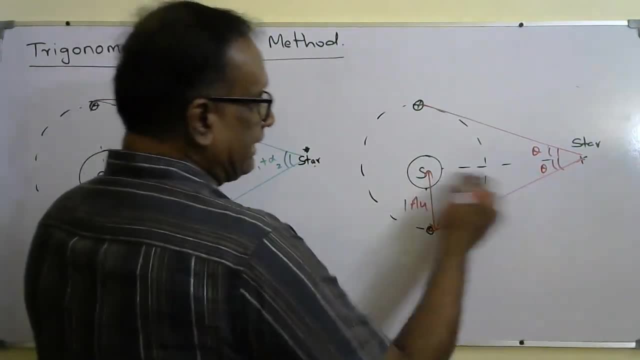 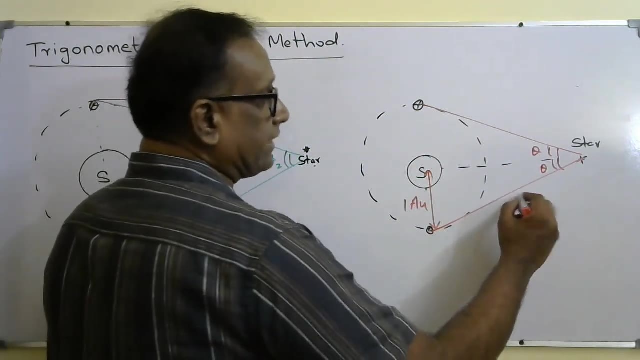 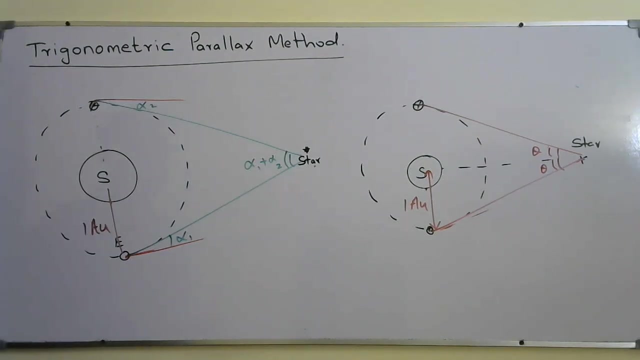 say theta, this also theta symmetrical. yeah, tan, theta equal one astronomical unit. over this length i can find the distance of the star from the sun, or i can use sine theta, which is one astronomical unit over this distance. so if the diagram is a symmetrical- but that won't happen always when we are doing practical- 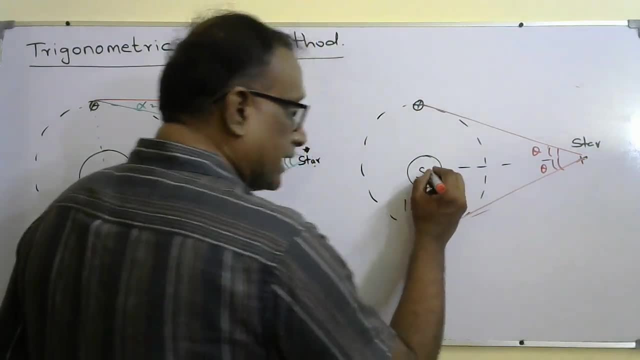 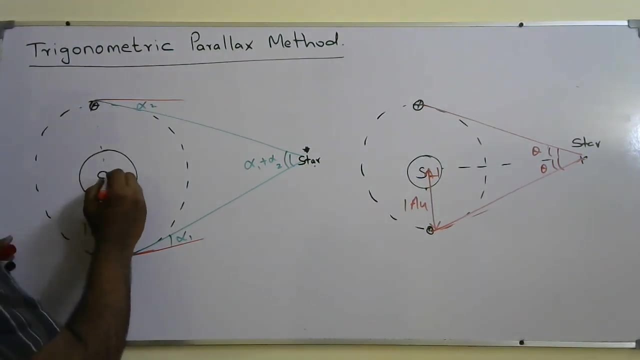 so the line, what we draw from the star to the sun and the line drawn from sun to the earth won't make 90 degree always okay. so here it won't make 90 degree. so we need to use the trigonometry. we can find it, but that type of calculations you won't get it. if you are getting a calculation, it will be in this: 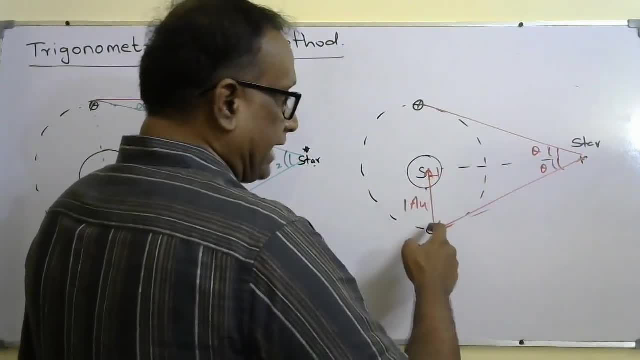 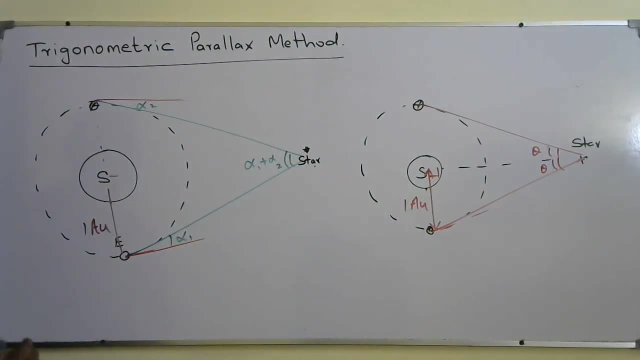 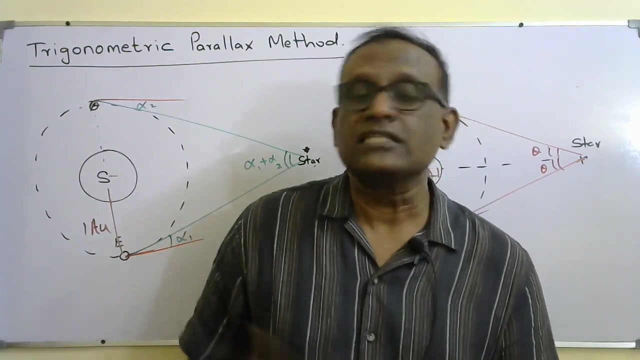 this format. This angle will be 90 degree. You can use tan theta or sine theta for this triangle. Okay, so normally they ask to describe the method that is called trigonometric parallax method. They normally ask to explain. So this is the four points. They give four marks. 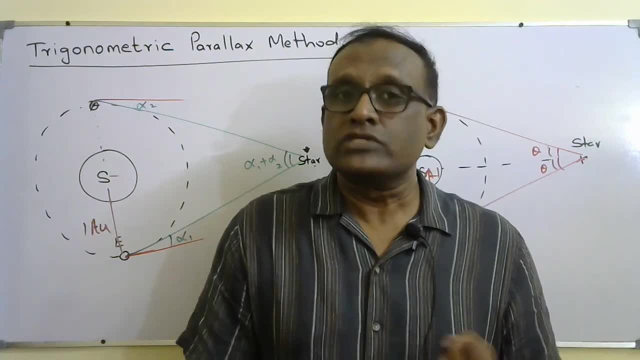 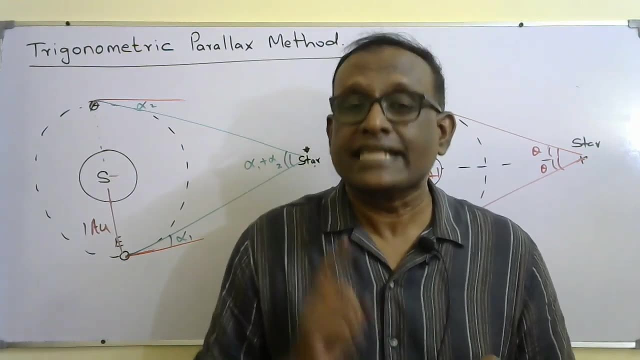 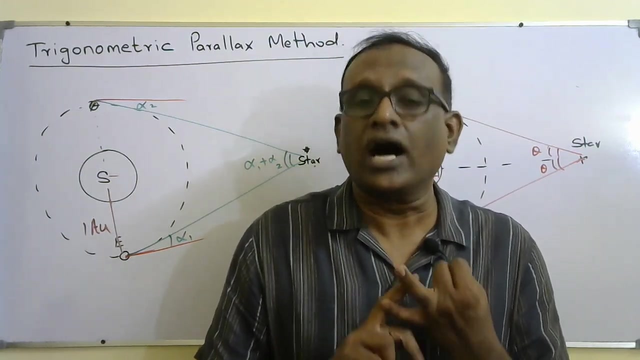 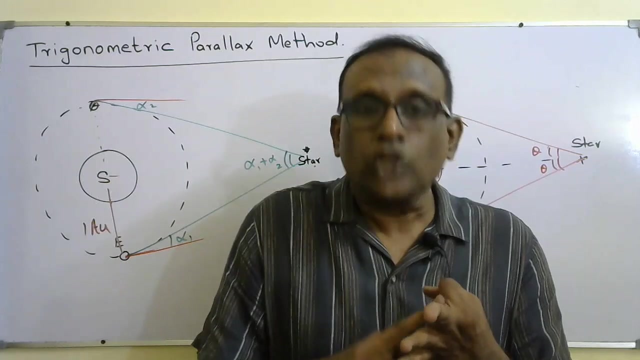 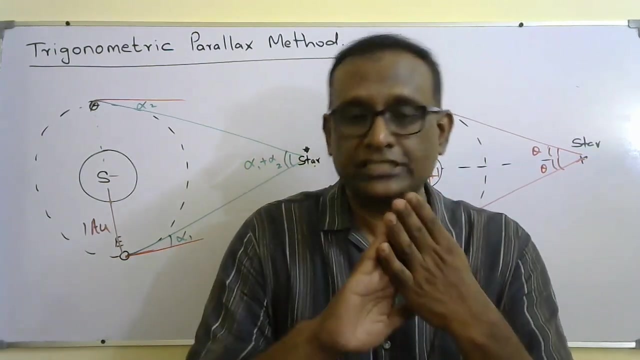 First, you should say: by using the light from far distance star as a reference light, take measurements during six months interval. By using these measurements, find the angular displacement or arc difference of the nearby star. Second mark: We should know the distance of the earth from the sun, which is one astronomical unit. Third mark: By using trigonometry, find. 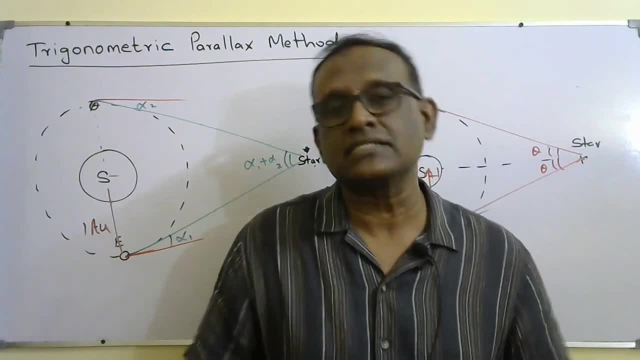 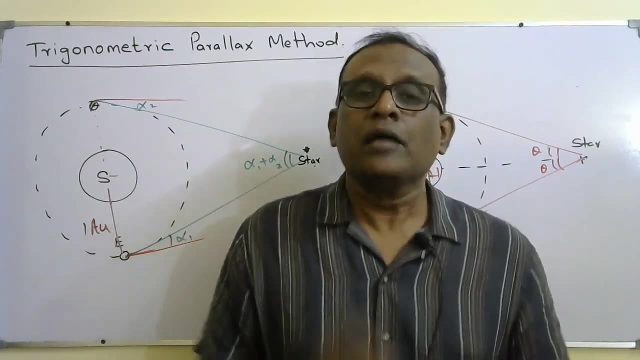 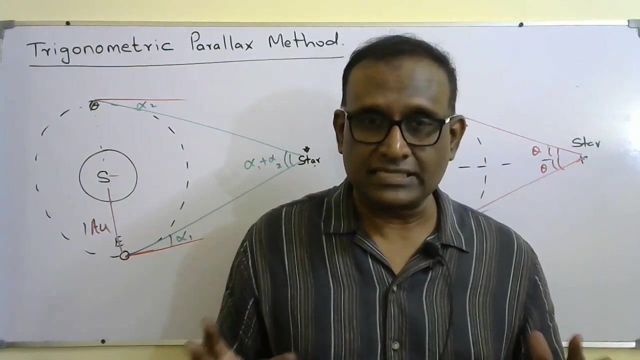 the distance of the star from the earth. Those are the four marks they gave Last. I think it appeared three times in the past year but that is the marks given for that. Again, I am telling measure during six months interval by using light from far distance star as a reference light Measure. 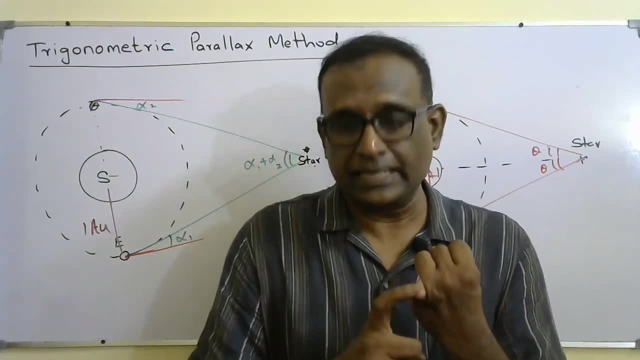 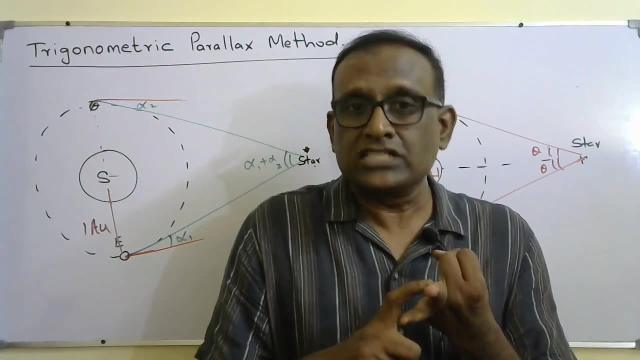 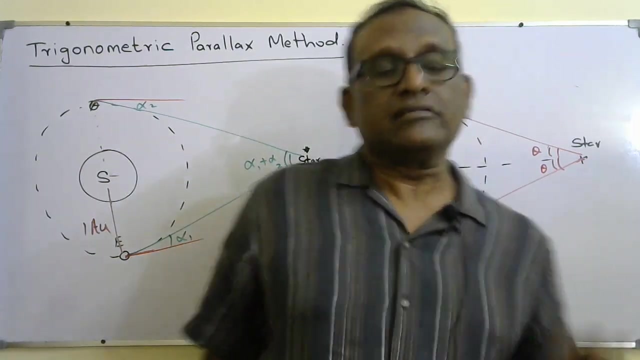 the angular displacement or arc difference of the nearby star. One mark: You should know the radius of the earth's orbit around the sun. You should measure by using trigonometric parallax. In trigonometry we can measure the distance of the star from the earth. These are the 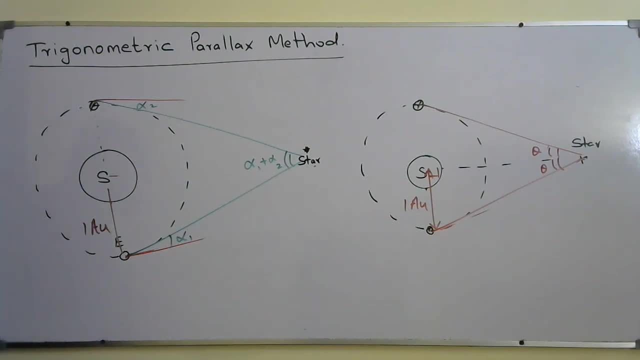 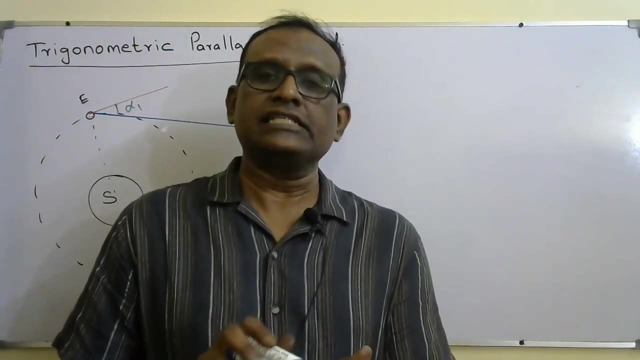 four points they gave in the past paper. What is the limitation of this method? Why can't we measure a star which is at a distance more than 100 parsec? If the distance of a star is more than 100 parsec, if the star 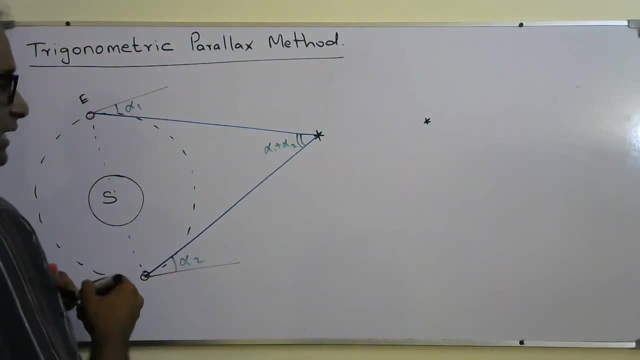 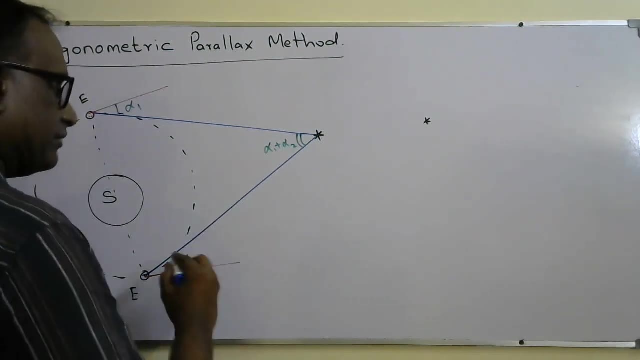 is somewhere here, what will happen? The angle, this angular displacement or arc difference, will become smaller. You can draw a simple diagram and see. It is difficult to draw it on the board, But if you draw you can see that this angle will become smaller. Compared. 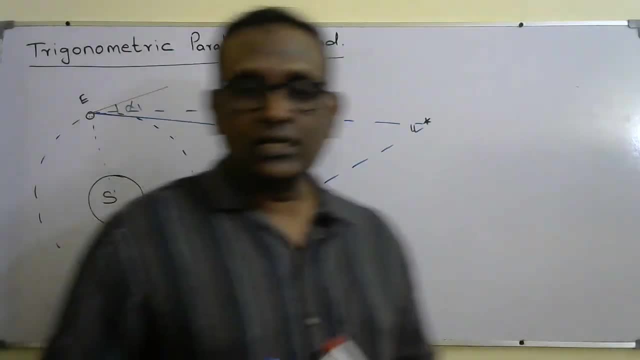 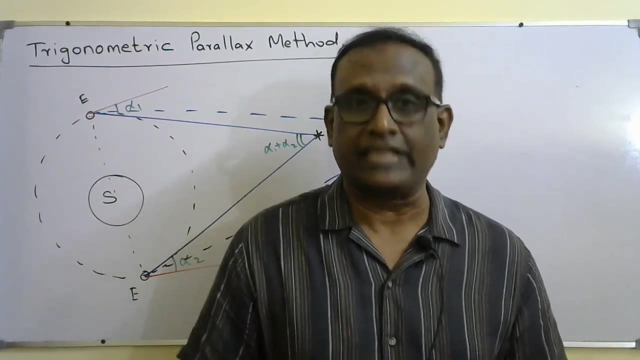 to this angle. this is smaller. When the angle becomes smaller, we won't be able to measure that angle by using any apparatus. Maybe it could become smaller than the precision of the apparatus, So the percentage uncertainty will become larger. So that's the reason this. 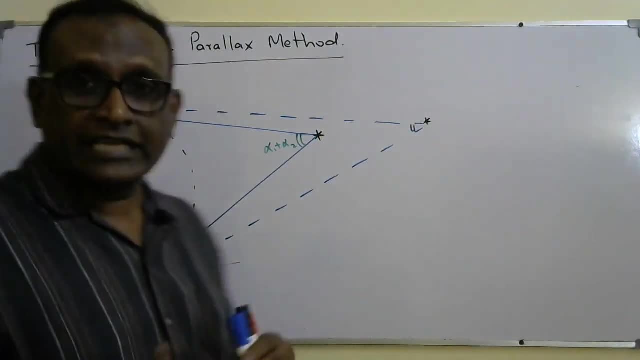 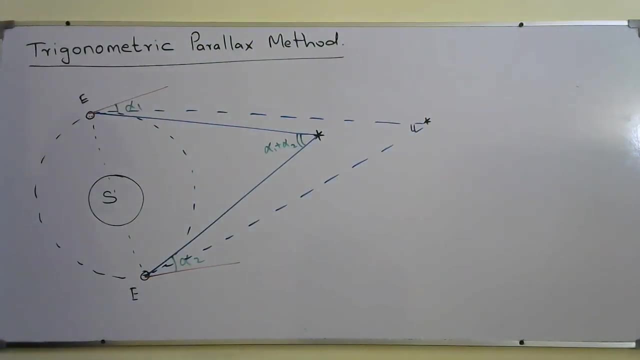 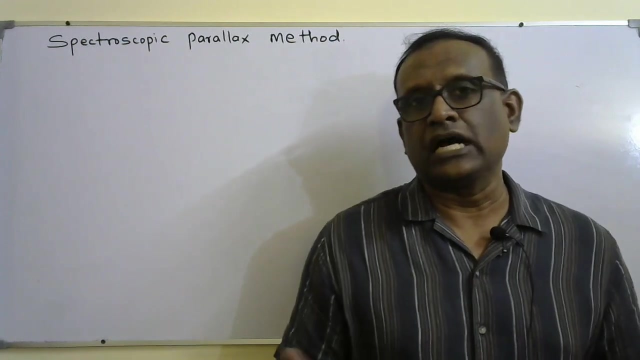 method has limitations, But this method is a good method for nearby stars. But this method has limitations. We can use this method only up to a distance of 100 parsec. So if the distance of a star is more than 100 parsec, we can't use trigonometric parallax. 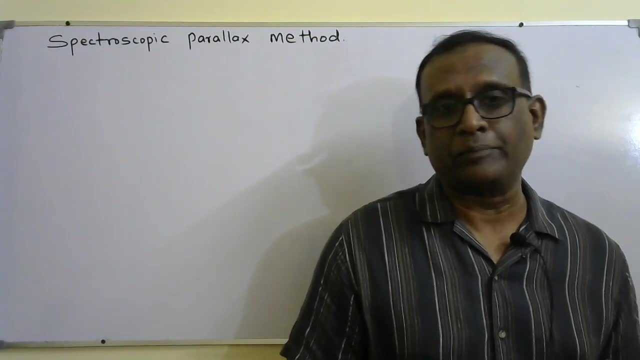 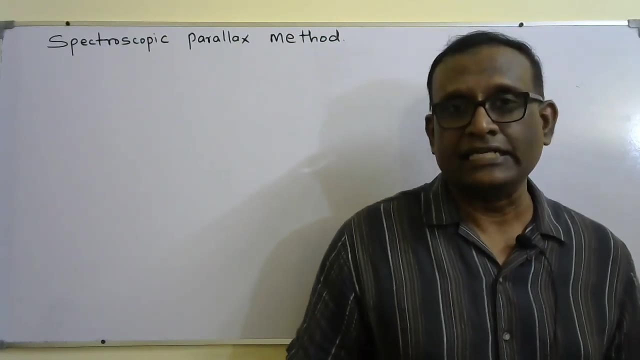 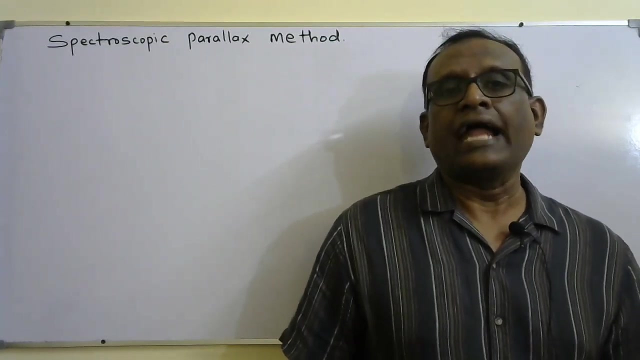 method. So the next method is spectroscopic parallax method. So spectroscopic parallax means here the spectrum is used. Actually, as I explained earlier how to measure the temperature Here, what we do, Suppose the telescope receives the radiation from the star and disperse its spectrum into 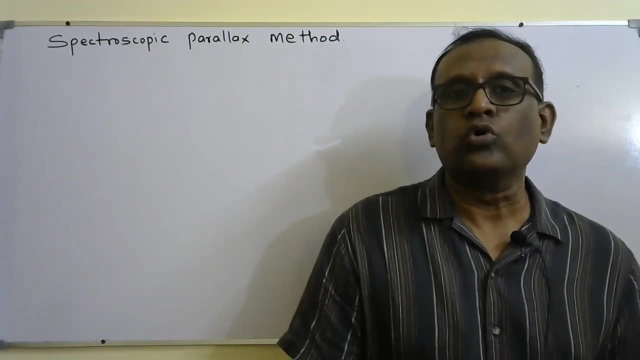 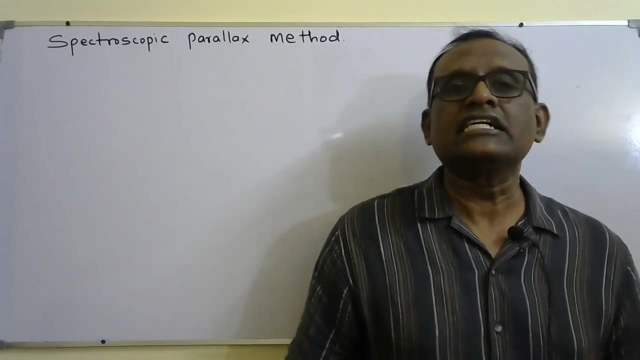 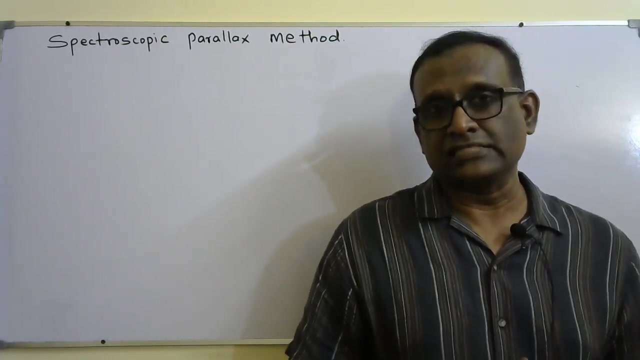 different wavelengths. Identify the most intense spectrum and find its wavelength By using Hertzsprung-Russell diagram. find the by assuming we should assume that the star is in the main sequence. That's one of the drawbacks in this method. We assume the 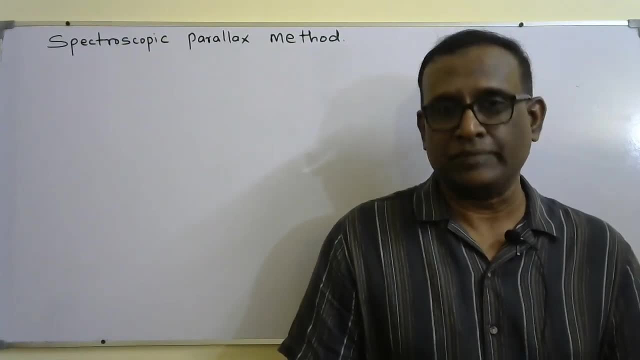 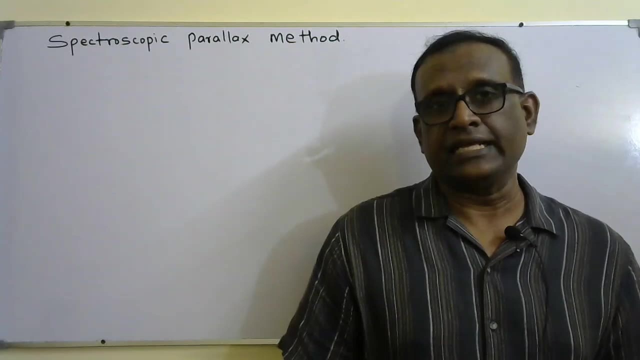 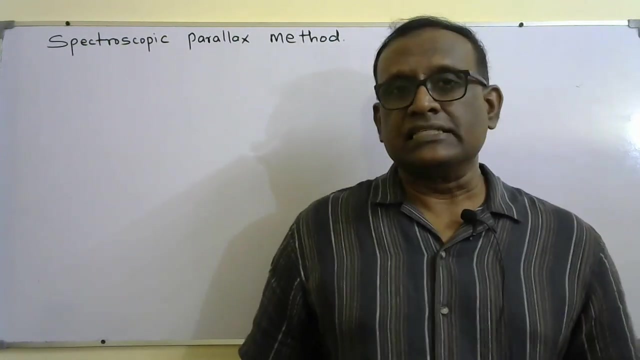 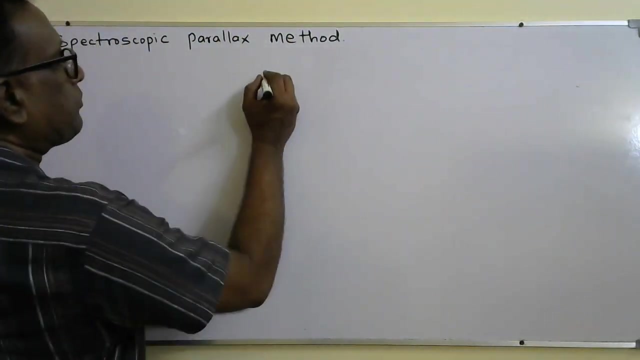 star is in the main sequence. Use the Hertzsprung-Russell diagram to find the luminosity of this star. After finding the luminosity of the star, we know the luminosity Measure, the intensity of the light from the star. So we know the intensity of the star, We know the luminosity, by using L equal 4.0. 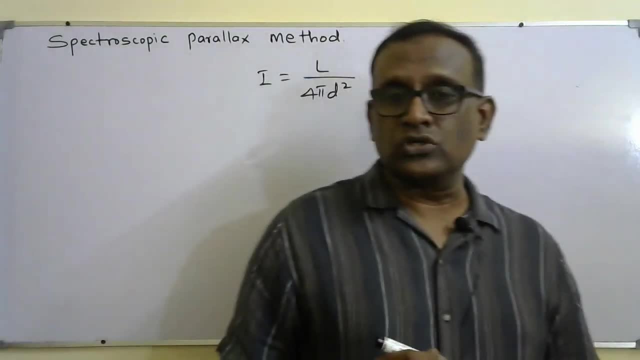 I equal L over 4.0.. This is where we had these equations in unit 2.. This is where we had these equations in unit 2.. This is where we had these equations in unit 2.. The intensity varies in the square law. 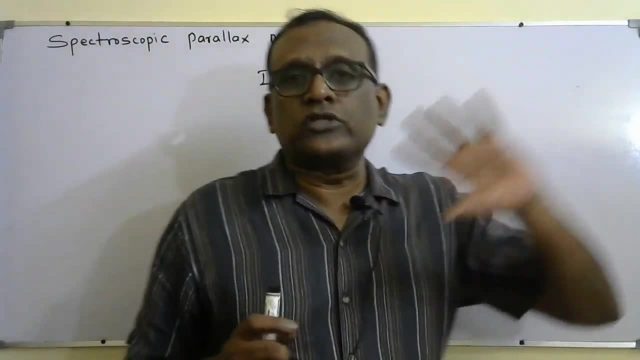 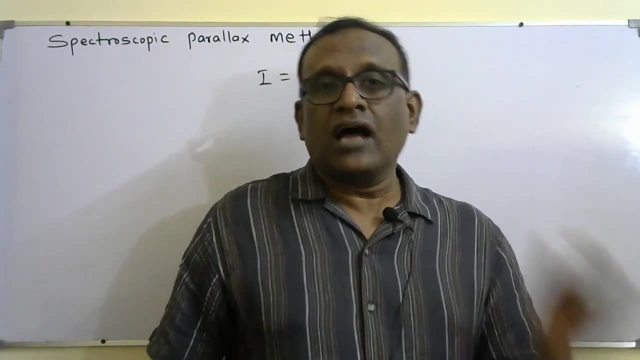 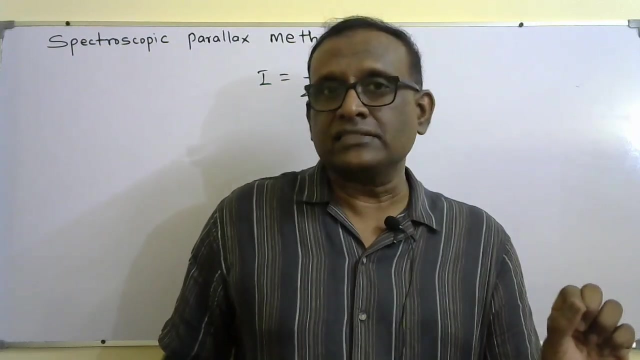 So what we do? Again, I am telling you: focus the telescope to the star, Receive the radiation, Identify its spectrum, Disperse it into different wavelengths, Identify the most intense radiation in the spectrum and find its wavelength. After finding the wavelength, use Wien's law and find the. 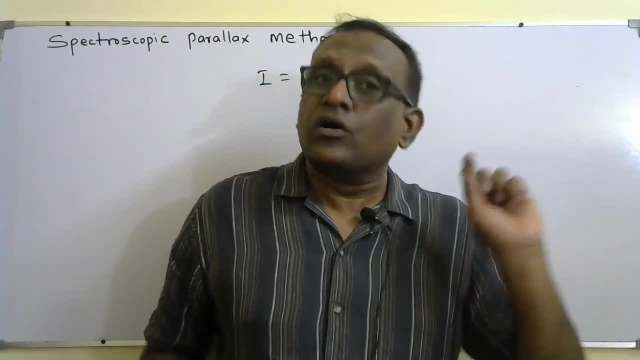 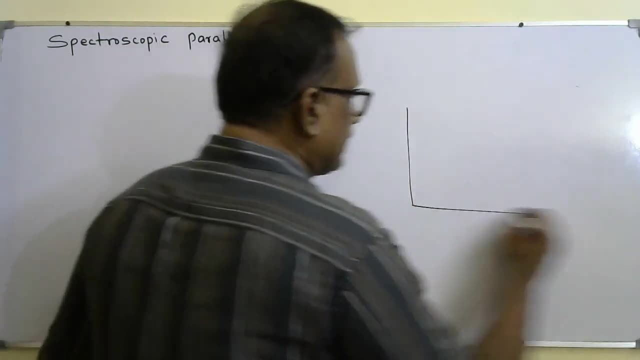 temperature. We have to find the temperature that corresponds to the wavelength with highest luminosity. Then use the Hertzsprung-Russell diagram. So the Hertzsprung-Russell diagram, this is the temperature, this is the relative luminosity. 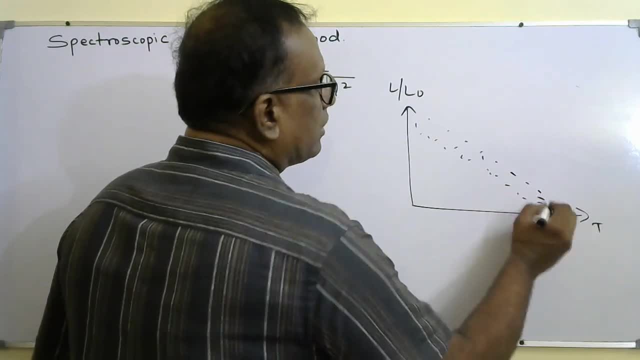 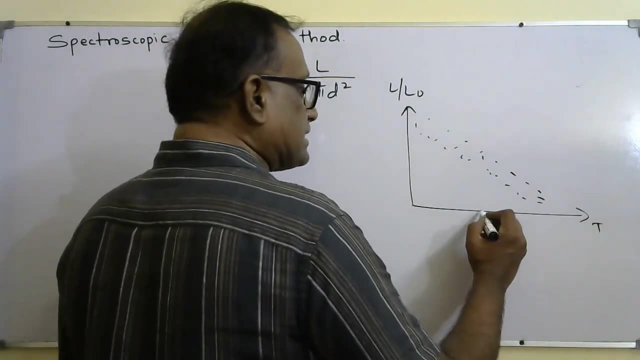 So this is the main sequence star. So we assume the star is in the main sequence. It's a wrong assumption, but there is no other option. We assume the star is in the main sequence. So if the temperature is something like this value: 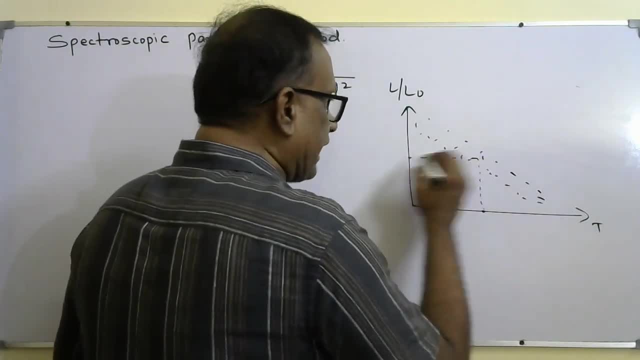 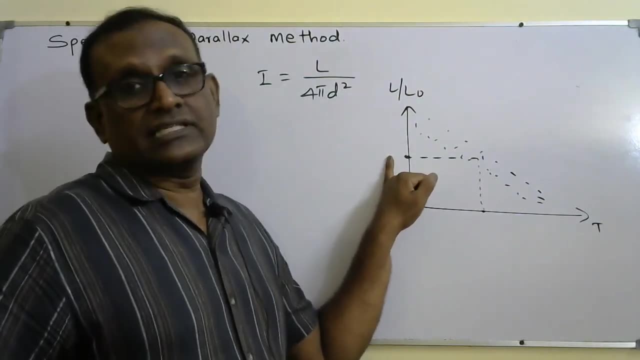 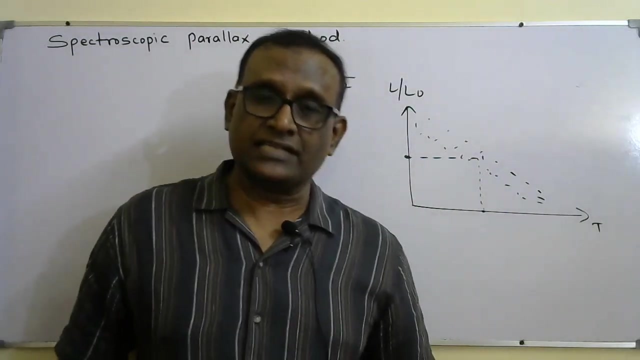 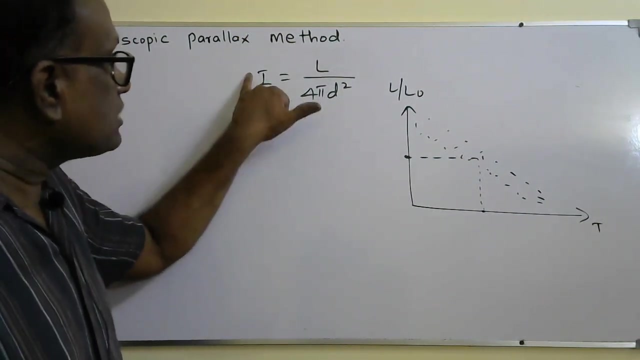 Then we can calculate the temperature. So this is the temperature From the HR diagram. find the relative luminosity. Since we know the luminosity of the sun, we can find the luminosity of the star. Now we know the luminosity of the star, Then measure the intensity or radiation flux for the light coming from the star. Measure the intensity: We know the luminosity. we found it By using I equal L over 4 pi d squared. find the distance. 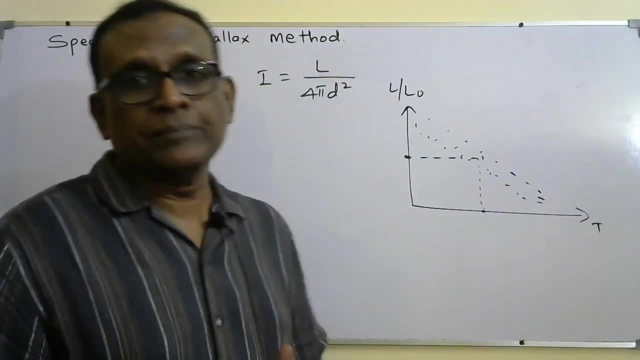 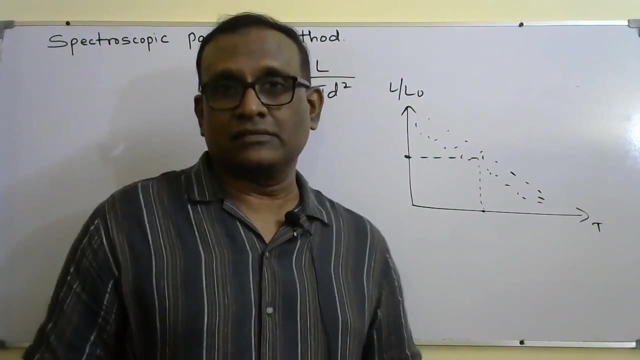 Okay, so here in this method, the drawback or the limitation is we assume the star is in the main sequence. That's one of the biggest method mistake. We don't know whether it's in the main sequence, but we assume the star is in the main sequence. 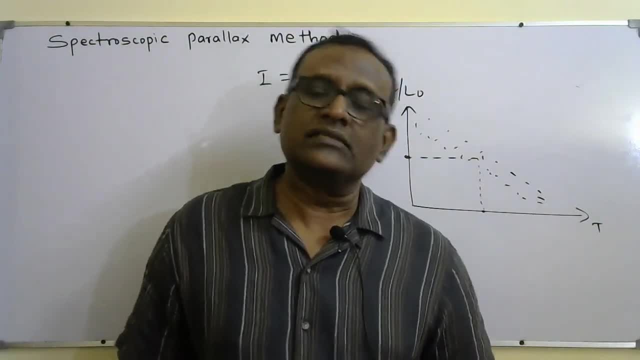 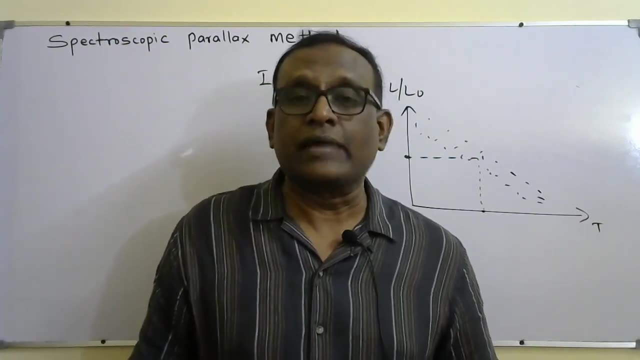 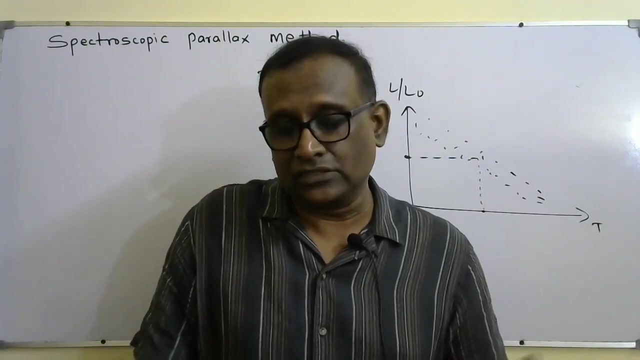 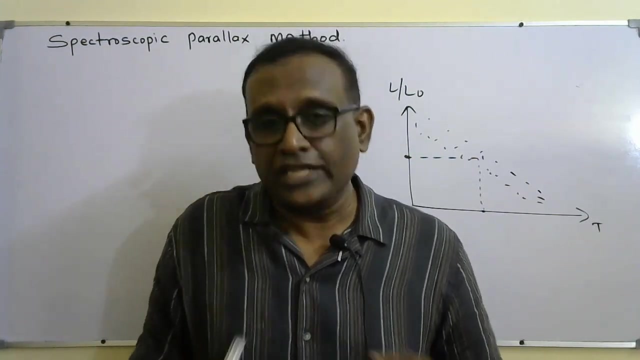 But when you go through different books or other internets they tell this method in a slightly different way, by using apparent magnitude, actual magnitude. But in your syllabus we don't use those Terminal, those words or those techniques: apparent magnitudes, absolute magnitude. So your syllabus we use this way, that is, measure the radiation from the star. 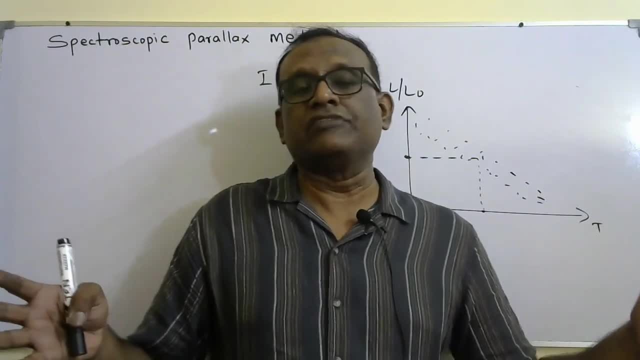 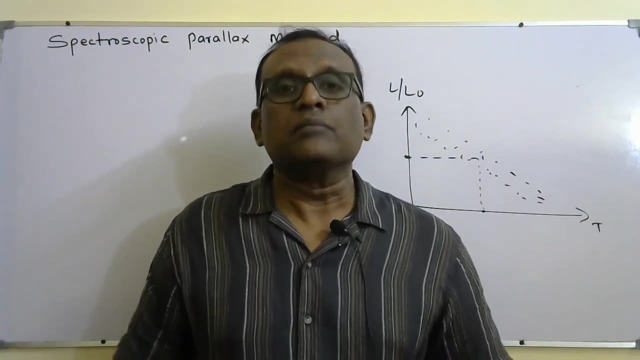 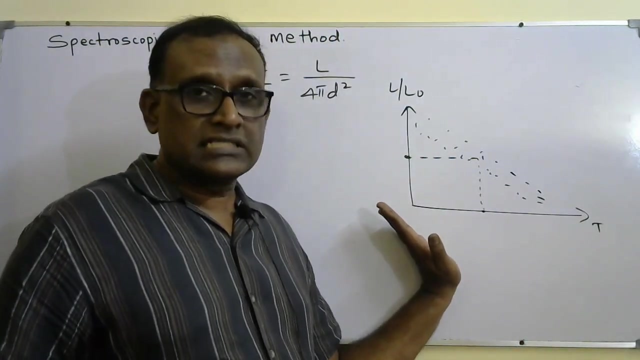 Find its spectrum, Disperse it in different wavelengths, Identify the most intense radiation, and the relevant wavelength should be measured By using Wien's law. measure the temperature of the star surface. temperature of the star: Use the H-R diagram. Assume the star is in the main sequence. By using the temperature, what we found? 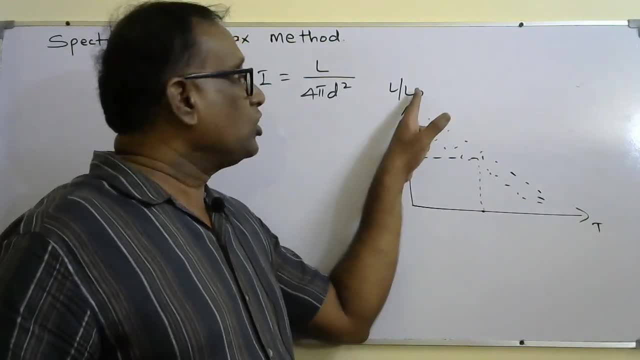 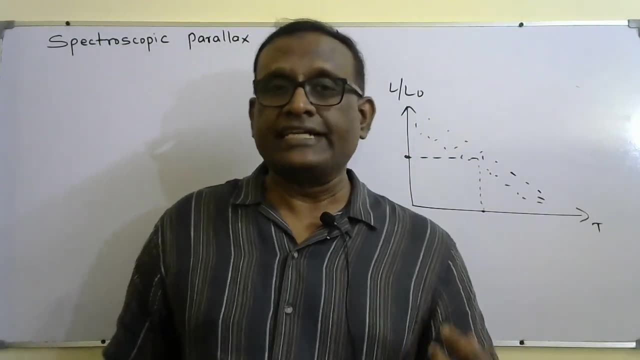 Find the relative luminosity of the star. Since we know the luminosity of the sun, we can find the luminosity of the star. Also measure the radiation flux, or the intensity of the radiation from the star. We know the I, We know the L, So find the d by using this equation. 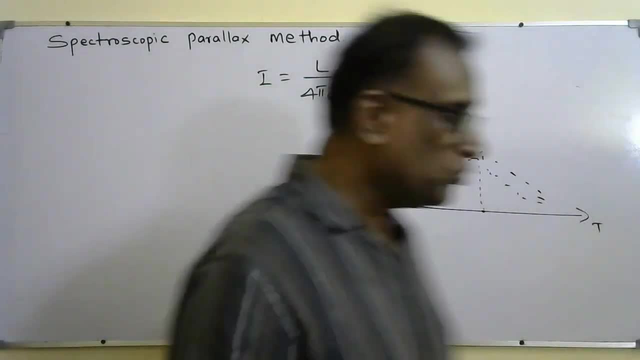 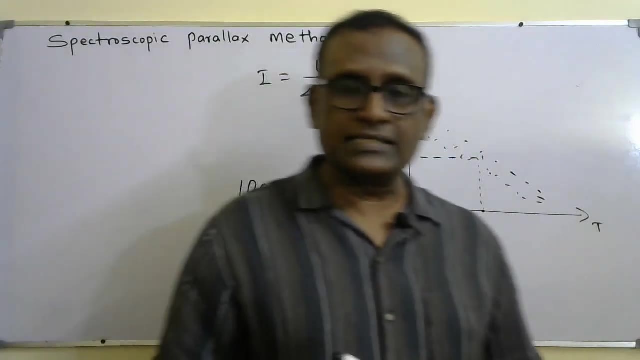 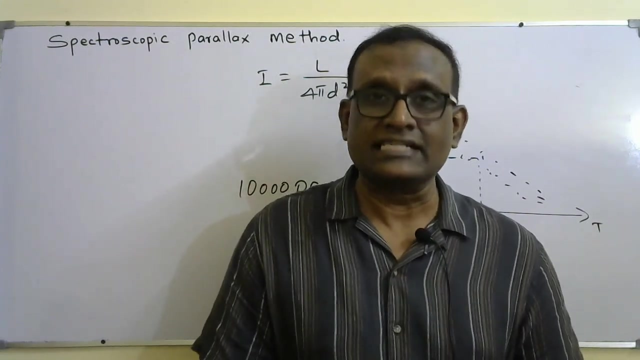 This method also has limitation. This method can be used up to a distance of ten 10,000 parsec. So if the distance becomes more than 10,000 parsec, what's the problem occurs? The problem is there will be difficulty in identifying the most intense radiation. You 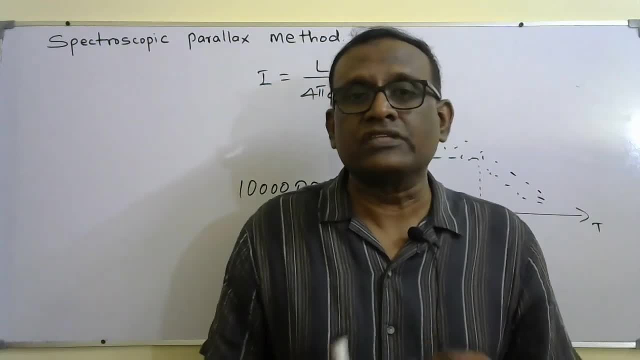 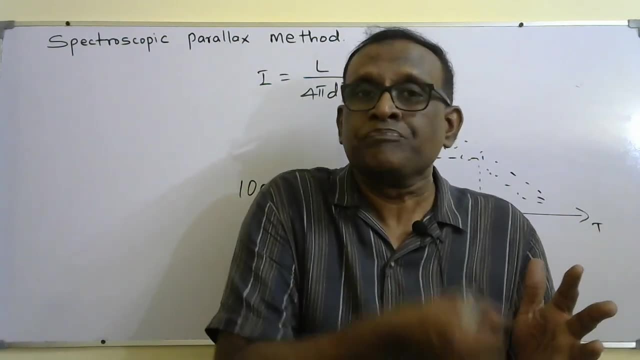 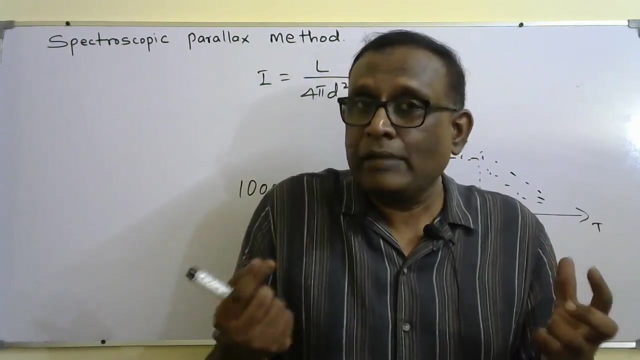 know that when the distance increases the intensity of the radiation. So here we are focusing the telescope and we are dispersing it. After dispersing it, we are measuring the intensity of each and every wavelength after dispersion, and we identify the most intense wavelength So we might be able to measure the intensity of the radiations. but the 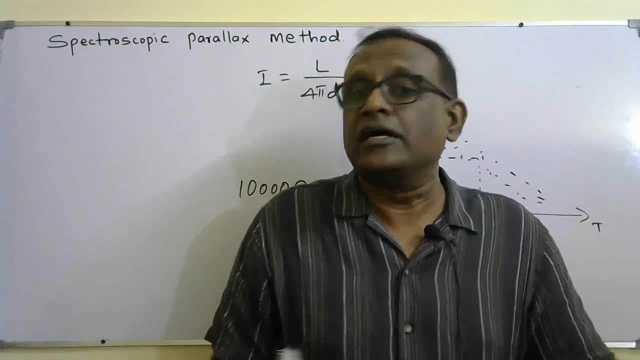 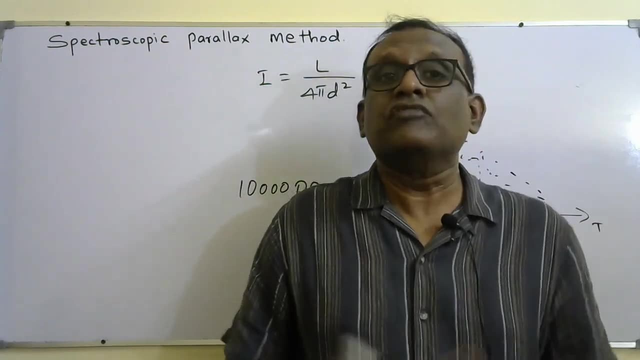 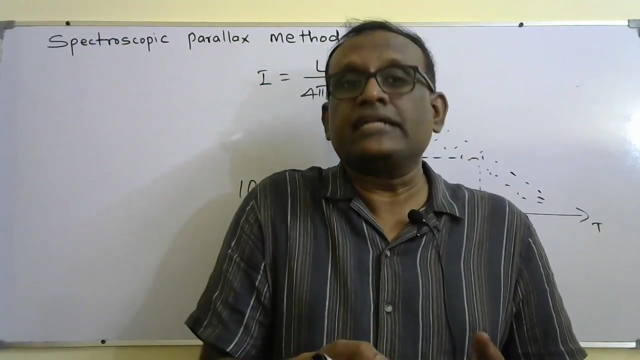 variation might occur beyond the least count of the measuring instrument. So if that happens we won't be able to identify the most intense radiation. There will be measurements. You might get numerical value for the intensity of each and every radiation after disperse. 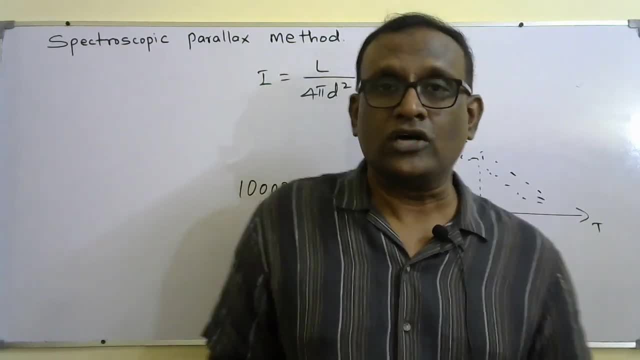 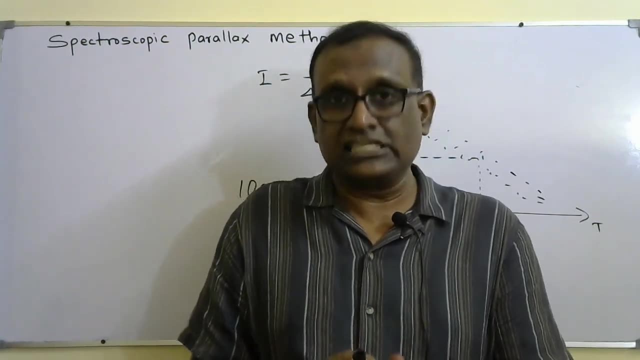 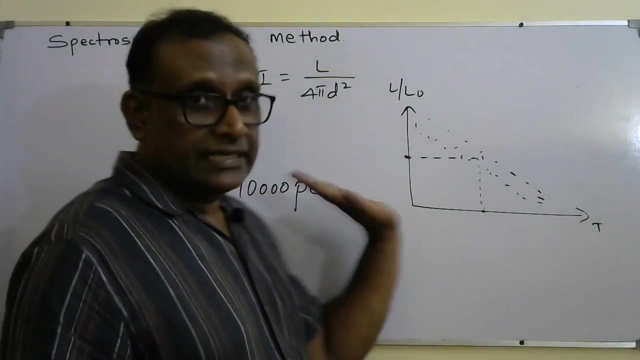 but you won't be able to identify the most intense radiation because they all might appear the same. There will be difficulty in identifying the most intense radiation when the distance of the star becomes more than 10,000 parsec. So when the distance becomes more than 10,000 parsec we can't use spectroscopic. 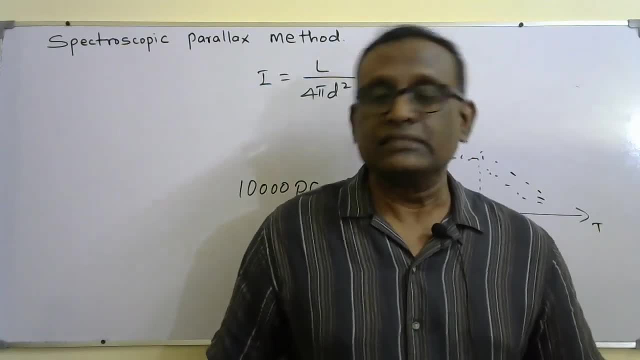 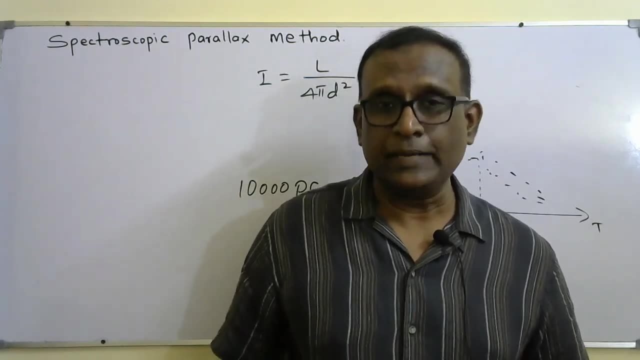 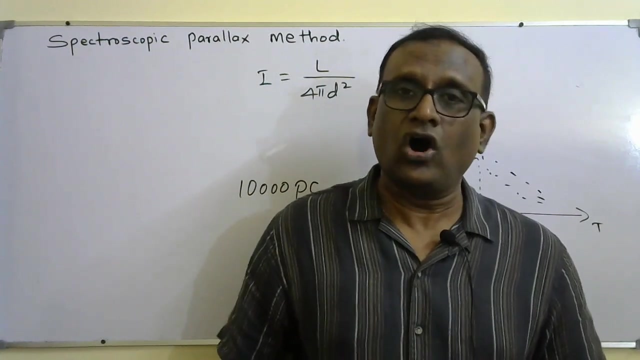 parallax method. We need to go for the next method. There we use standard candle. That means standard candle means a star with The known luminosity. We can. There are two different methods. We can use a seth variable as a standard candle or we assume the luminosity of a star is known. Either way we can do. 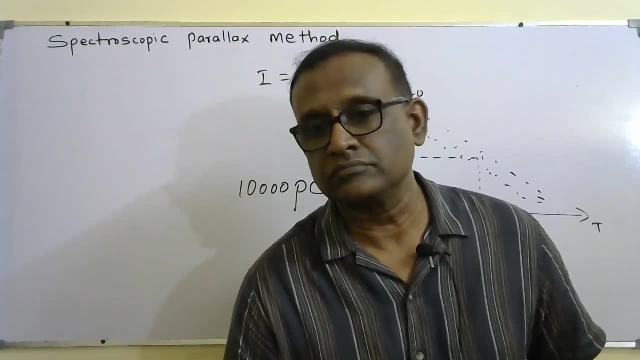 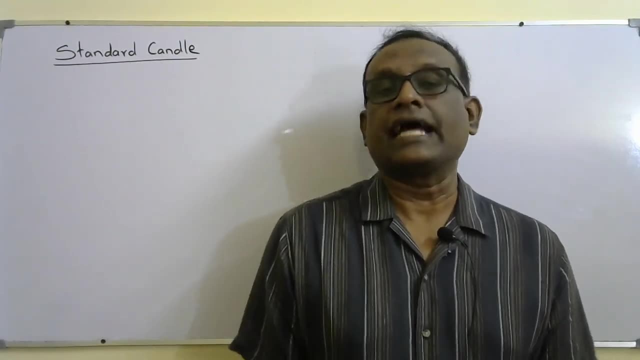 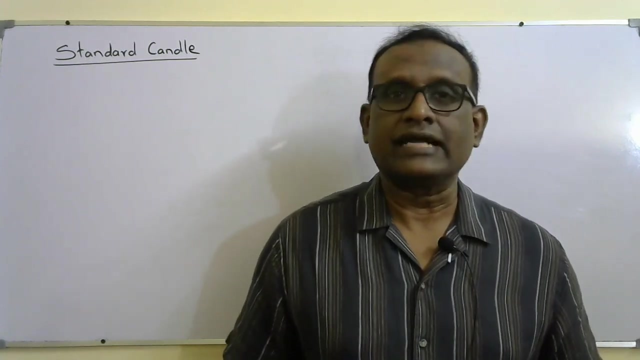 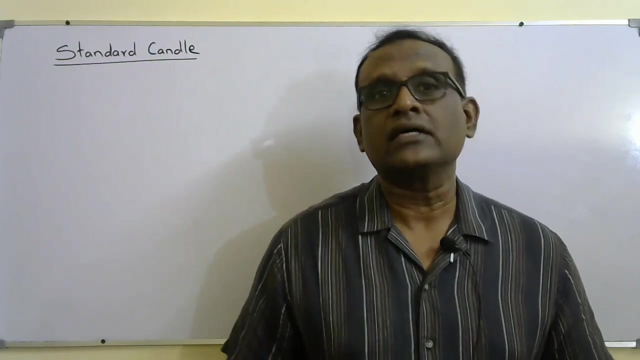 I'll explain that in my next method. Okay, Next topic is standard candle. What do you mean by standard candle? means a star or an astronomical object with known luminosity. So time they asked in the past paper what a standard candle means: a star or an astronomical object with. 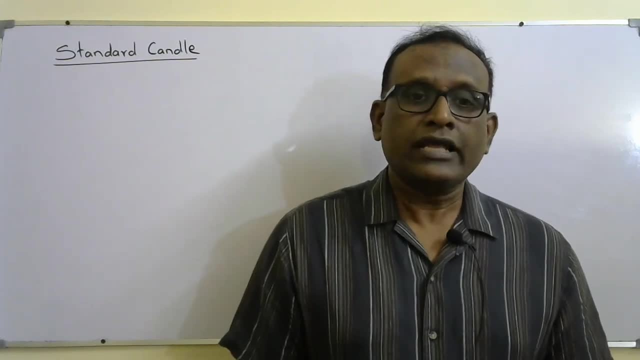 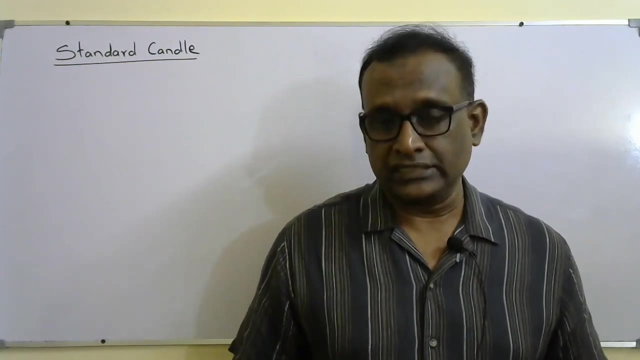 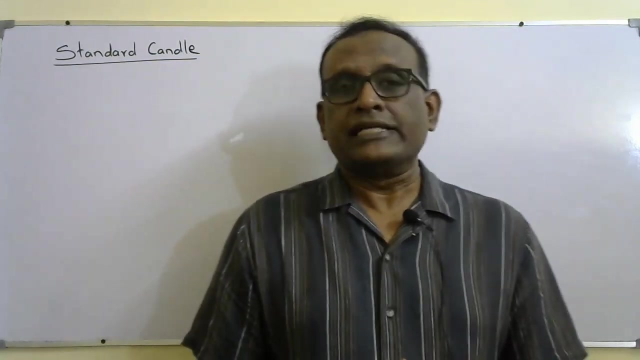 known luminosity, is called standard candle. okay, we can use standard candle in three different ways to find the uh distance of a galaxy or star. the first one, it's like this: uh, we should be able to measure the distance of a nearby star by using a trigonometric parallax method. so we should be 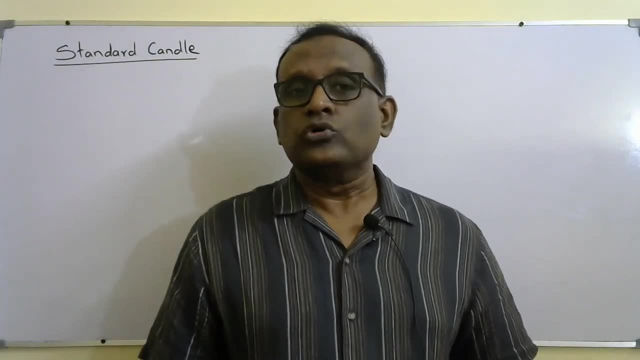 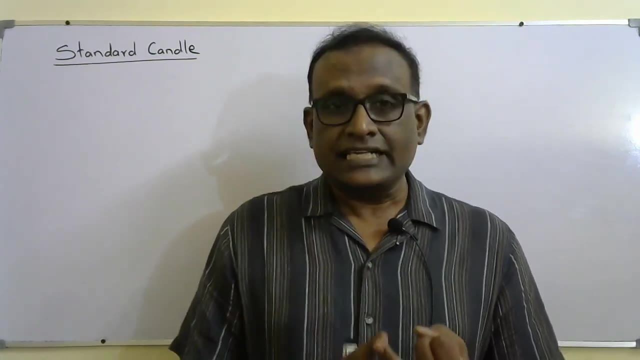 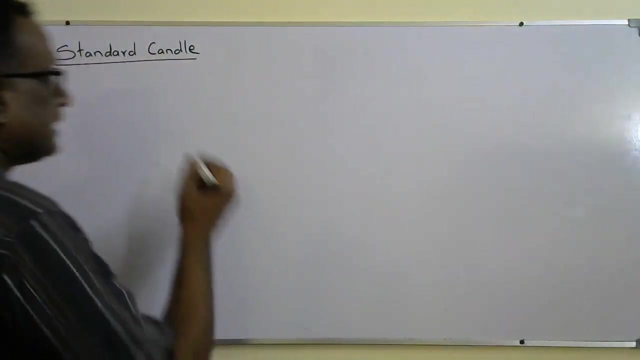 able to measure the distance of nearby star by using trigonometric parallax method. so we know the distance. we should be able to measure the intensity or radiation flux of the radiation from that star, so we will be able to measure the intensity or the radiation flux of it. we are 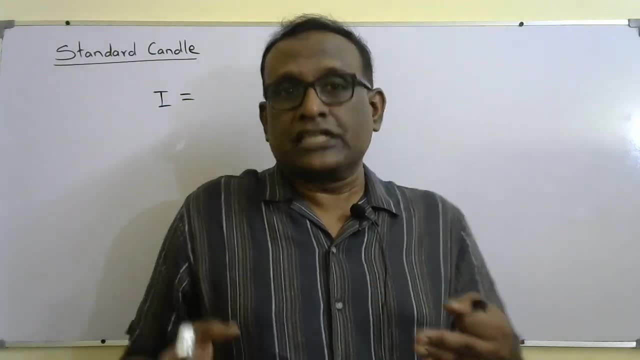 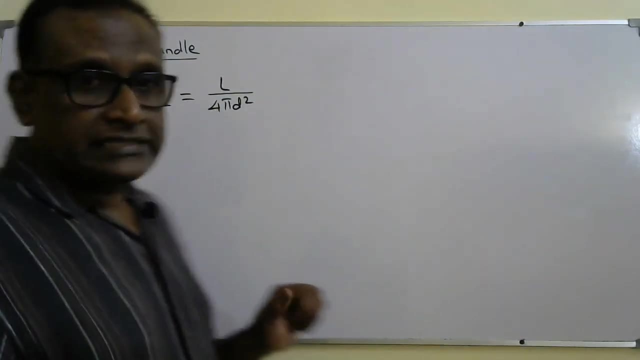 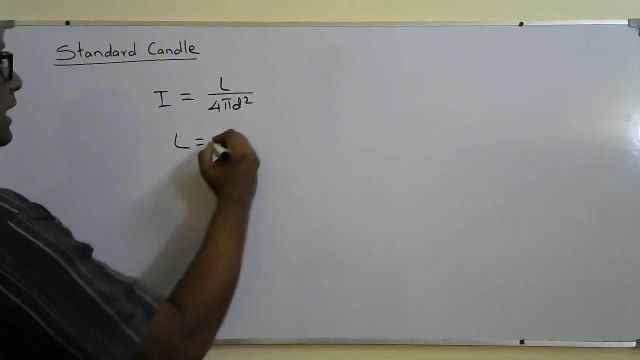 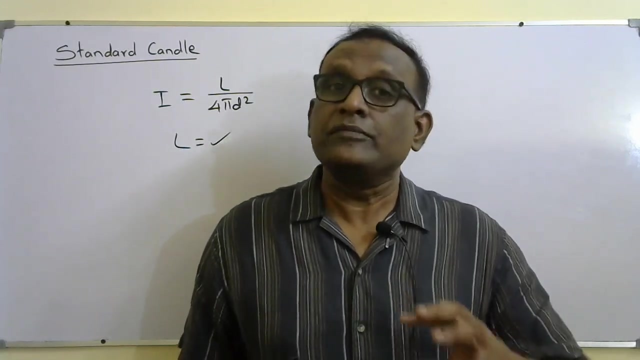 able to measure the distance of that star by using trigonometric parallax. so by using I equal L over 4 pi d squared, we will be able to measure the luminosity of that nearby star. okay, we can find the luminosity without any problem. then we need to measure the distance of. we need to measure the. 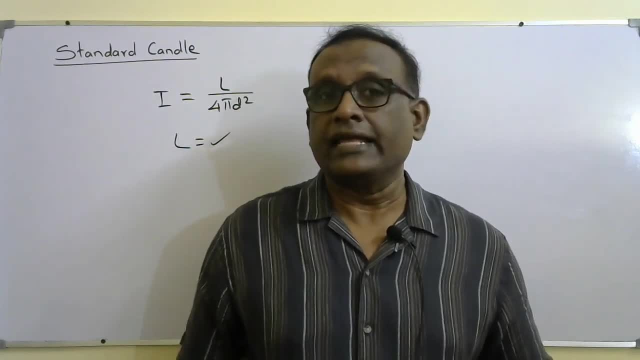 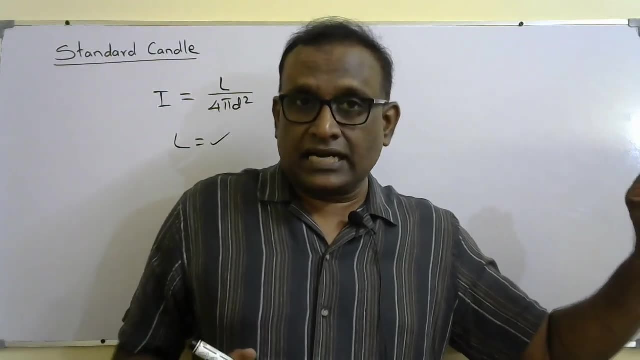 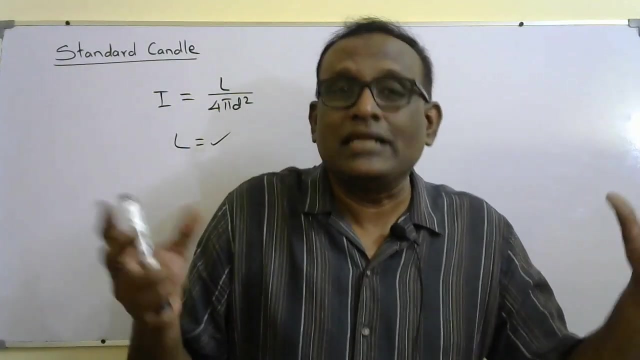 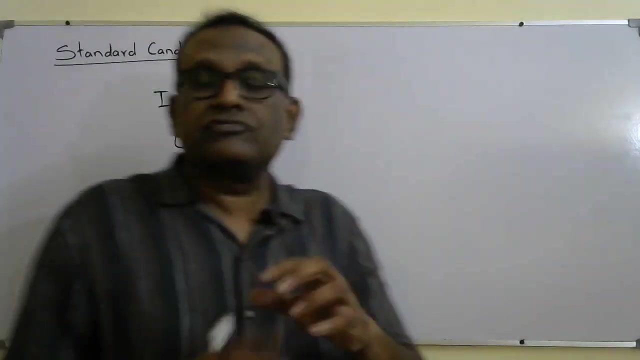 distance of a far distance star. okay, there, what we use? we assume the luminosity of this far distance star is same as the luminosity of nearby star, or we assume both stars are similar stars. by taking that assumption, we use this luminosity for what we measured. for the nearby star, that luminosity is same. 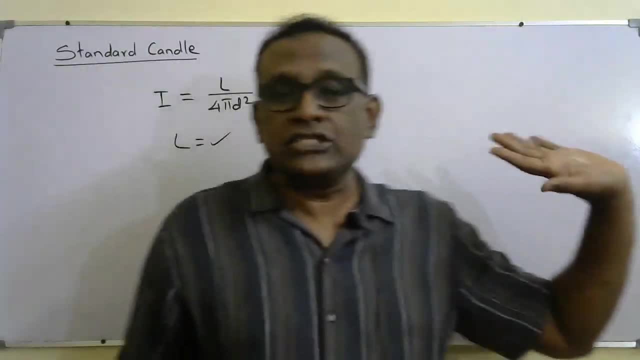 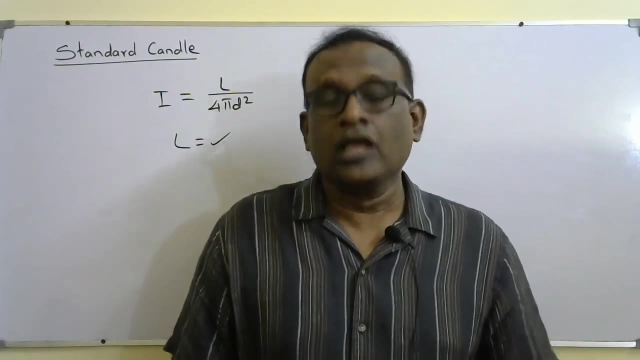 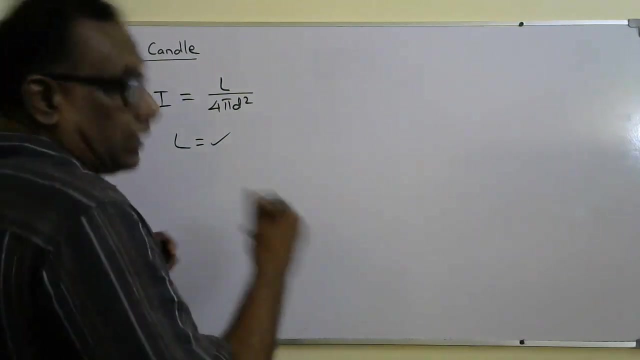 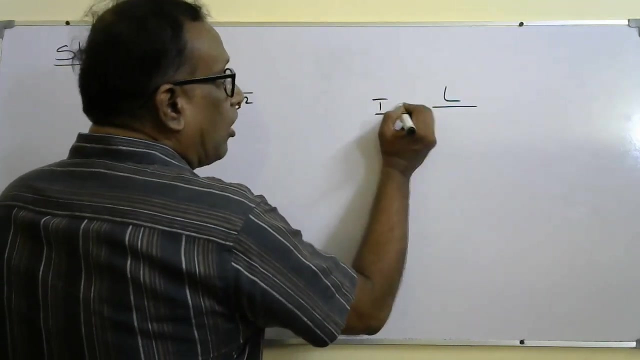 for the far distance star because we assume both stars are similar stars, is an assumption so it might go wrong. if this assumption is wrong, we assume the luminosity of far distance star is same as the luminosity of nearby star. so we know the luminosity of the far distance star. we measure the radiation flux of the star. we know the. 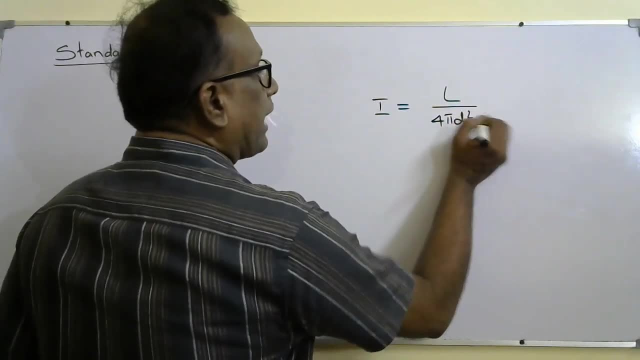 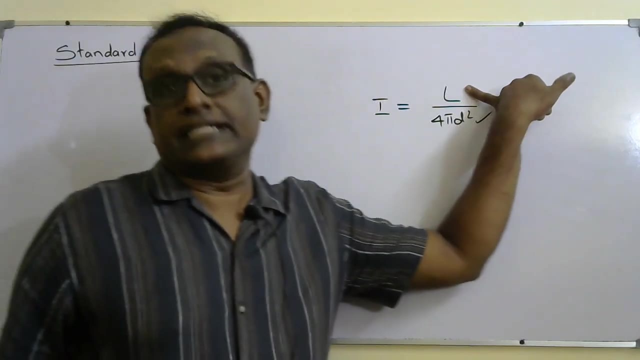 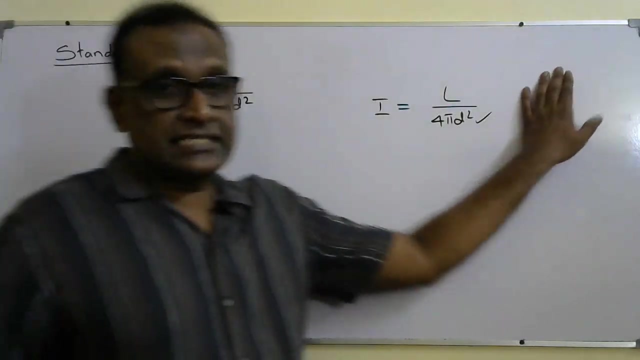 I. so by using 4 pi d squared we measure the dV. so here this is the standard. and because we know the luminosity of far distance star, how do we know we measure the luminosity of the nearby star. this star and far distance star are similar stars, so we don't know the luminosity of 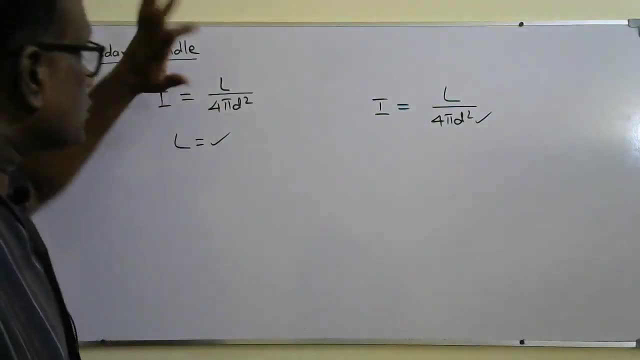 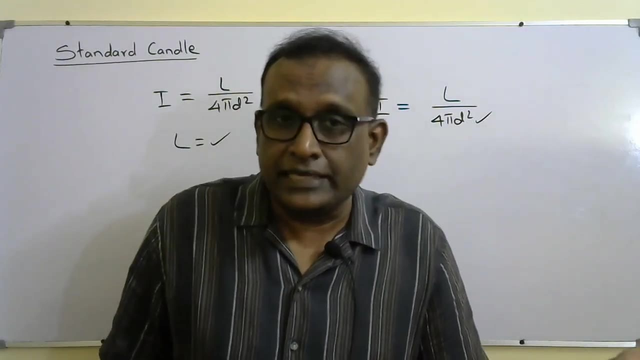 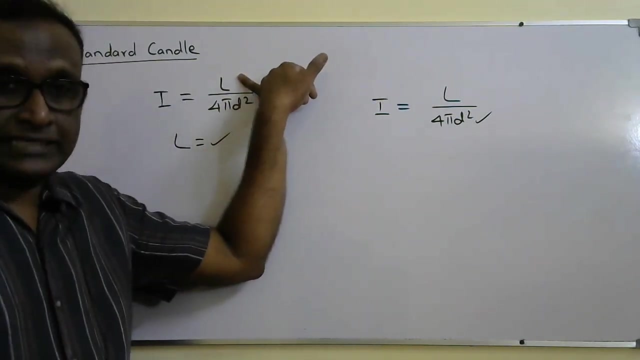 far distance star initially. so we measure the luminosity of nearby star. how do we measure? we know the distance. we can measure the distance of nearby star by using trigonometric parallax, hypnometric parallax D. we measured I, we measured L, we calculated for the nearby star. 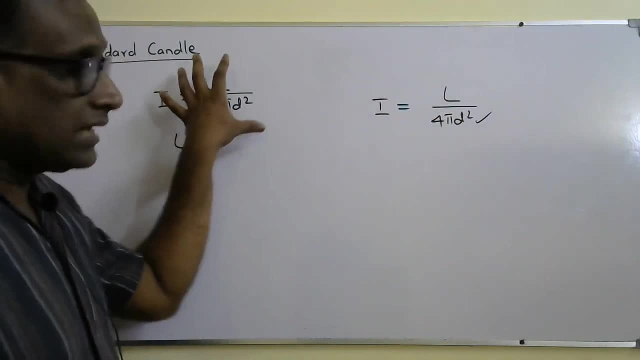 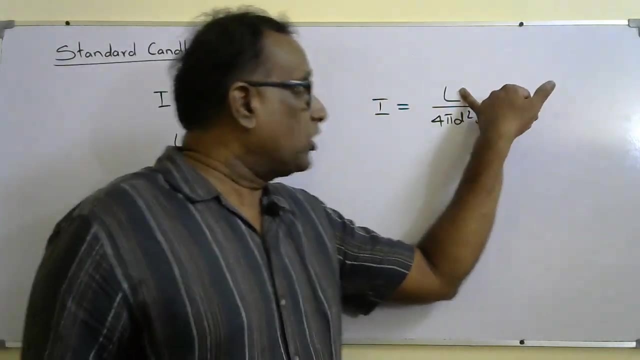 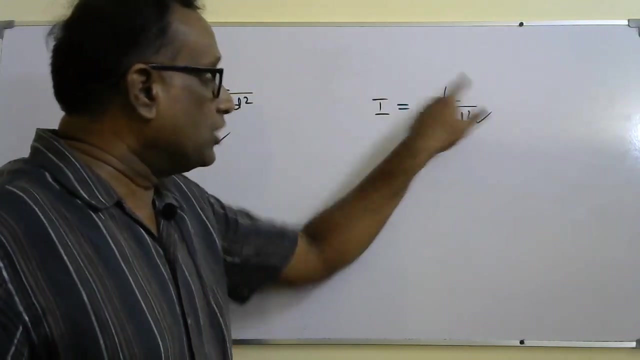 Then we assume the far distant star and the nearby star are similar stars. Our aim is to find the distance of far distant star. So we know the luminosities are similar. We measure the intensity. We know the luminosities are similar. So I and L are known. We find that D. But this way when 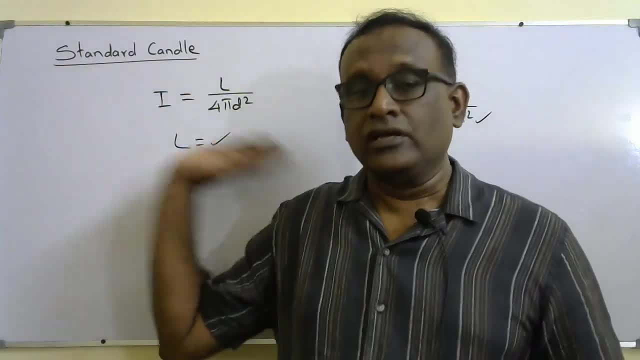 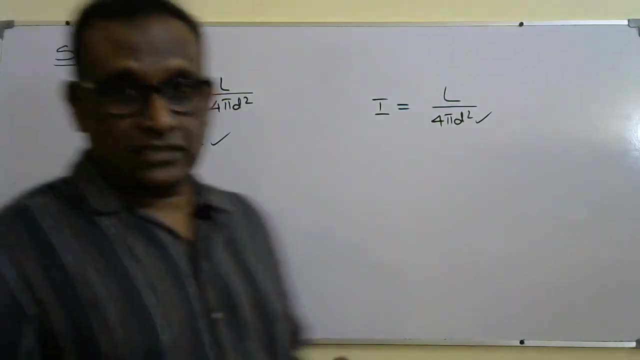 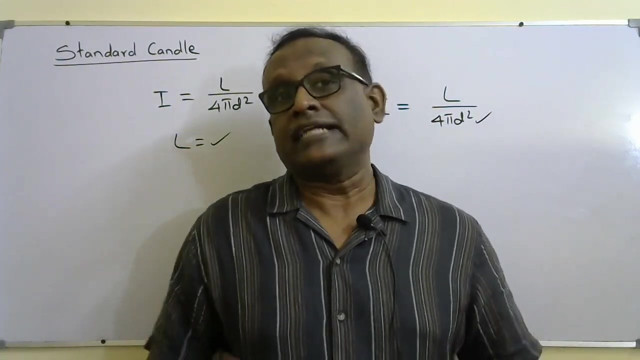 we are using standard candle method in this type of measurements. we make an assumption, that is, the far distant star and nearby star. we consider two different stars. They are similar. We assume that their luminosities are same. We assume that if that assumption is wrong, then the measurement 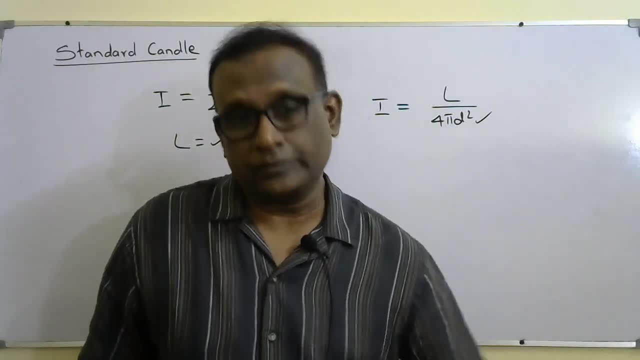 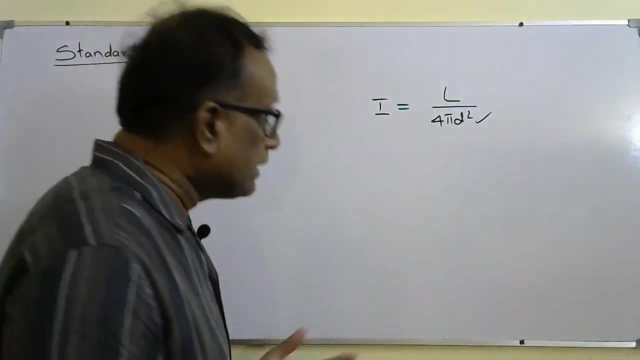 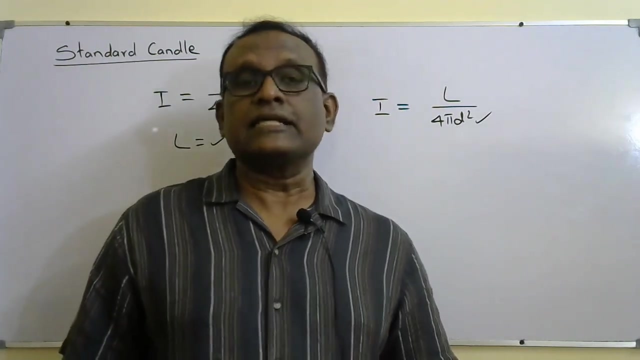 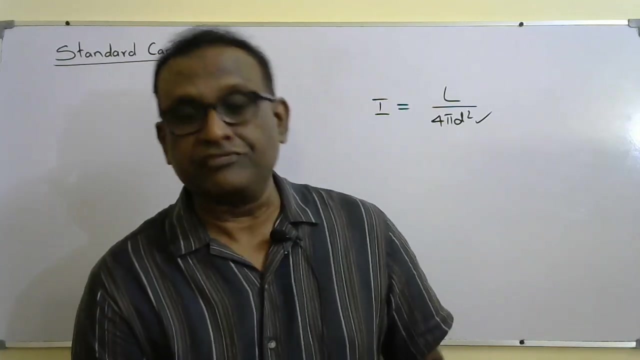 what we do in distance will go wrong. So this is not a good method, But this method also introduced in your study In your syllabus. they are using this method also in your syllabus. We take it as a standard candle, one method. The second method is we use Cepheid variable as a standard candle. Okay, what is Cepheid? 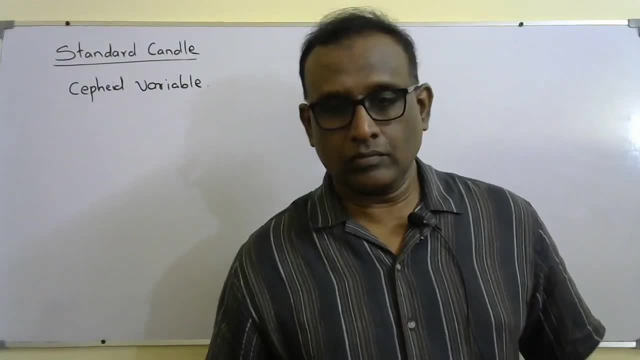 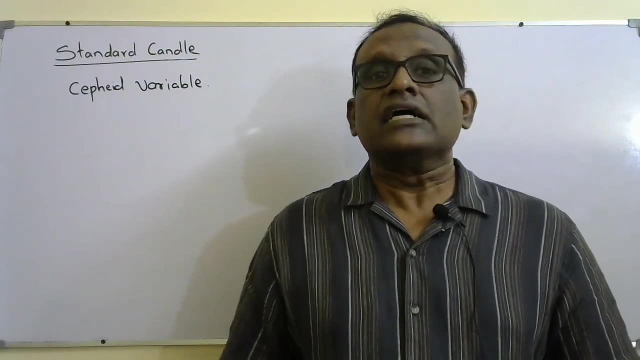 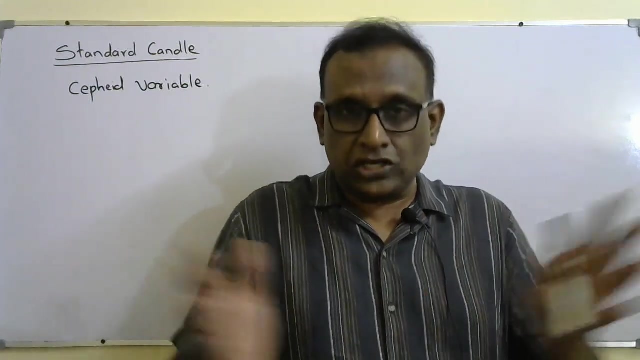 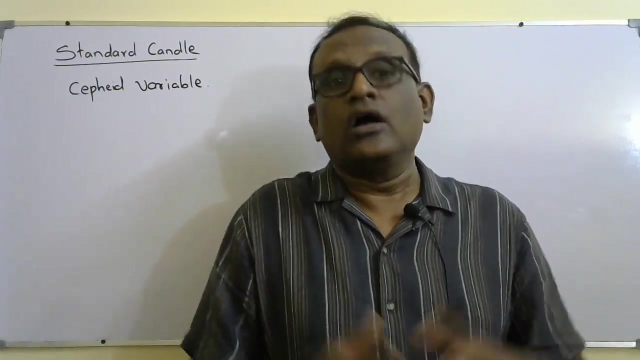 variable. Okay, what is Cepheid variable? So Cepheid variable is a star in which the luminosity varies periodically, Because that star expands and contracts periodically due to variation in its pressure, So the surface area changes with same amount of time intervals, So the luminosity will vary. like this, If you. 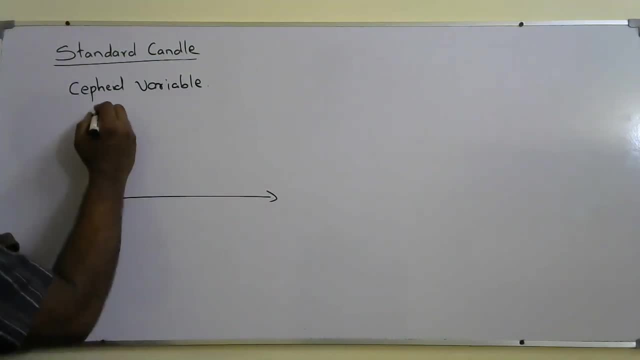 see the luminosity of the star, or Cepheid variable. with time there could be variations like this: a proper time interval: There will be variations like this. So Cepheid variable is a star in which different Cepheid variation, Different Cepheid variables have. 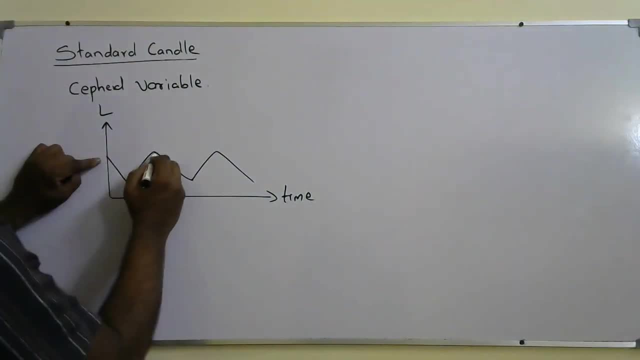 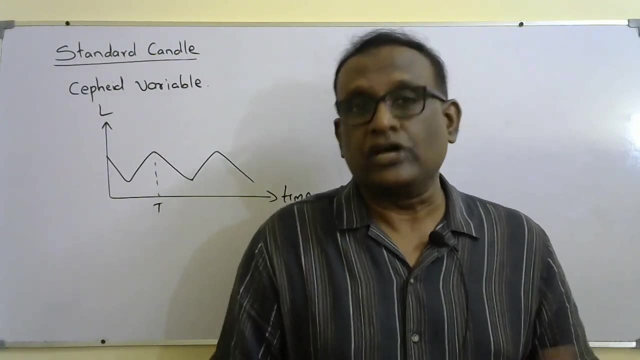 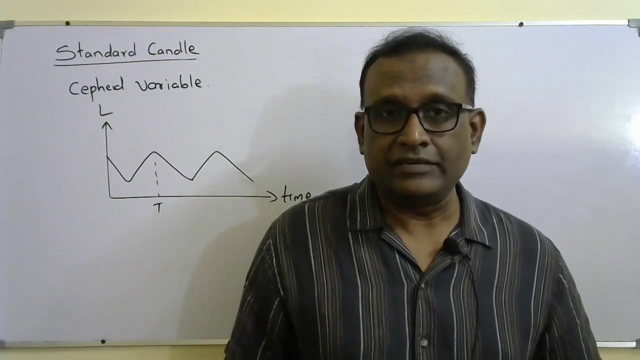 different time period. So this is the one time period. This is the time period. So for aimthere Cepheid variables, the time period of expansion and contraction could be different. Okay, So there are many Cepheid variables closer to us and we could measure. 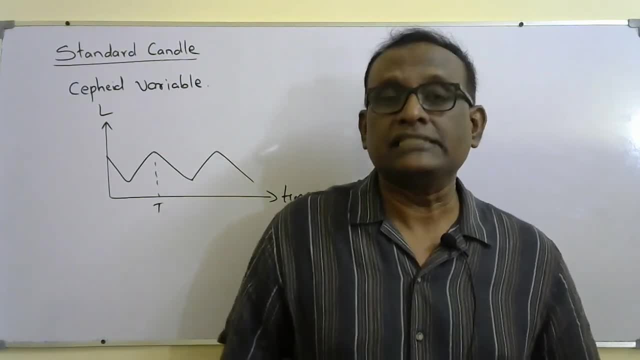 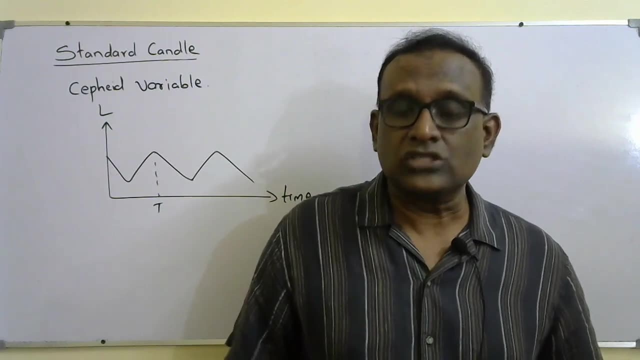 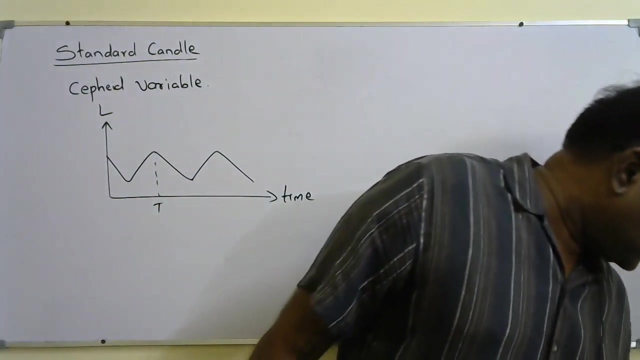 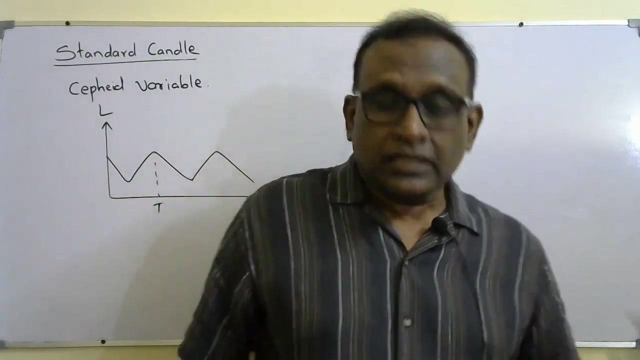 their distances very accurately, So we can measure their average luminosity accurately. so there are a lot of severe variables closer to us. we are able to measure their average luminosity because luminosity is varying with time, so their average luminosity and their time period of expansion contraction accurately we can measure then if we plot a graph of their 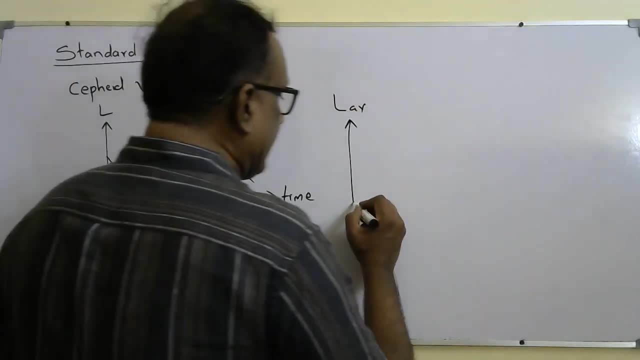 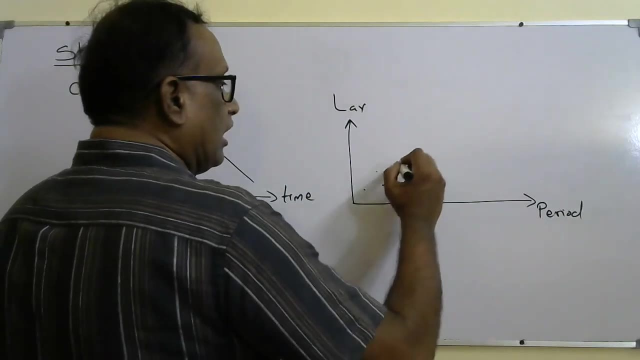 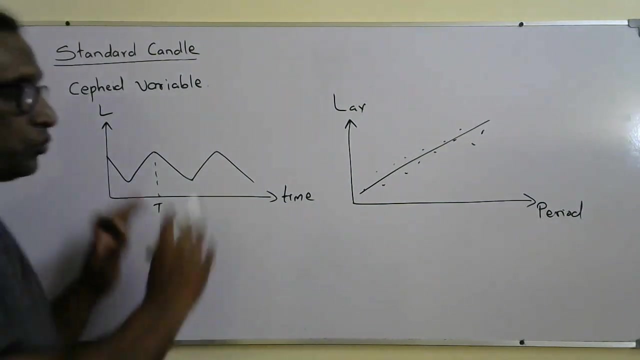 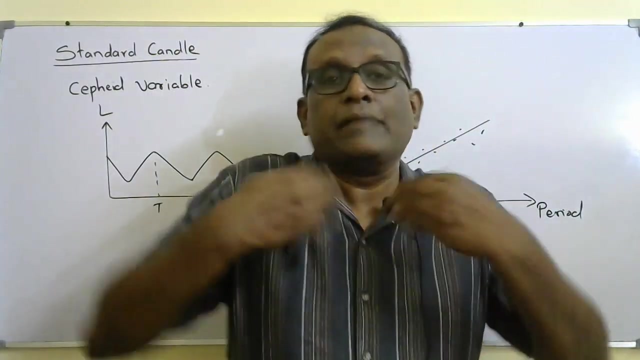 average luminosity against time period of expansion contraction. the basic line will be a straight line. the basic line will be a straight line. okay, so we got these information by using safe heat variables. those are closer to us. we are able to measure their luminosity by using: 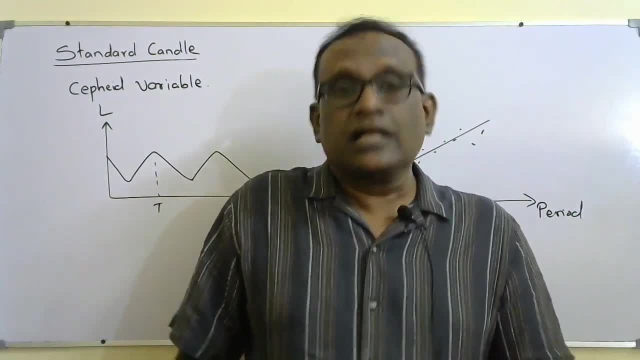 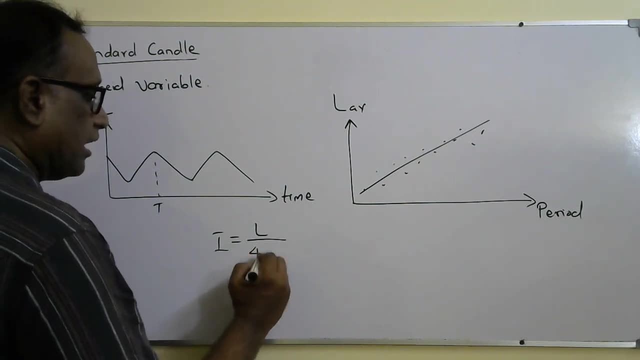 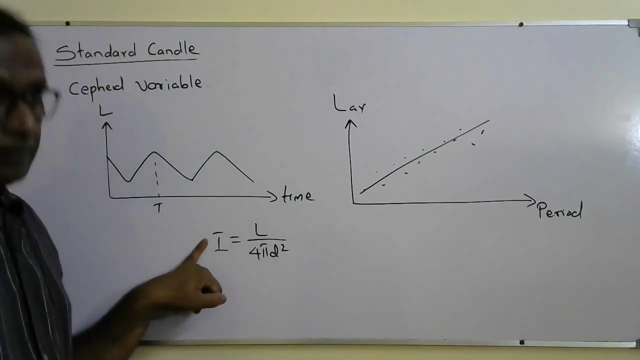 cryptometric parallax method, the distance could be measured. we can measure their intensity by using i equal L over 4 pi D squared. we can measure their luminosity or average luminosity. we can measure their intensity or average intensity. those are closer to us. we can measure their distances by using cryptometric parallax method, so we can find. 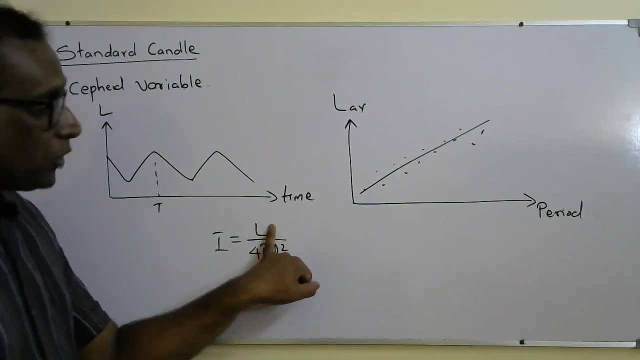 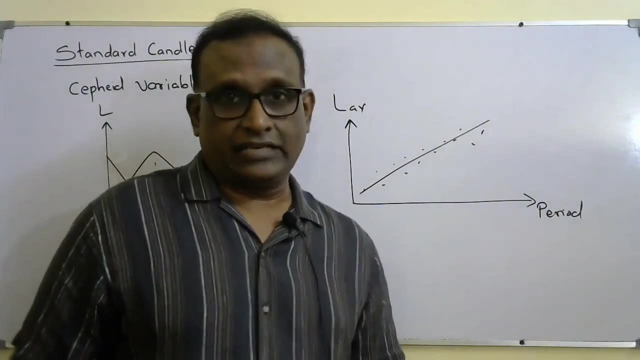 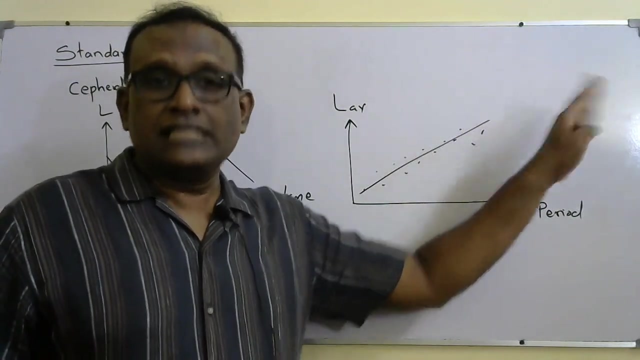 their average luminosity and if we plot a graph of average luminosity against period of expansion contraction interaction for different Cepheid variables, the best fit line will be a straight line. We got this data by using several Cepheid variables closer to us. 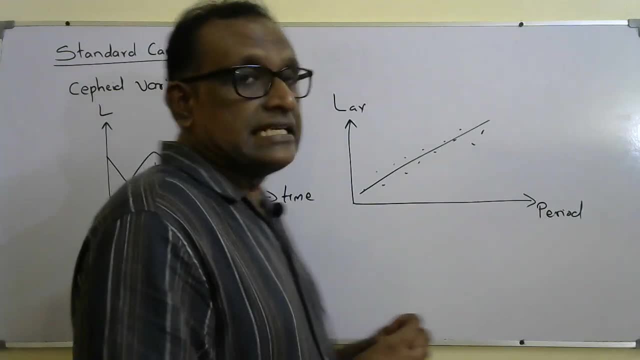 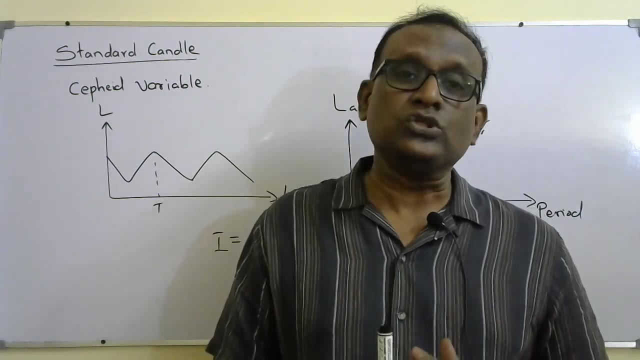 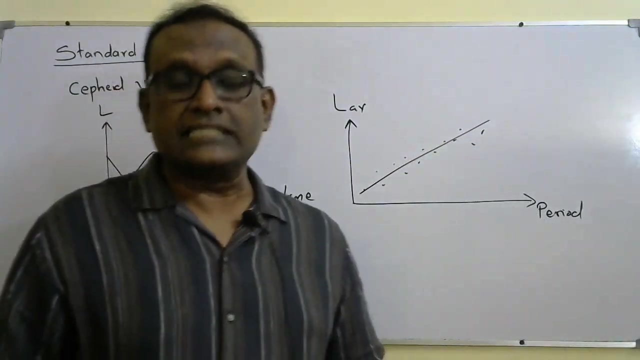 Right now we can use this information to find the distance of a galaxy. Mostly this method, the Cepheid variable as a standard candle method, is used to measure the distance of a galaxy which is far away from us. Okay, so how to measure the distance of a far away galaxy? We should search and find a. 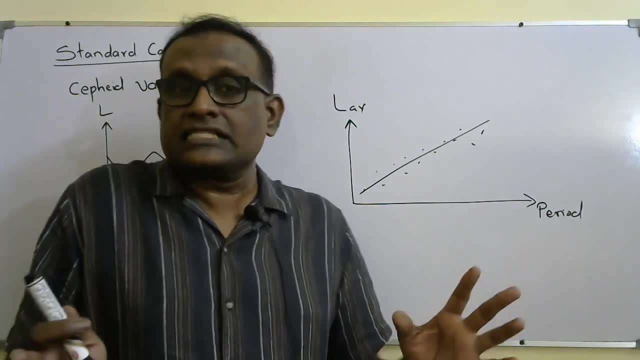 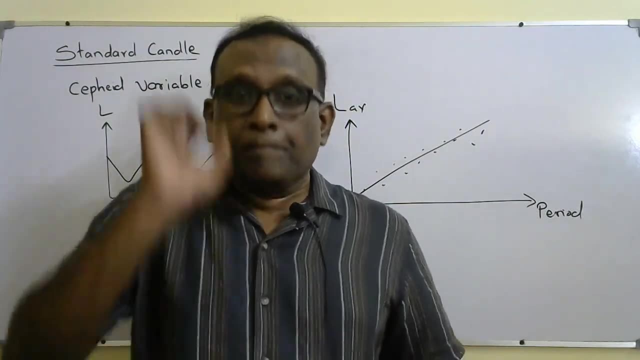 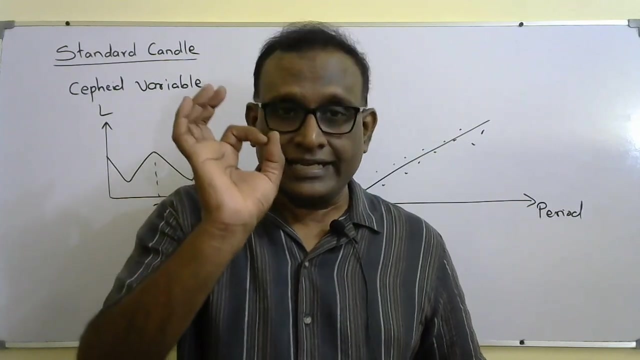 Cepheid variable in that galaxy. That galaxy might have several sephids variables. pick one sephid variable from that galaxy. Measure its period of expansion, contraction. When you observe the intensity and how it varies, you will see the intensity will vary periodically. from that you can find. 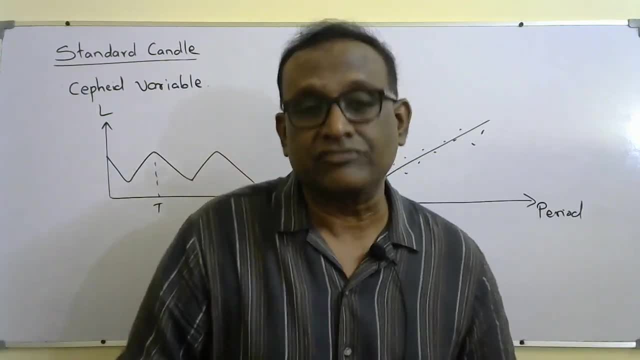 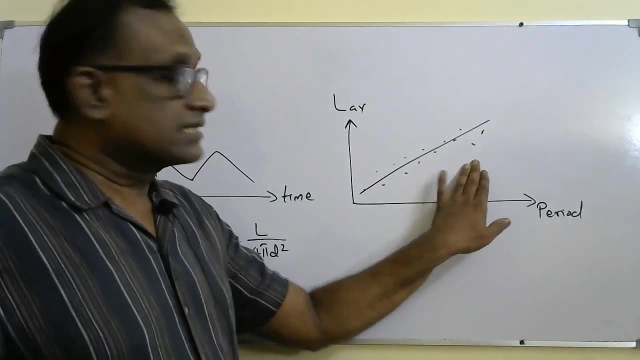 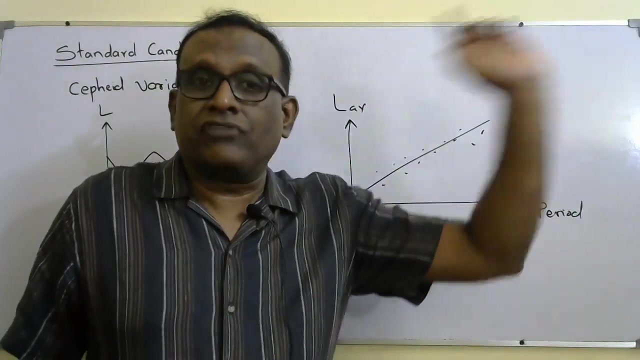 the period of expansion and contraction of that Cepheid variable in a far-distance galaxy. You know the period of expansion and contraction. Use this graph By using this graph, since you know the period of expansion and contraction of that Cepheid variable in a far-distance galaxy. 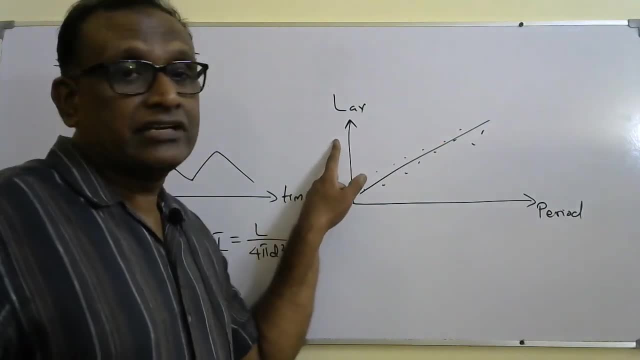 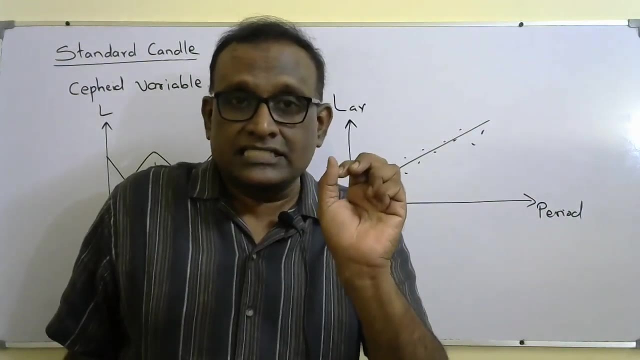 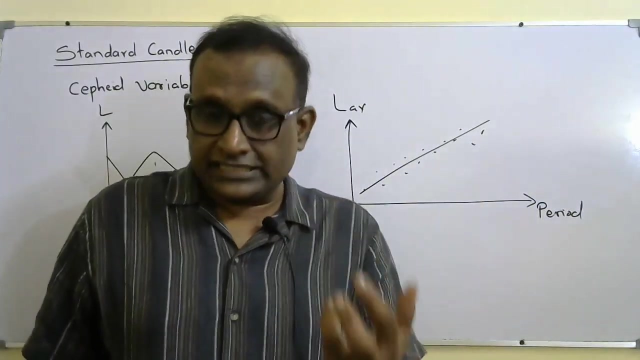 use this graph. From this graph, find its average luminosity. Now you know the average luminosity of that specific Cepheid variable in a far-distance galaxy. You know the average luminosity, Measure the average radiation flux or intensity of the radiation. 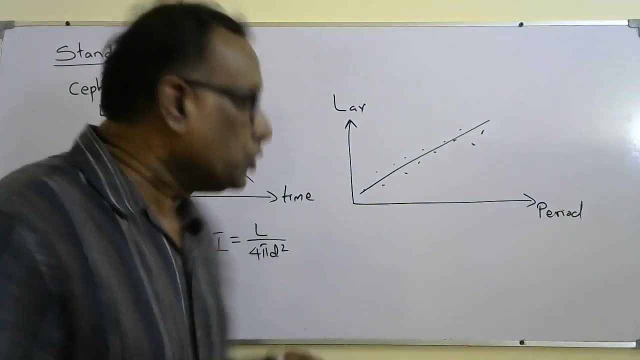 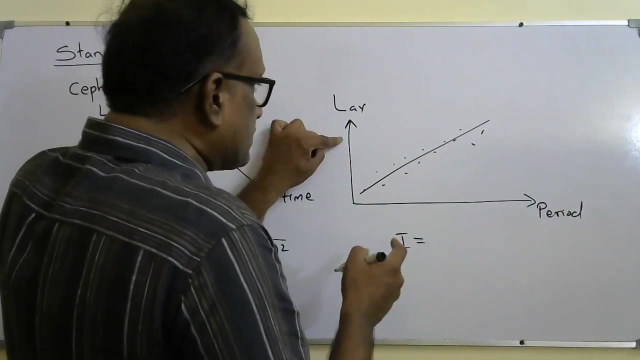 from that specific Cepheid variable. So you know the intensity. You measured it from the Cepheid variable in a far-distance galaxy. You know the average luminosity. You found it by using this graph. You know the average luminosity. 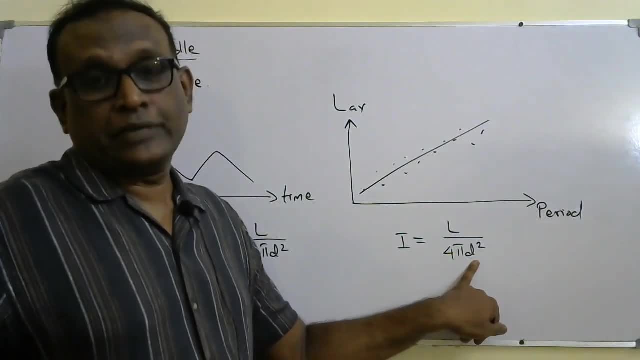 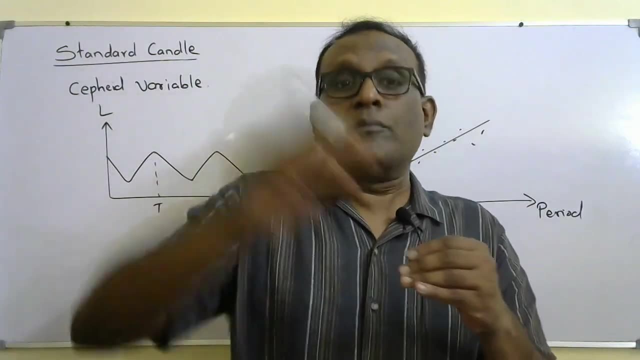 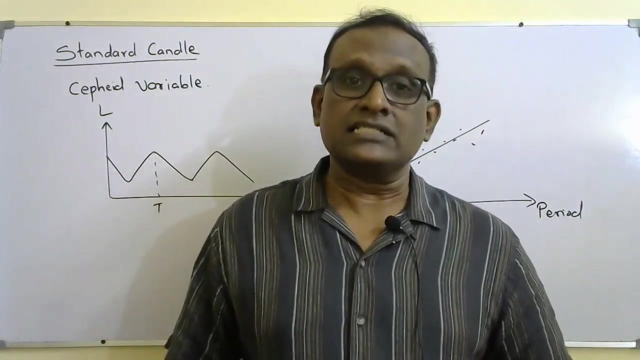 By using this distance, find the distance of that particular Cepheid variable in that galaxy, Like that in that galaxy. take the distance or measure the distance of different Cepheid variables in that galaxy and find the average distance of the galaxy. 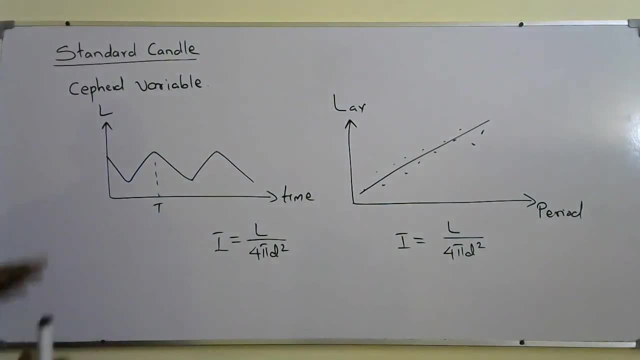 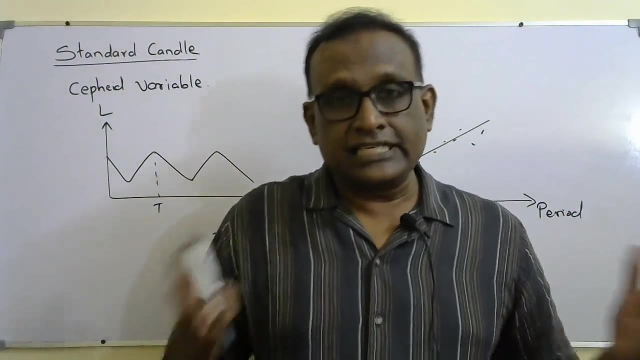 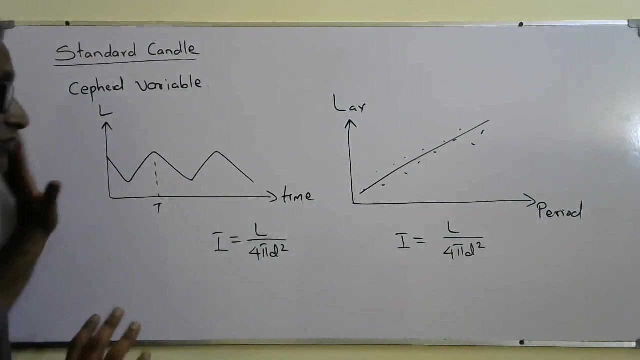 I hope you understood Again. I will quickly repeat again. Cepheid variable means a star that has periodic expansion and contraction due to periodic variation in its pressure. So luminosity will vary periodically. Different stars have different period of expansion and contraction. 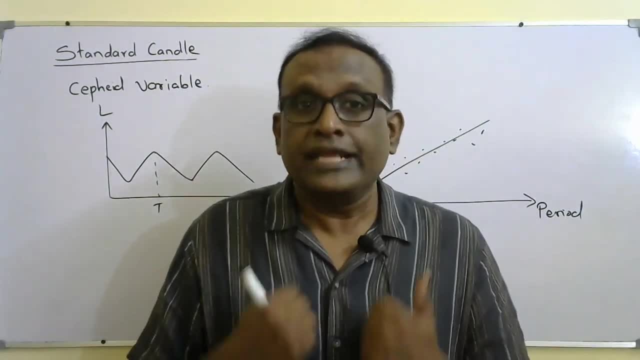 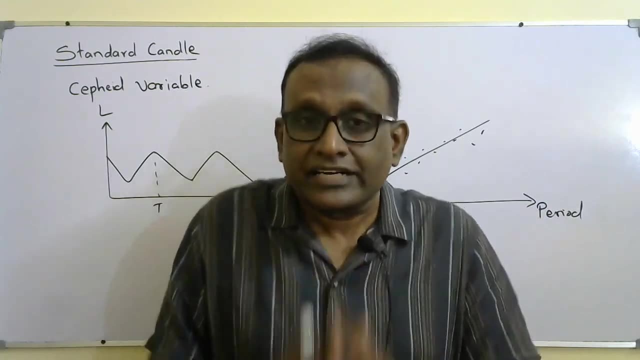 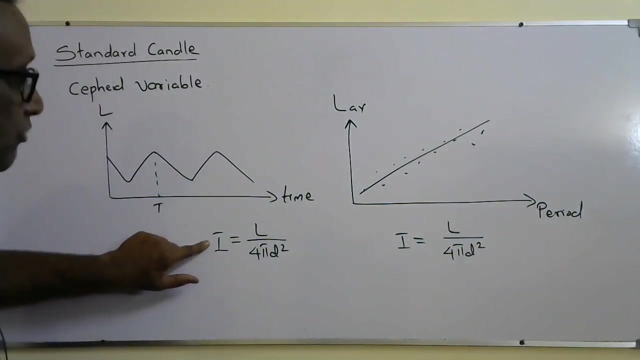 There are many Cepheid variables closer to us. We can measure their distance by using trigonometric parallax without any problem. We can measure their average intensity or average radiation flux, Since we are able to measure their average intensity and we are able 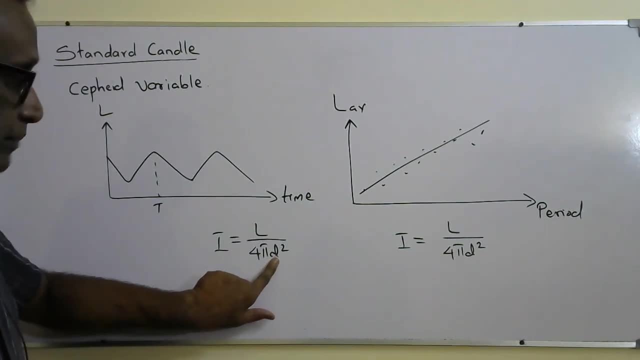 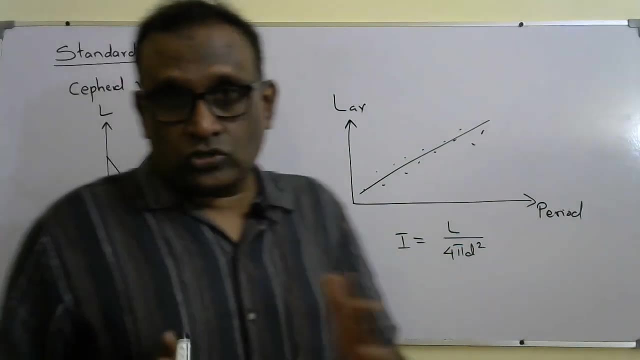 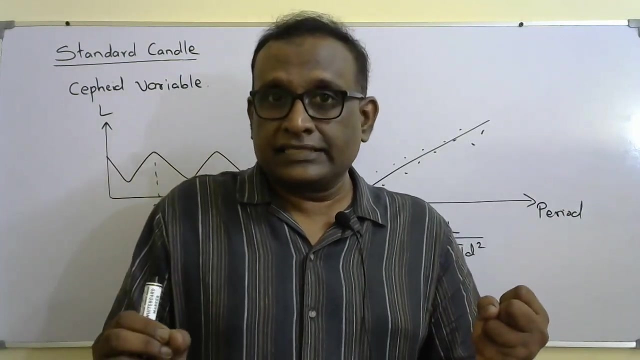 to measure their distances. by using trigonometric parallax method, we are able to measure their average luminosity. There are several Cepheid variables closer to us. I told So if we take average luminosity and the relevant period of expansion contraction for different 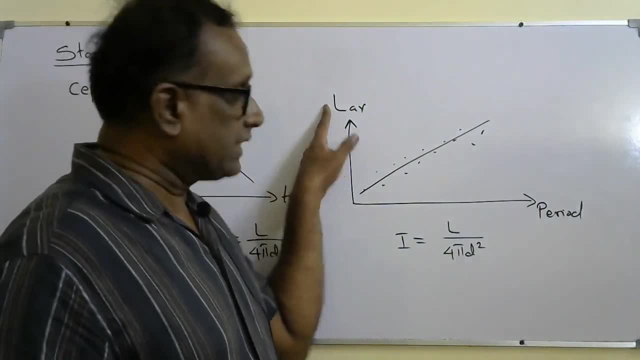 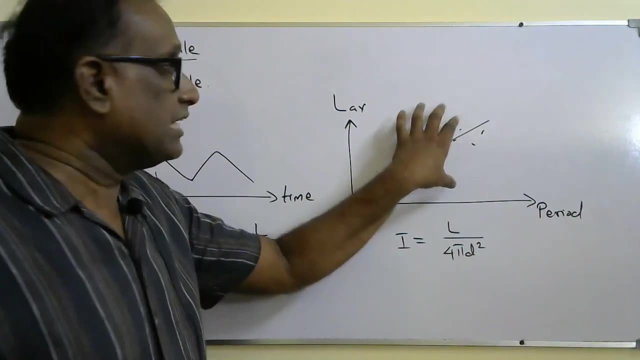 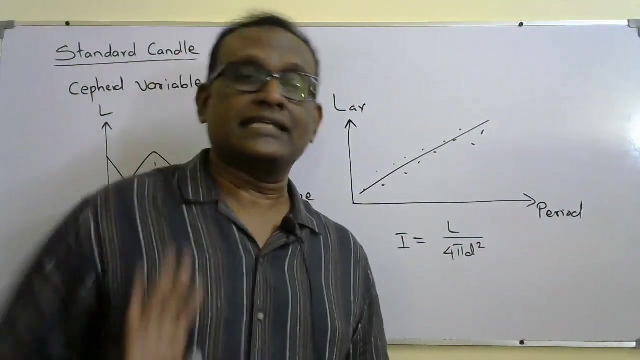 Cepheid variables and if we plot a graph of average luminosity against period of expansion contraction, the best fit line will be a straight line. We are going to use this information to find the luminosity of a far-distance Cepheid variable in another galaxy. 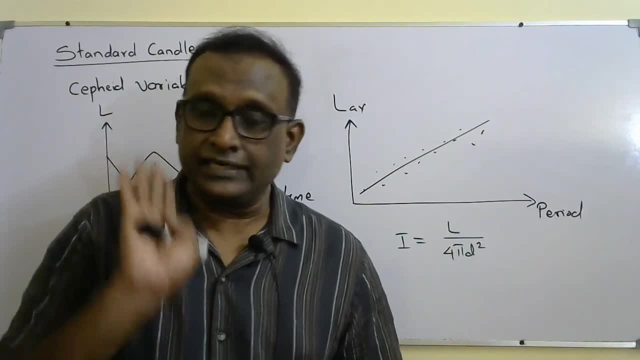 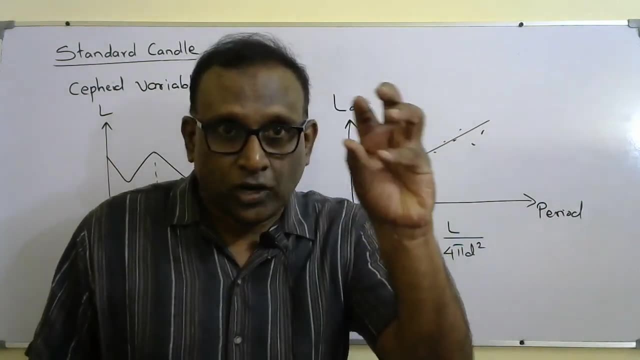 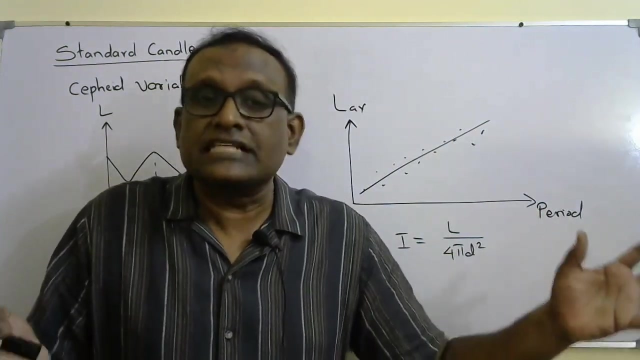 Our aim is to find the distance of a far-distance galaxy. To find the distance, we should search and spot a Cepheid variable in that far-distance galaxy. There could be many Cepheid variables. Take one particular Cepheid variable. 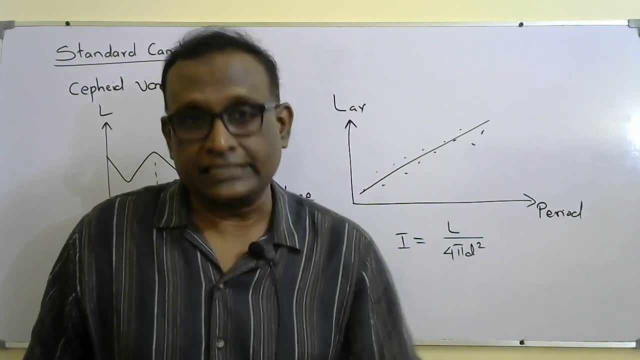 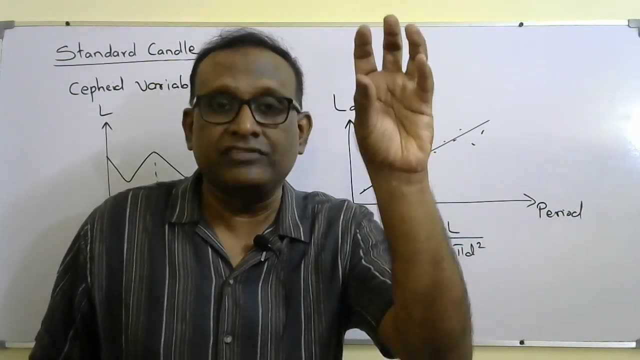 Find out its period of expansion in contraction? How can we find its period of expansion? contraction: How can we find its period of expansion? contraction: find the period of expansion and contraction? Receive the radiation continuously from that Saphir variable and you know that intensity or radiation flux from that specific Saphir. 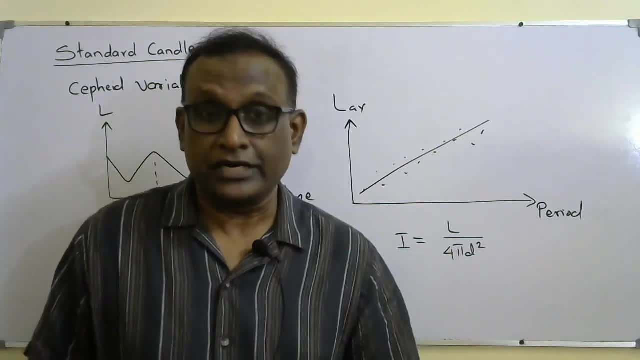 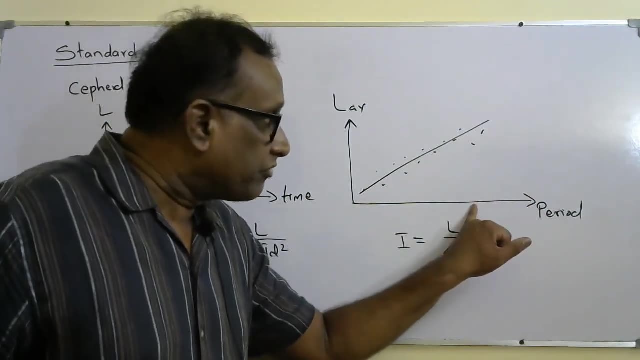 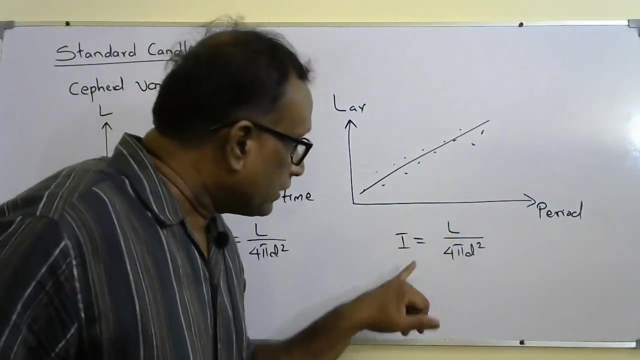 variable. have a periodic variation From that. find the period of expansion and contraction of the Saphir variable. Use this graph. By using this graph you can find the average luminosity of that Saphir variable in far-distance galaxy. Okay, you know the average luminosity. 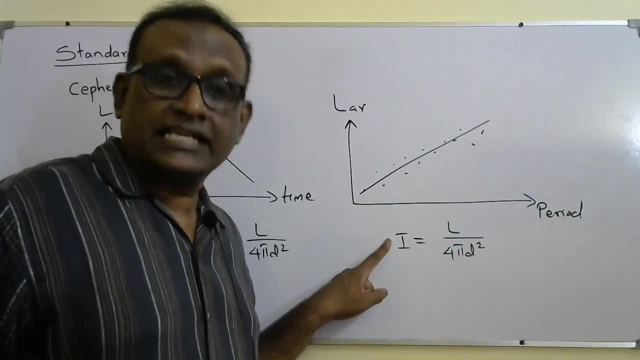 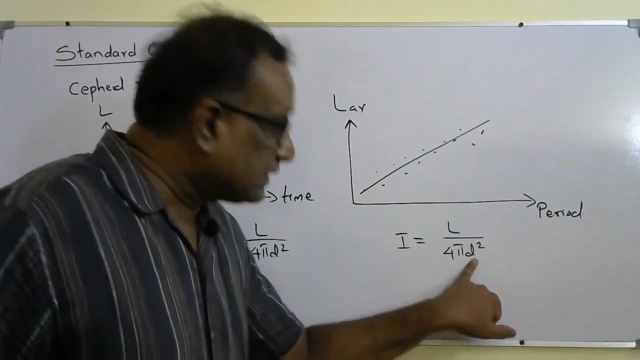 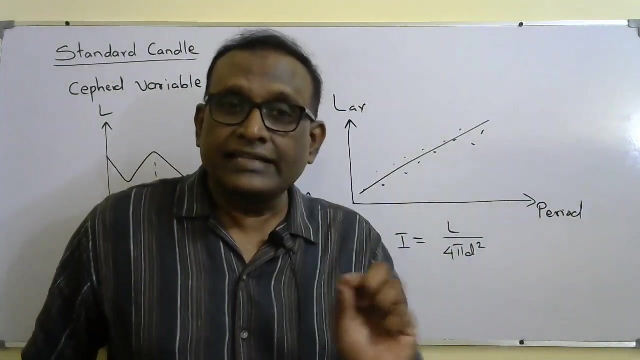 You can measure the average intensity of the radiation from that specific Saphir variable. So I you know, L you know. By using this equation, find the distance of that Saphir variable in the far-distance galaxy. Same way, find the distance of different Saphir variables. 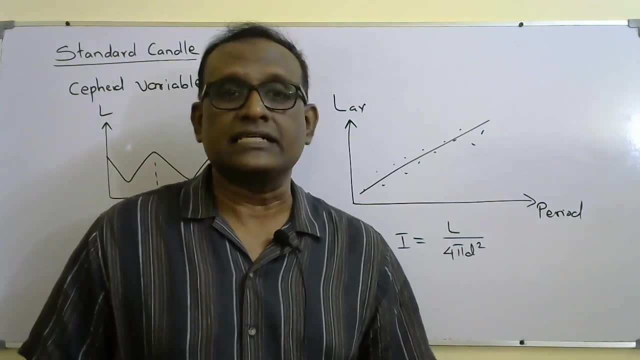 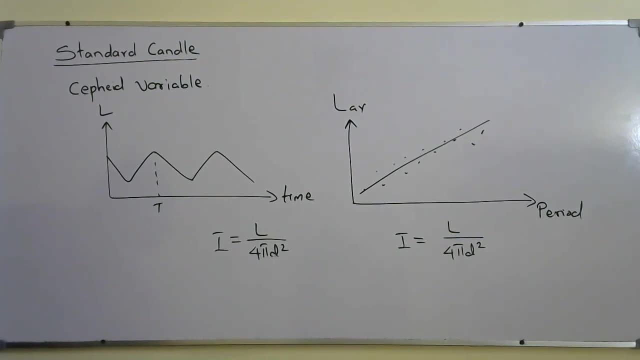 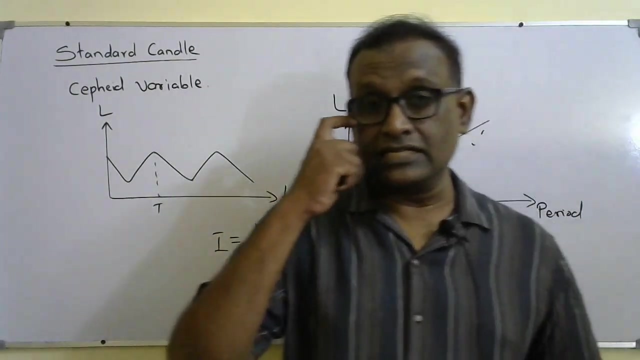 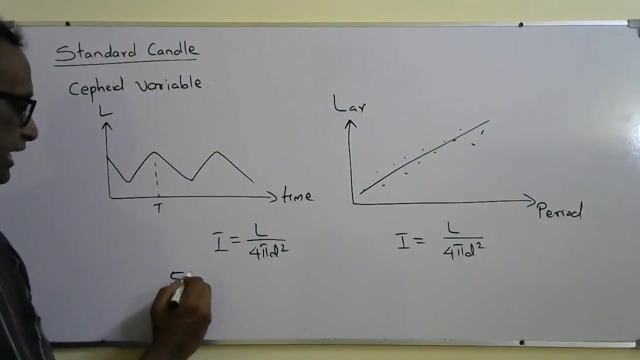 in the same galaxy? Okay. Find the average distance of the galaxy from Earth. Okay, so this method also has limitations. using Saphir variable as a standard candle, This method can use up to maximum distance of 50 mega parsec. Okay. so if the distance becomes more than this, the problem is: I define. 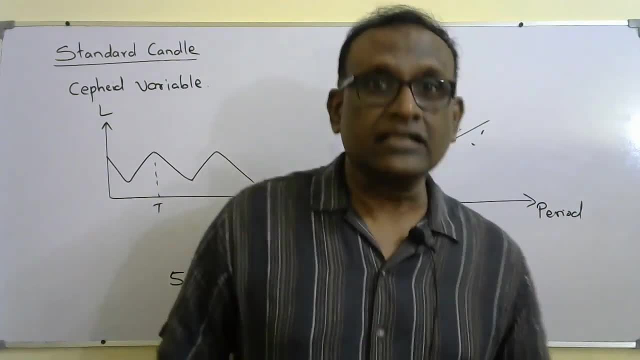 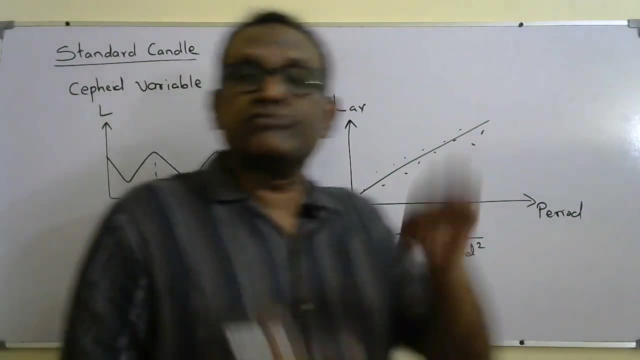 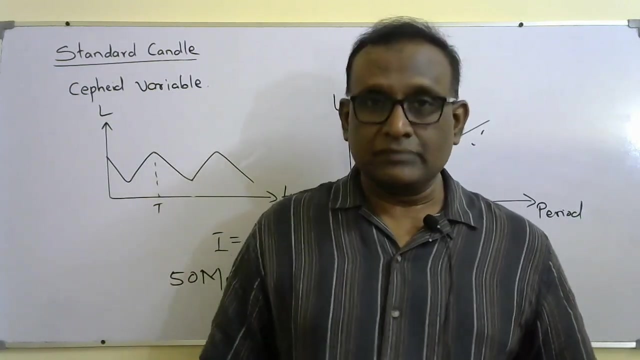 the, or measuring the variation in the maximum and minimum intensity or maximum minimum luminosity. I define the difference between maximum and minimum intensity or luminosity of the Saphir variable will be difficult by using the measuring instrument, So we won't be able to find the. 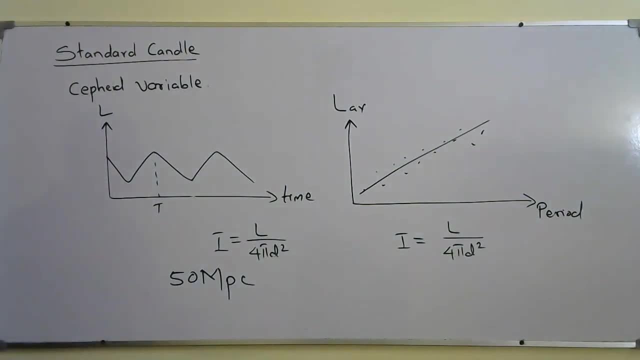 period of the Saphir variable. So that's a drawback or the limitation of this method. So we can measure up to A distance of 50 mega parsec using Saphir variable as a standard candle. Okay, so if the distance of a galaxy? now we don't need to measure the distance of a particular. 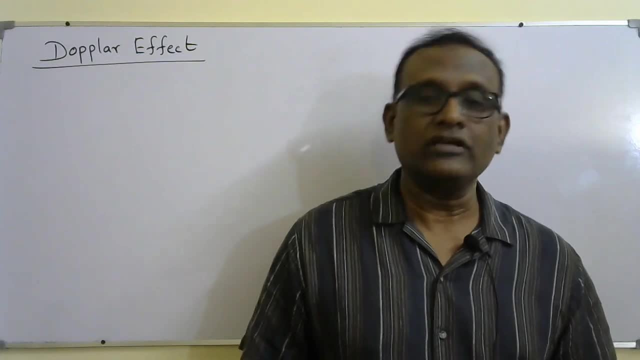 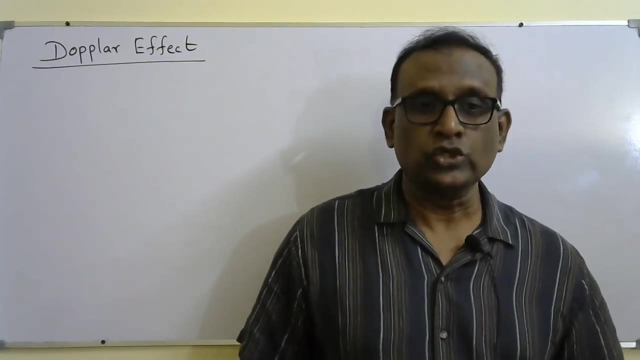 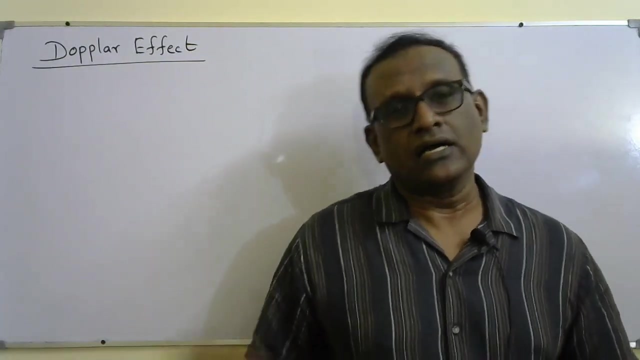 star, We measure the distance of a galaxy. now, If the distance of a galaxy is more than 50 mega parsec, we follow another method in which we use Doppler effect. Doppler effect is also nothing related to cosmology. Okay, Something related to waves. Some of the syllabus they teach Doppler effect with wave theory. 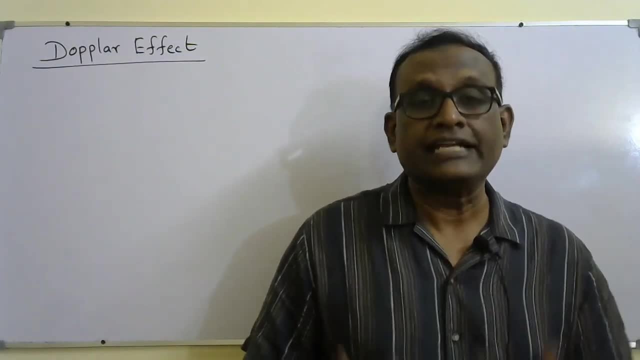 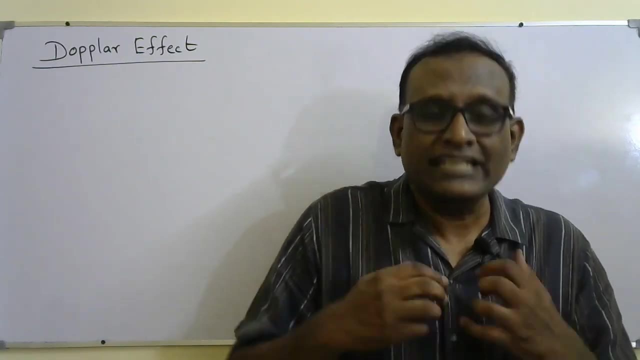 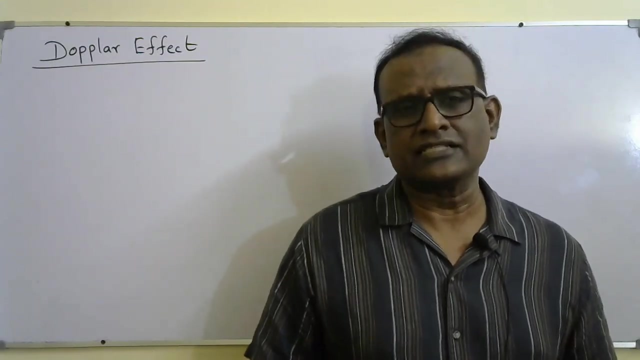 Okay, What is? Doppler effect means when there is relative motion between the source and observer, the wavelength of frequency measured by the observer will be different compared to actual wavelength or actual frequency emitted from the source. For example, you would have noticed that when ambulance approaches you, when the ambulance moves towards you are stationary and when the ambulance approaches you, you will hear the siren with higher frequency. When the ambulance moves away from you, you will hear the siren- the sound of the siren- with lower frequency. So that is due to relative motion. 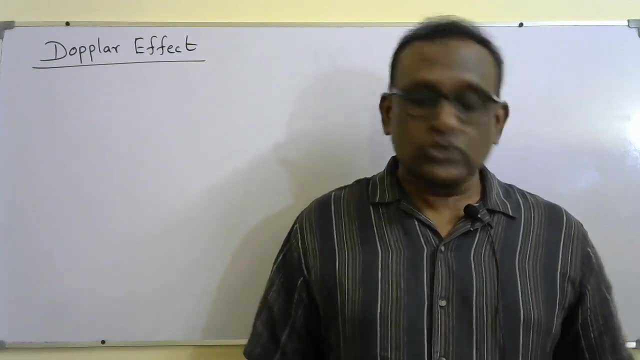 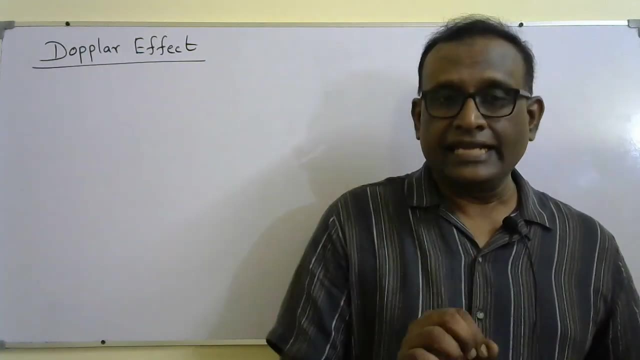 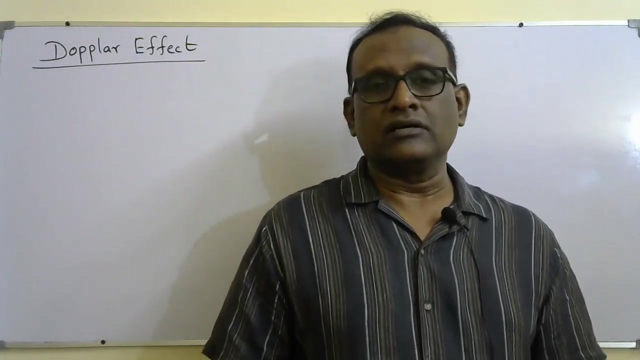 between you and the ambulance. So I did a complete lesson on Doppler effect. I'll give you the link for that. It's a separate video. I'll give you the link for the Doppler effect fully. I did a complete video in the description. 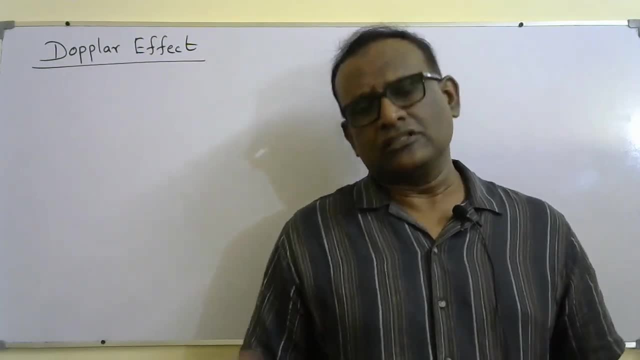 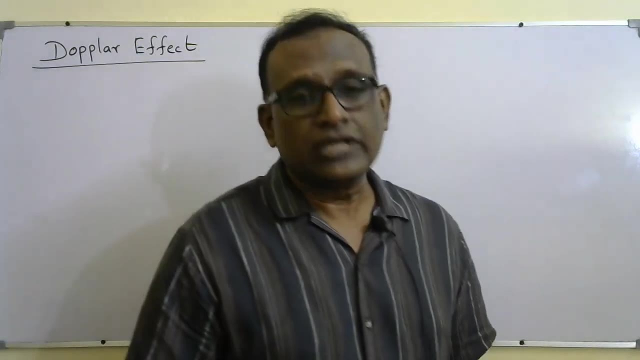 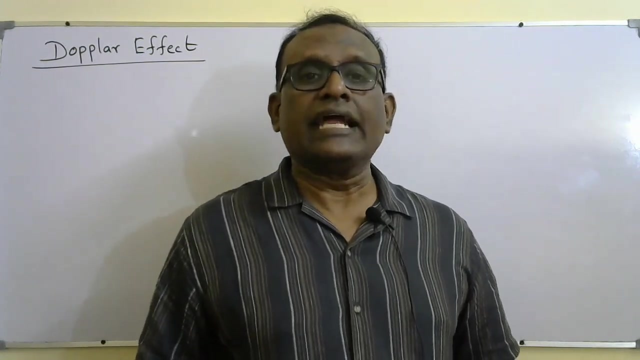 of this video. I'll give the link for that Those who are interested. you can watch that. Okay, So Doppler effect- what is that? Several times they ask that. So in case, if they ask what is Doppler effect means you can say change in wavelength and frequency due to relative. 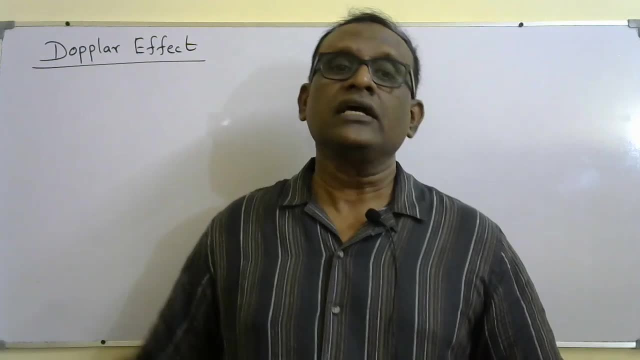 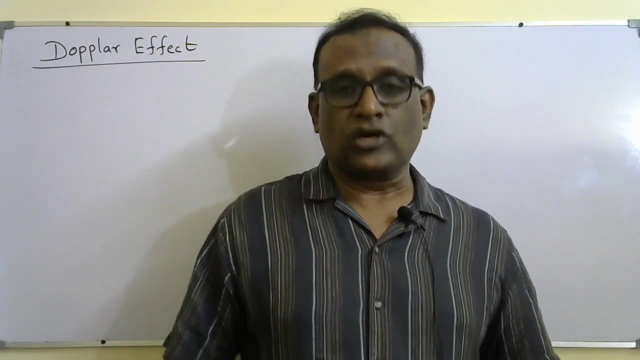 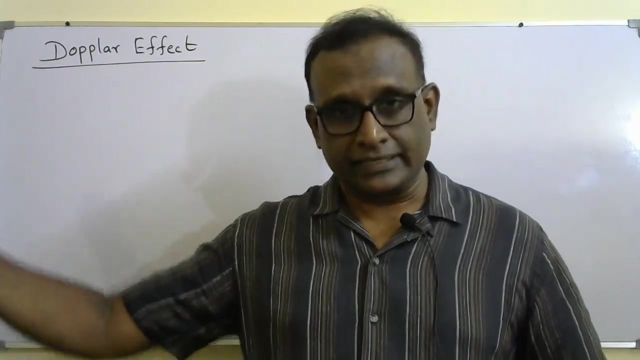 motion between the source and observer is called Doppler effect, So I call Doppler effect. when the source is moving towards a stationary observer, the wavelength measured by the observer will be smaller than the actual wavelength emitted by the source and the frequency measured by the observer will be higher than the actual. 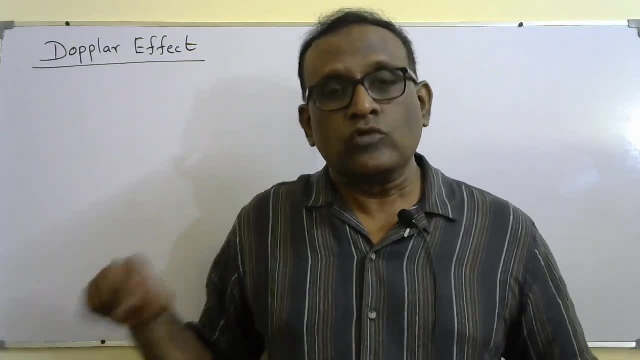 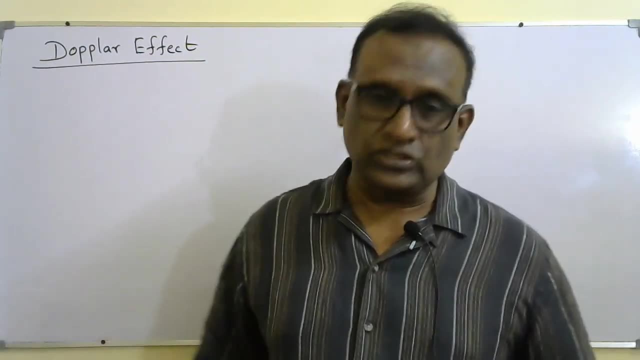 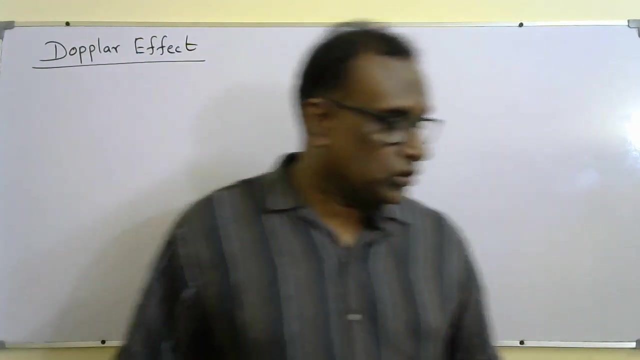 frequency from the source. Same way, if the source moves away from a stationary observer, wavelength measured by the observer will have a larger value than the actual value and the frequency measured by the observer will have a smaller value than the actual value. So in your syllabus we have Doppler effect equation only for electromagnetic waves, Actual. 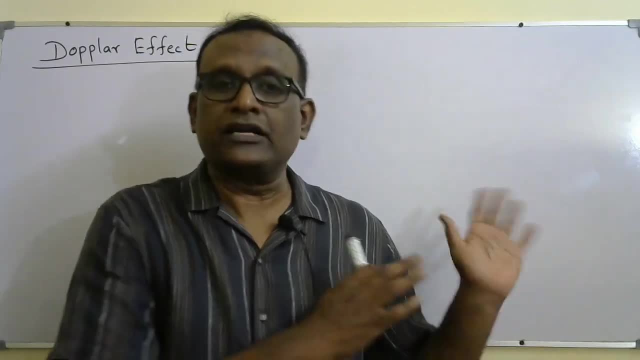 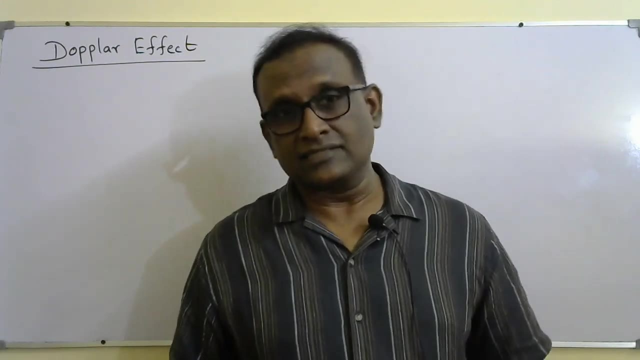 Doppler effect equation related to sound is different compared to what I'm going to show the equation now. So this equation is valid only for electromagnetic radiations- right Light and electromagnetic radiation. So the Doppler effect equation in your syllabus we use is delta, f ohms. 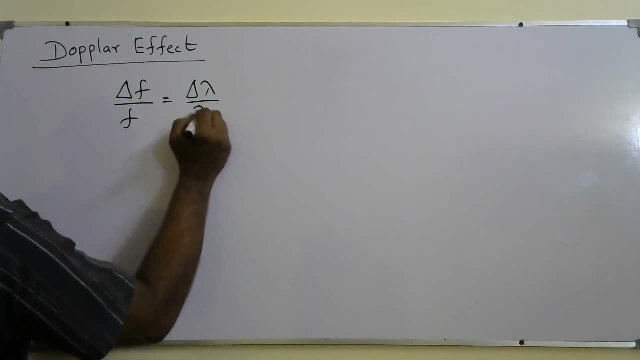 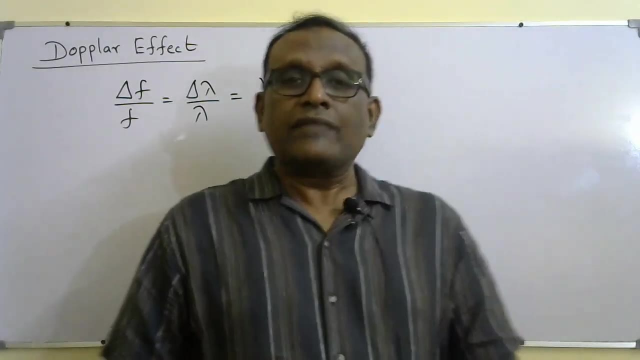 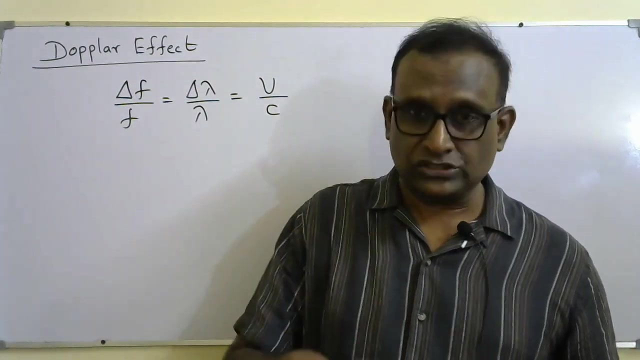 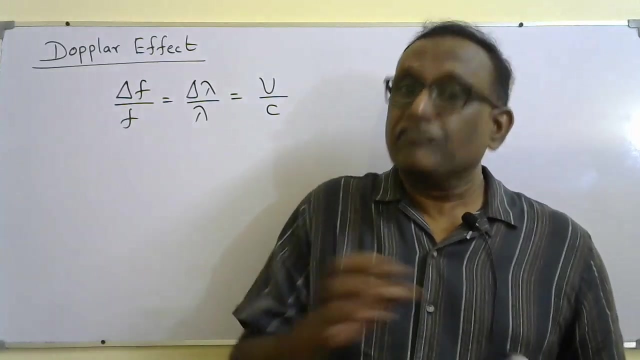 Delta f over f. equal delta, lambda over lambda. equal v over c. Okay, delta f means I told that whenever the wave source moves towards you or moves away from you, the frequency that you measure will be different compared to actual frequency. So delta f is the difference between the apparent frequency. Apparent frequency means frequency. 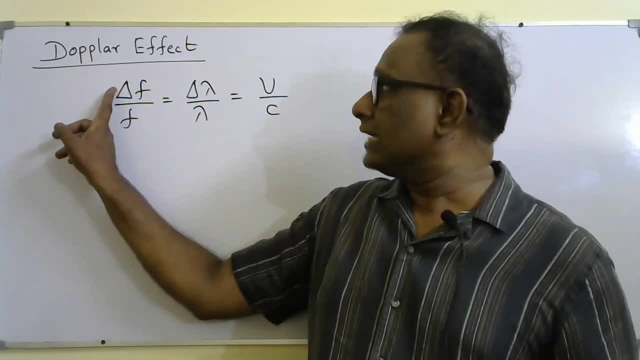 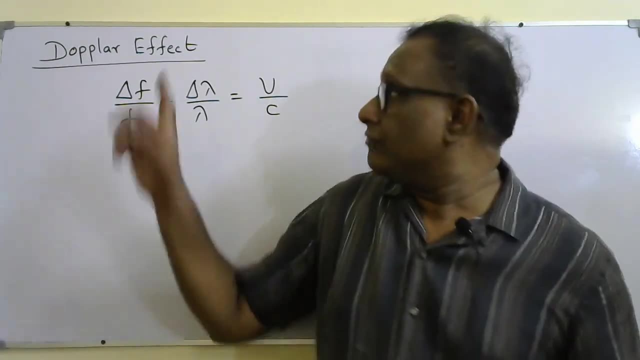 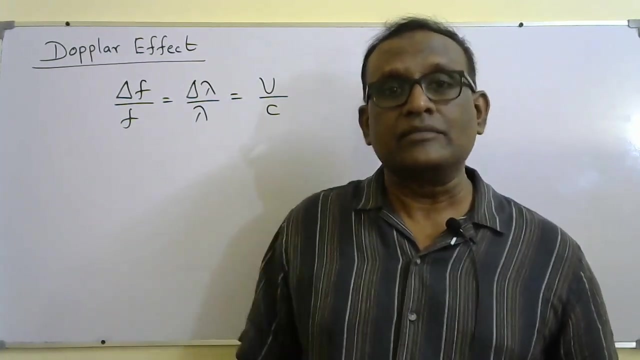 measured by the observer is called apparent frequency. So delta f is the difference between the apparent frequency and the actual frequency. Same way, delta lambda is the difference between apparent wavelength and actual wavelength. Apparent wavelength means wavelength measured by the observer is called apparent wavelength. So delta lambda means difference between the apparent wavelength and the actual wavelength. Here f is the actual wavelength emitted by the source- sorry, actual frequency emitted by the source. source lambda means actual wavelength of the wave emitted from the source, where v is the speed of the wave source relative to observer, c is the speed of electromagnetic. 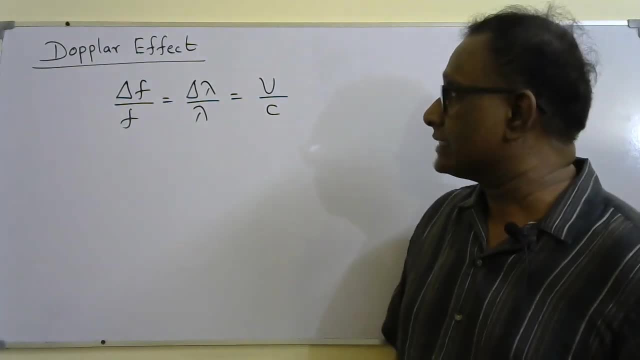 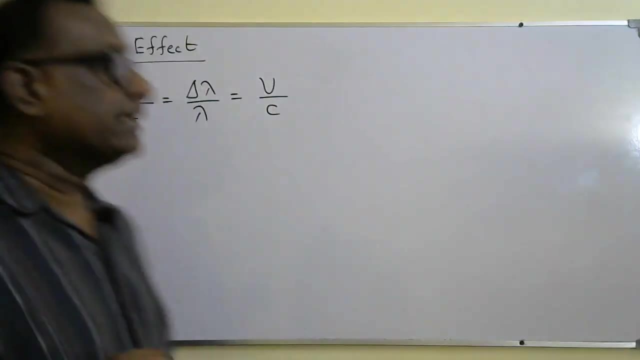 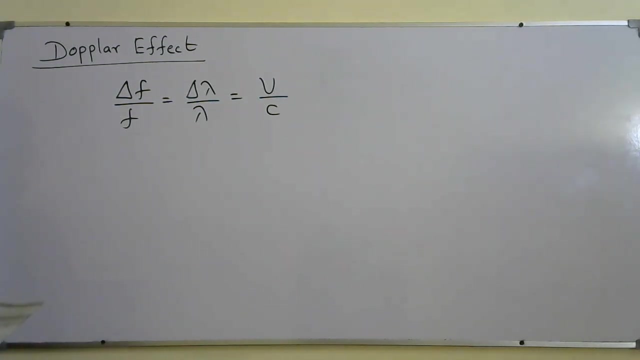 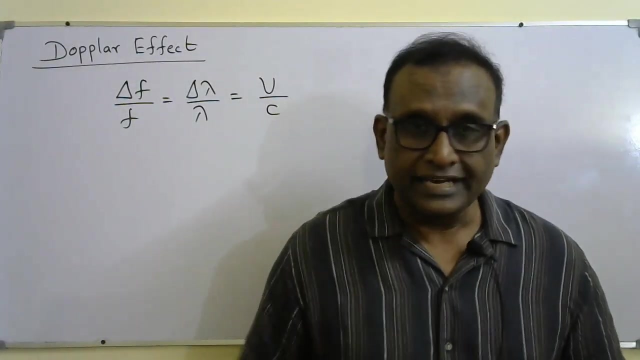 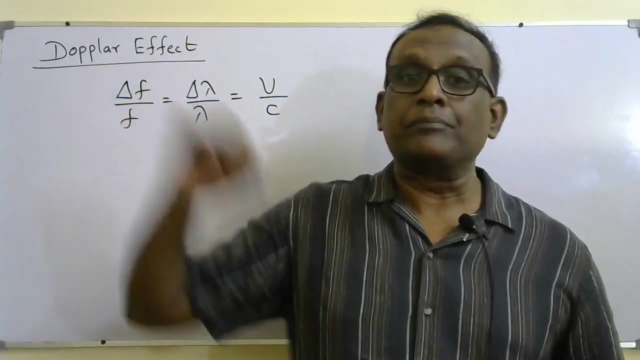 radiation, which is 3 into 10 to the power, 8 meter per second. So this is the Doppler effect equation, only applicable for electromagnetic radiation. Ok, so you should know in your syllabus. when the wave source relatively moves away from the observer, the apparent wavelength becomes larger. 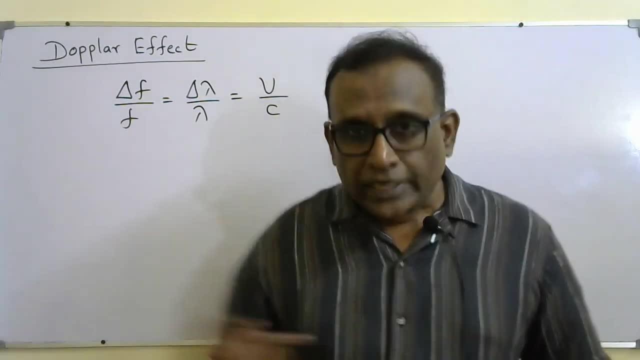 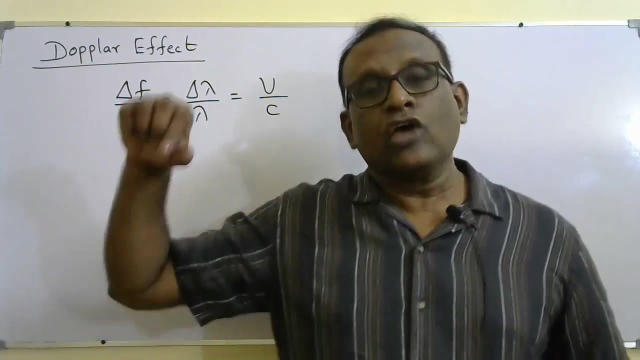 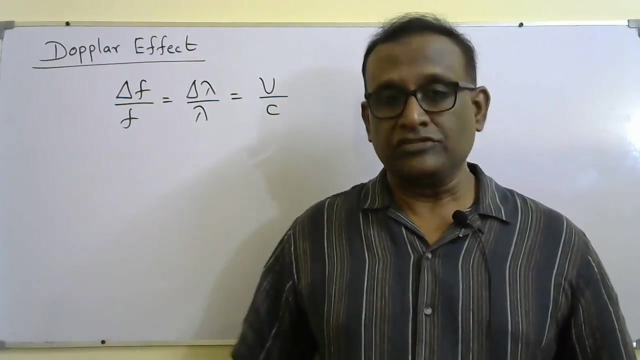 than the actual wavelength wavelength. when the wave source moves towards the observer, apparent wavelength will become smaller than the actual wavelength. same way, in terms of frequency, when the wave source moves away from the observer, apparent frequency will become smaller than the actual frequency. and then the wave source moves towards the observer, apparent frequency will become larger than the actual. 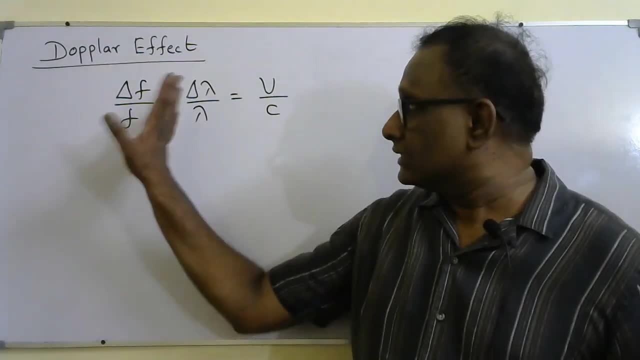 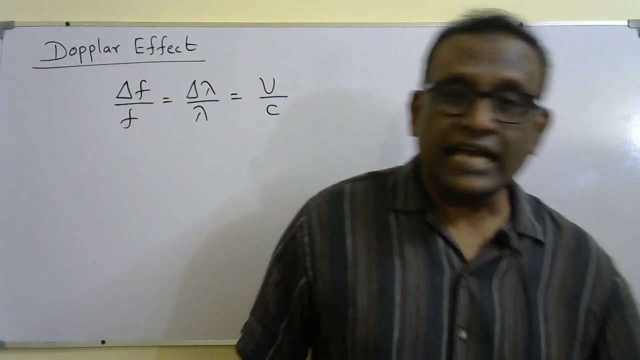 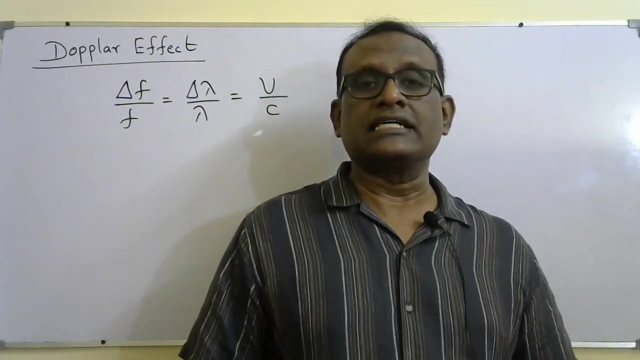 frequency. so we use this method, this Doppler effect, to measure the speed of recession of the galaxies. you know, all the galaxies have almost the same type of absorption spectrum. so you know what is galaxy. galaxy means it consists of several billions of stars. a group of stars is called galaxy. so if we focus, 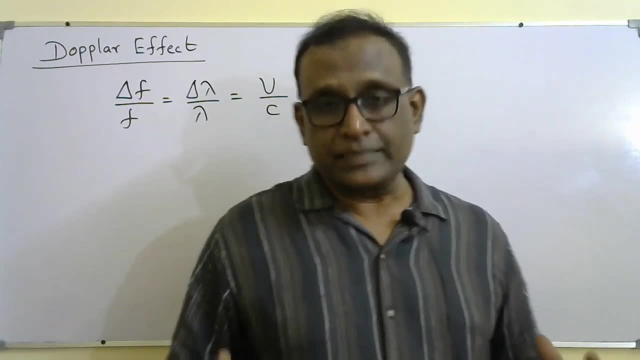 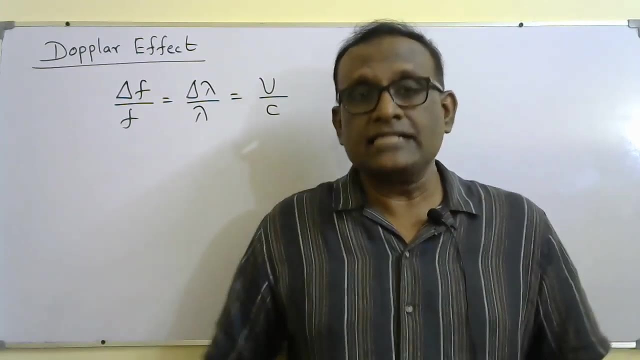 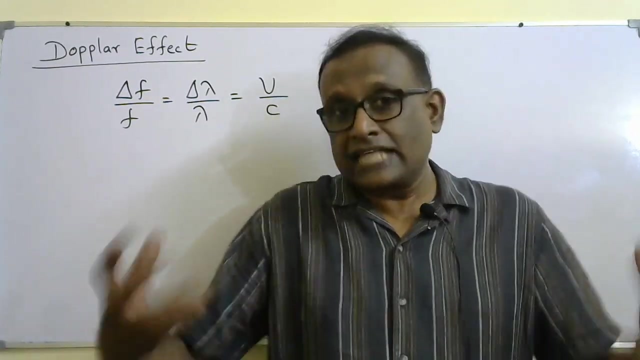 the telescope to different galaxies. their emission spectrum should be almost the same but there will be absorption spectrum. you know absorption lines due to the certain frequency of radiations absorbed by the gases in the galaxy, the gases of the stars in the galaxy. so when we observe different 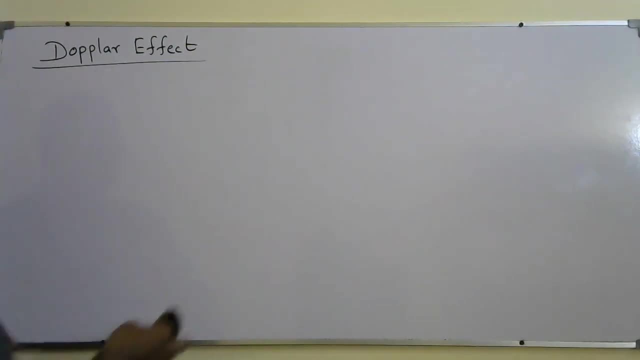 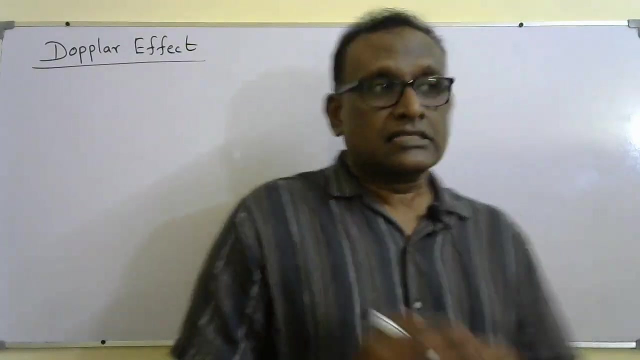 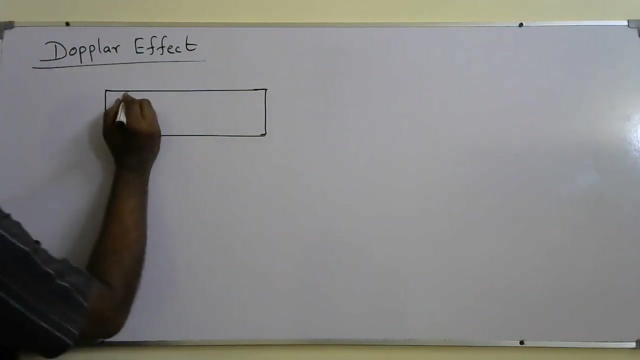 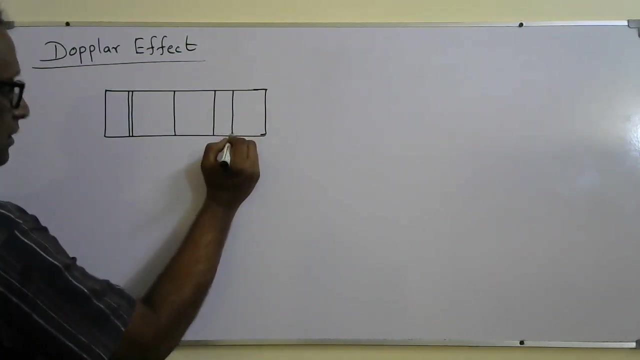 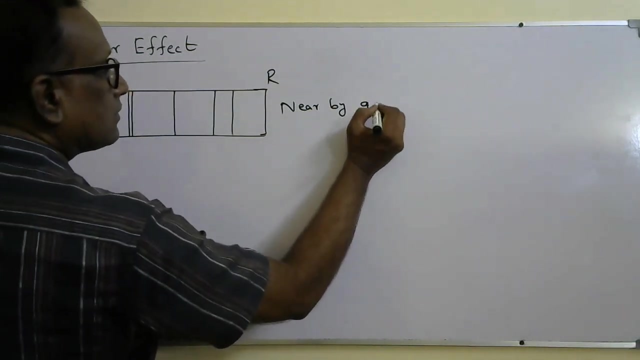 galaxies those are closer to us and far away from us. they found the absorption lines are identical. say, for example, when you consider a nearby galaxy- nearby galaxy- if the absorption lines are like this: this is violet, this is red, this is nearby galaxy. if you see the absorption. 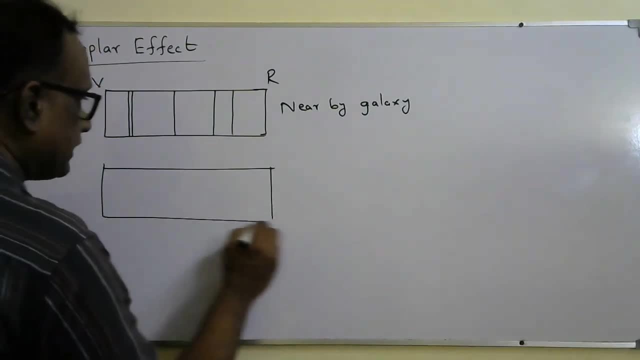 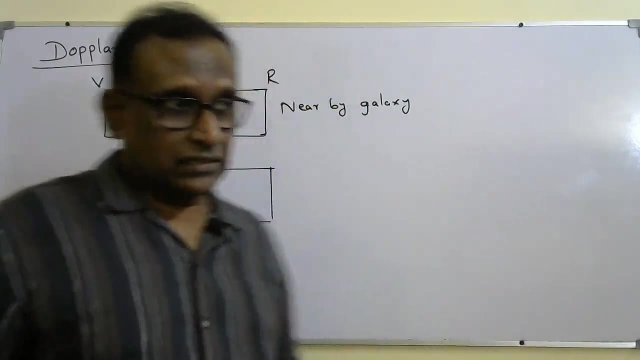 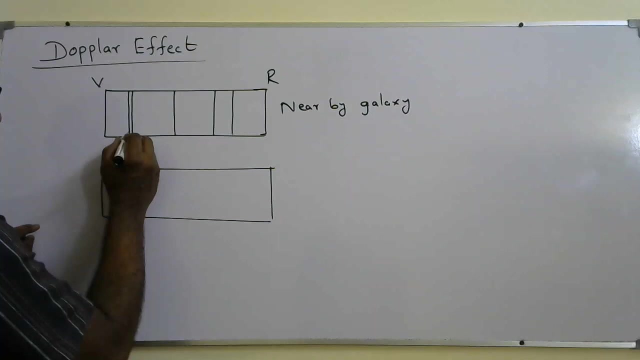 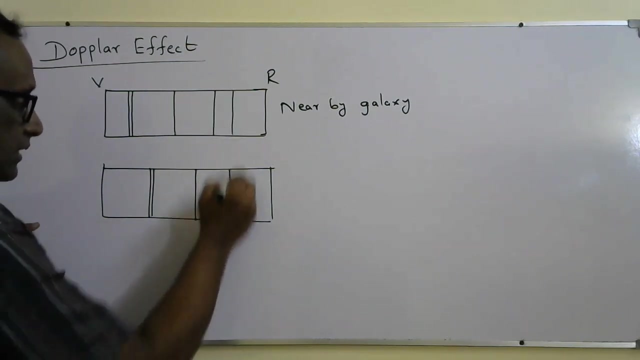 spectrum in a far-distance galaxy, the absorption lines. these are the absorption lines, but you learned in unit 2, under spectrum So far distance galaxies, the absorption lines have a similar pattern. The double line will appear here. the single line will appear here. this single line will be here. this single line will be here. 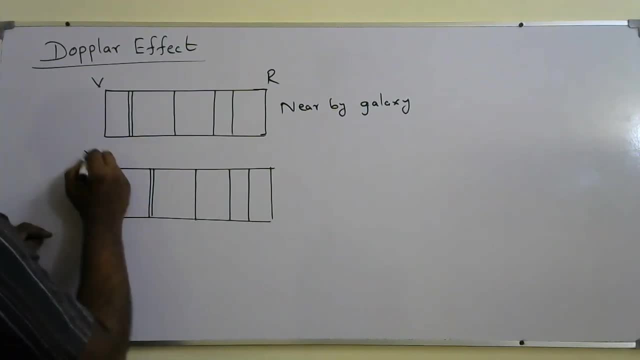 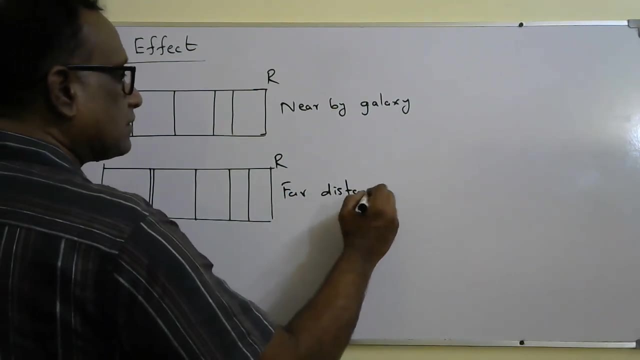 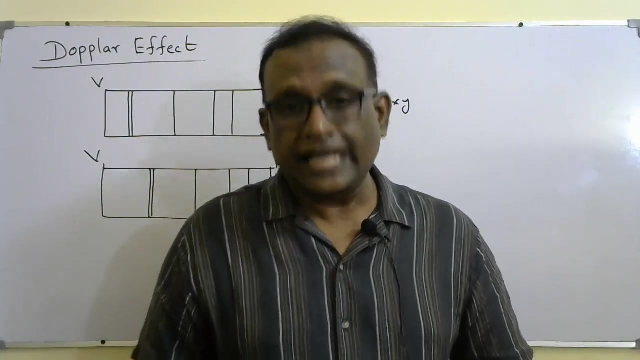 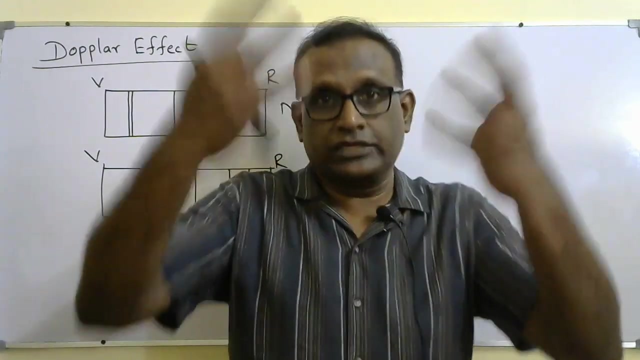 So the similar pattern, but the absorption lines will be shifted towards red color. This is far distance galaxy. So far distance galaxies have shift in absorption spectrum, or absorption lines means. according to Doppler effect, those galaxies are moving away from us. So they are the light. 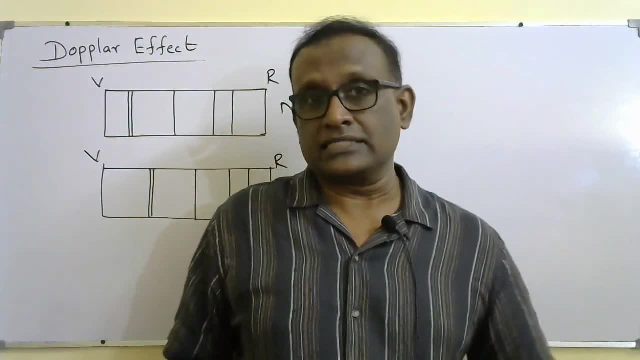 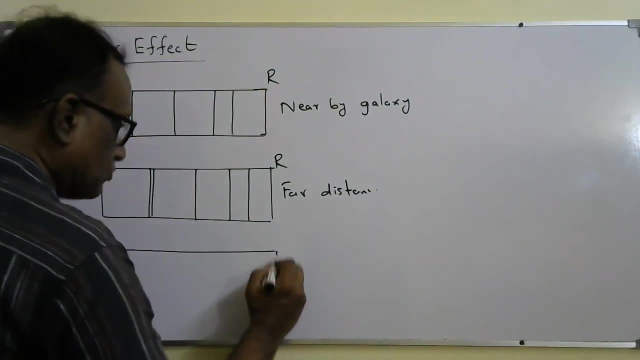 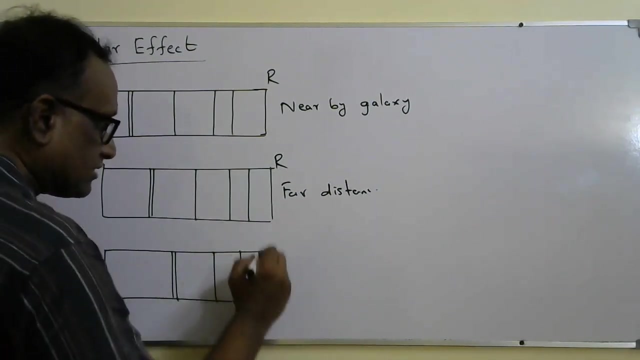 sources, wave sources. they are moving away from us. When you see another galaxy, which is much far away from us, in which the absorption lines will be similar, but this double line will be somewhere here. this single line here, this single line here, this will be here. 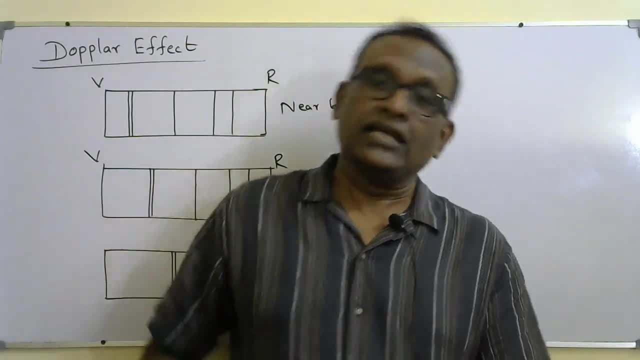 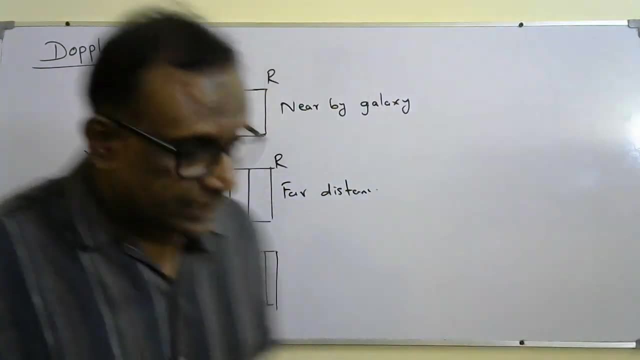 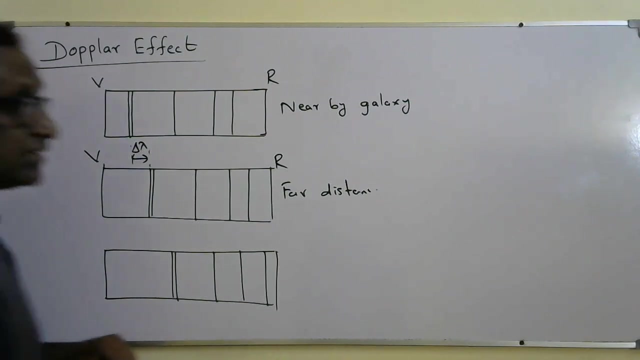 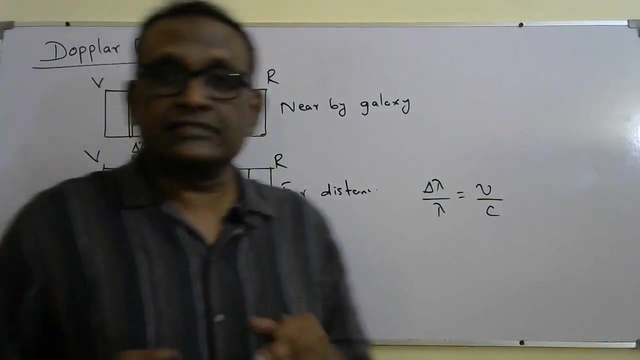 So it will have further shift towards red color. They are moving away from us because the wavelength is increasing towards red color. So by using the shift, by using the shift in the wavelength and by using the Doppler effect equation, We could be able to find the speed of recession, the speed at which those galaxies are moving. away from us. So what Hubble did for different, different galaxies? he measured the speed of recession of those galaxies by using Doppler effect method Also, he measured. also, he measured the distances of those galaxies by using Cepheid variable as a standard candle if the galaxies are at a distance less than 50 mega parsec. 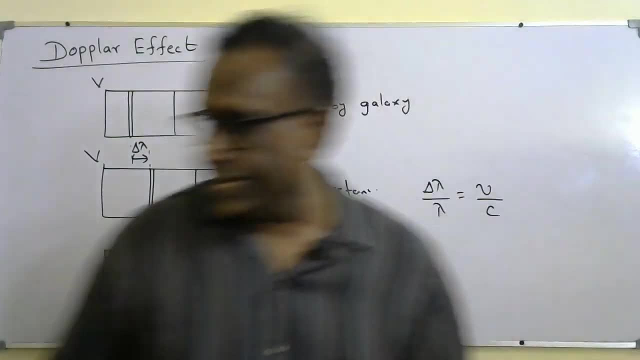 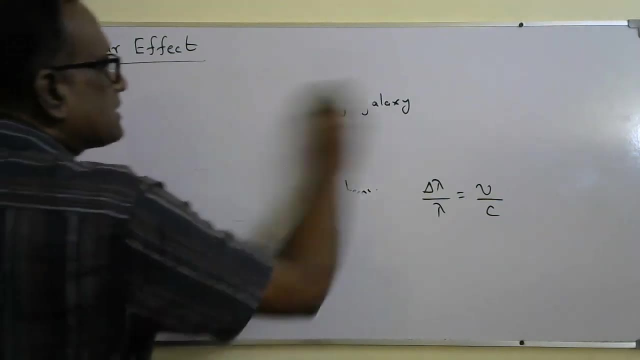 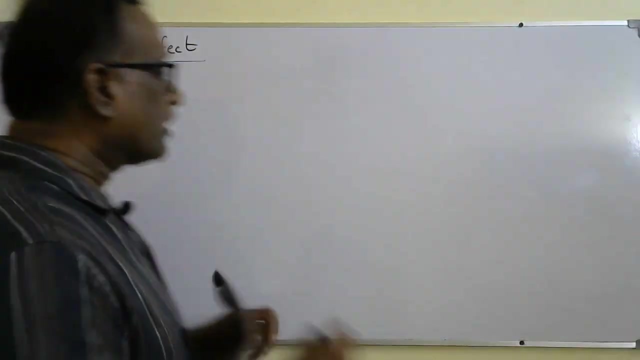 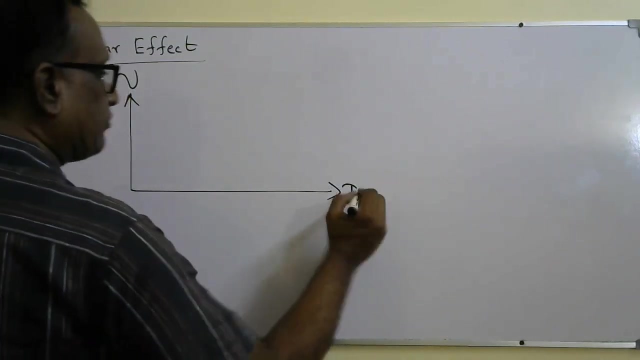 And when he plotted graph of speed of recession against distance, the distance of these galaxies were measured by using Cepheid variable as a standard candle. So the galaxies those are less than 50 mega parsec. He got a graph like a speed of recession against speed of recession against distance graph. 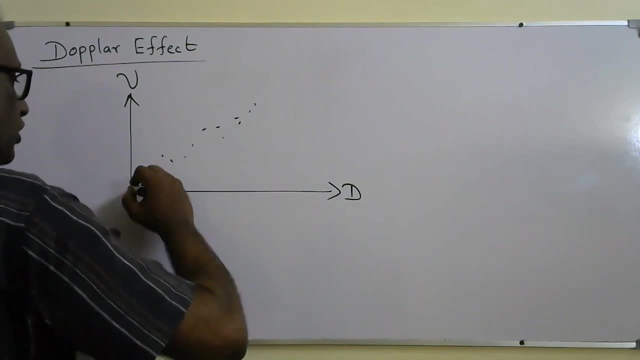 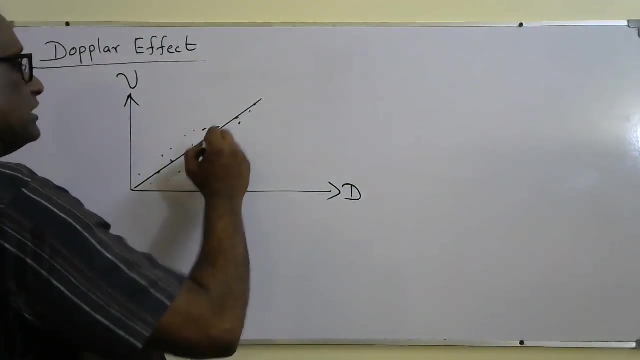 The best fit line is a straight line through the origin. So it's actually not a perfect straight line. The best fit line is a line which is passing through origin. So the distance is measured by using Cepheid variable as a standard candle. 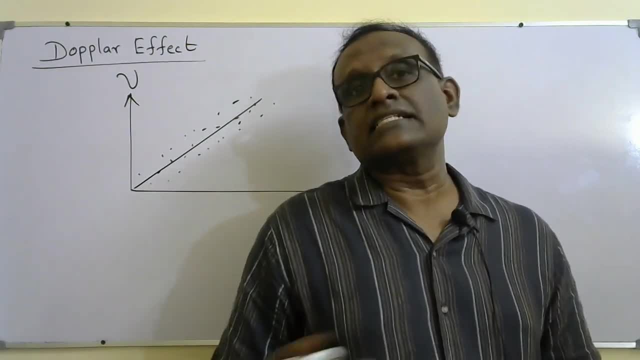 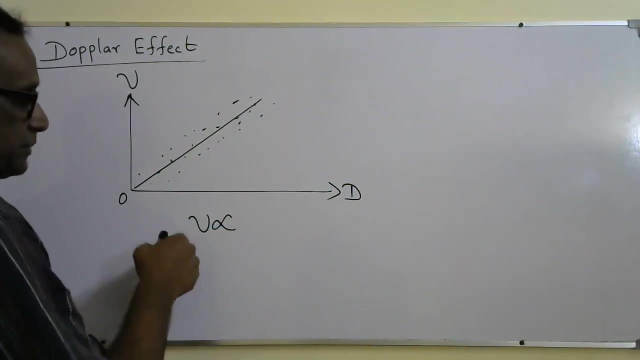 So he would have used Doppler effect method, He would have used the galaxies. those are at a distance less than 50 mega parsec. So from this graph, he said, we proportional to speed of recession, is directly proportional to distance of the galaxy from us. 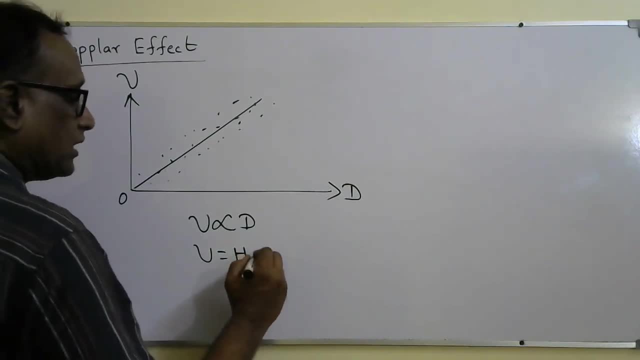 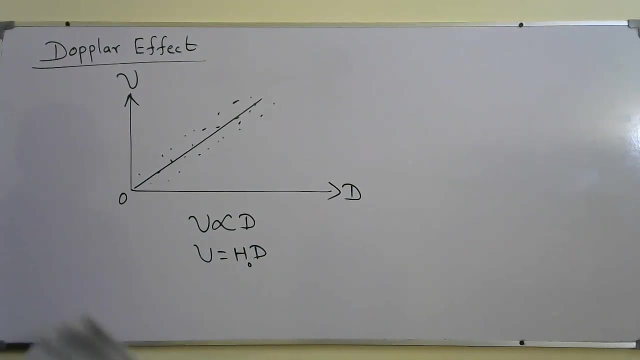 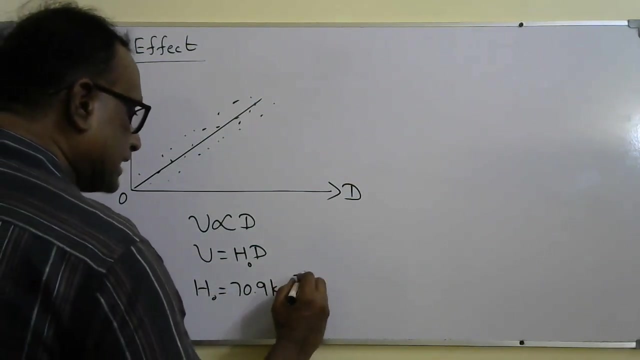 So speed equal a constant. later that constant is called Hubble constant H, or some books they call H naught. So the value of H naught is almost equal to 70.9.. Kilometer per second, per mega per second. So the distance was measured in mega parsec. 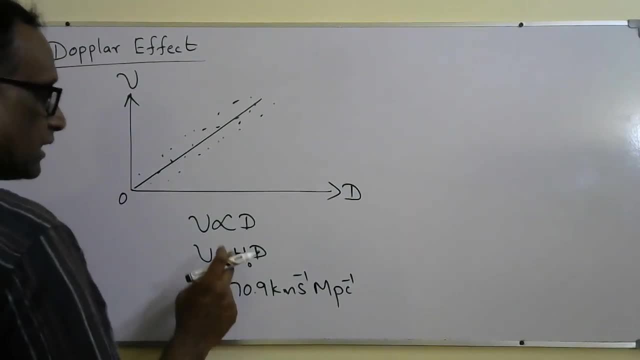 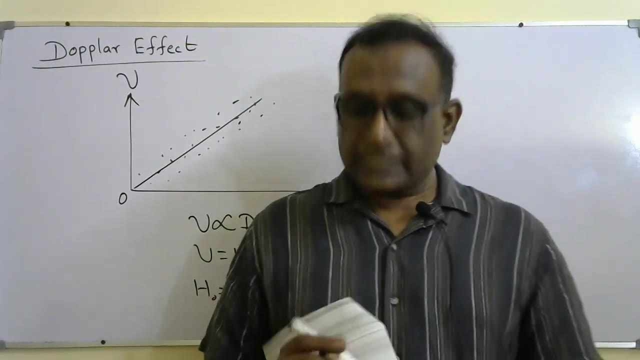 The speed of recession was measured in kilometer per second, So the Hubble constant is in the unit of 70.9 kilometer per second, per mega per second. The Hubble constant has very large uncertainty because the distance, the measurement of distance, 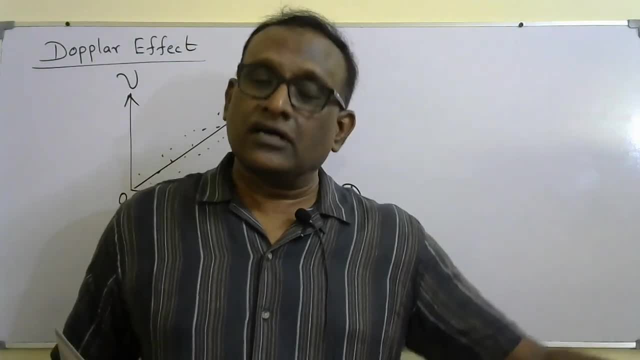 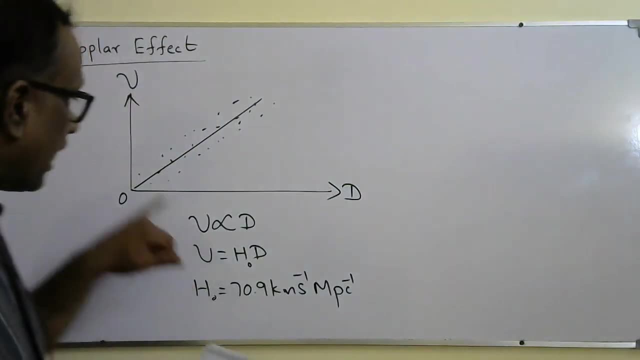 has very large uncertainty because it's almost up to the maximum distance, Up to the distance of 50 mega parsec, and he used Cepheid variable method. So there is larger uncertainty in the measurement of distance because of large uncertainty in the measurement of distance. 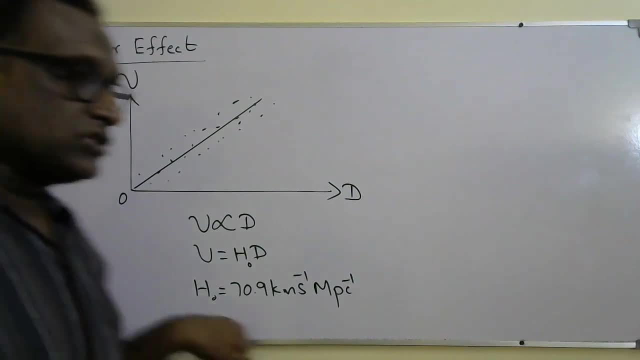 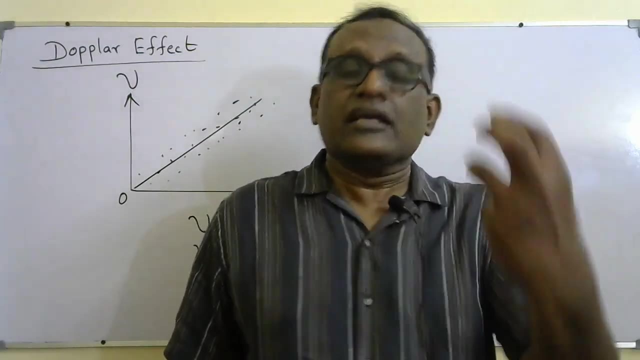 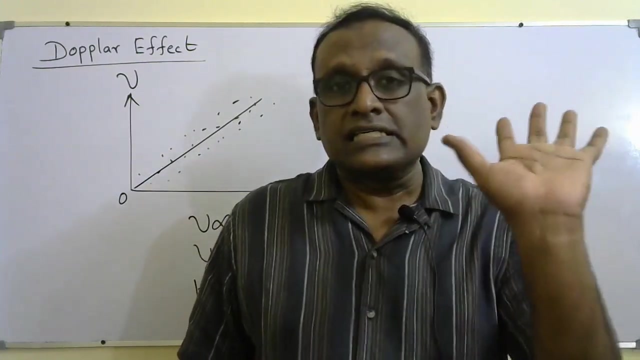 Hubble constant also has large uncertainty. Okay, so now we can use this graph to find the distance of much far away distance galaxies. Say, there's a galaxy which is much far away, more than 50 mega parsec. So in that galaxy, Measure the redshift. we call. redshift means delta lambda or lambda. measure it from the. 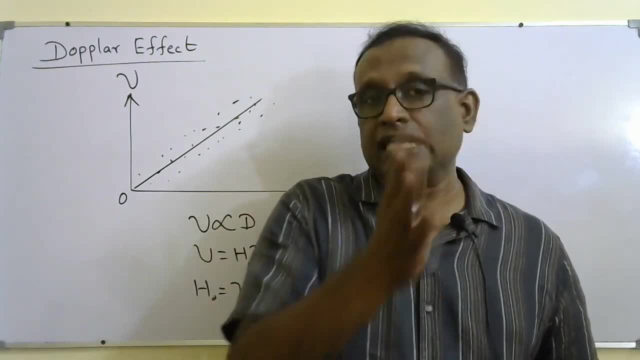 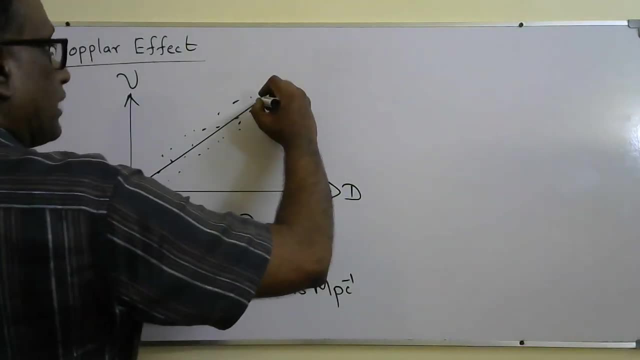 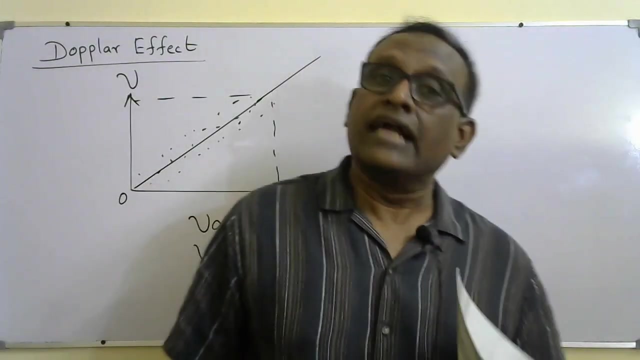 absorption spectrum, Measure the shift delta lambda. So from that find the speed of recession of the galaxy. If you know the speed of recession of the galaxy, you can extrapolate this graph. So from that you can find the distance of that galaxy, which is more than 50 mega parsec. 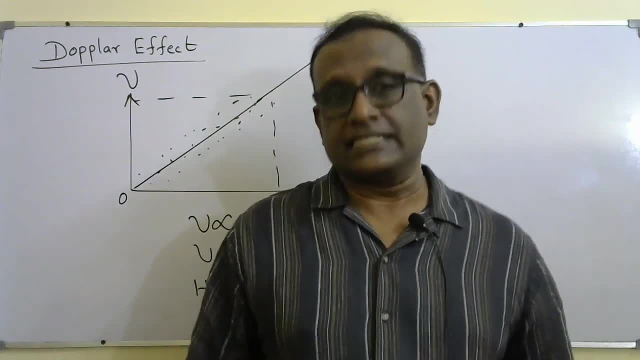 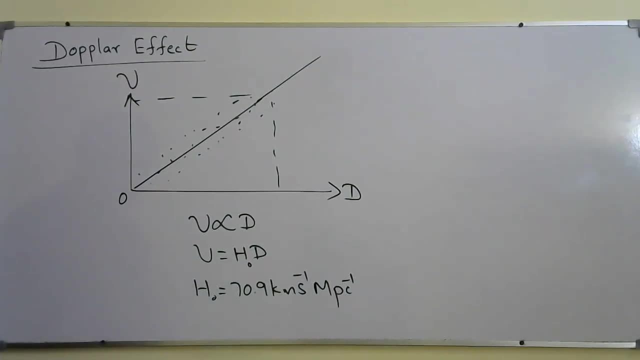 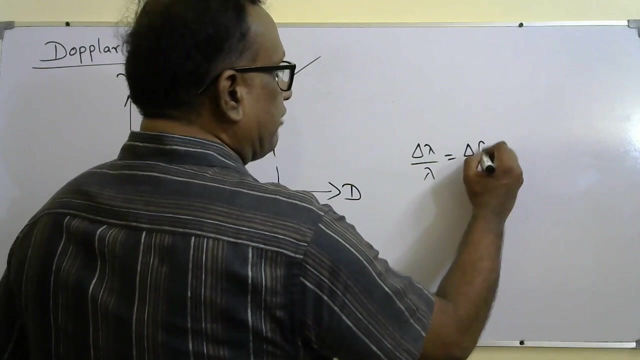 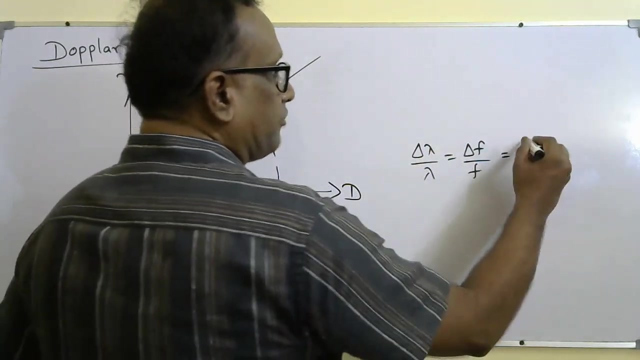 But there will be large uncertainty In that distance because Hubble constant has larger uncertainty. So in the Hubble, in the doctor equation we call delta lambda over lambda equal delta f over f, equal v over c. This ratio, whether delta lambda or lambda, or delta fof or v over c, this ratio is called 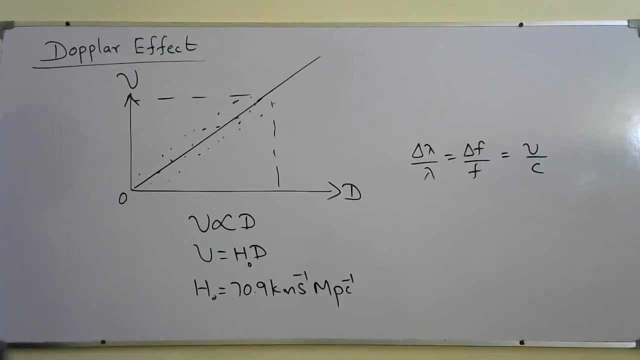 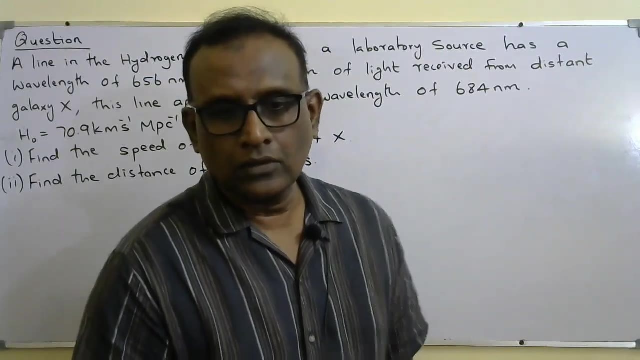 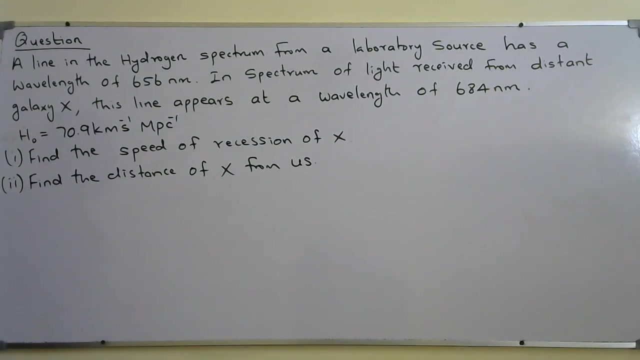 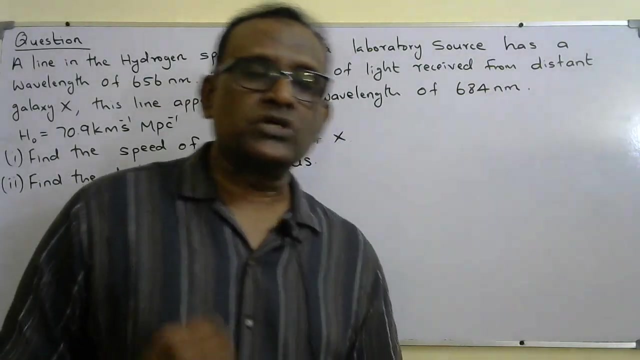 redshift. Okay, Okay, Okay, Okay. There could be a question like this: Light in the hydrogen spectrum from a laboratory source has a wavelength of 656 nanometer. So that's actual wavelength. So laboratory source, or we can say, in our galaxy there is no relative motion. 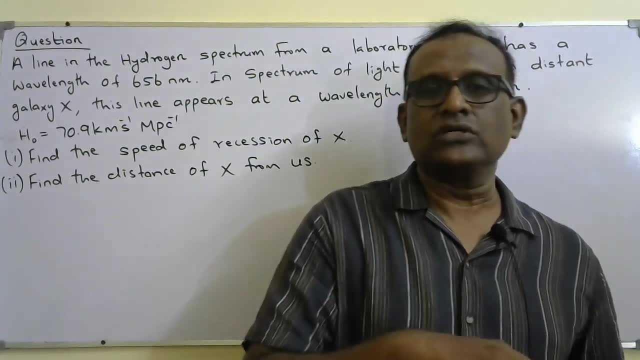 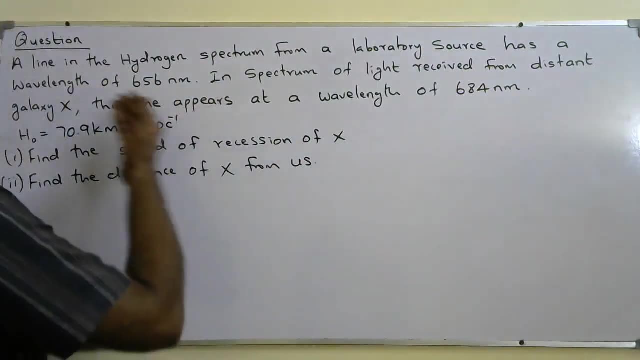 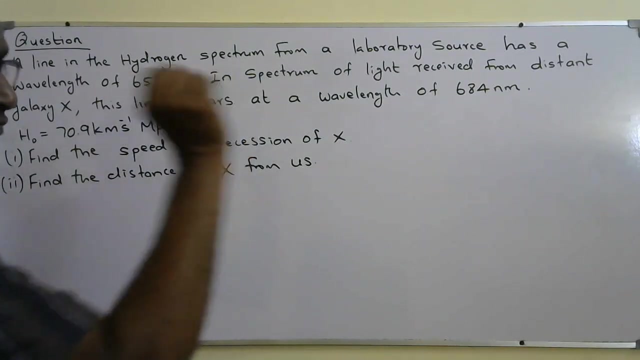 When we consider our galaxy, all stars are related to us. They are at rest. our galaxy is at rest, related to us, is it so? all we can see that is a wavelength measured from the laboratory. so there is no relative motion in the laboratory. so that is the actual wavelength of 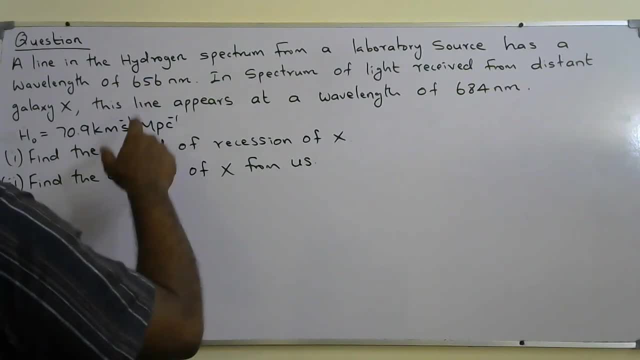 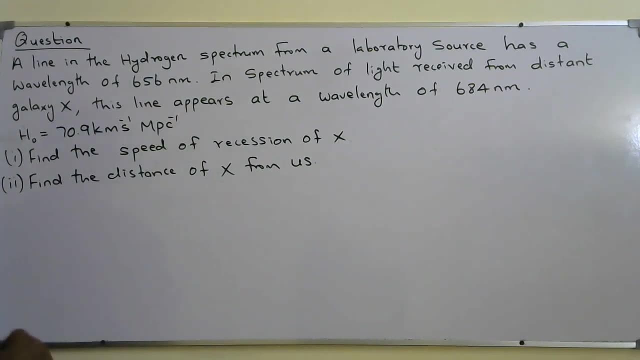 that particular line of hydrogen. if the spectrum of light received from distant galaxy x, this light appears at a wavelength of 684 nanometer means there is a increase in wavelength. so this is the apparent wavelength. hubble constant is given. first part, find the speed of recession of x. so we 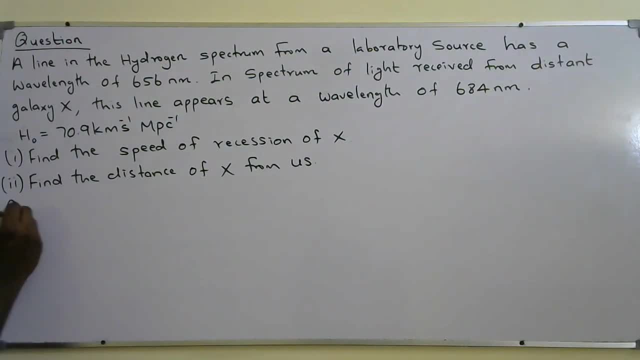 need to use doppler equation. so first part: delta lambda over lambda equal v over c. so delta lambda means the difference between 684 and 656 over actual is the laboratory wavelength. that's actual wavelength 656 equal v. the speed of recession over 3 into 10 to the power 8. so 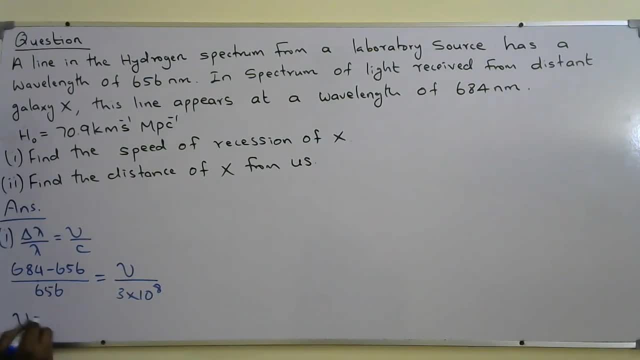 you solve it, you will get the speed. so speed of resistance will become 1.28, 10 to the power, 7 meter per second. so related to us. it's moving away from us at this speed. second part: we need to find the distance of it. we can find by using the differential equation. 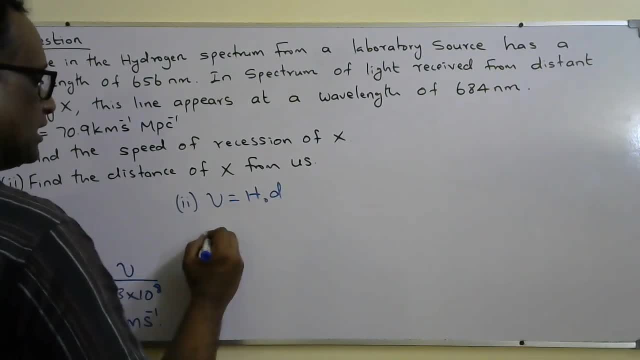 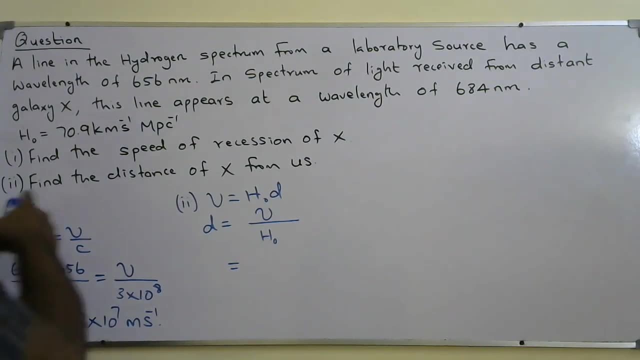 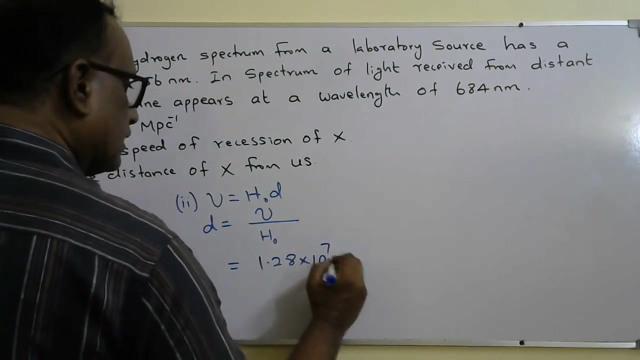 Harvard's law V equal H naught D. so D is going to be V over H naught. so we can find it in mega parsec. they'll find the distance we can give it in parsec, mega parsec. V is you know, 1.28, 10 to the power, 7 meter per second over H naught is. 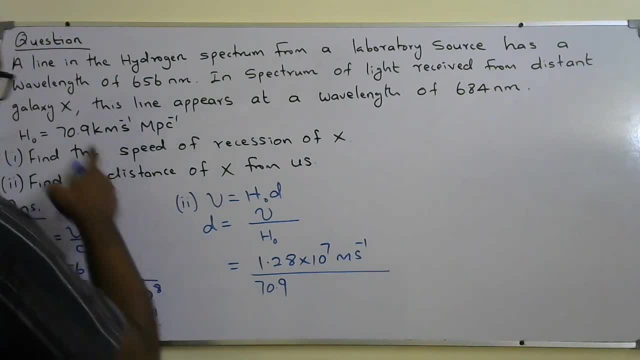 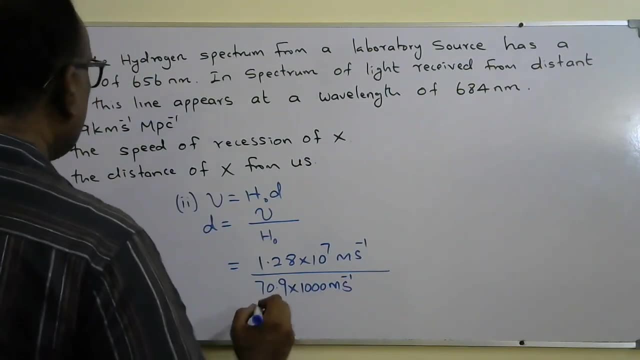 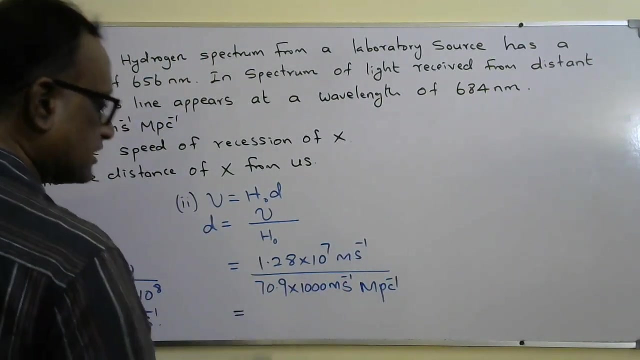 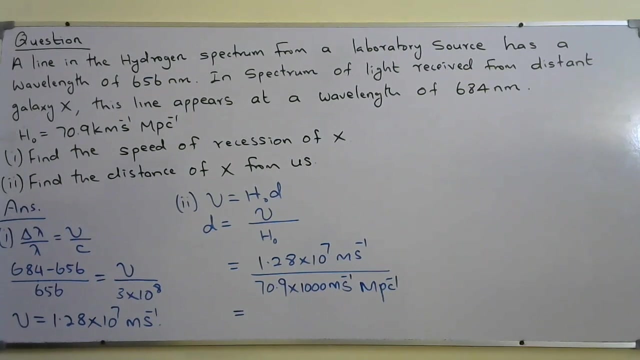 given 70.9 kilometer. so we'll convert meter because here is meter. so multiply by thousand meter per second per mega parsec, and so mega parsec will go up meter per second, meter per second will get cancelled, so we'll get the final answer in mega parsec. solve it. 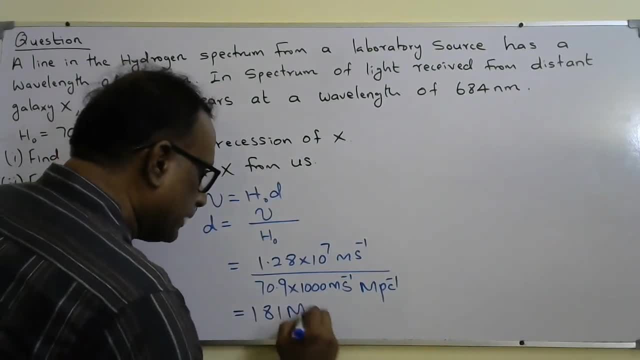 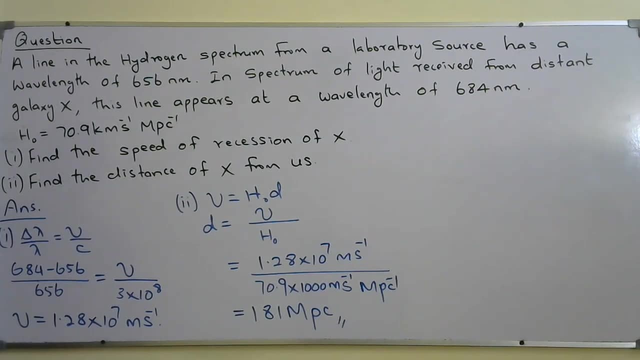 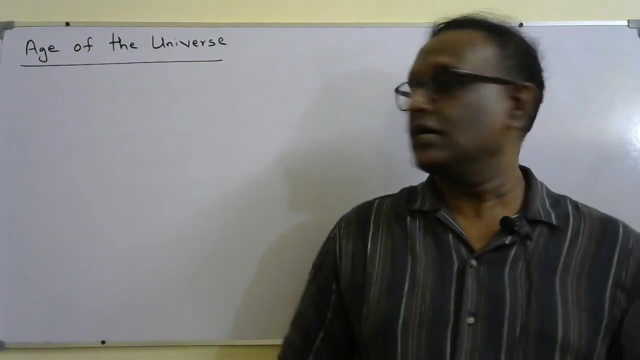 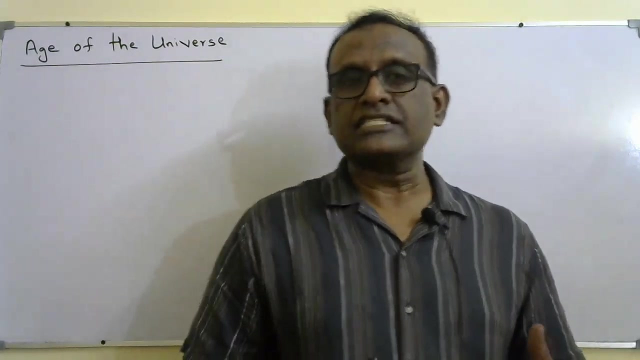 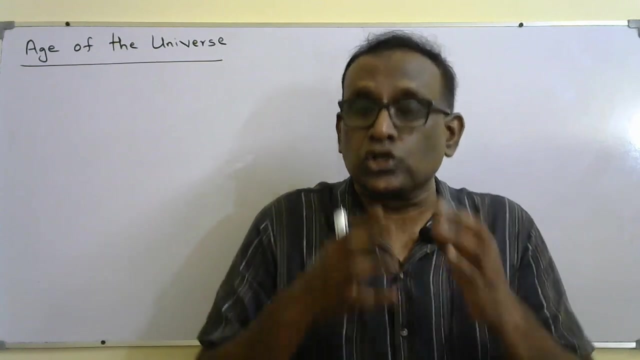 so almost 181 mega parsec. so the next thing is about how to estimate the age of the universe from the big bang. okay, so we assume there are. we take two assumptions. first assumption: we take all the galaxies before big bang. all the galaxies were together in. 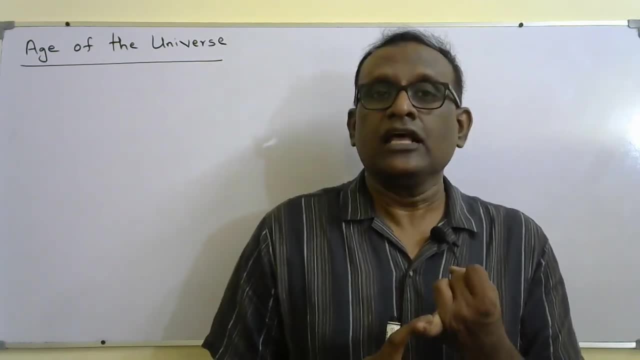 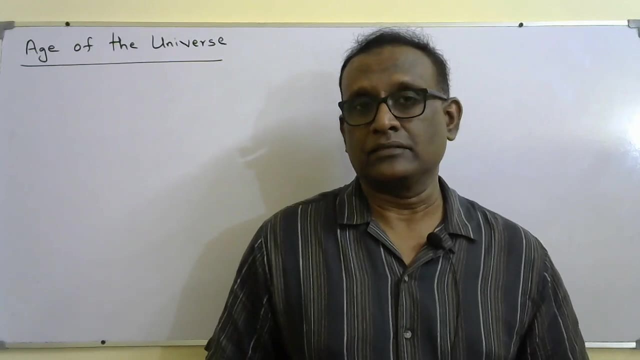 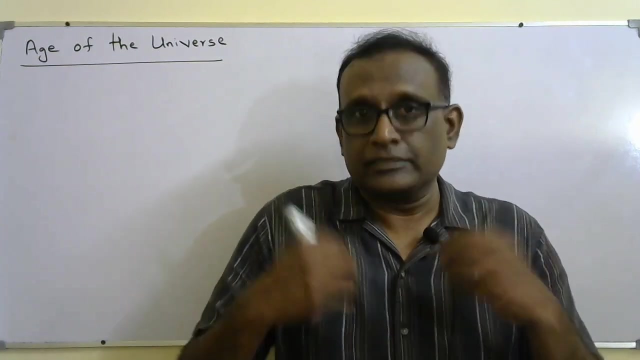 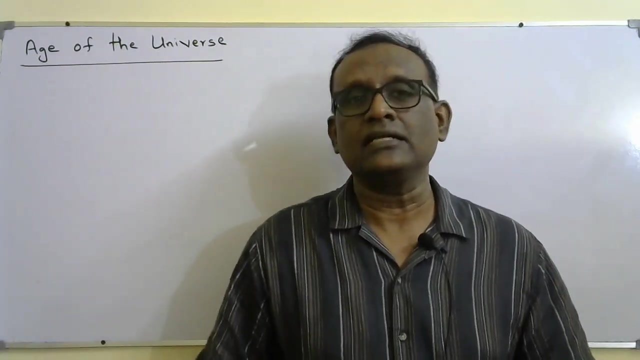 closer to us. first assumption, second assumption: all the galaxies are moving away from each other at constant speed after the big bang. two assumption again. i'm saying first assumption: all the galaxies are together, closer to us. that means we are the midpoint. the earth or our solar system or our galaxy is the mid of the universe. we assume like that. then, second assumption: all. 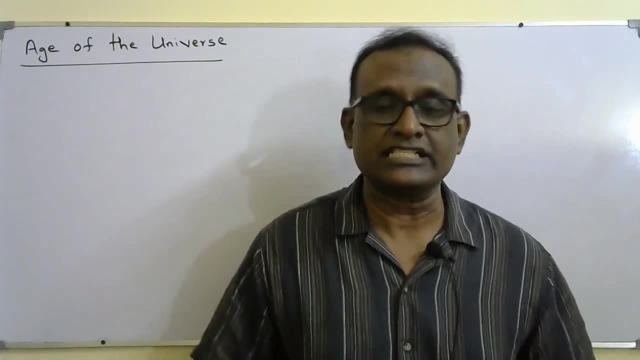 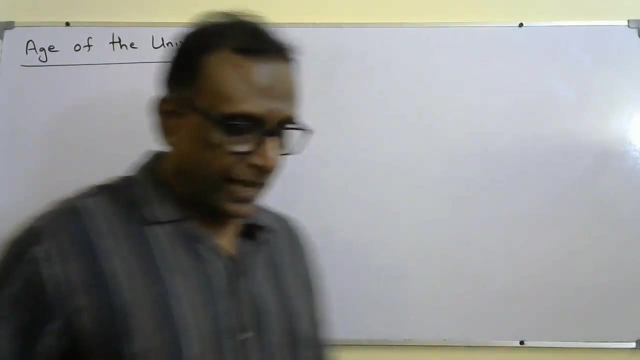 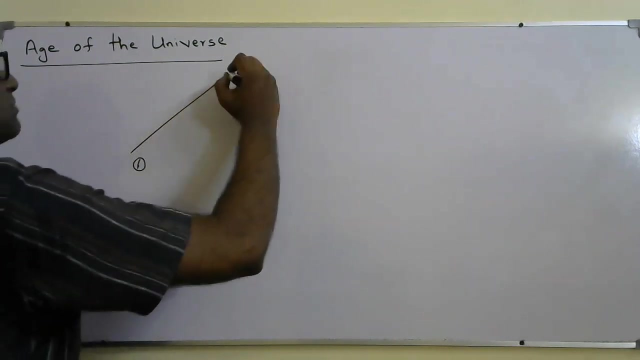 the galaxies are moving away from us at constant speed after big bang. so by using that we can find the age of the universe. okay, so imagine we are here and there is a galaxy somewhere here, another galaxy. so the distance it has moved is d and we assume it's moving at constant speed. 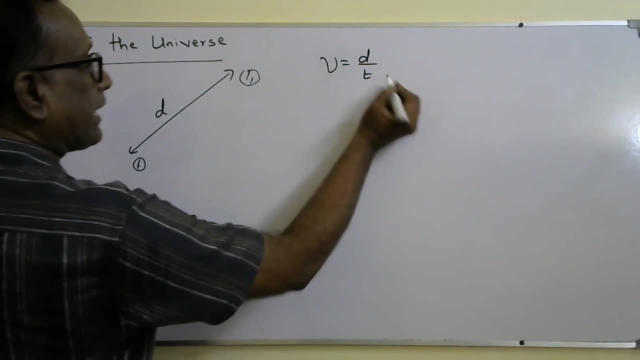 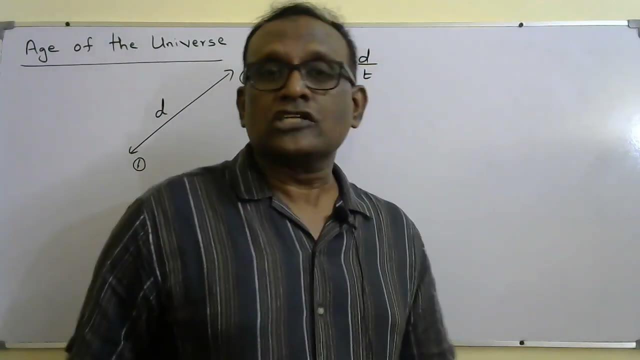 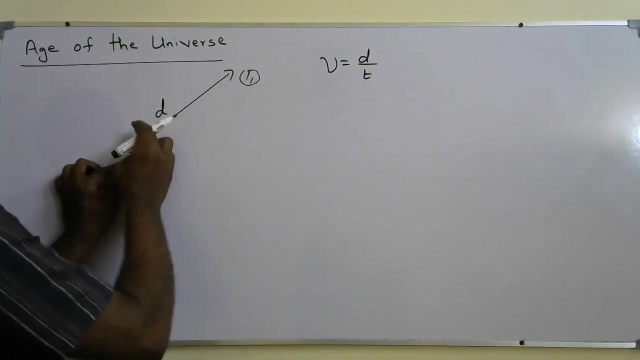 so we know that speed equal distance over time. so the time taken by this galaxy to come this distance is the age of the universe, because we assume all these galaxies were together with us. now it has gone to this position. a distance d away from us means, if i find the 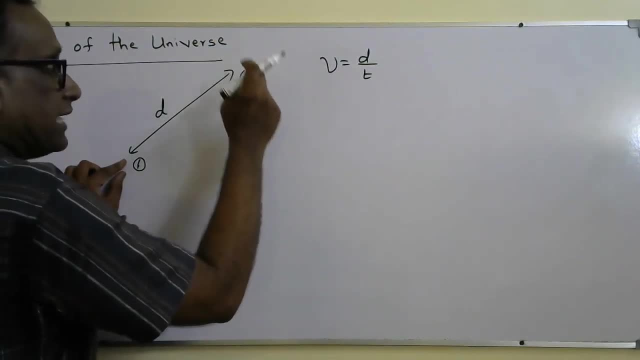 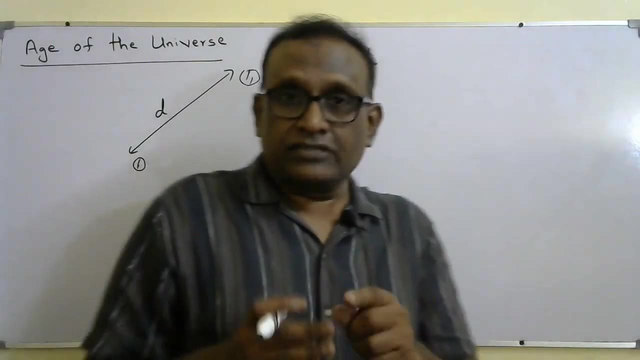 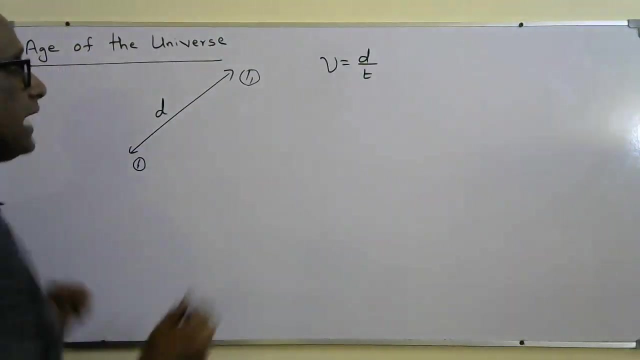 time taken by the galaxy to this galaxy to reach this position, or the time taken by the galaxy to move a distance d from us, is the time duration from the moment of big bang. that is the age of the universe. so speed, equal distance over time. so time, equal distance over speed. but it will. 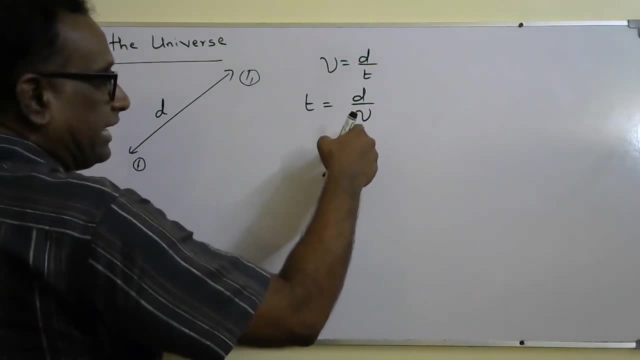 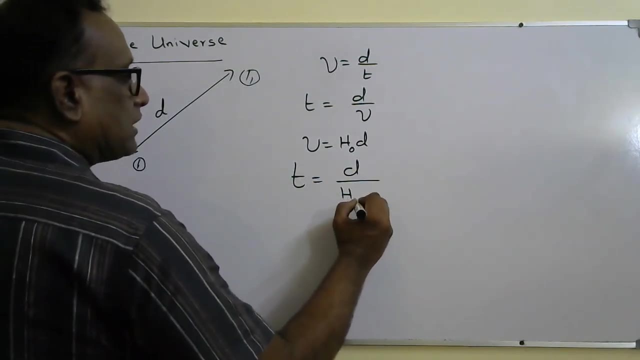 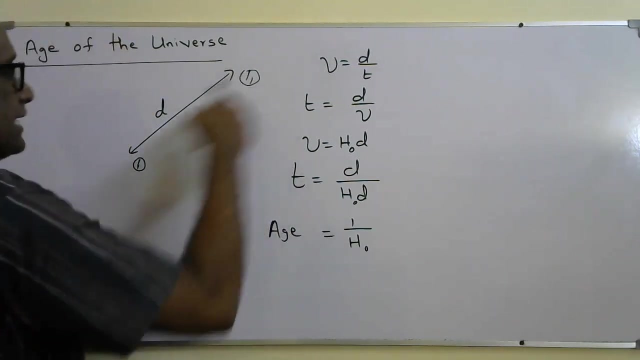 a very approximate method, so, but i know that v equal h naught d, so time, equal d over h naught d, d and d will get cancelled. one over h naught. that is the age or the time taken by this galaxy to complete a distance d from the moment it was with us. 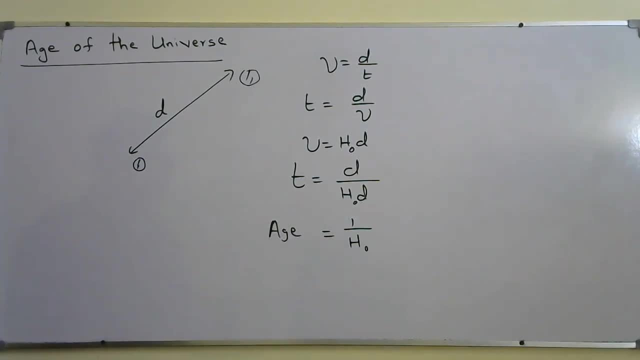 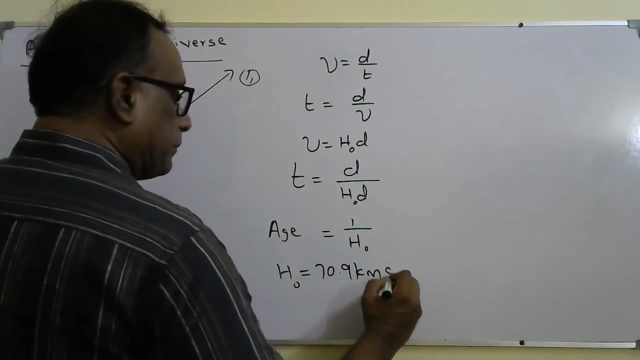 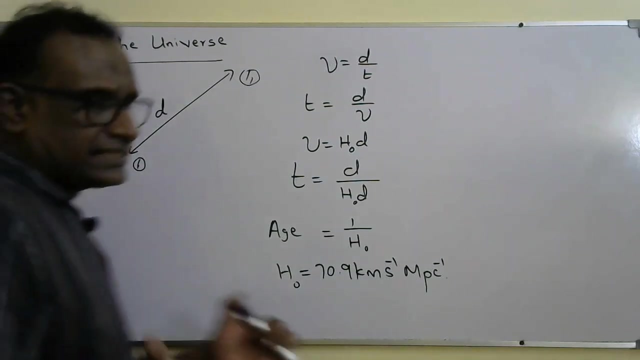 just before big bang. so age is given by one over h naught. you know the h naught is equal to 70.9 kilometer per second, per mega per second. okay, we'll find whether we are getting you know. you can check it in the internet or any books. it says: age of the universe is almost 14 billion years. we 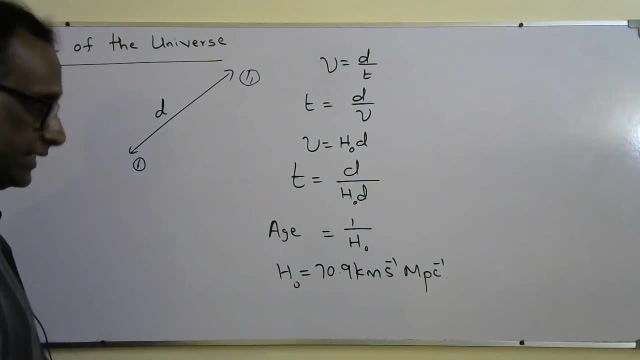 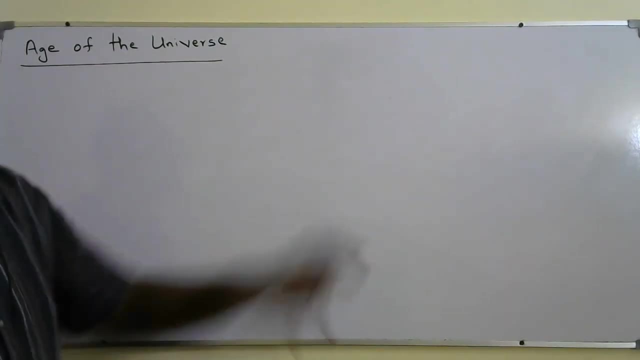 will see whether we are going to get the age 14 billion years. you'll find it. now. you can see i've changed the expansion period all the way over the x axis. you should be able to get that expression: aquilo viendo seiner, so age equal. 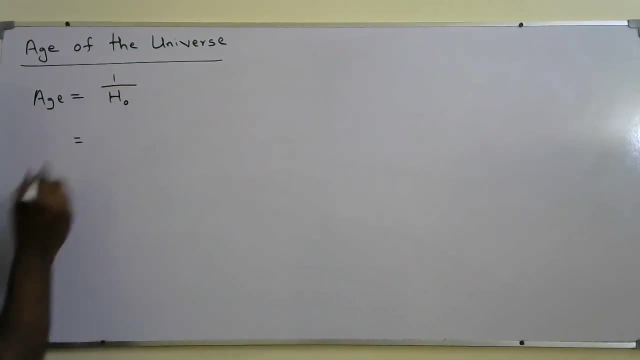 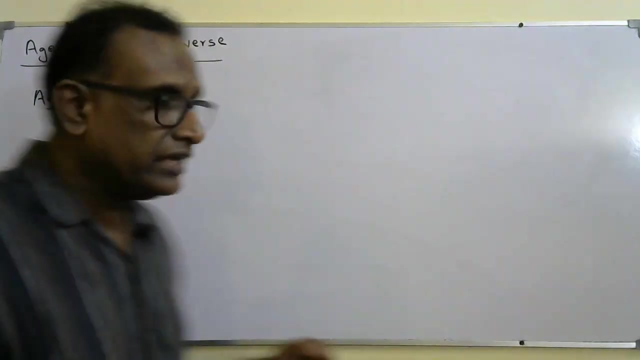 one over h naught. so first i should convert h naught to simplify to a normal unit rather than mega false x. so we will find out that first h not is equal to 70.9 kilometer per second per megabit per second. okay, that means we need to tube the. 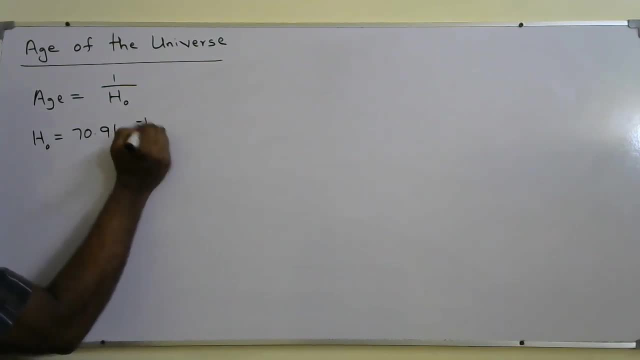 value on this? whats the value of h naught lord? Okay, that means 70.9 kilometers, so 1000 meter per second. per megaparsec means megaparsec. is it Per mega? there's an index. minus 1, means 1 over megaparsec. 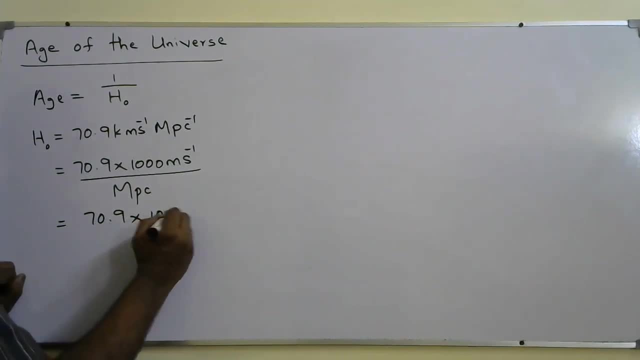 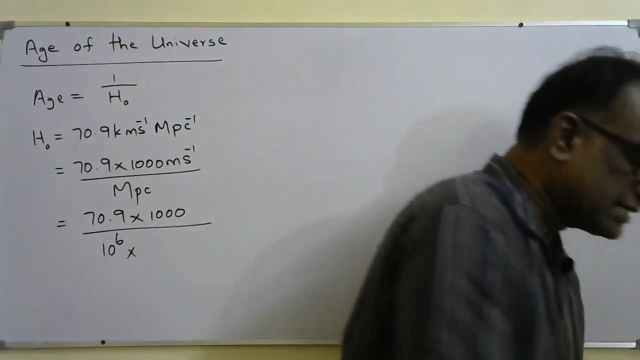 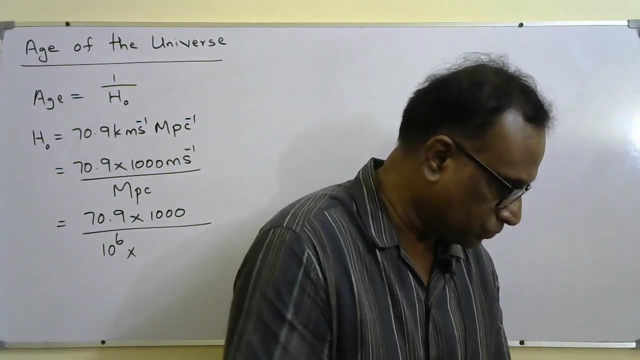 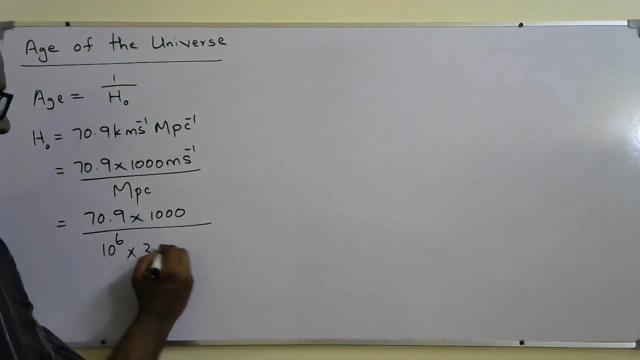 So convert this 70.9 into 1000 mega 10 to the power: 6. 1 PC. that will be given in the question paper whenever they ask this question. 1 PC is equal to- I already derived it. 1 parsec is equal to 3.09, 10 to the power: 60 meter. so here meter per second, is it? 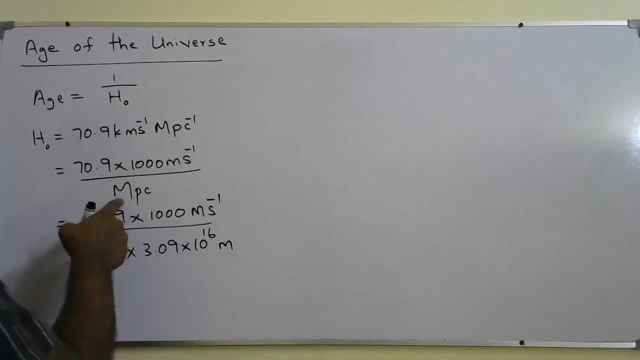 So 70.9 kilometer per meter per second megaparsec. so it's going to be. Sorry, I think I made a mistake. 70.9,. okay, I'm fine, that's right. yeah, meter per second. 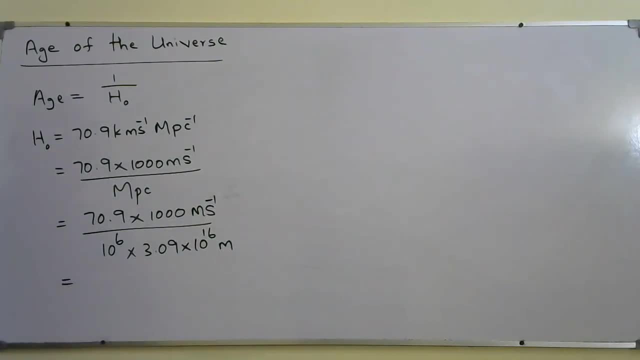 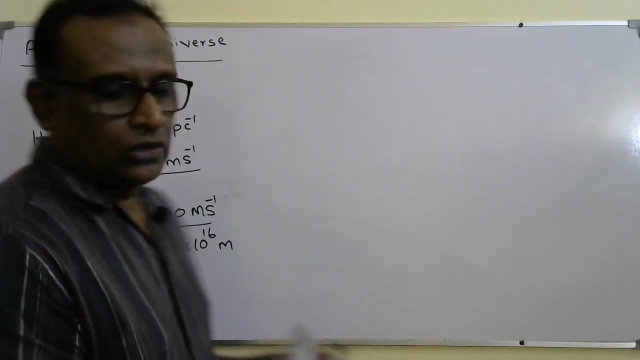 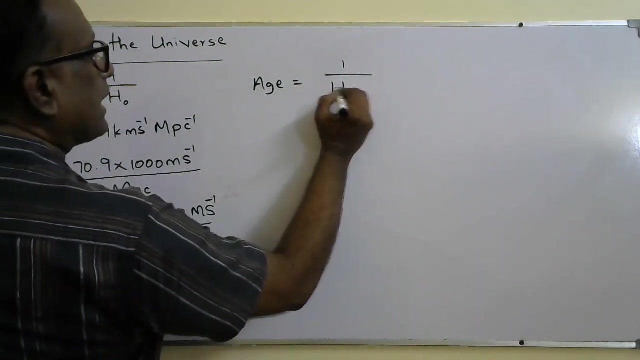 Okay, we'll get the answer in parsec. sorry, we'll get the answer H0 in parsec. Okay, so that's the value of H0, so H of the universe equal 1 over H0, so that is going to be 1 over parsec. 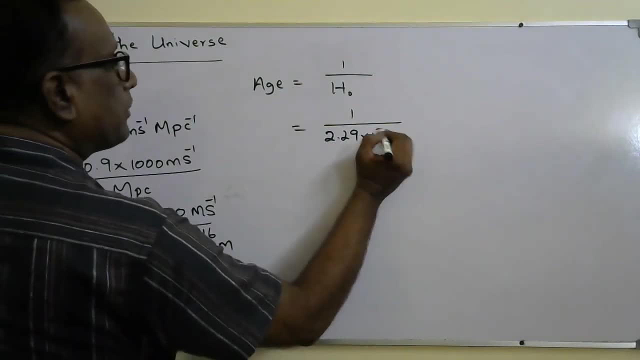 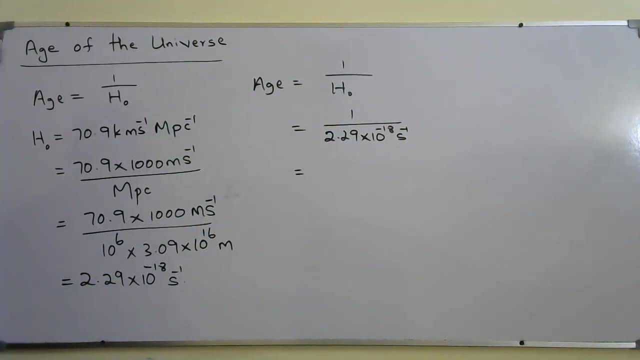 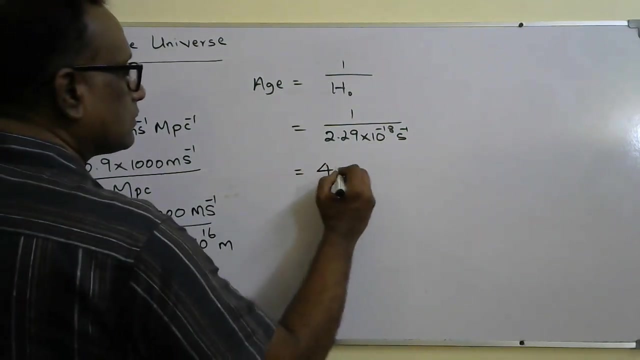 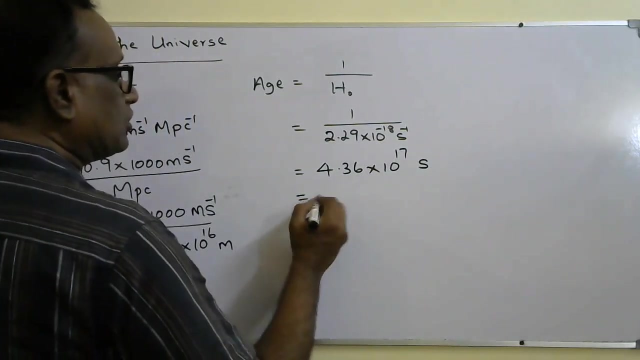 2.9.. 10 to the power, minus 18 per second. so when it goes up it will become second. So solve this value. That will be 4.36.. 10 to the power: 17 seconds convert to billions of years. 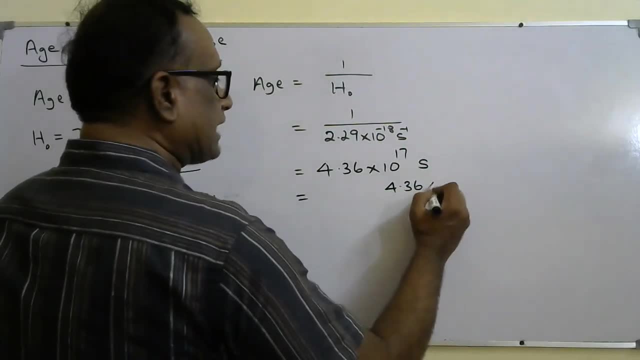 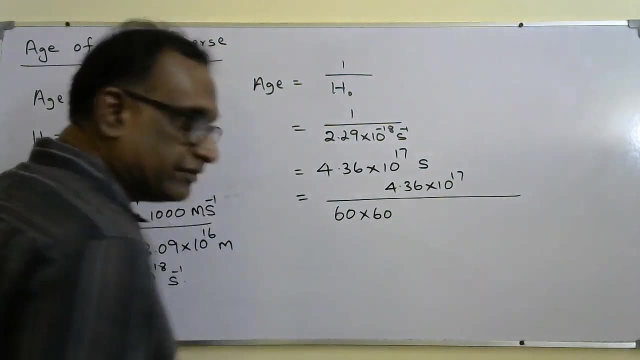 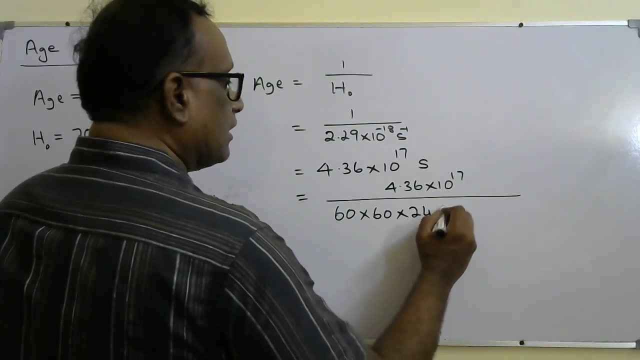 So to convert this to 4.36.. 10 to the power, 17.. To convert to minute divide by 60.. To convert to hour divide by 8 to the 60.. So, second to minute hour, hour to day, day to years, billion. 10 to the power, 9, billion years. 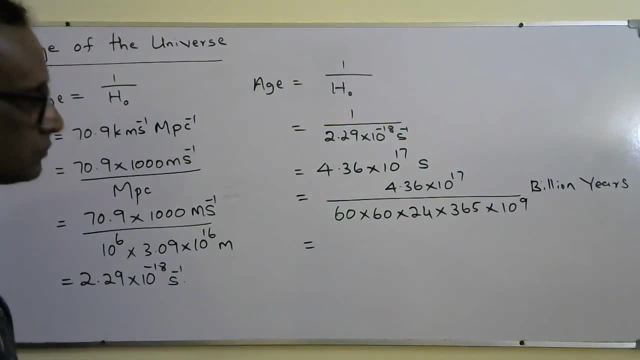 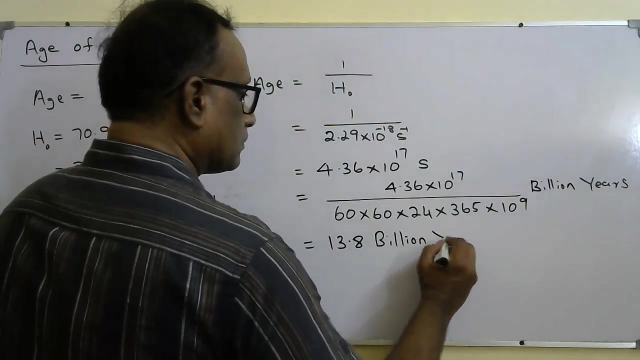 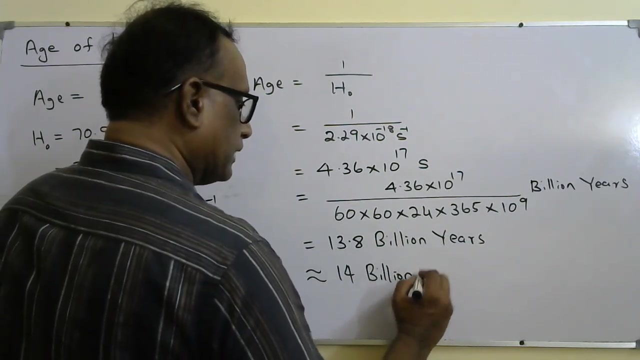 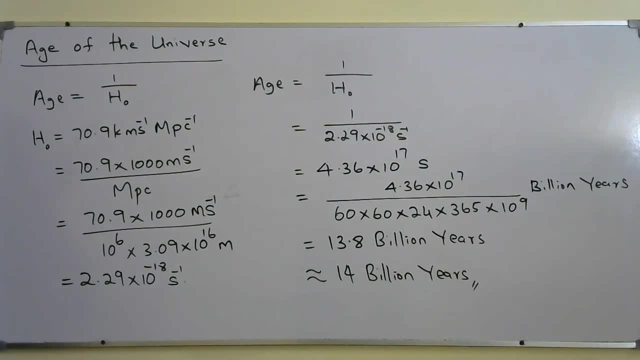 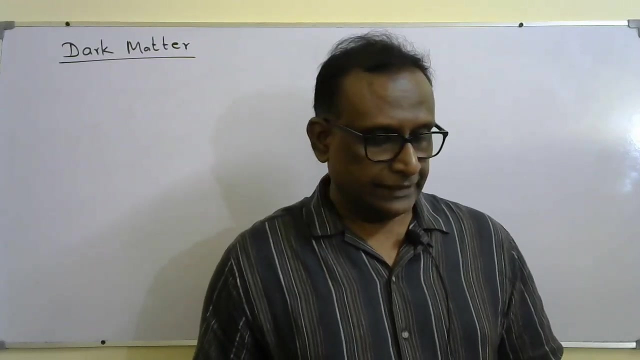 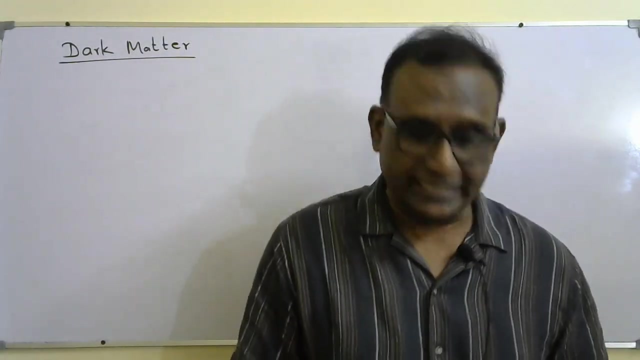 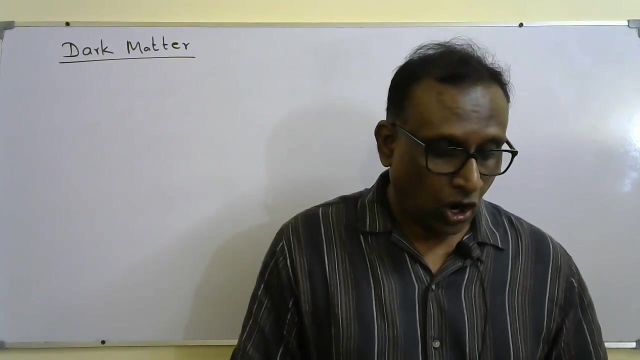 We can ask this calculation. Okay, so the next topic is dark matter. So what is dark matter? It means it's a compost of particles that do not interact with electromagnetic radiation. Or you can say dark matter is a compost of particles that do not absorb or reflect, or 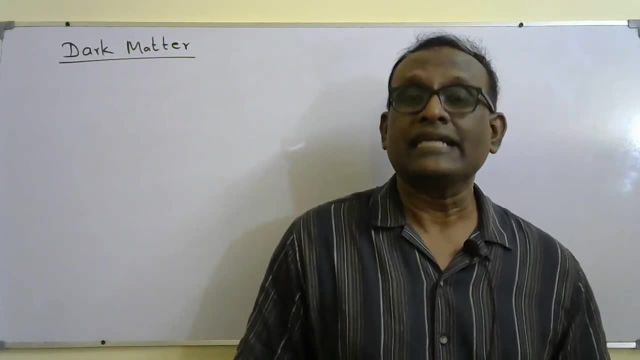 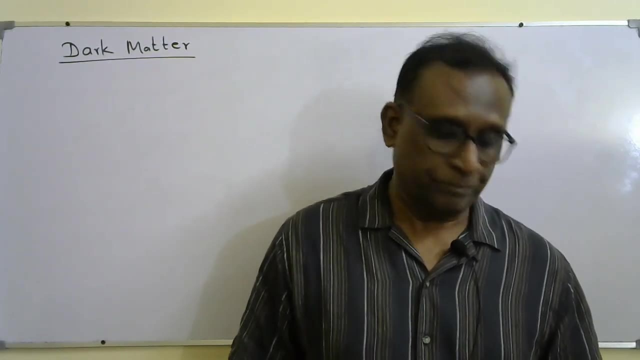 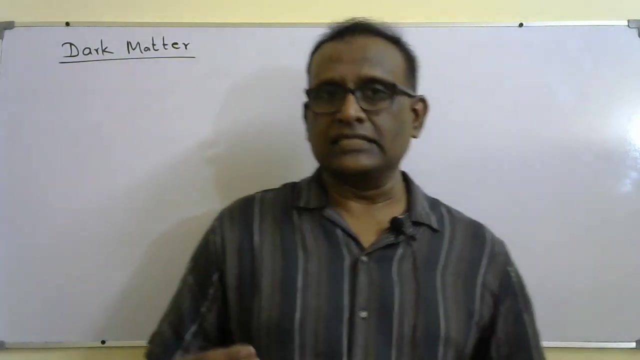 emit any electromagnetic radiation, but it can interact gravitational, by using gravitational field, with other matter. that is the dark matter. Okay, so what is the evidence for dark matter? So you should be able to understand the meaning of dark matter. It's a compost of particle. 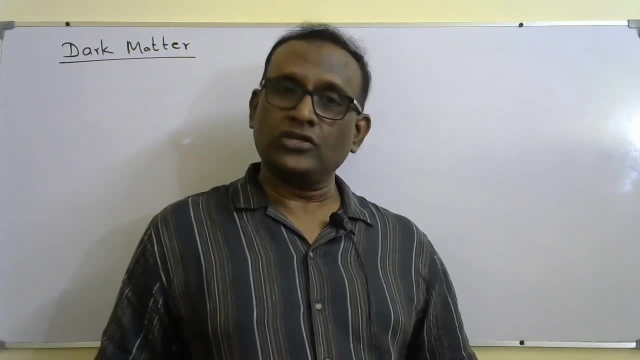 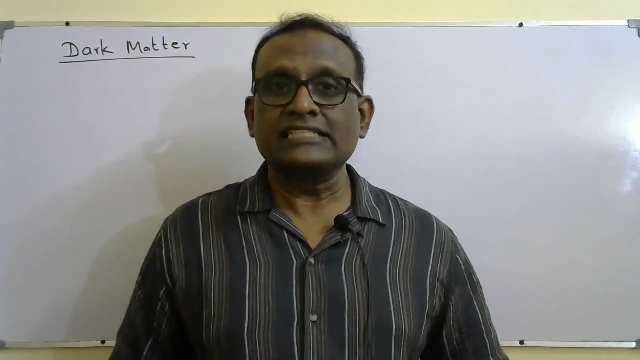 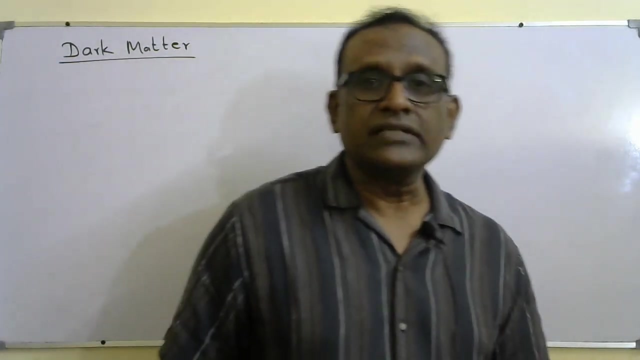 It does not interact with electromagnetic radiation. Or you can say it does not emit or absorb or reflect any electromagnetic radiation, but it has gravitational interaction with other matter. So what is the evidence for dark matter? So this is the evidence for dark matter. It's like this. 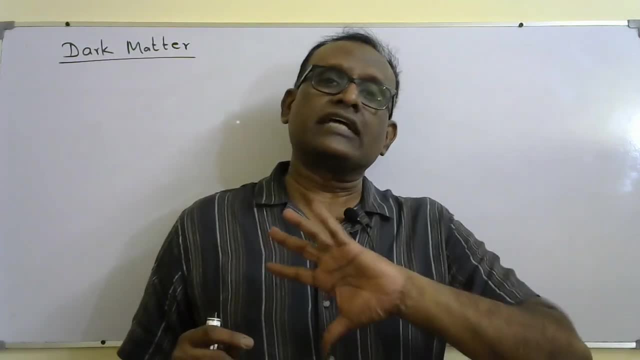 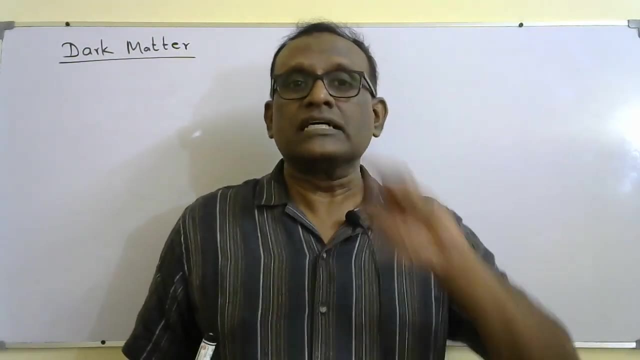 You know, when you consider a particular galaxy, most of the galaxies, at the center there is a black hole And most of the stars are spiraling around the nebula. The nucleus of the galaxy, Nucleus of the galaxy, is the center part of the galaxy. When you consider a galaxy, most of the stars in the galaxy are concentrated closer to the nucleus. The other stars are highly spread out in the outer region of the nucleus. So when we consider a galaxy, for example, this is the nucleus of the galaxy. 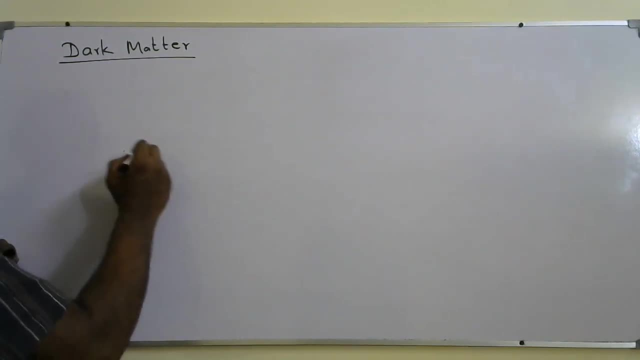 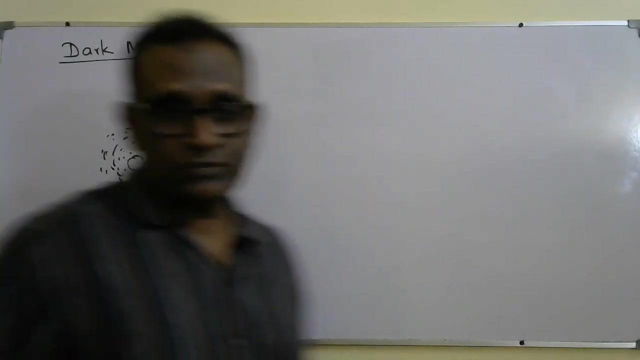 There will be a black hole And most of the stars are very closer to the center of the galaxy, of the galaxy. So we can assume most of the mass of the galaxy is concentrated at the center of the galaxy. We can assume most of the mass of the galaxy is concentrated at the center of the galaxy. 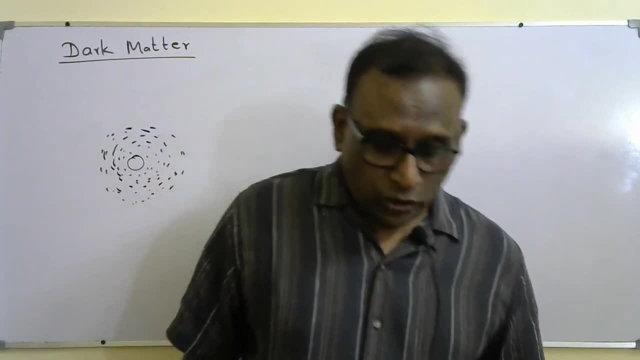 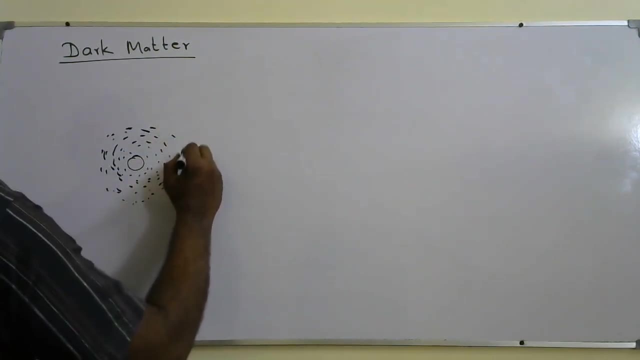 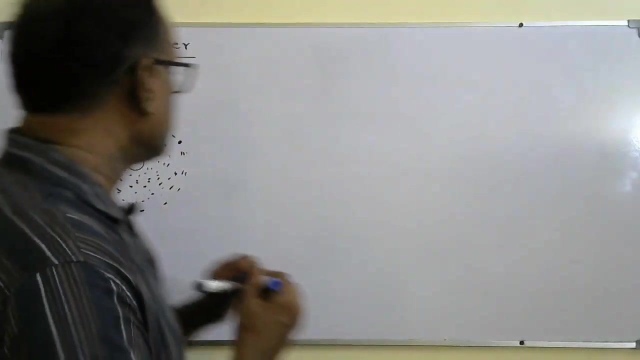 due to visible matter such as stars. Okay, so we know that in gravitational field, you would have learned. when a star moves around a galaxy, it moves due to the gravitational force acting on it. The gravitational force acting on it is the f equal g mm over r squared. We can see the 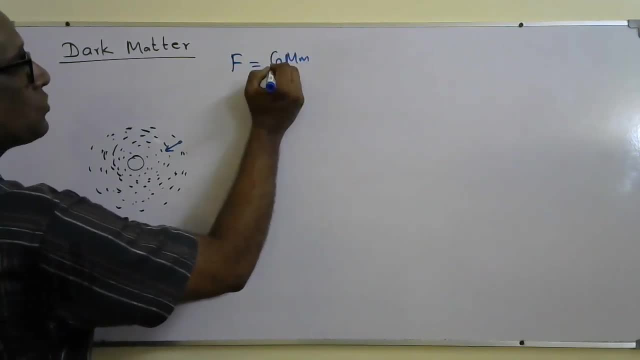 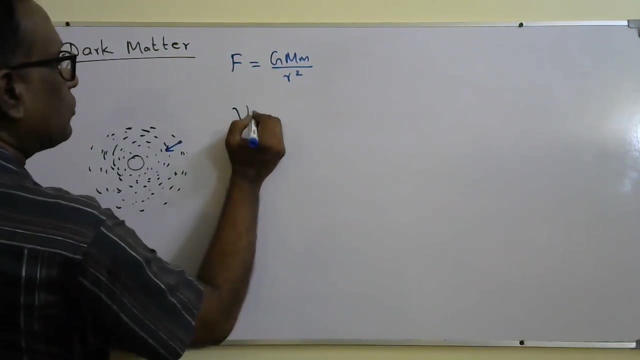 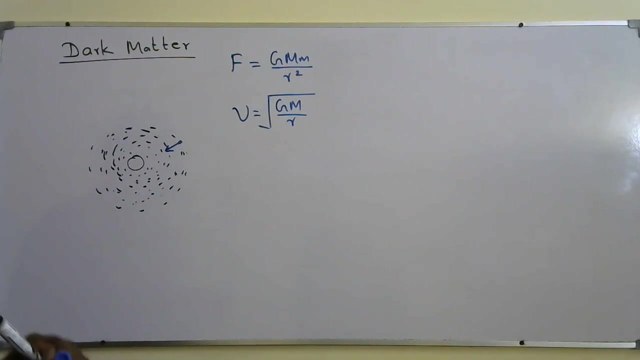 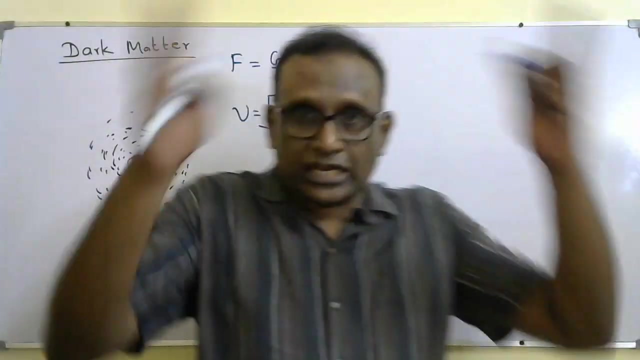 gravitational force f equal g mm over r squared and the speed of the star when it orbits the nucleus of the galaxy is given by: v equals square root of g m over r squared, Where m is the mass enclosed within the spherical path. You know the star is moving on a circular. 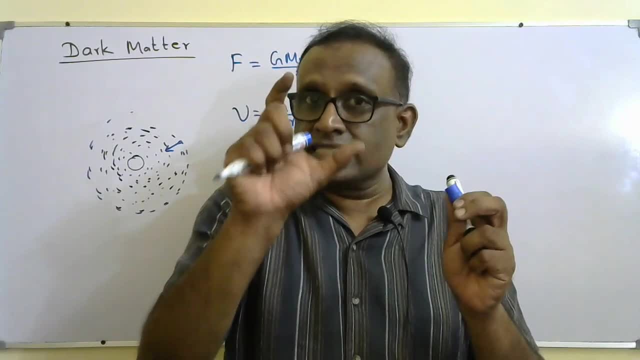 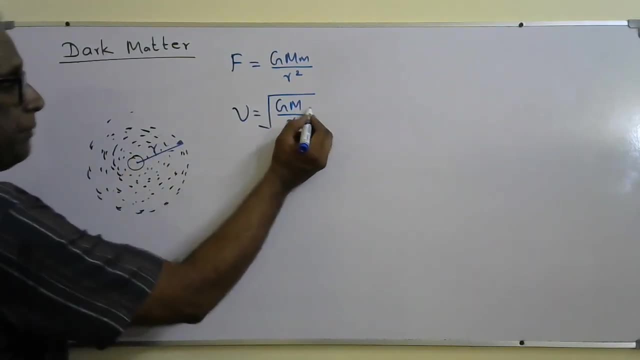 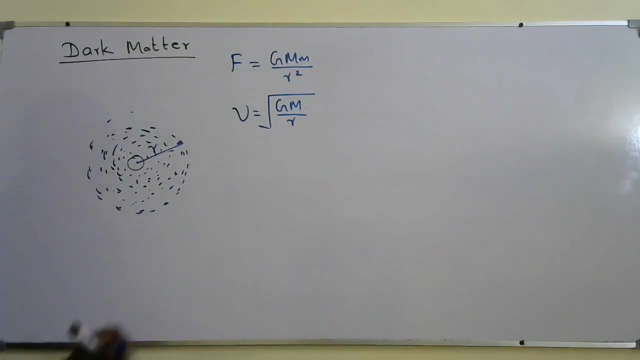 path. We can assume a sphere of the radius or the distance r of the star from the center of the galaxy. If I say that distance is r, So m is the mass of the stars enclosed within the sphere which has radius r. It's actually Gaussian. 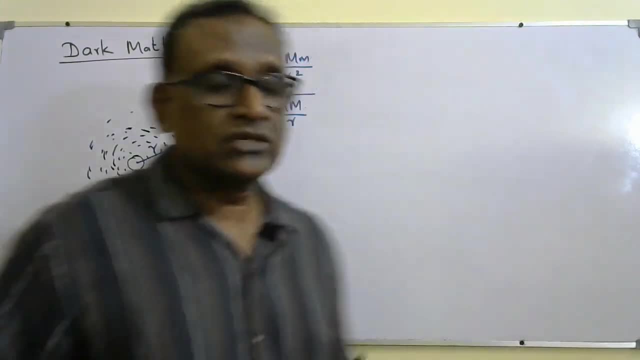 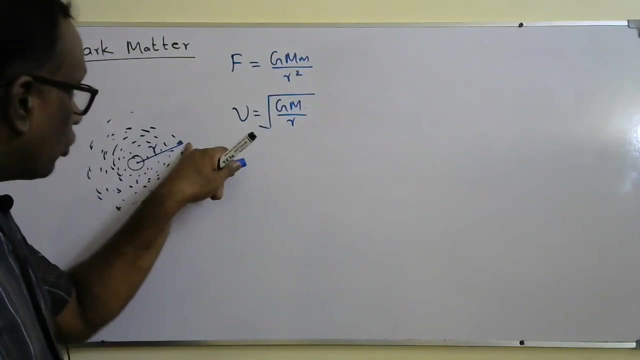 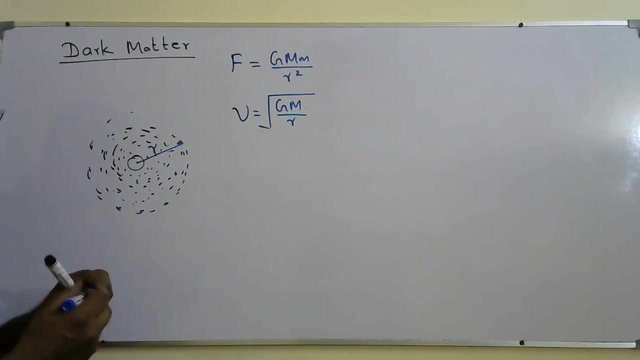 But the word Gaussian law is not in your syllabus. So Gaussian law says m is the mass enclosed within the region occupied by the motion of the star. So that is the m. Okay, so what observation they made? I told that most of the mass of a galaxy are concentrated closer to the nucleus of the galaxy. 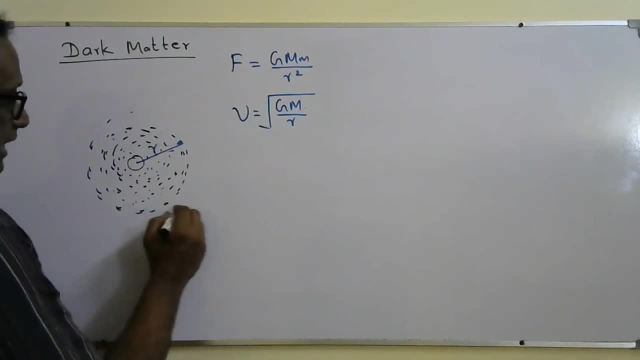 So when we consider n, the star, which is far away from the nucleus, the radius of the star is larger And its speed, when we consider So its speed should be given by v, equals square root of g, m over r here. So you can argue: the radius of the star is larger, So it might include more mass. But that's not the case. 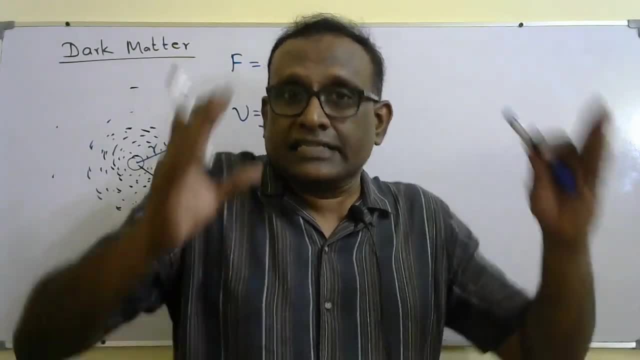 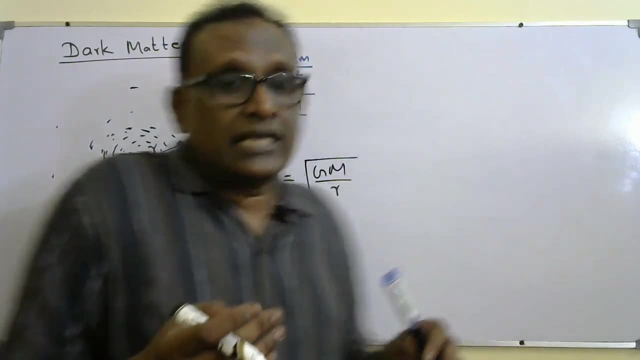 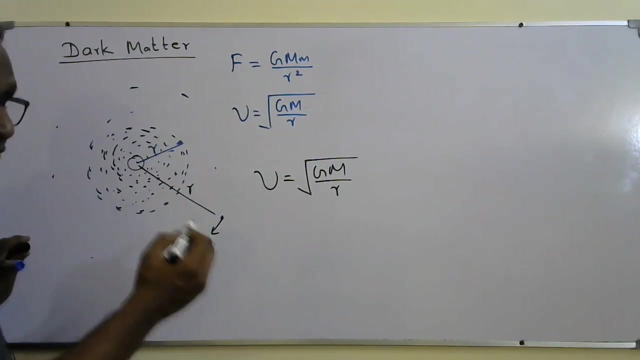 Because most of the mass is concentrated near to the nucleus. So that's no That most of the mass means the mass due to the visible matter Stars enclosed within the, within the or closer to the nucleus. So the mass enclosed due to the visible. 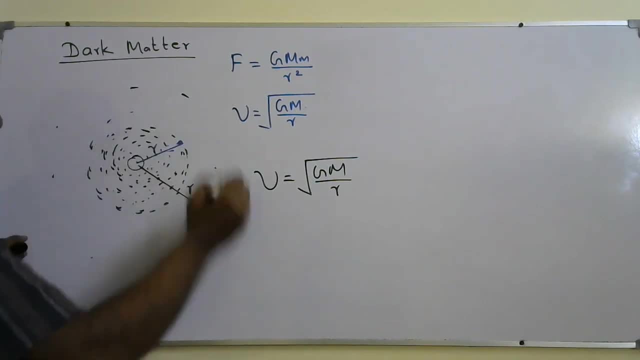 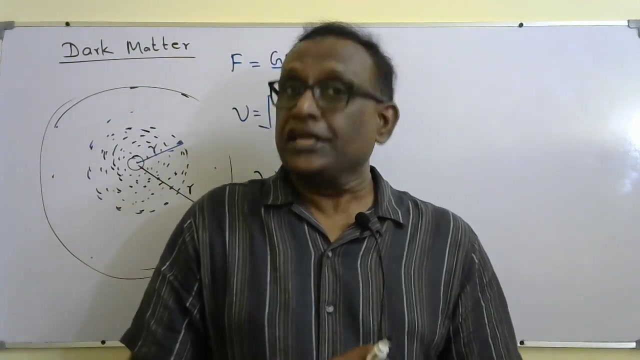 stars within this sphere or within this sphere is almost same, There's no big difference. The mass enclosed within this sphere or this sphere should be almost same, because most of the visible stars are concentrated closer to the nucleus or closer to the center of the galaxy. So when we think about this speed, we 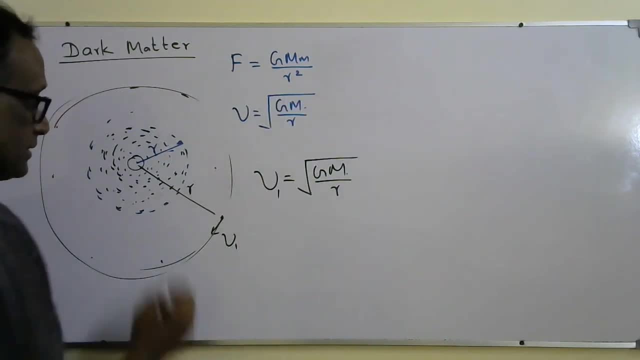 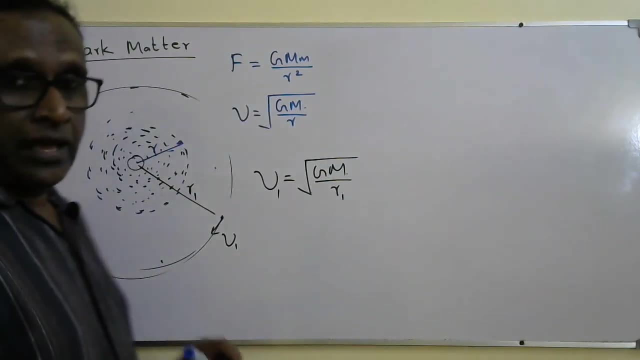 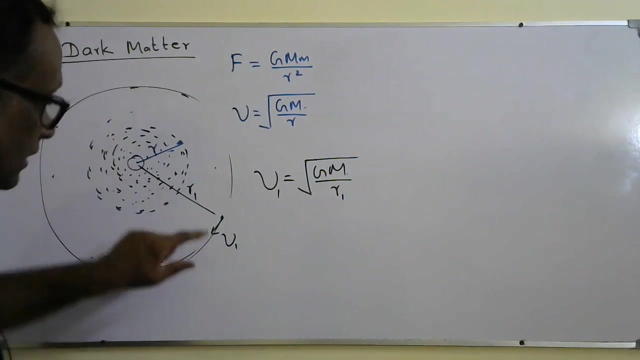 want where the mass is same as this mass but the distance. r1 is larger, so this star should have lower speed. But when they measured by using satellites, when the scientists measured the speed of a star in a far distance from the nucleus of the galaxy, they found the speed v1 and speed v are almost the same. 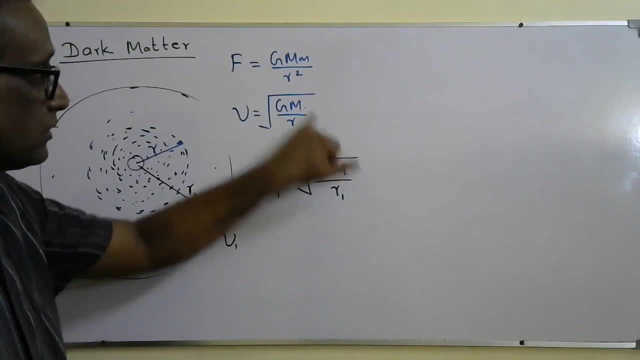 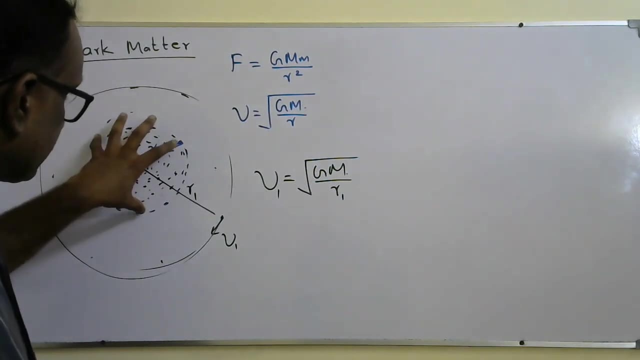 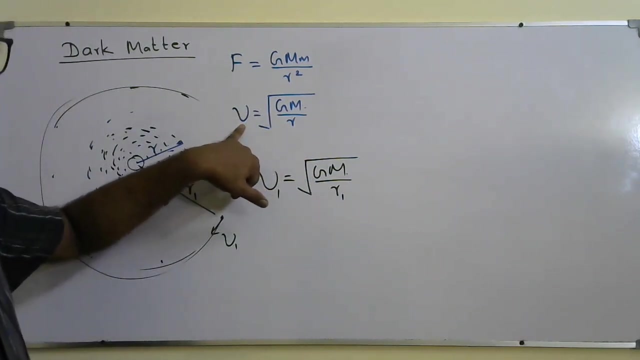 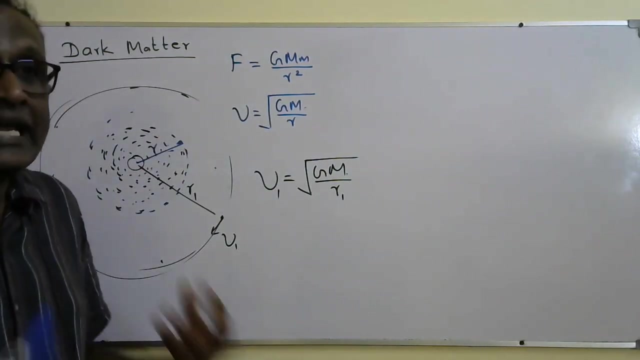 There are arguments that the mass should not have very big difference in terms of visible stars, because most of the stars are concentrated closer to the nucleus. but r1 is much larger than r, so v1 should be much smaller than v. But when they measured v1, they observed v1 is almost equal to v. How is it possible, Then they 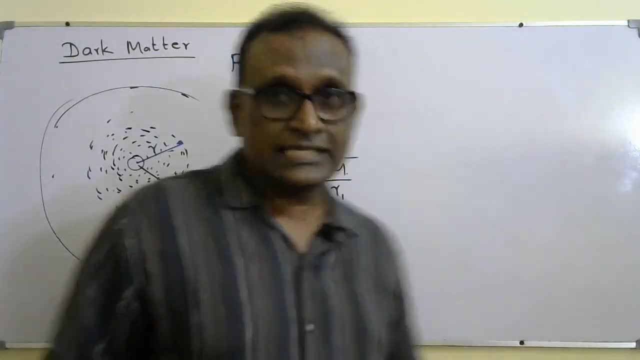 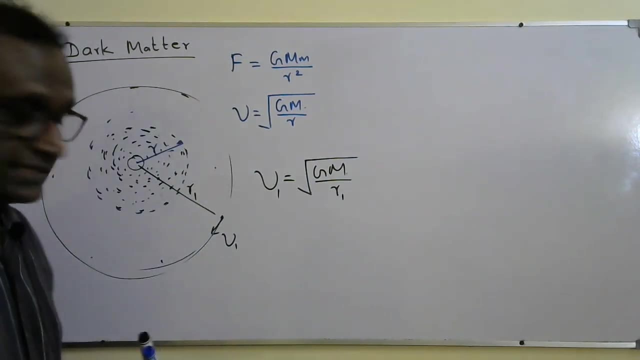 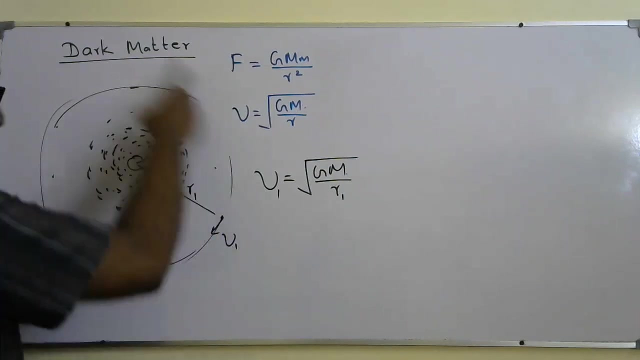 gave a conclusion. The only possible conclusion we can say here is: okay, the mass of the particles that is placed, given as the decomposited mass should be, ág begins to creating a new mass and v is equal to the mass that is in the center of the quarter ofечатwald. but when we consider a star, 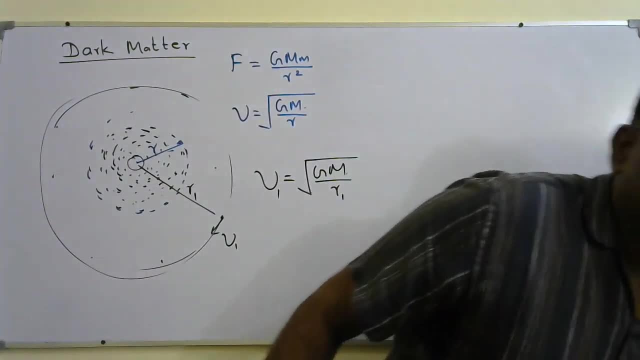 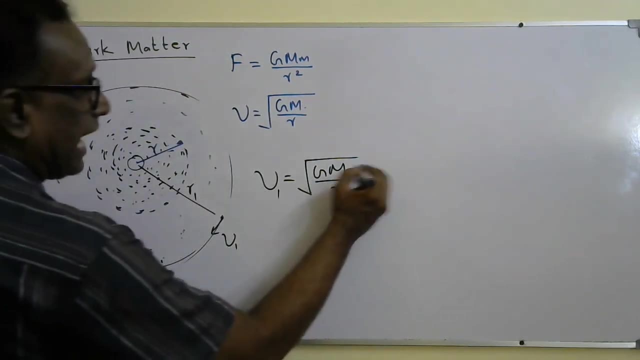 which is канале, organization of theCIoseronics, a star that is having the realistic mediums. here we get aค square mass And r1 is equal directly between these two. now theع developing the s Kant eigen walkusting in our property is a. 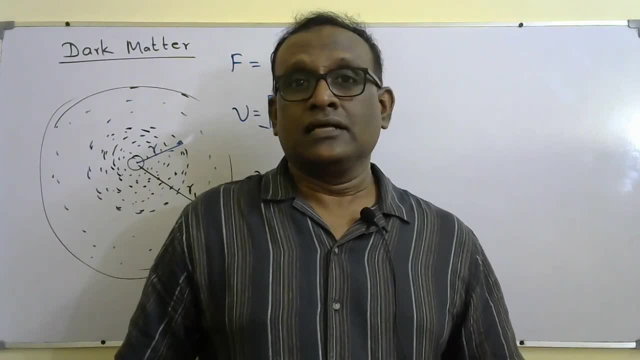 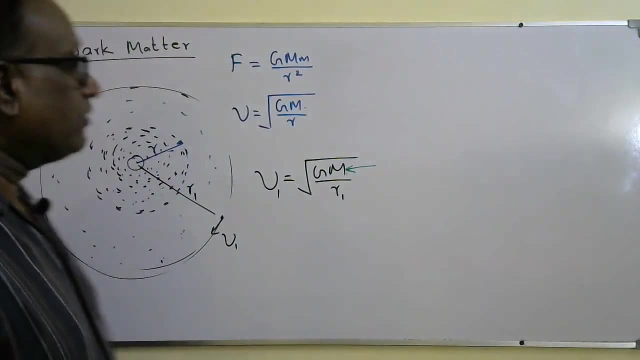 renumeration of number 1, that else there is no in the sking. But iflight alien producto g datos, which means e1 and v becomes the same data, and they Жsenad that mass is due to dark matter. okay, so that's the only evidence scientists have. 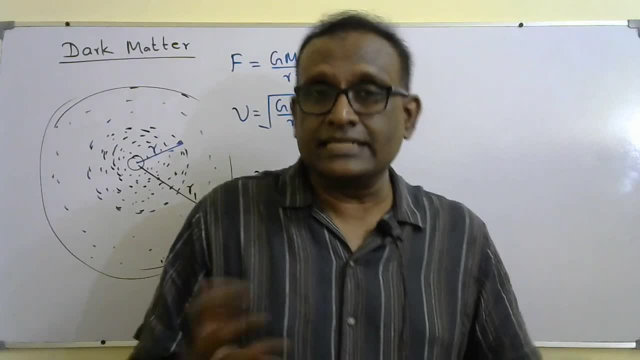 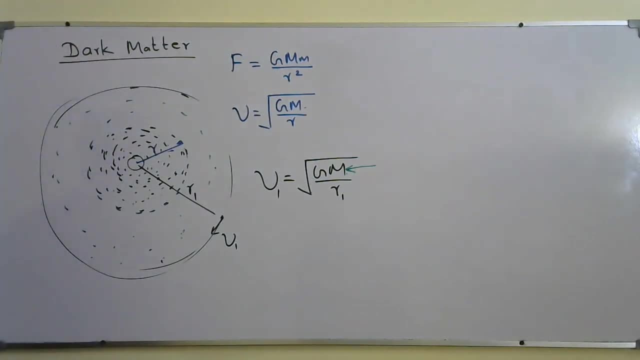 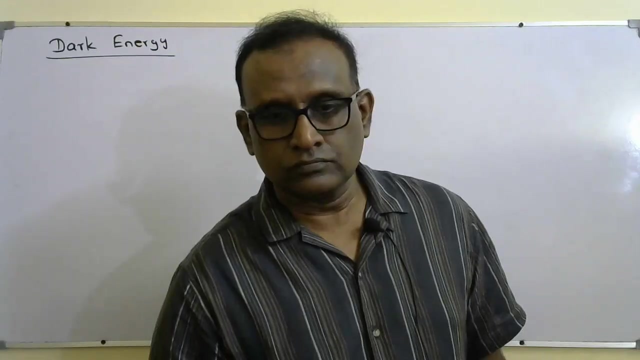 but there's one more evidence about gravitational lensing, not in your syllabus, but in your syllabus. this is the only evidence we talk. so this is the evidence we can tell in your syllabus to show the existence of dark matter. okay, what is dark energy? okay, so what's the evidence of dark energy? you know all the. 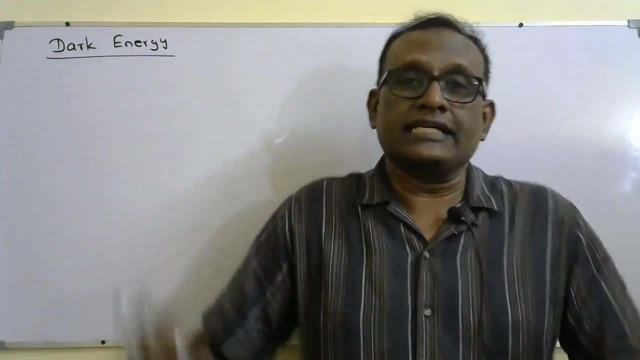 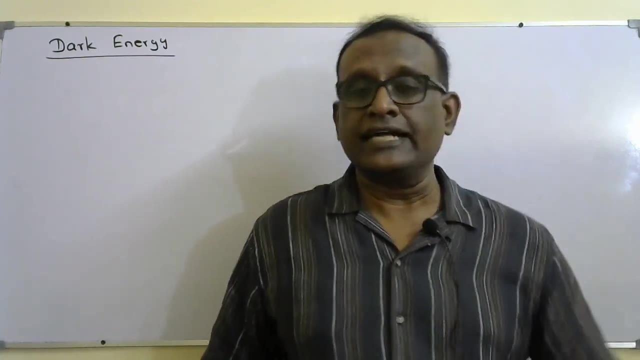 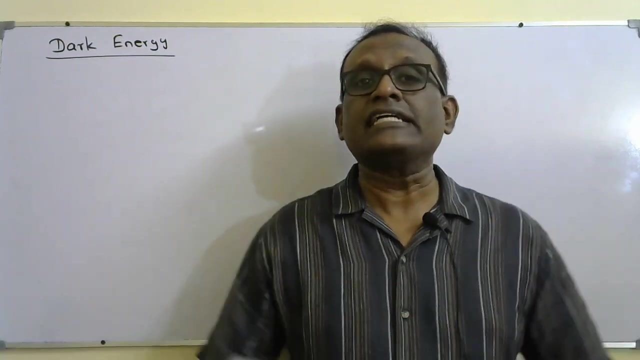 galaxies are receding from each other or receding from us. moving away from us, we have the Doppler effect equation: there's a red shift in the absorption line, so they are moving away from us. but even when they are moving away from each other, there must be gravitational pull towards each other, so they should slow down. they. 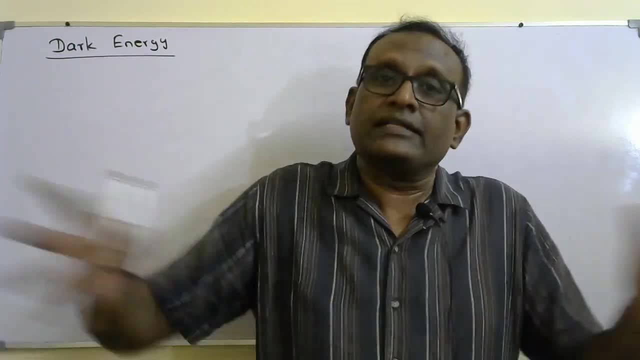 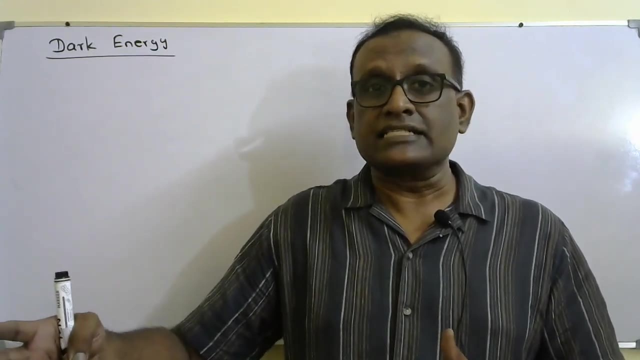 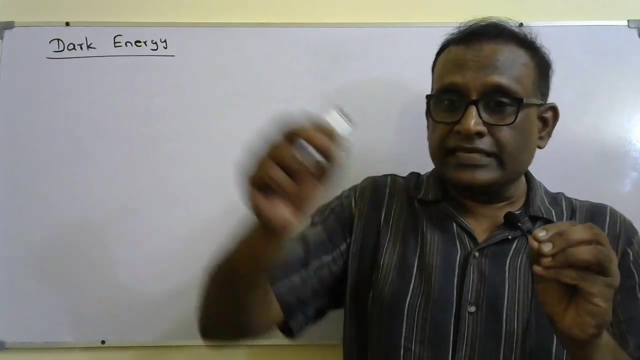 experience gravitational force towards each other, even when they are expanding. but we know that according to Hubble's law v equal H, naught d, the distance increases, their velocity is increasing. that means when a galaxy is at a particular distance today, maybe after a few years, when the galaxy 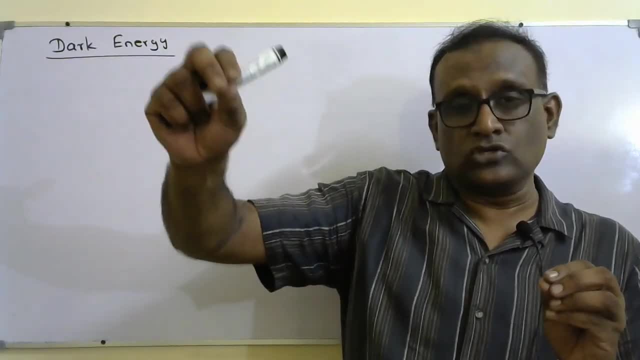 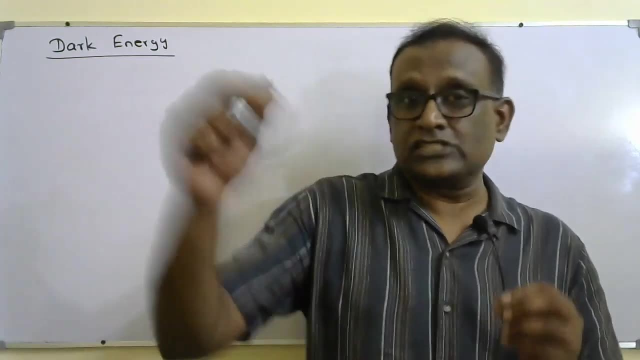 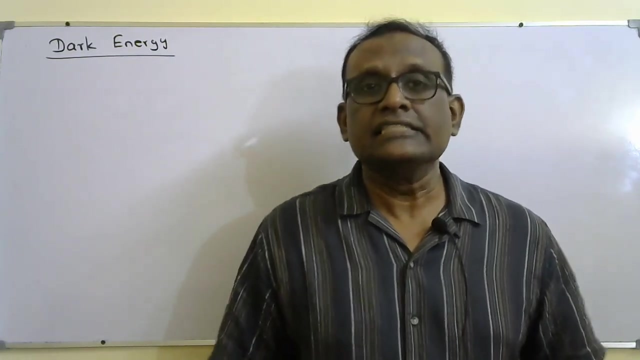 comes to this position, or after millions of years. when the galaxy goes to this position, the speed is increasing, even when it has gravitational pull towards each other, which is opposite to the motion motion of expansion. so how is it going to work? how is it possible? from where are they getting the energy for acceleration? they 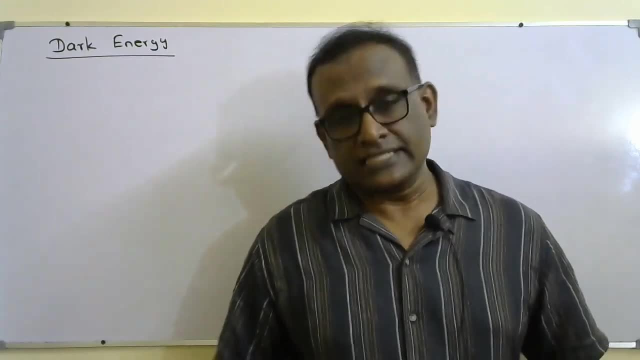 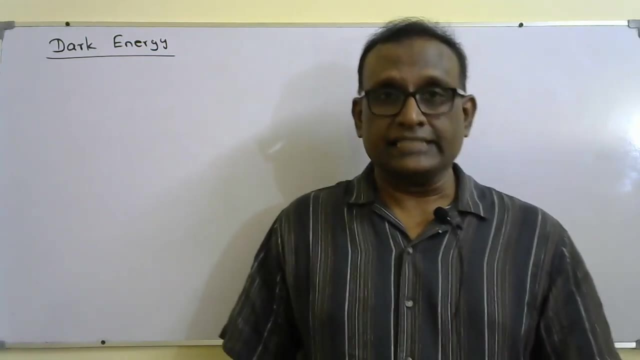 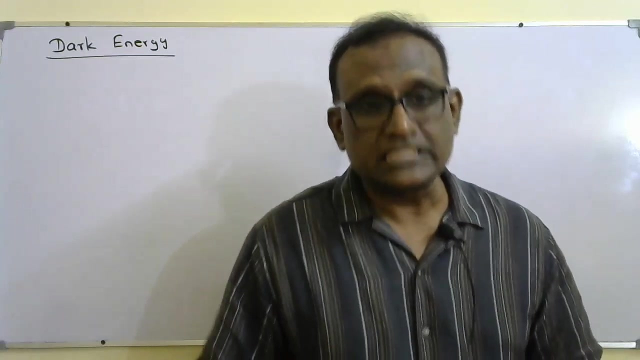 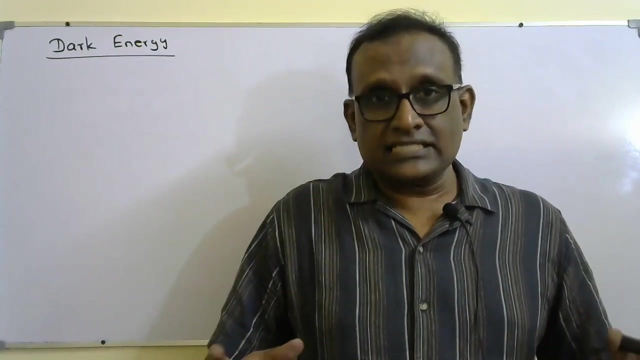 are gain in energy, gain in kinetic energy. so it's another puzzle. so this energy increase in velocity is due to unknown energy which is filling the distance or filling the region between the galaxies. that energy is called dark energy. so dark energy is the energy which is accelerating the galaxies to 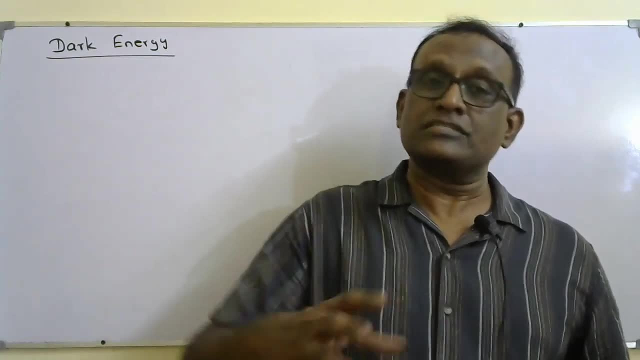 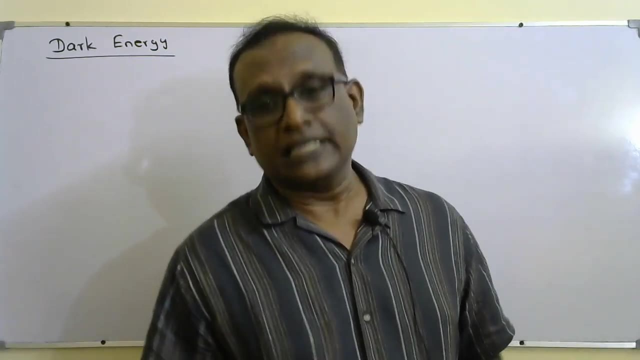 move away from the galaxy and the galaxy is moving away from the galaxy and the galaxy is moving away from each other such that their velocity or speed increases. the evidence for increasing speed is the Hubble law, that is, the dark energy. okay, so very common question. friends ask you know we learned? 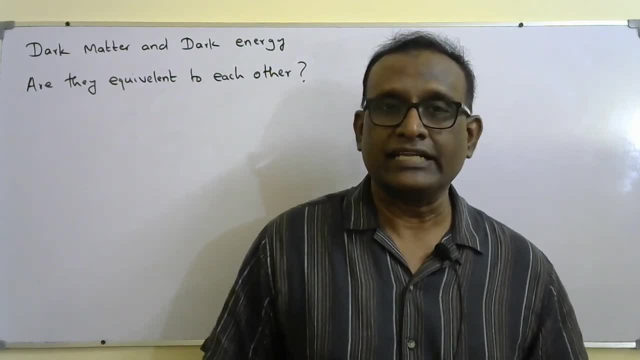 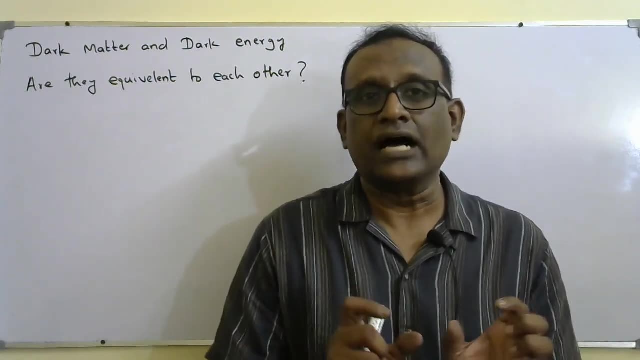 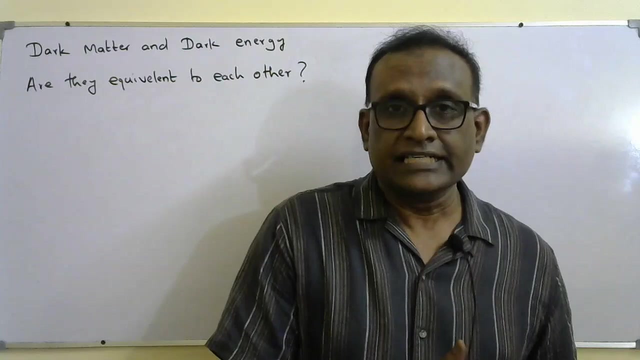 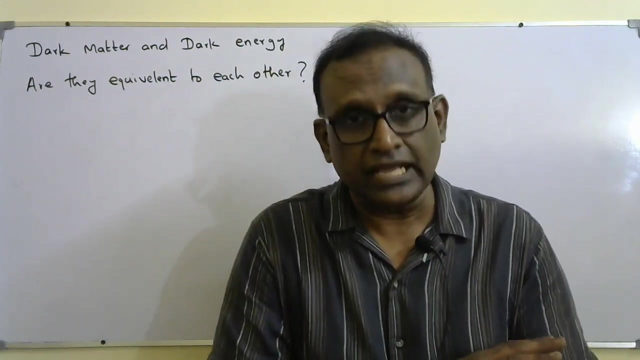 that in unit four, according to special theory of relativity, mass has equal energy, energy has equal and mass. so dark matter, dark energy, the word dark is the same, but one is matter, the other one is energy. so students normally they ask: is the dark energy is equivalent of the dark matter, or is the dark matter is equivalent of the dark energy? no, they are completely two different things. one is dark matter that exists within the galaxies that provides gravitational effect, that provides gravitational pull to matter which has no interaction with electromagnetic radiation. but dark energy exists between the galaxies which provides the energy for acceleration of the galaxies. so they are two complete different. 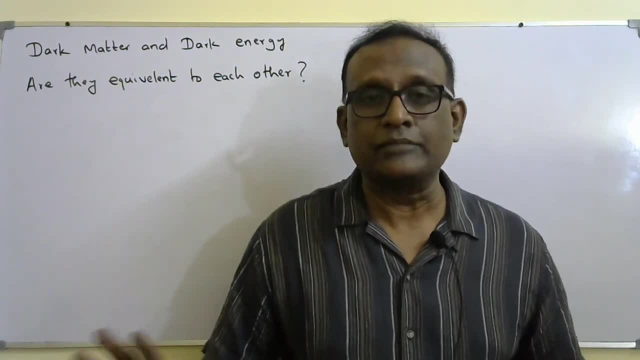 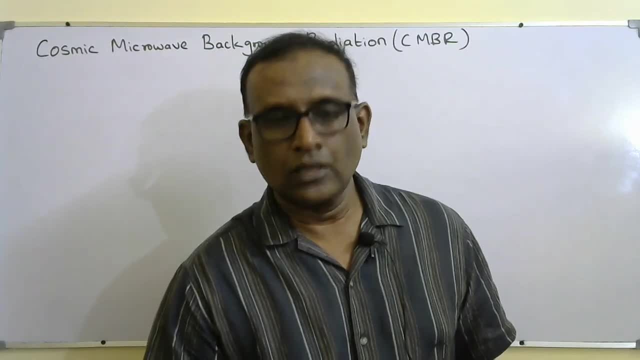 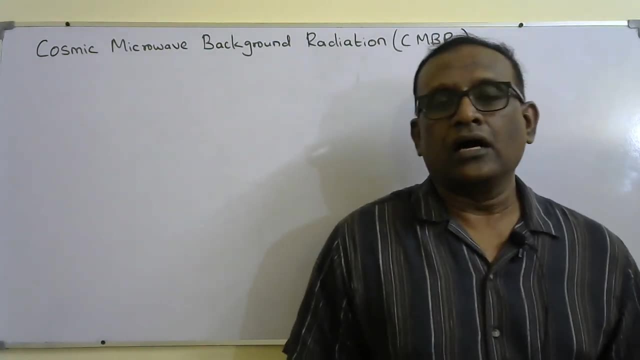 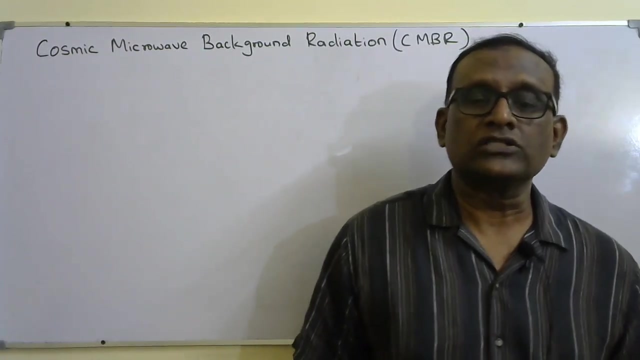 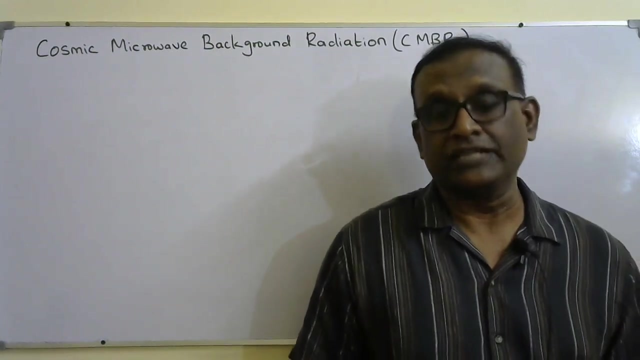 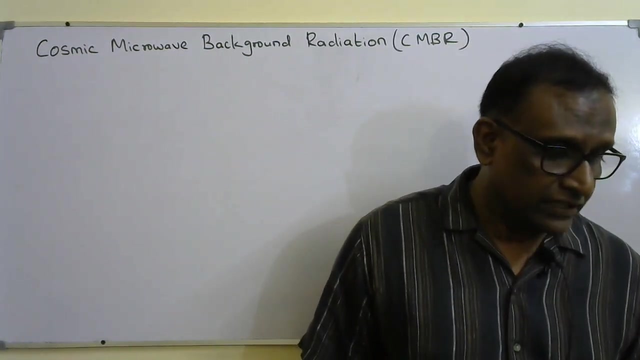 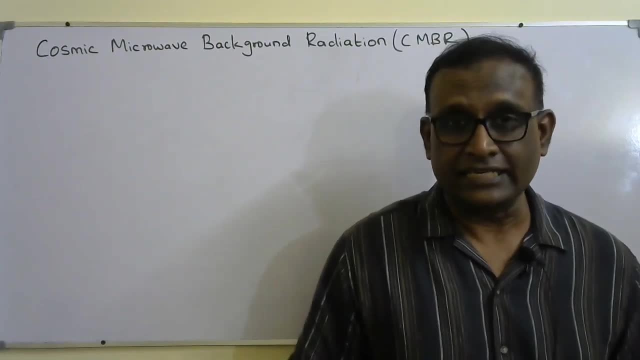 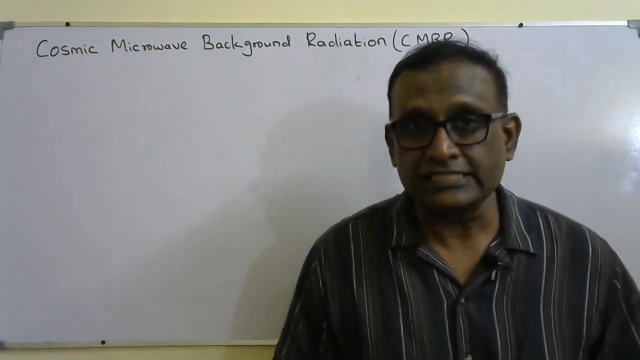 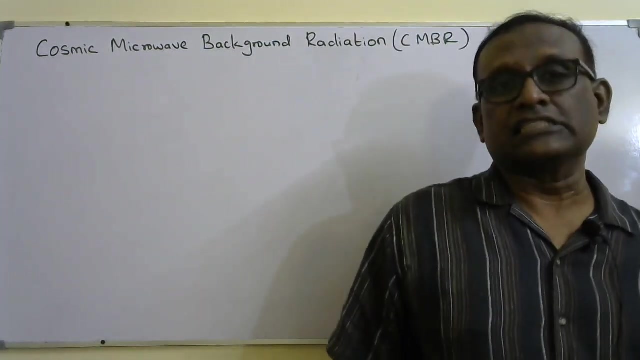 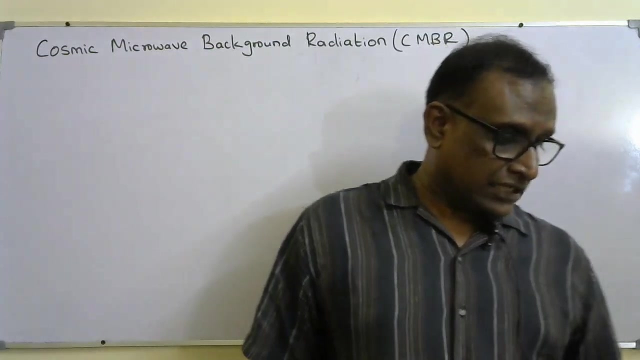 they found it was. it had the same intensity all part of the sky, all part of the earth, in different time, different locations. there is no difference in the intensity. so later scientists did research about it and they found that, according to big bang theory, uh, after the almost thirty eight thousand years, 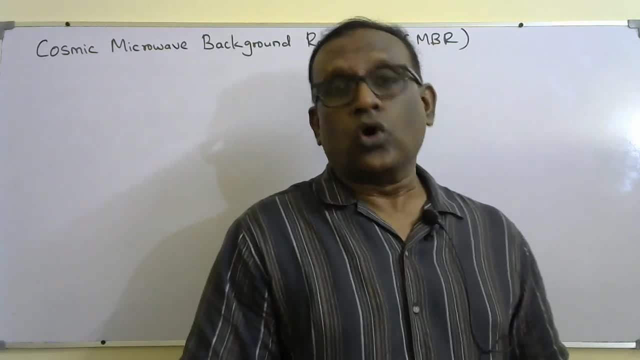 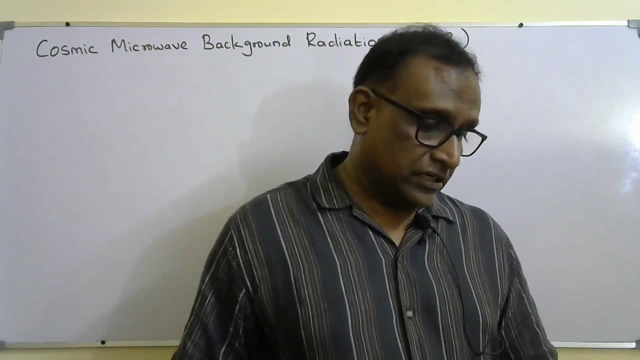 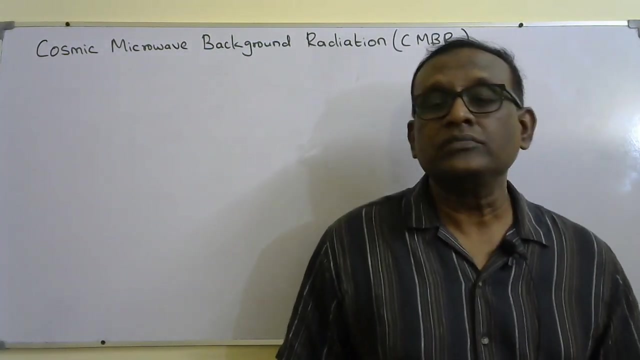 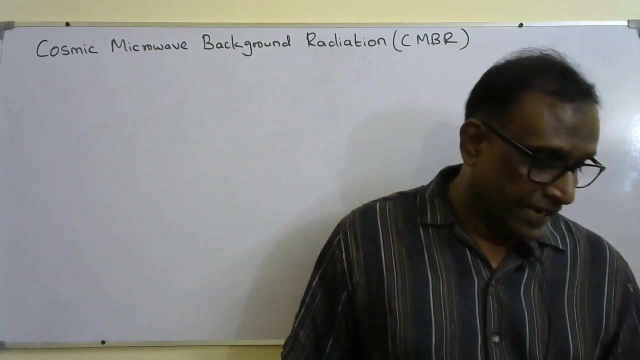 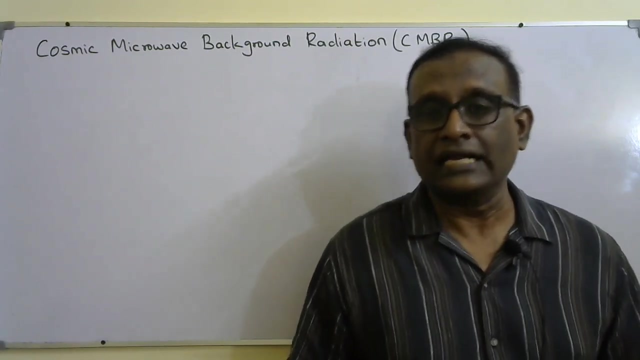 from the big bang, uh it. the universe war consists of uh uh. it consists of uh dense uh plasma. then, when it cooled down after three, thirty, eight thousand years, uh, it formed uh electrons and protons, but they coupled together strongly. but later, when the universe expand and cool down the these protons and electrons, they formed hydrogen atoms. 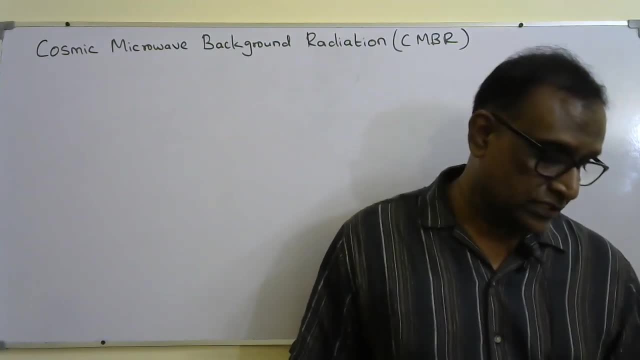 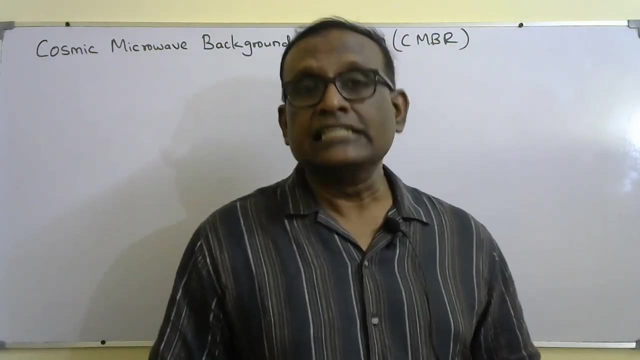 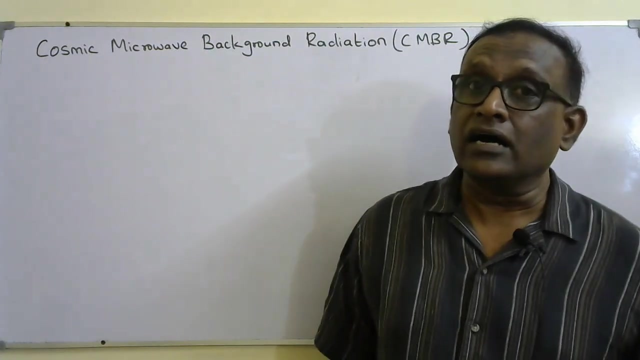 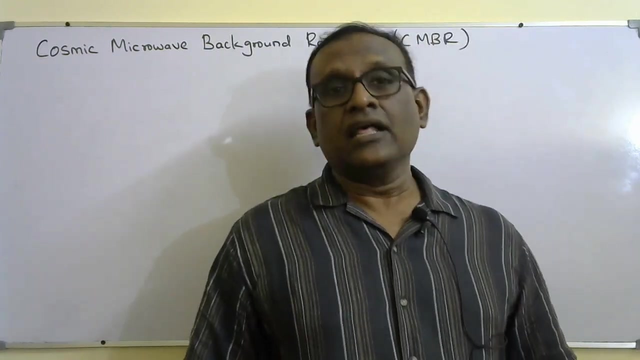 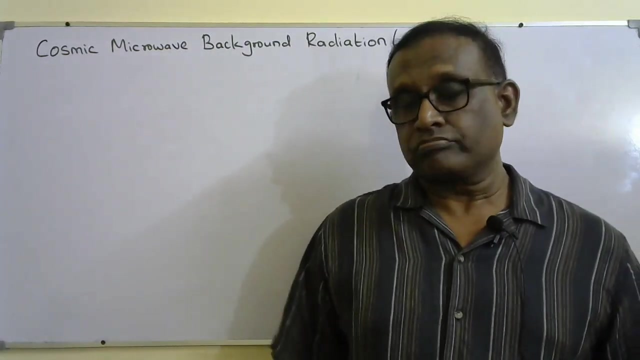 when these hydrogen atoms are formed. this process is called recombination. when these hydrogen atoms are formed from the protons and electrons, energy was released and that energy was initially, at that time, high radiation was with high energy radiation with high frequency. but when the universe expand further, the temperature decrease and the radiation now in the region of microwave. 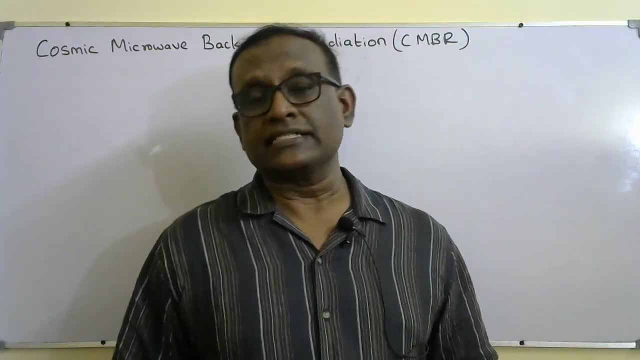 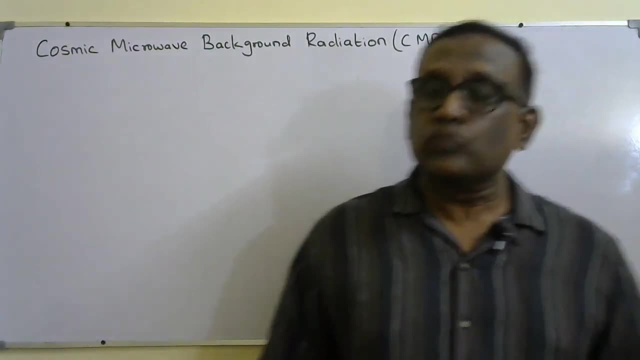 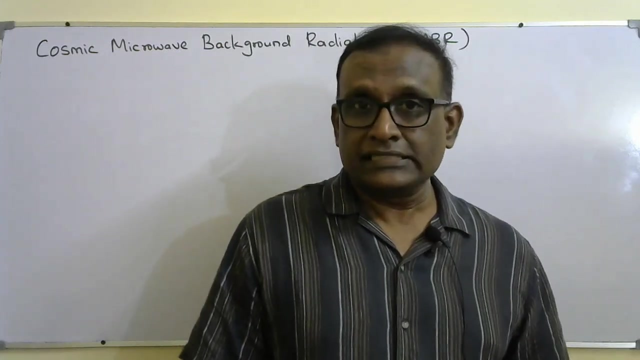 with a temperature of average temperature of 2.7 Kelvin. so what is the evidence of CMDR? so cosmic microwave background radiation is one of the evidence for Big Bang, in which initially it was a high-temperature plasma. because of the Big Bang, the universe is expanding and